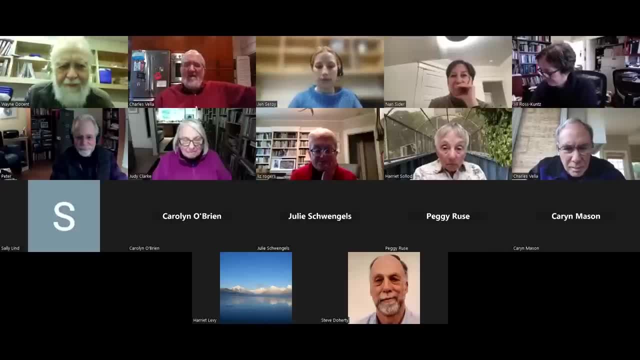 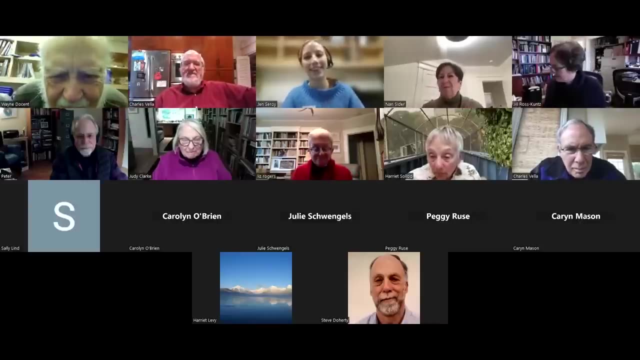 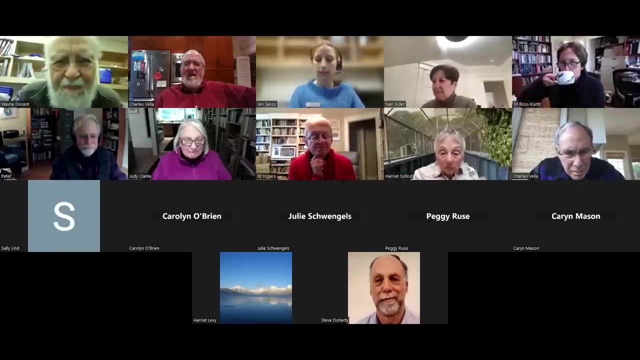 And I will continue. Oh, nice, Good call, And I'll continue admitting them in. But thank you guys all for being here And huge thank you to Charlie for putting this on, And Métis really was the one who arranged all this. So I'm just here to moderate, But a couple reminders. This: 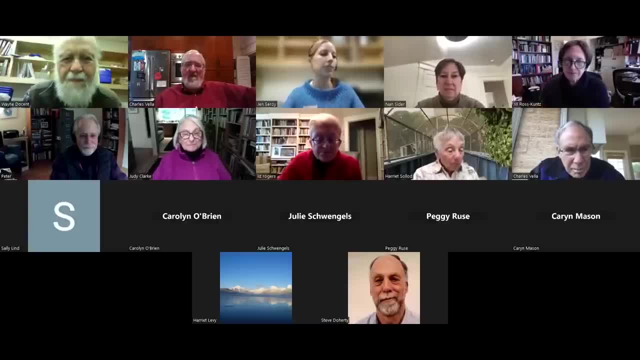 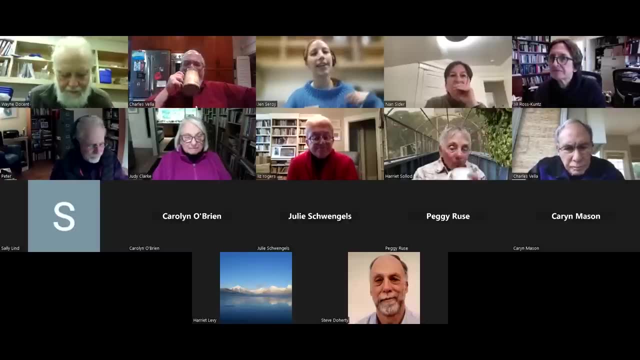 is not a training for Human Odyssey, So any docents who are not trained in Human Odyssey, this isn't like a training that means you can then engage in there. It is just a informational session to hear about some of the discoveries and all of the research that Charlie and his 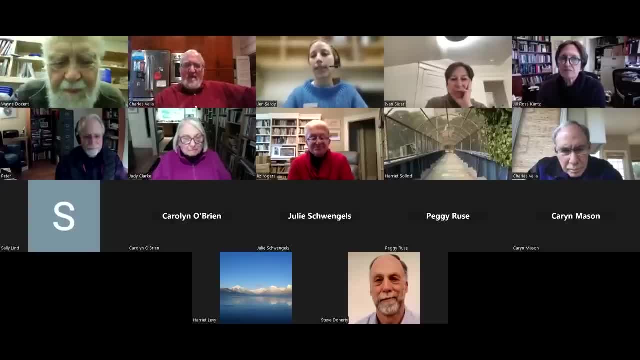 class and his people like to talk about. And then at the very end, if we have time, we can just have some like open discussion or questions and answers, But we won't be talking about the exhibit, the Human Odyssey exhibit. There are no, as far as I. 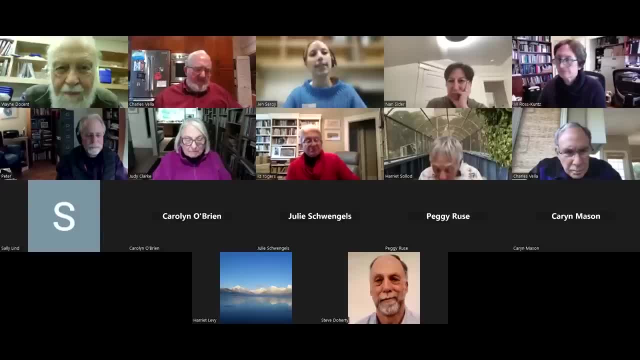 know there are no plans to update any parts of that exhibit, And so we're just going to leave that topic out of it. Jen, just a quick question: What's the time frame? How much time do we get with Charlie today? 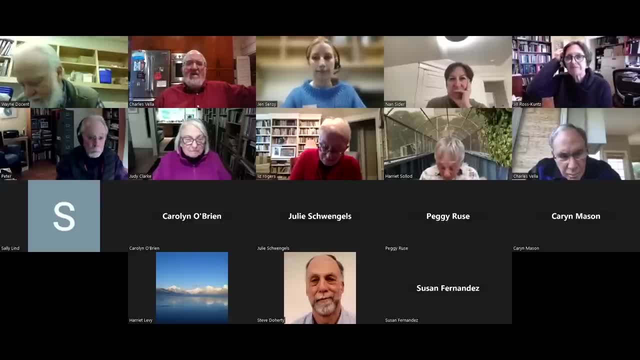 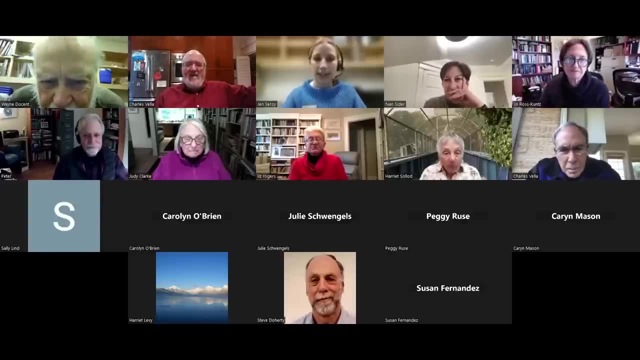 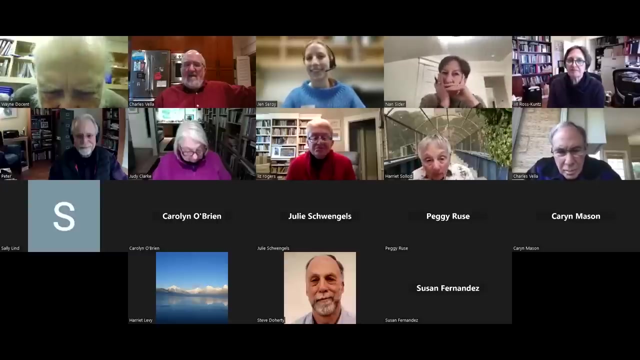 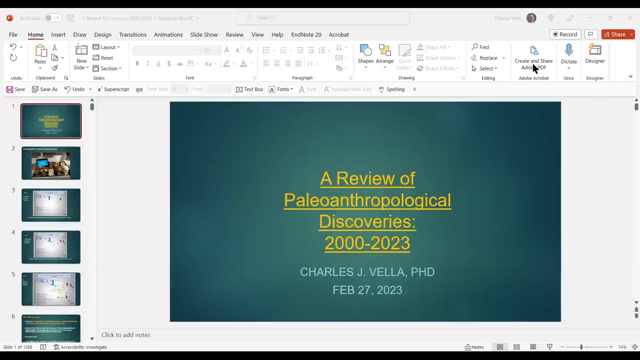 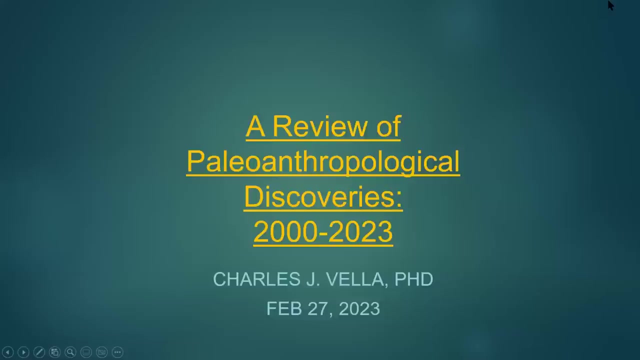 It is scheduled until 3 o'clock And with that, Charlie is still muted, but I'm going to hand it over to you. There he is Okay. Thank you, Can everybody hear me? Yes, Okay, And everybody can see a review of Paleoanthropological Discoveries. 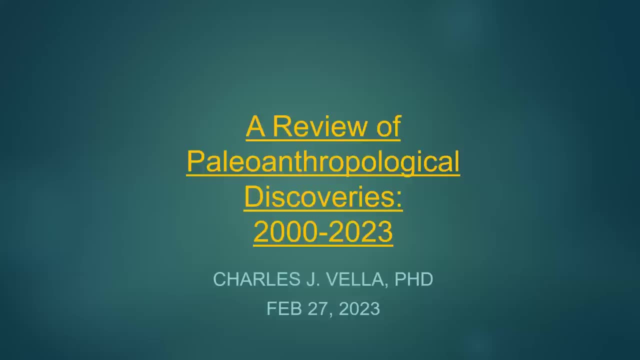 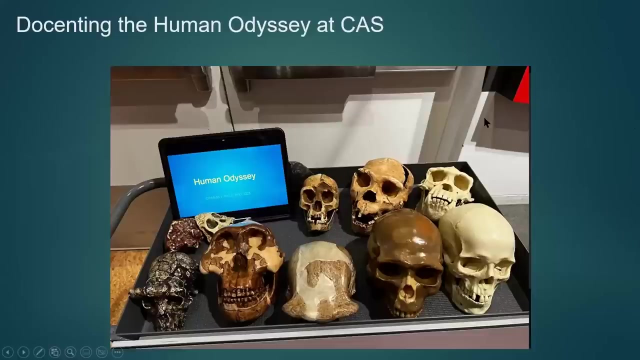 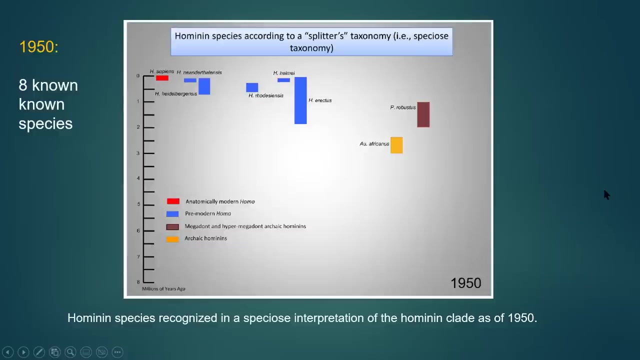 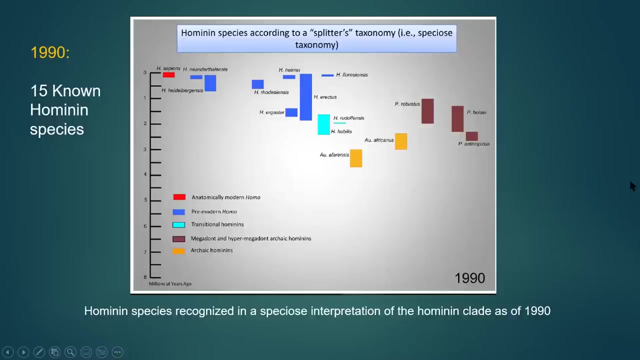 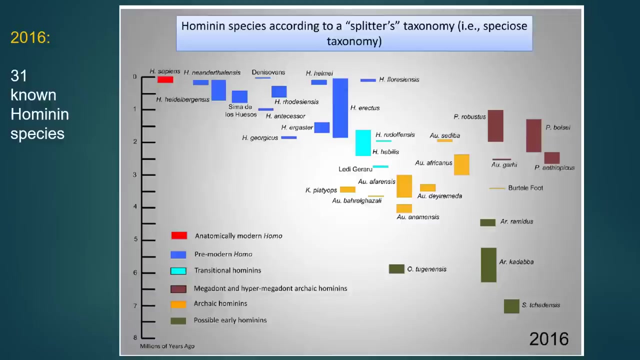 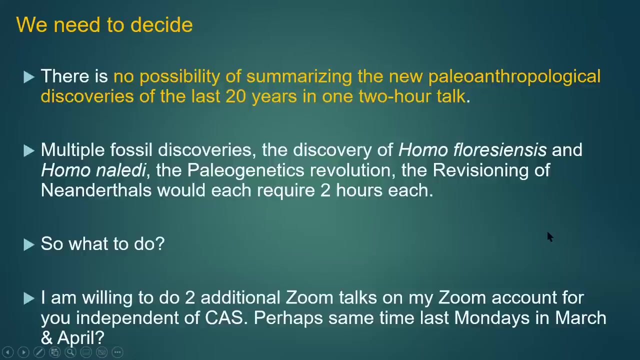 Yes, Okay, I'm going to hand it over to Charlie to offer two more two-hour talks to cover the paleogenetics evolution and the re-envisaging of Neanderthals. Possibly we can talk about it by email or somehow the same time in the last Mondays in March and April. it would be my suggestion, But I can only. 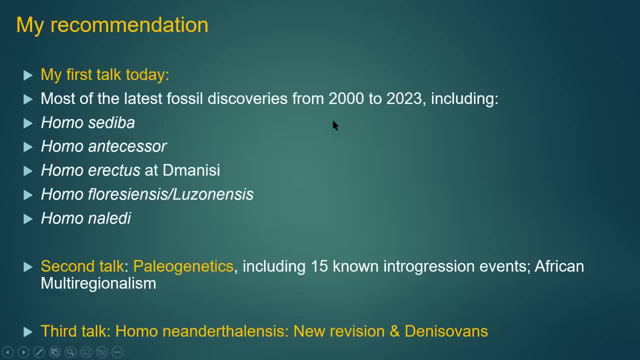 cover so much I have way too many slides even for this one. All right, Okay, So the next talk I want to do today is cover the big ones- at least name them- from Sediba, Flores, Nelidi, etc. And then the next talk would be on paleogenetics And the 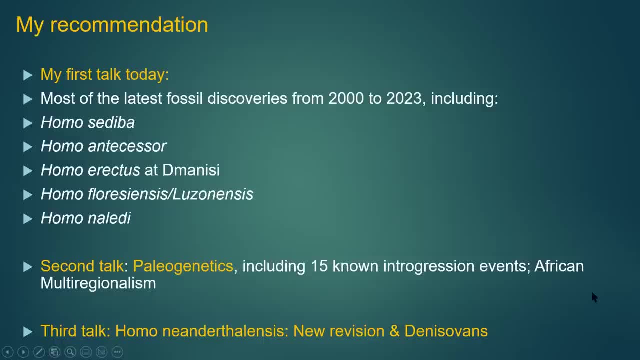 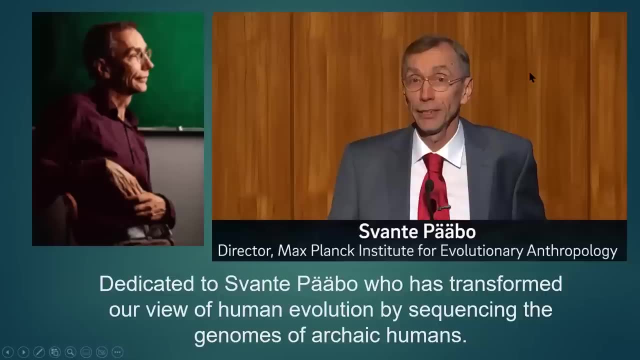 talk after that would be on Neanderthal, the new revision and Denisovans. okay, I want to dedicate this talk to Font Habo, who invented the field, basically, And I'm going to pass that on to Charlie, um and uh. so, uh, hello to him. um, who am i? just in case you don't know me, because i didn't recognize. 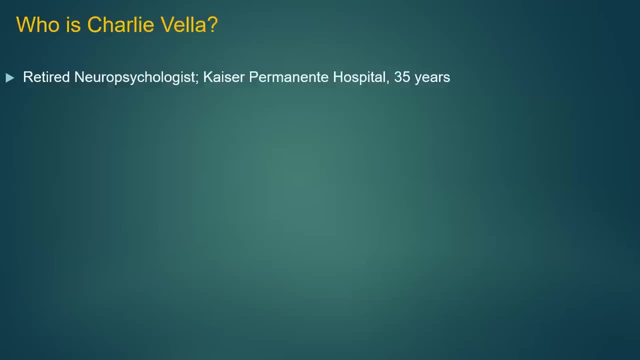 some of you there, i'm a retired neuropsychologist. i worked in psychiatry for 35 years. you would not want to see me professionally because it meant something was not working right with your brain. i started docenting um uh, sorting freshwater snails uh downstairs in 2009 and then went. 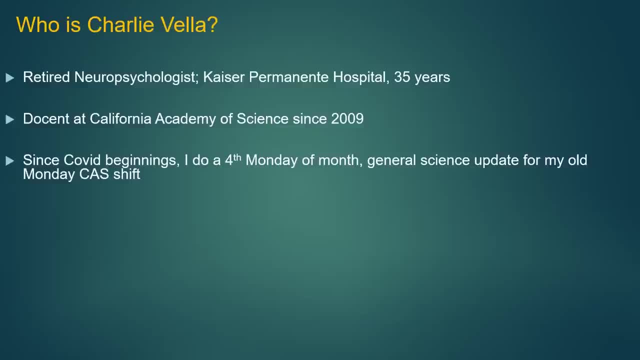 upstairs to start human odyssey. uh, since covid beginning, i do a fourth monday of the month with um. uh, cast staff um up doing a general science update. you're welcome to join that if you want. and since 2019, um, i've been teaching a two-hour once a month class for san francisco states only on their human 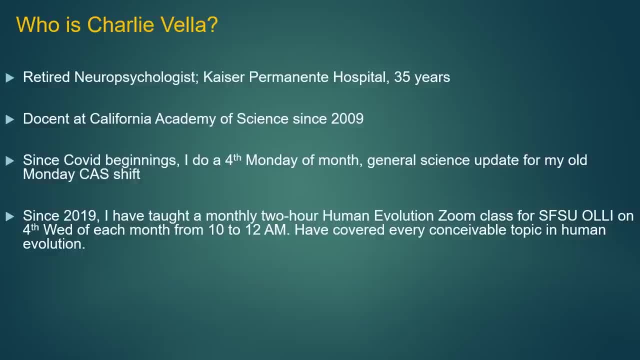 evolution interest group. you can join that, but you have to pitch in 50 bucks a year for that. all prior 45 two-hour lectures are downloadable at my website. okay, if you're um interested, and i'll put this up on my website as well when we're over. uh, that's my 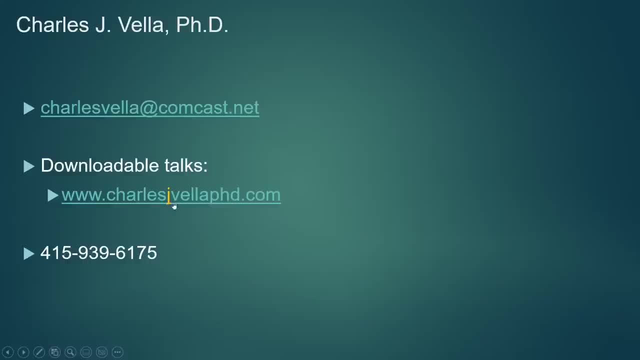 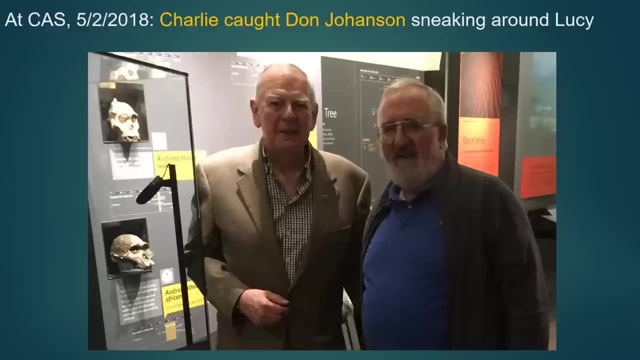 um. charles vela, comcastnet. charles j vela, phdcom. and there's my phone number. okay, um, i caught um don here. let me see if i can get rid of joe hansen sneaking around lucy at the academy in 2018. he didn't take it um and 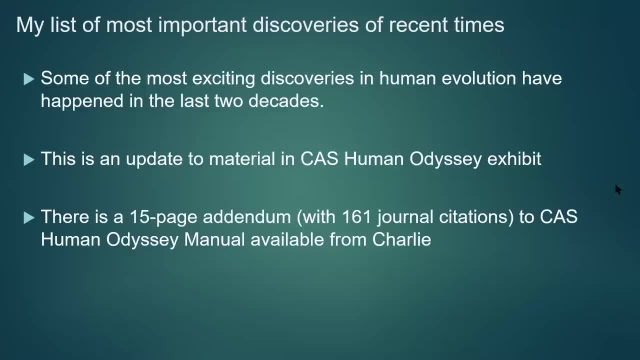 i'm not sure if i can get it to him. i'm going to have to go to him. but he's so i'm still not sure what he's doing. oh, go ahead and grab it, okay. i'm not sure if i can get it to him. i'm not sure if i can get it to him. i'm going to have to go to him. 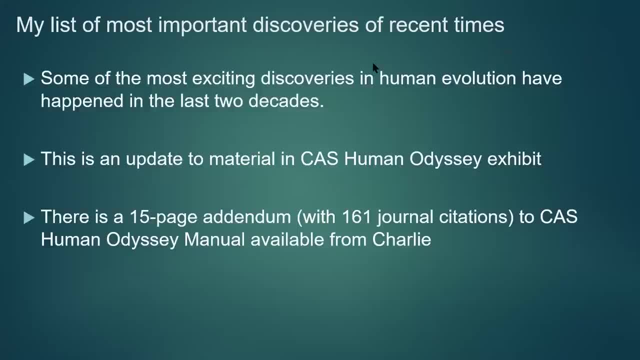 um. so some of the most exciting discoveries in human evolution have happened in the last 20 years. this is kind of an update to um material uh uh in the cast uh human odyssey exhibit. we're uh in the process of um completing a 50-year experience with uh human. 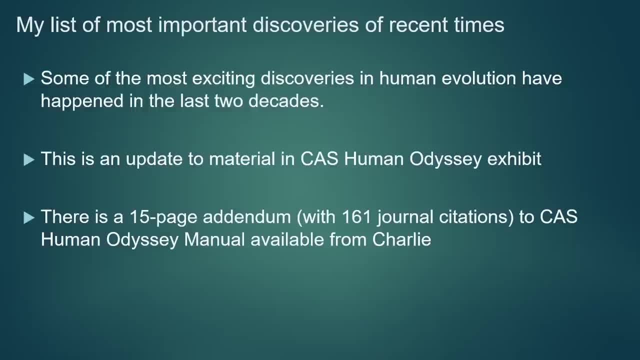 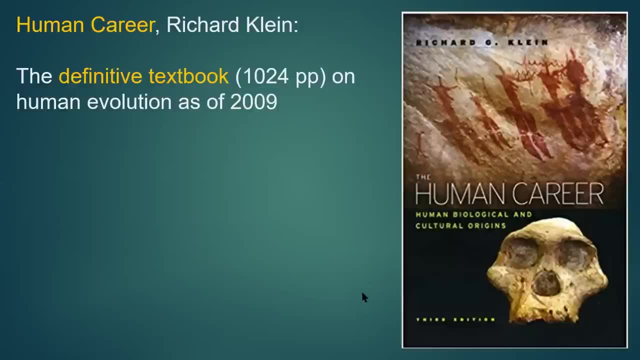 15-page addendum to the Human Odyssey Manual that is available for me if you're interested. All the citations are in there. The definitive textbook on this topic, I believe, is Richard Klein of Stanford's Human Career, and then also Conroy and Ponser's. 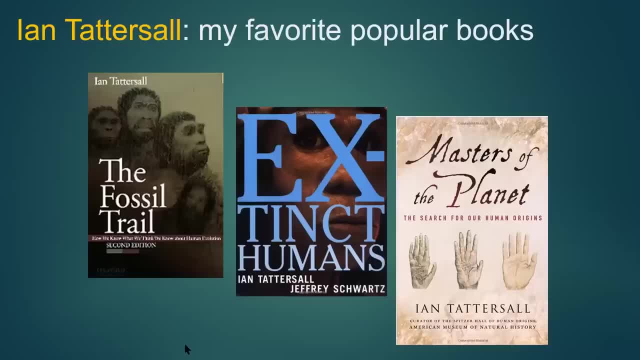 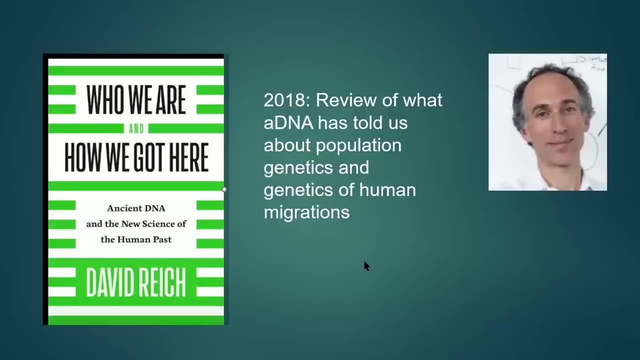 Reconstructing Human Origins. all right. For popular books, I think there's nothing better than The Fossil Trail, Ian Tattersall, a terrific writer, And then, most recently, Who We Are and How We Got Here, by David Reisch of Harvard, talking about the entire ancient DNA. 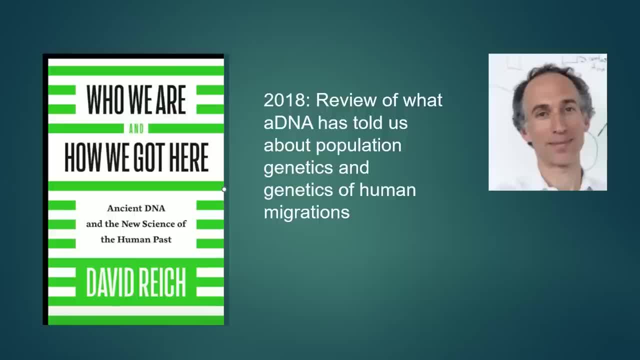 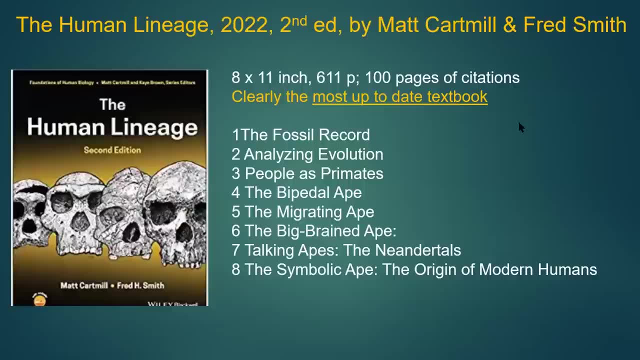 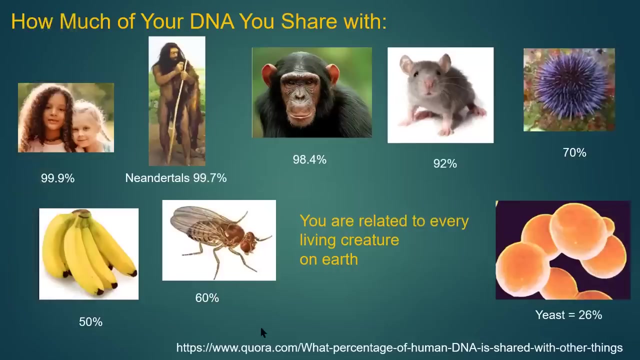 related particularly to population genetics and the genetics of human migrations and what that has taught us, And the most recent textbook that I think is probably the best, most up-to-date, is this one: The Human Lineage by Kirk Mill and Fred Smith People. when I do my pitch at the Academy, I always show- I have an iPad and I show this slide. 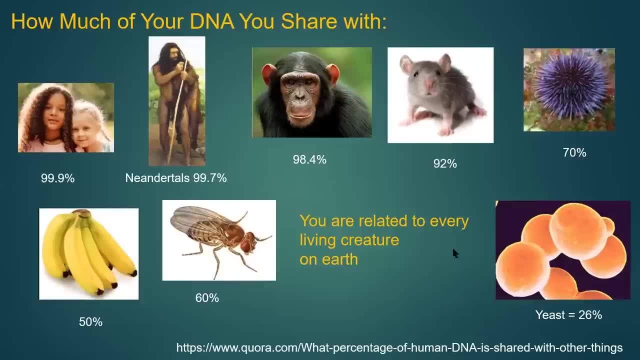 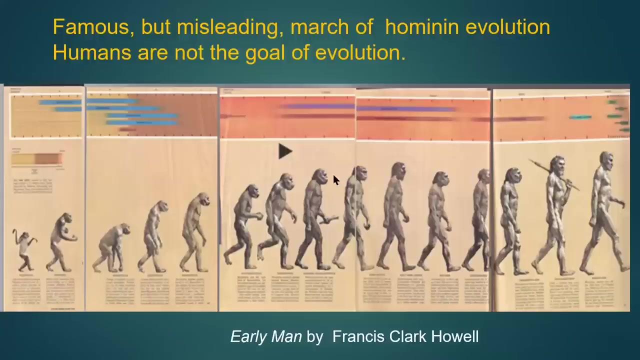 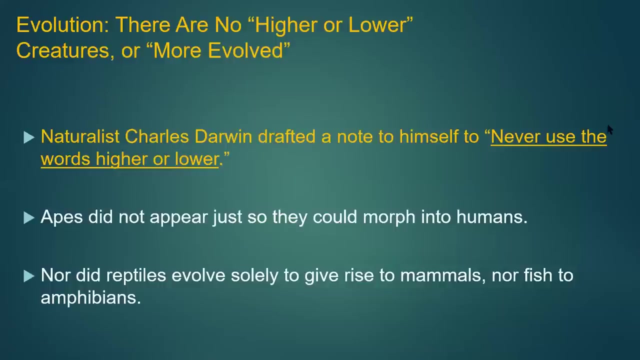 to remind people how much DNA we all share and that the kids love the fact that they share 50% of their DNA with a banana. So this is the famous 1965 early man, the misleading March of Progress. picture nice, picture, great, but humans are not the goal of evolution. okay, despite what the human odyssey exhibit may say. 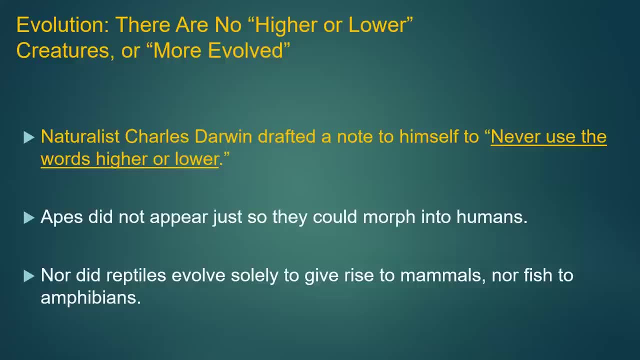 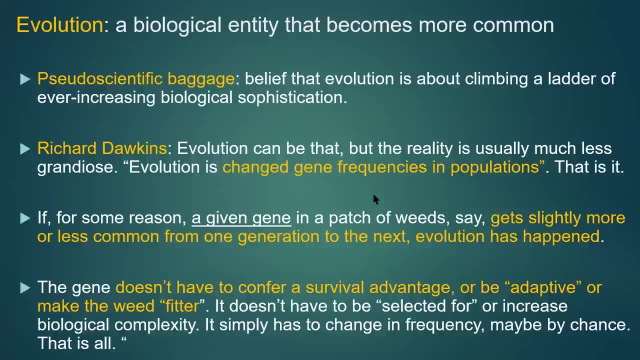 Charles Darwin drafted a note to himself saying never use the words higher or lower. Apes do not appear just so we can more fit to humans. We are not the end goal of evolution, or simply one spec, is it? The belief that evolution is about climbing a ladder of ever increasing biological sophistication is false. 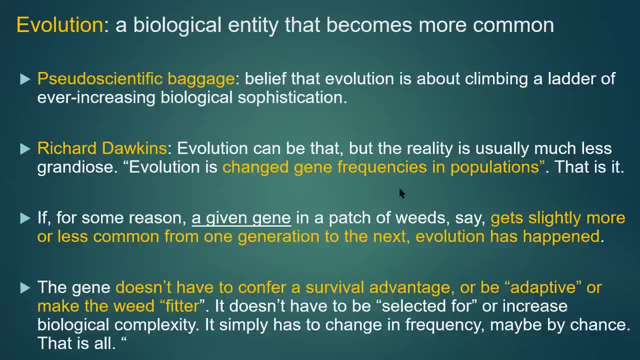 Richard Dawkins says evolution can be that, but the reality that the future is ever increasing biological sophistication is false. Richard Dawkins says evolution can be that, but the reality that evolution is ever increasing biological sophistication is false, is usually much less grandiose. Evolution has changed gene frequencies in a population. 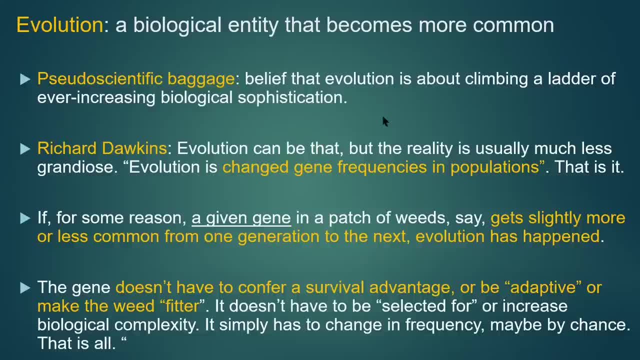 That's it. And if, for some reason, a given gene in a patch of weeds gets slightly more or less common from one generation to the next, then evolution has happened. The gene doesn't have to confer a survival advantage or be adaptive or make the weed fitter. It doesn't have to be. 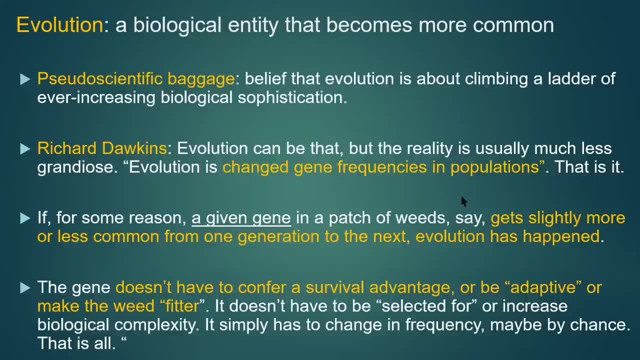 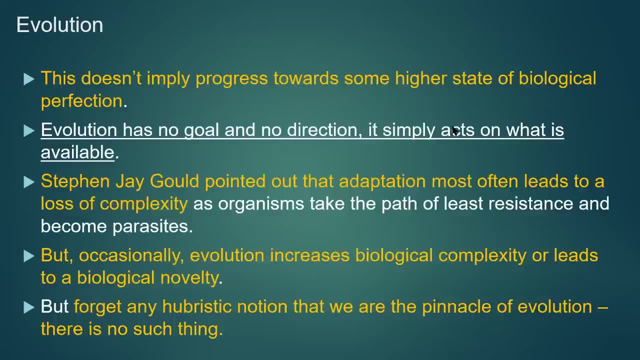 selected. It simply has to change in frequency, maybe by chance, and that's about it. So I'm going to skip a few as we go. Stephan J Gould pointed out that adaptation most often leads to loss of complexity. So evolution has no goal, no direction. It simply acts on the variation it finds in a biological 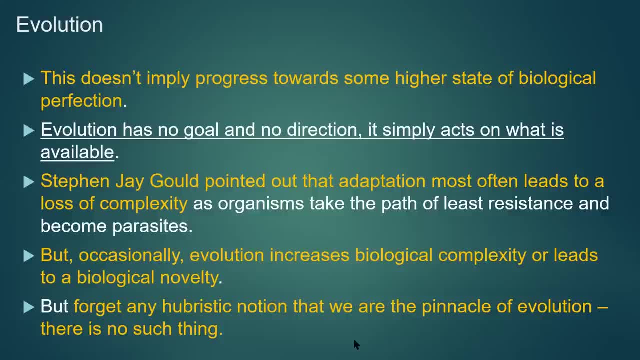 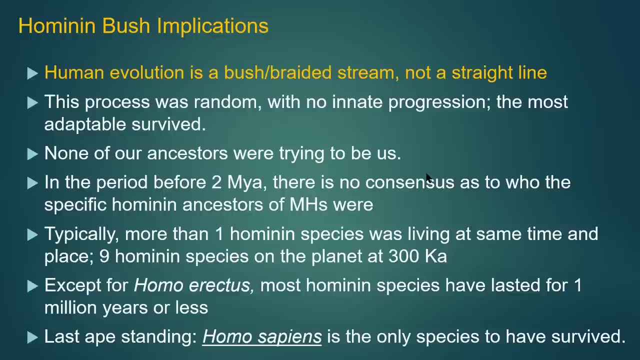 entity. So forget any Stephan J Gould. None of our ancestors are trying to be us. We also in the period before two million years ago. there's no consensus as to who the specific hominin ancestor of modern humans is. That's still. 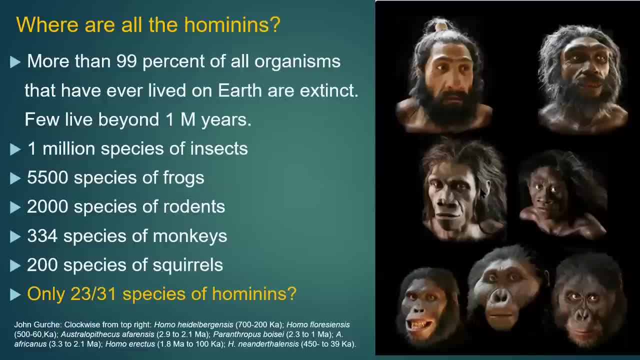 a contentious event. So my question of where are all the humans? more than 99% of all organisms that have ever lived on the planet are extinct. Few live beyond one million years. We're not there yet. I usually comment about the fact that there are 2,000. 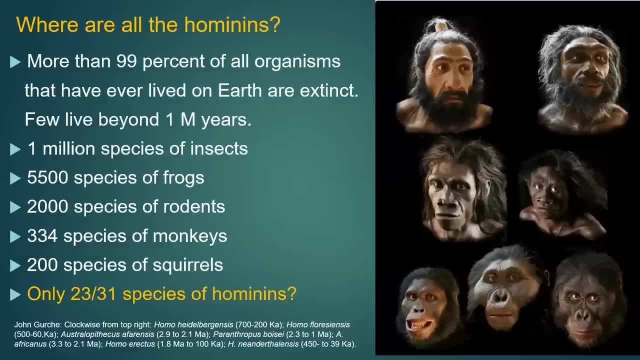 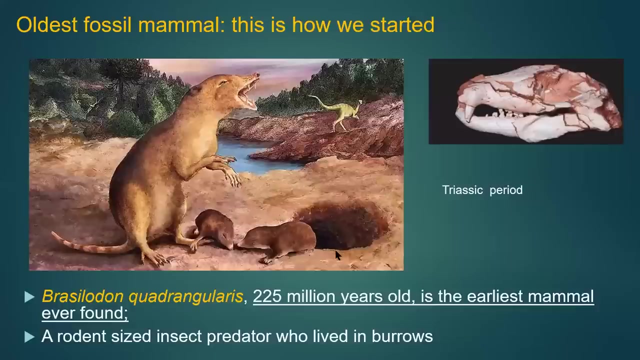 species of rodents and in comparison we've only got 23 species of hominin. We have not found very many. As an example, paleontologically, only 10% of Africans are extinct, So we're not quite sure if the population of Africa has been explored. So the chances are there are way more. 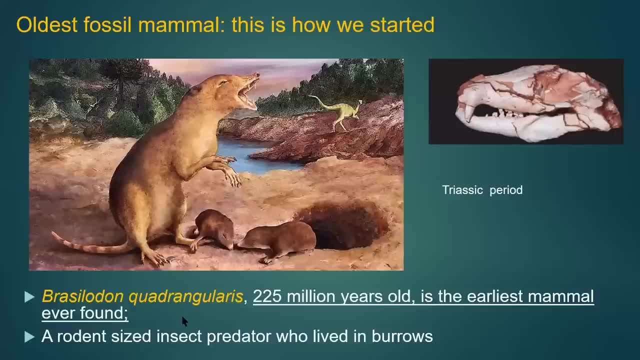 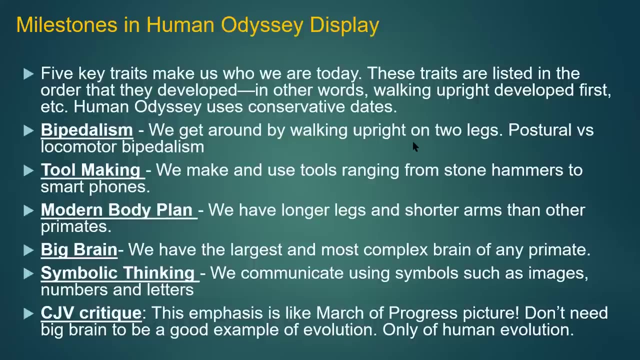 hominins. we simply haven't found them. This is one of the oldest mammals around, found in Brazil, 225 million years old, rodent size insect predator who lived in burrows while T rex and gang were up on top stopping around. 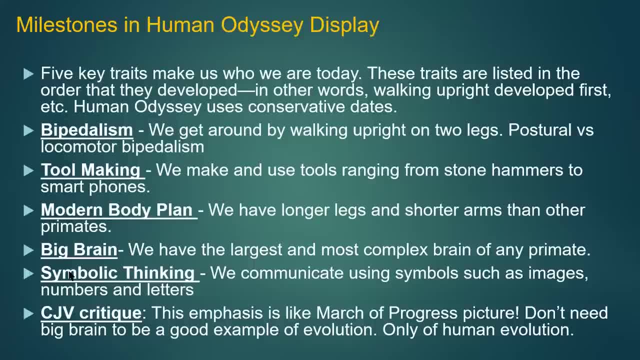 Stephan J Gould. This is one of the milestones currently exhibited in the human odyssey exhibit. I would comment that this is human odyssey because again, this is sort of like the march of progress picture. You don't need a big brain to be a good example of evolution, only of human. 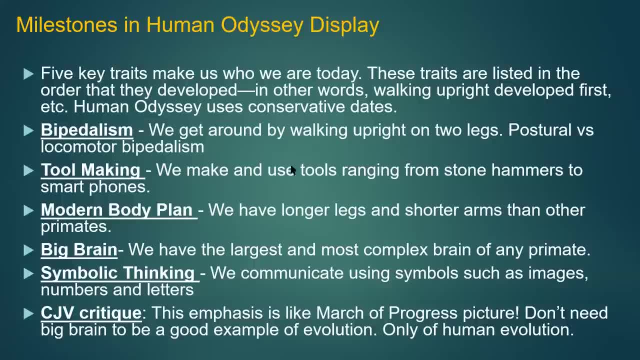 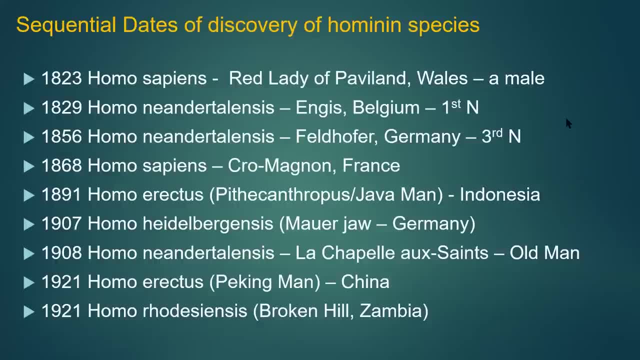 evolution. The whole question of when toolmaking happens, you'll see in a second, A very quick review. 1823, the first Homo sapiens discovered the Red Lady of Pavlodon in Wales. It was a male. The third finding of Homo neanderthalensis was in Beldhofer, Germany. We then see Cro-Magnon. 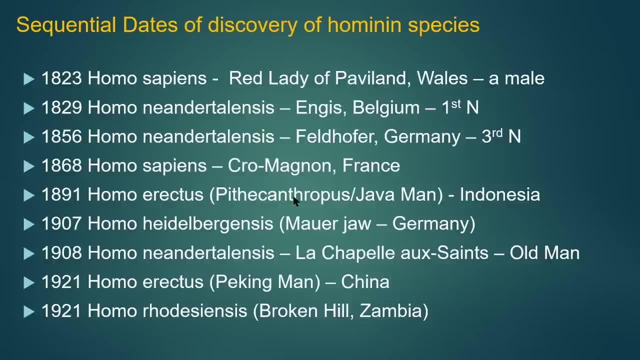 Then we see Pitcairnus dubois finds it in 1891 in Indonesia. The Mauer jaw is found in the Mauer jaw. The Homo neanderthalensis is found in Germany, first example of H burgensis, Then the La. 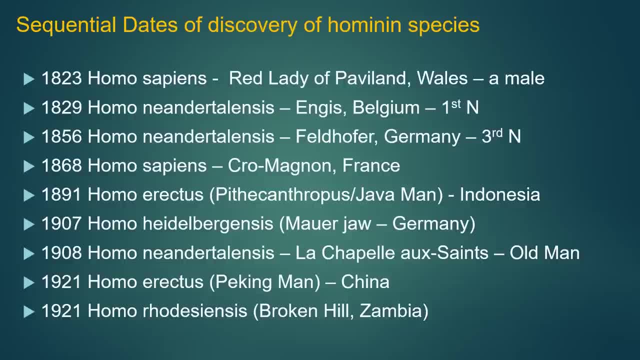 chapelle aux centes. Neanderthal in 1908.. This is the old man on whom all the bad imagery of Neanderthal began to achieve. Homo erectus. Peking man in China. And then the broken hill skull in 1921 is important for later discussion. 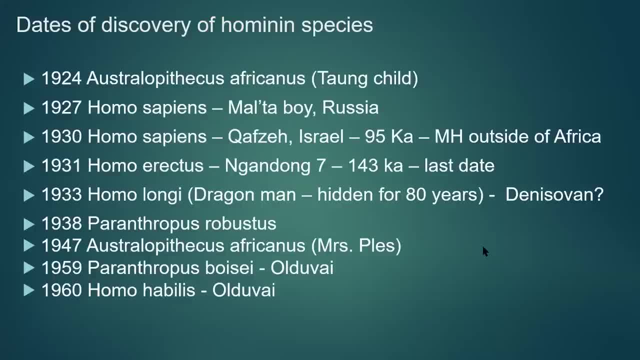 Then we get the Tong child Australopithecus africanus. Robert Dart, when he took it to London, accidentally left it in a cab and the police thought they had a murder suspect on their hands. The Malta boy in Siberia 1927, unknown then, hugely important in terms of ancient DNA, as we'll see. 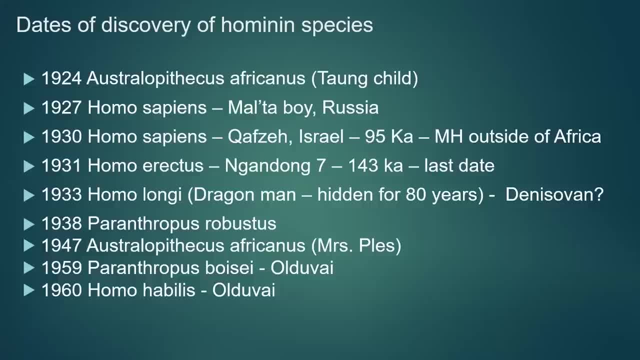 The Nangdong Homo erectus was discovered in 1931, and it is the last exhibit of Homo erectus dated to around 143 K. Homo longi has been named only recently because the finder hid him for 80 years in a farmer's well. 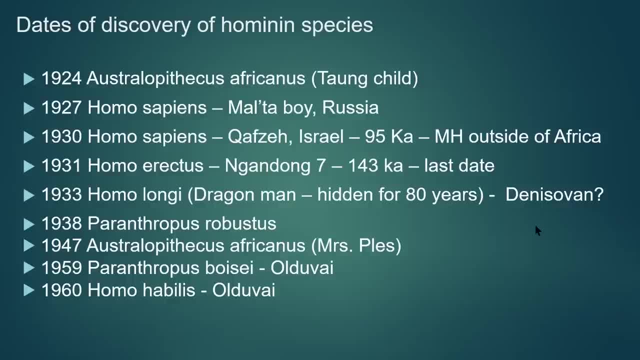 And now the question is: was he an example of Denisovans? Then, in 1959, 1960,, at Olduvai Gorge, the Leakeys discover first Paranthropus bozi and then Homo habilis. We'll talk about them. 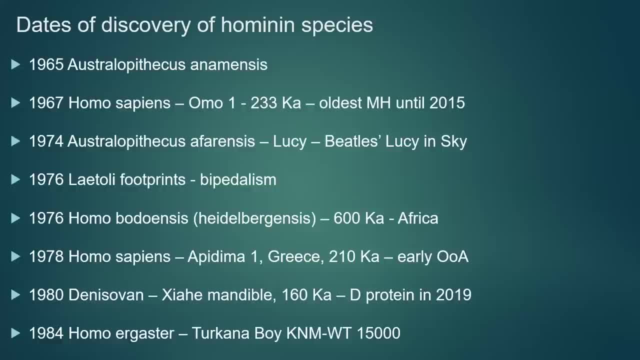 The Homo oneskull discovered in 1967, Homo sapiens and now dated to 233 K, was the oldest modern human until 2015.. Lucy, discovered in 1974, named after the beetles Lucy in the sky with diamond, by Don Johansson and gang. 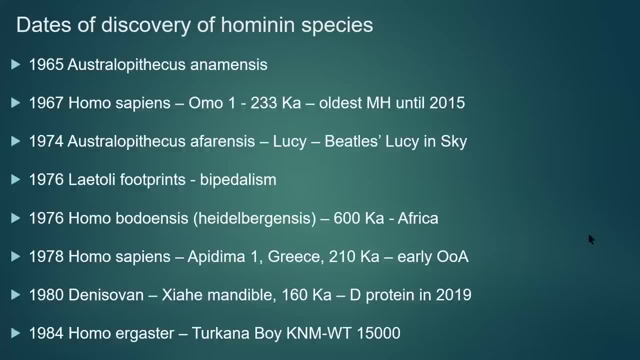 The Laetoli footprints. Then in 1978, a skull at Epidema Reis was found that people now believe is a modern human at 210 K early migration out of Africa. The Denisovan Zia tibet mandible was discovered in 1980, and protein analysis makes us think that it's Denisovan. 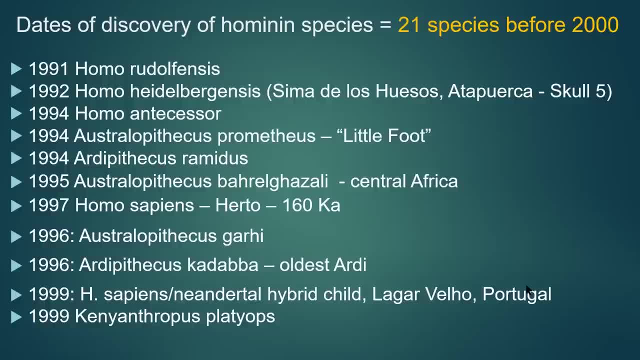 Turcana boi Homo erectus in 1984. And then the Cima de los Huesos in Alacuerca, Spain, are discovered in 92, considered Hydrobregensis Then, And Tissasaur shows up. 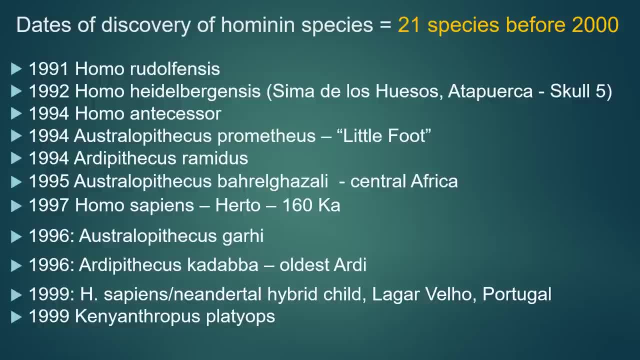 Then Littlefoot in South Africa, Then Ardhi Ramidus shows up, Then the only Central African Australopithecus was discovered, Then the Herto Homo sapiens skull was discovered, Finally Cananthropus platyops. 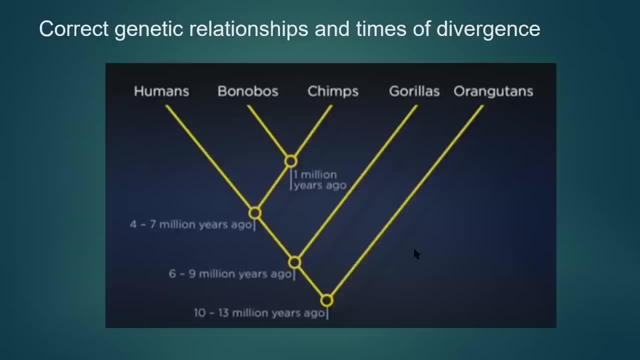 which we'll see in a second. So currently the thinking is that divergence occurred between us and orangutans around 13 million years ago, between us and gorillas at 9 million years ago and us and chimps and bonobos around 7 million years ago. 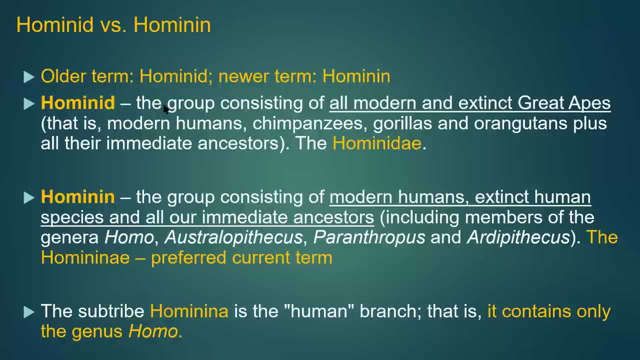 So just a comment: the term hominid versus hominin- this is now the preferred current term. It is a group of all modern humans, extinct human species and all our immediate ancestors, So it includes Homo, Australopithecus, Panthropus, et cetera. 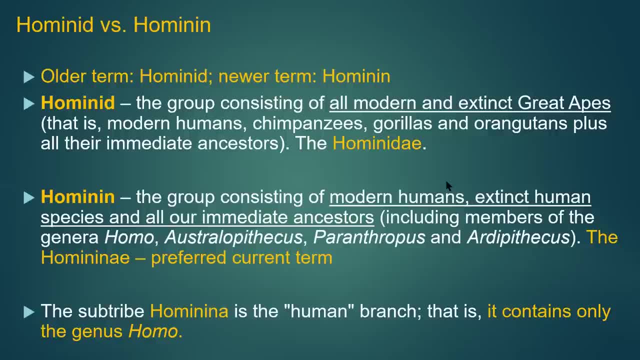 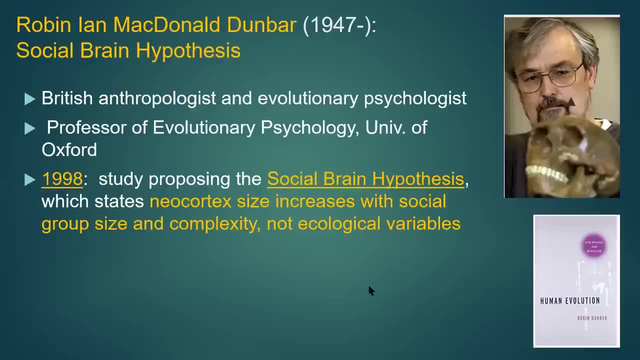 So it contains only the genus Homo, basically not orangutans et cetera, which are hominids. I would comment, because this is my favorite theory of why our brains got as big as they did: Robin Dunbar came up with the social brain hypothesis, and what it states is that 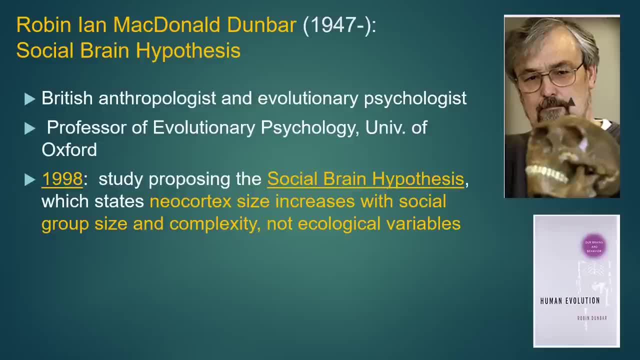 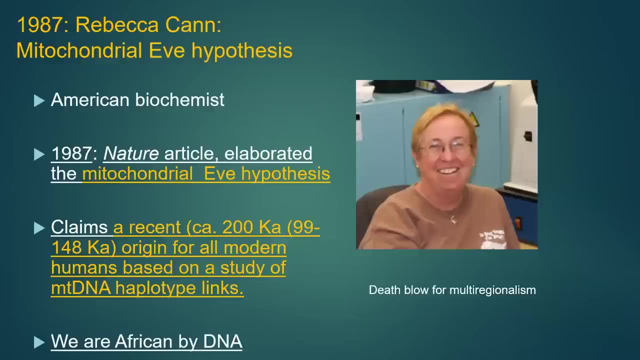 neocortex size increases with the social group size and complexity not correlated with ecological variables. So it is our sociality which profounds, So it is our sociality which profoundly influences who we are basically. And then I've got to mention the mitochondrial eve hypothesis. Rebecca Kahn at Berkeley came up. 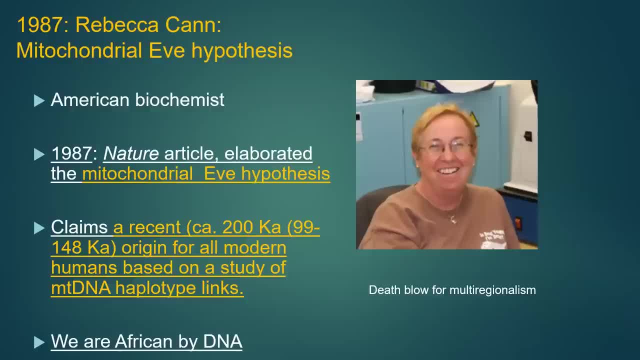 with the idea that all modern humans descend from a single African woman dated around 200 K, 99 to 148 K is the most recent, And this was based on a study of mitochondrial haplotype, And so we are all African by DNA. for whoever's in charge, 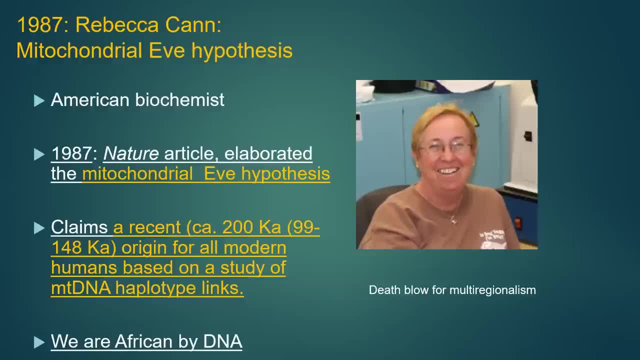 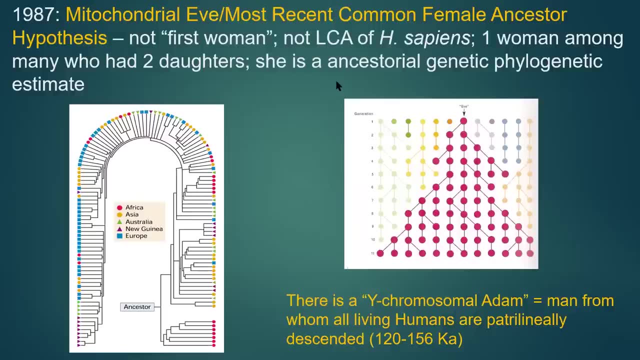 I keep getting Larry Cook and trying to be admitted on my screen. Okay, So this concept is that the most recent common female ancestor Is what this hypothesis is. It's not the first woman, It's not the last common ancestor. It is one woman among 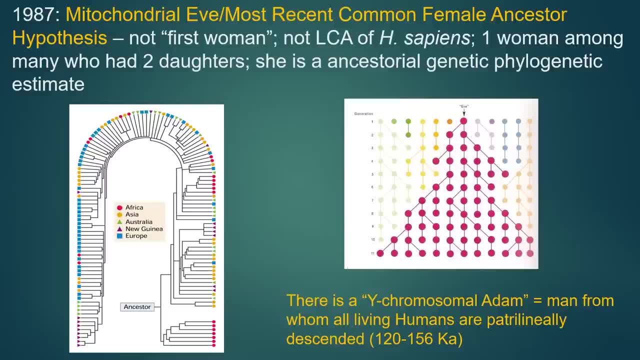 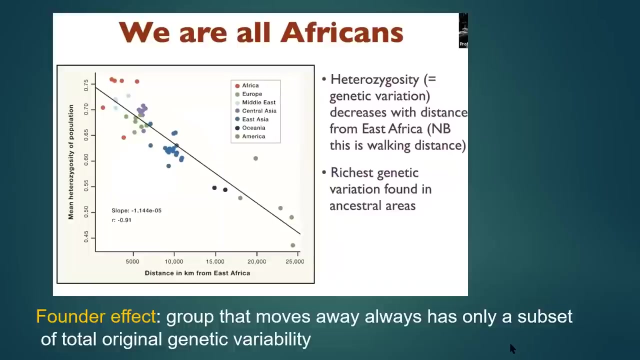 many who had two daughters and ended up being the mother of us all. She is an ancestral genetic phylogenetic estimate. basically There is a Y-chromosomal atom who lived, who is our patrilineal descendant from around 120 to 156 K. So basically we are all African by DNA. 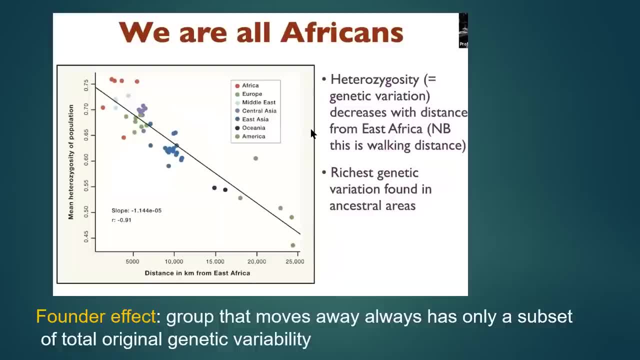 And an important study looked at heterozygosity, that is, how much genetic variation we have, And what they found was that that decreases with distance from East Africa. The further away you get, the less genetic variation, The farther back in time. 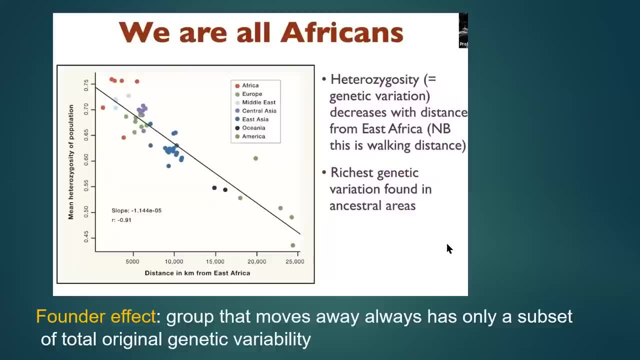 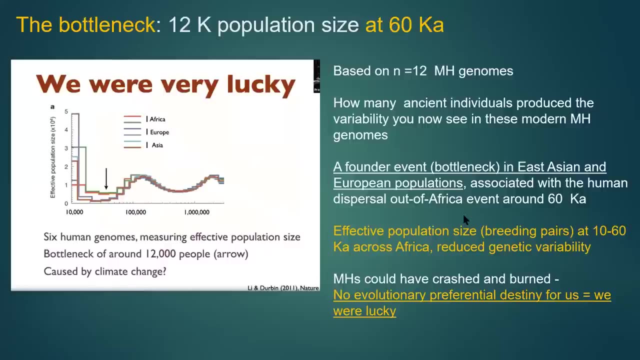 And you find- And this is all based on the founder effect- that as a group moves away, it always has only a subset of the total original genetic variability that started in Africa And, importantly, the famous bottleneck event Around 60K, based on a genetic analysis. 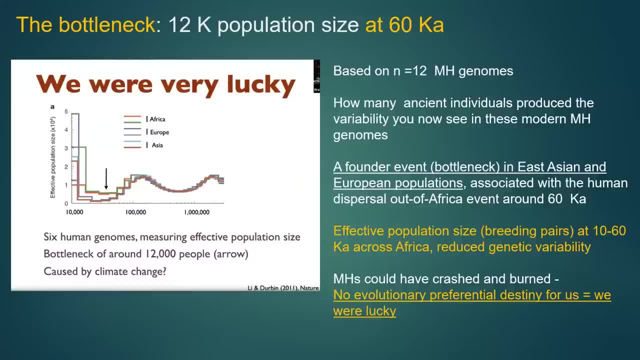 That there was a founder event in East Asia or Europe associated with our out-of-Africa dispersal around 60K. So the important point of this is: right around the same time that Neanderthal disappeared, we could easily just as easily- have disappeared as well. 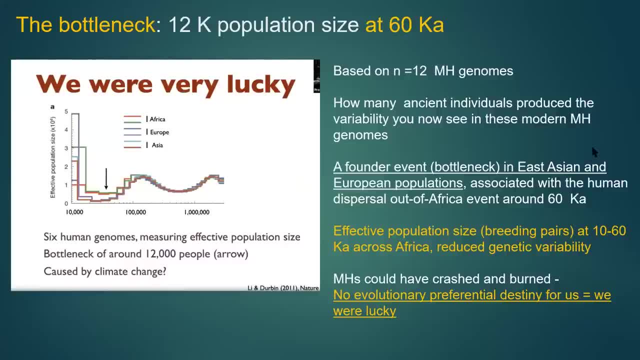 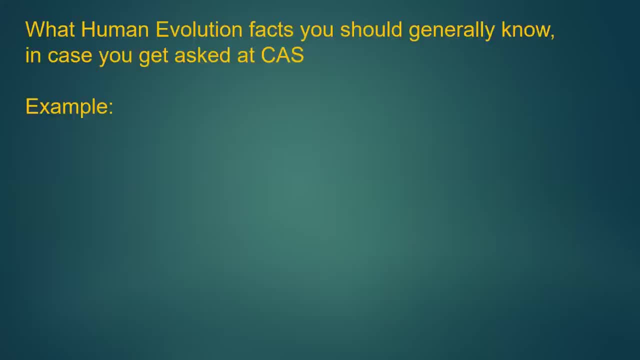 That's evolution and the consequences of genetics basically. So I'm going to show what human evolution facts you should generally know in case you get asked at CAST. Interestingly, in the last three weeks, after telling them about we are all genetically from Africa. 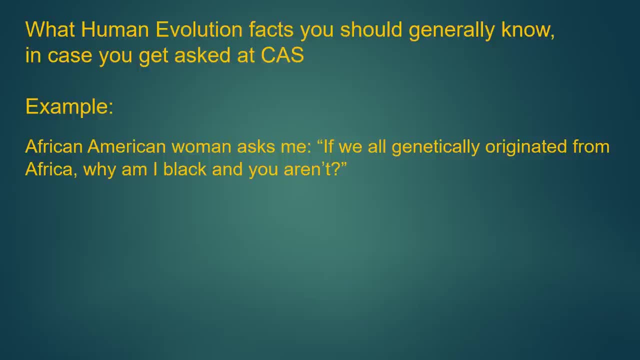 an African-American woman in front of me asked me: Charlie, if we're all genetically originated from Africa, why am I black and you aren't? Okay, Okay, great question. So we ended up talking about latitude, not race, Okay. a 12-year-old kid starts crying and says: 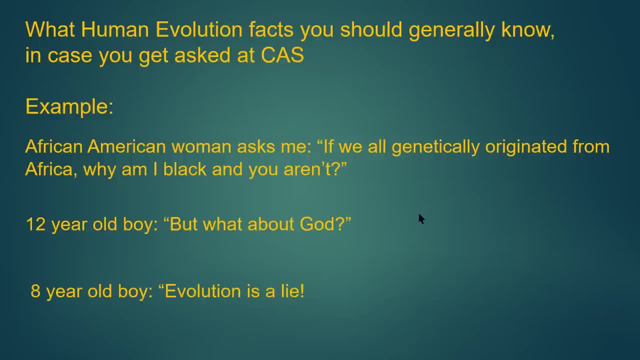 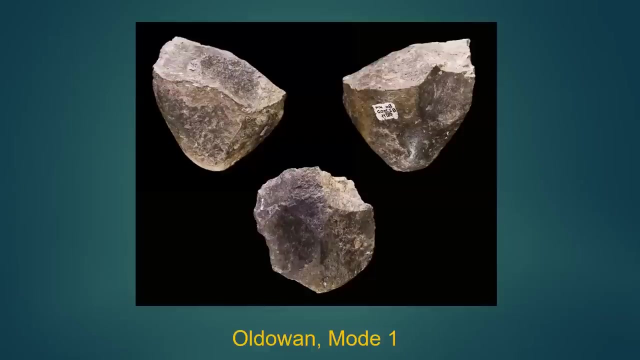 but what about God? And this week an eight-year-old boy, evolution is a lie and then walks away. Okay, so great expectations out there, And very quickly. the basic stone technologies. this is the old, The one basically around pebble that's knocked against each other. 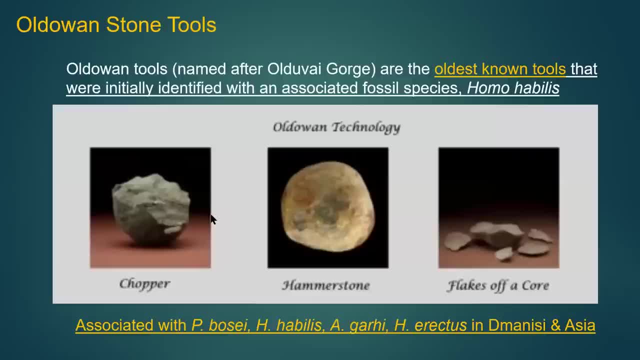 to produce a flake And for the longest time they were considered the oldest known tools. They're associated originally with homo habilis and bozai, then gari, homo erectus. in Asia, This is an Acheulean handaxe that 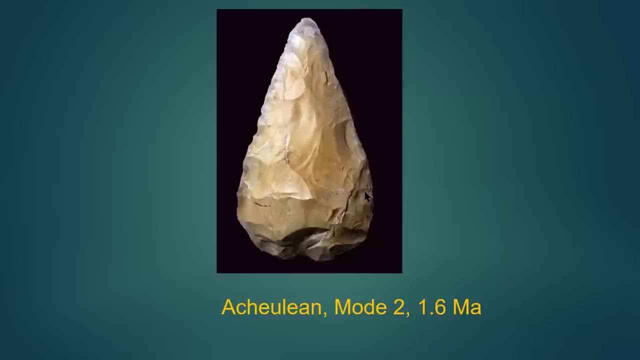 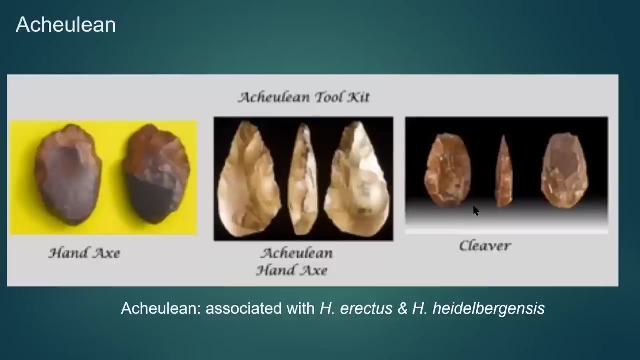 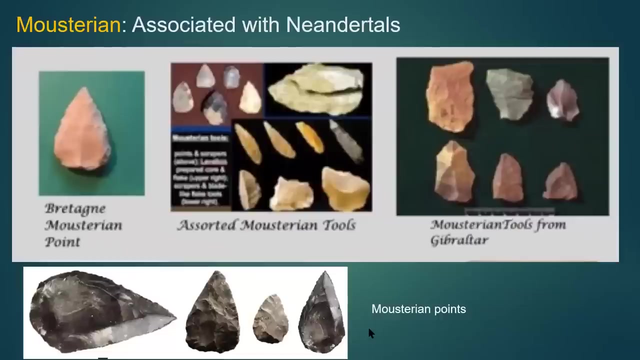 was around for almost 2 million years. It was a great tool, Could be as sharp as a surgeon's scapula, And they had cleavers as well, typically associated with erectus and heidelbergensis. The Mastarian tradition is the Neanderthal one. 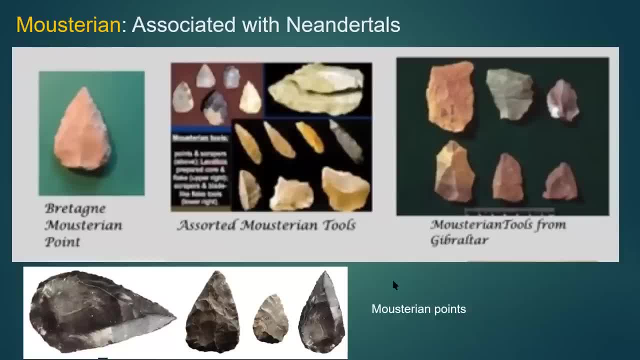 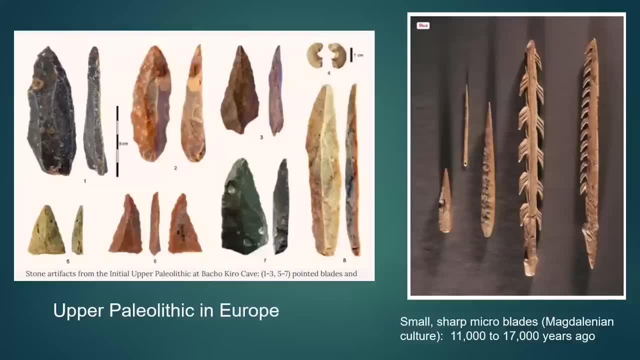 Also the Le Voix technique as well, where you clip off a piece And then the Upper Paleolithic starts showing bladettes very thin, sometimes beautifully carved, as well as the introduction of bone and wood pieces. These are microblades from around 17,000 K- 17,000. 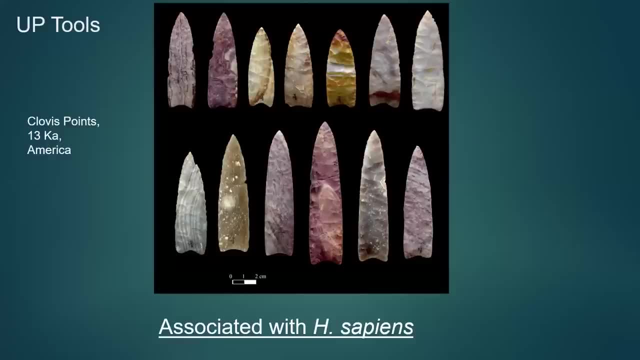 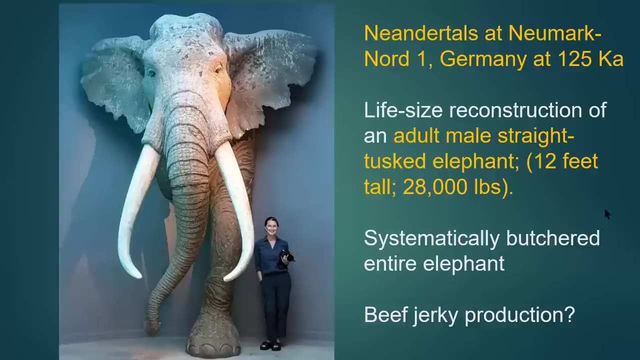 And these are Clovis points from America, And the Upper Paleolithic is typically associated with Homo sapiens, but there are some Neanderthal claims as well, And just published- I have to tell you this, even though this isn't what I was going to cover- a study of Neanderthals at Newmark Nord one in Germany, a coal mining plant that had 125 K. 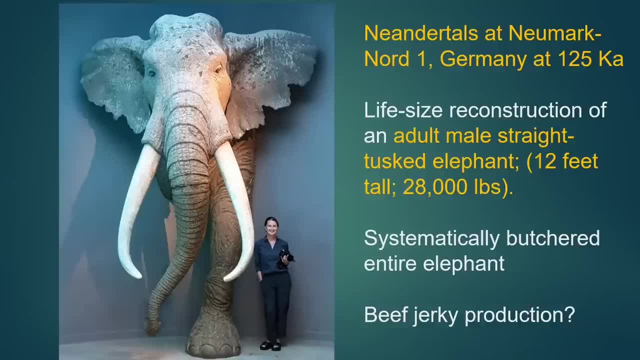 Neanderthals. Neanderthals were hunting this, the largest mammal that ever walked the planet, 12 feet tall, 28,000 pounds. 70 of these guys were found at this site. They were systematically butchered. 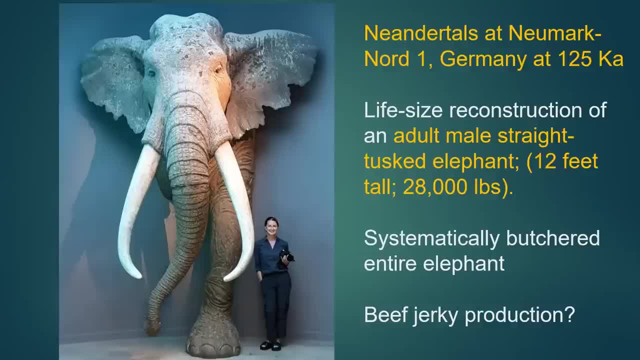 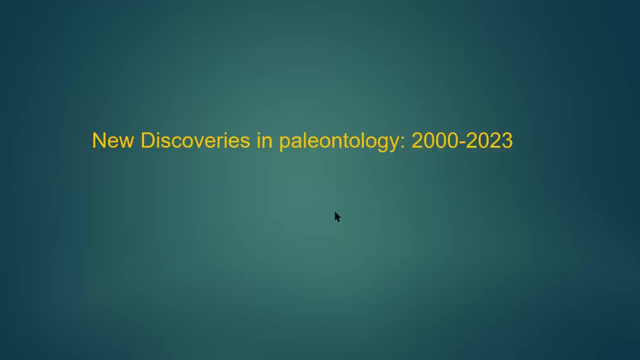 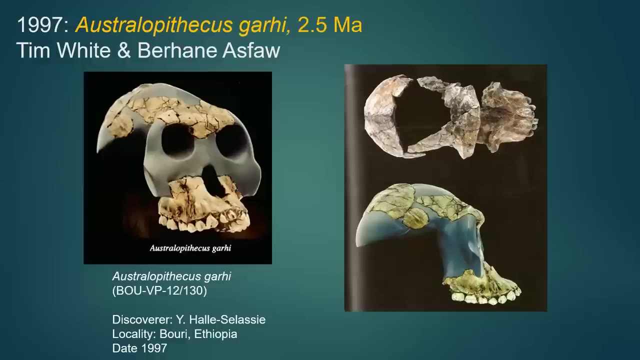 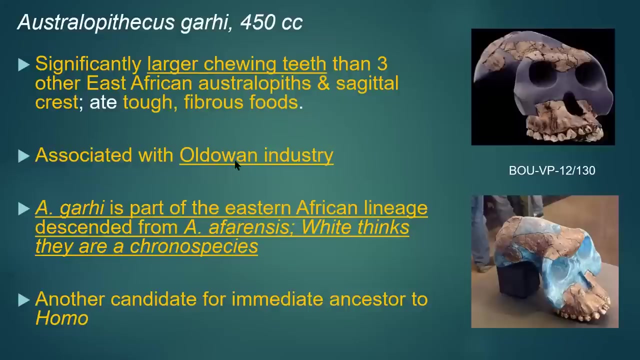 And the question is: were Neanderthals producing beef jerky by heating up for preservation purposes? So great study just published? So the last 25 years. Australopithecis gari, 2.5 million years ago- I always liked the blue infill- had slightly larger back molars associated with the Oldowan industry. 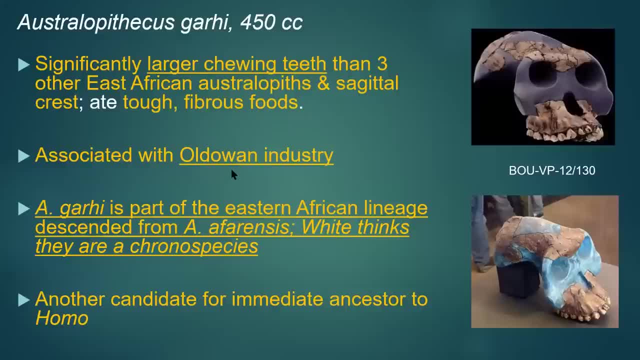 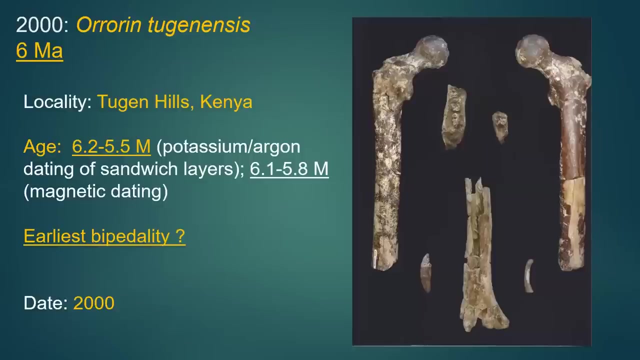 So here's an example of a pre-Homo using tools. Basically, Tim White of Berkeley thinks they're basically related to Lucy Afarensis, basically, but another candidate for an immediate ancestor to Homo, Aurora intergandensis, dated to 6 million years, the Tugan Hills in Kenya, possibly the earliest bipedality evidence. 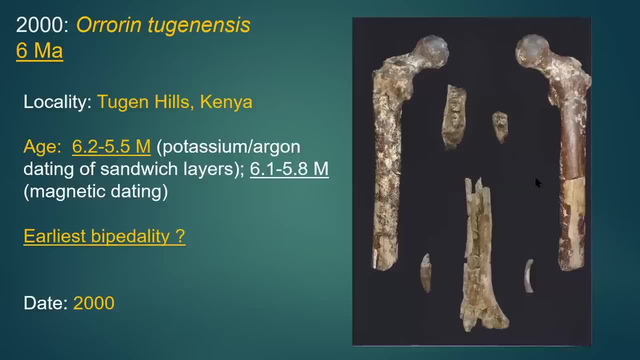 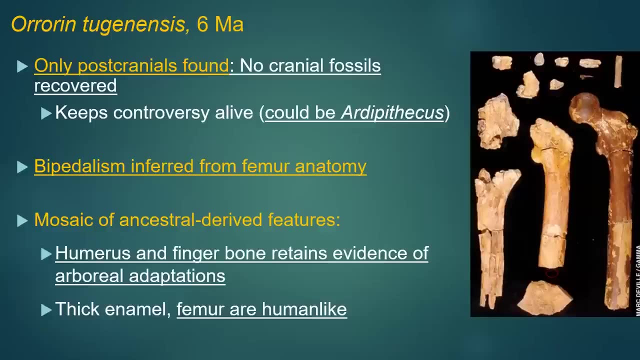 And we only have Postcranial femur kinds of bones to see but no cranials and that sort of keeps it. Some people think this could in fact be Ardipithecus and the bipedalism is inferred from the structure of the femur anatomy. 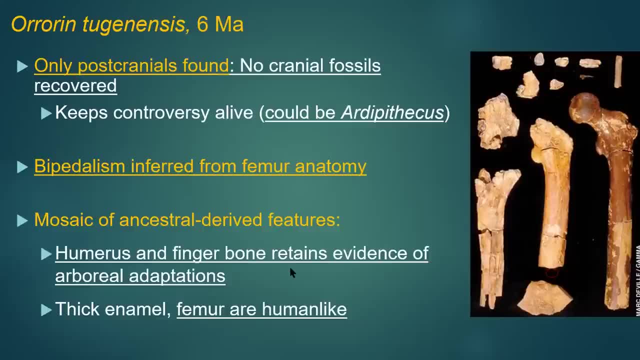 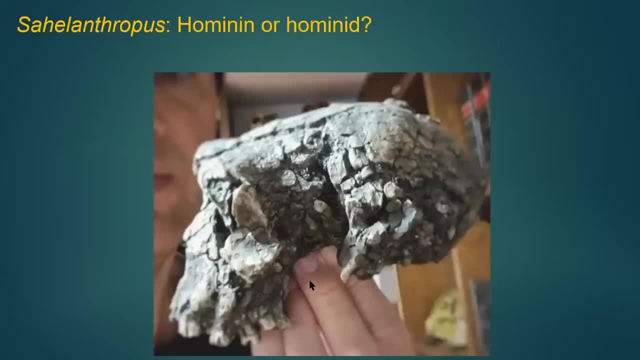 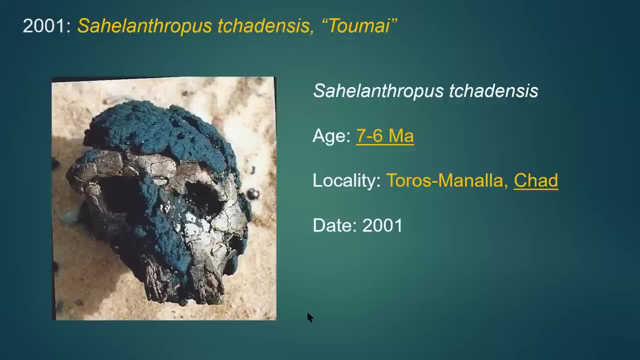 The humerus and finger bone are definitely arboreal adaptions, but the femur is a little more human-like. Sehalanthropus- is this a hominin or a hominid? or a hominoid Found in the middle desert in Africa, at Chad, dated to 7 to 6 million years ago? 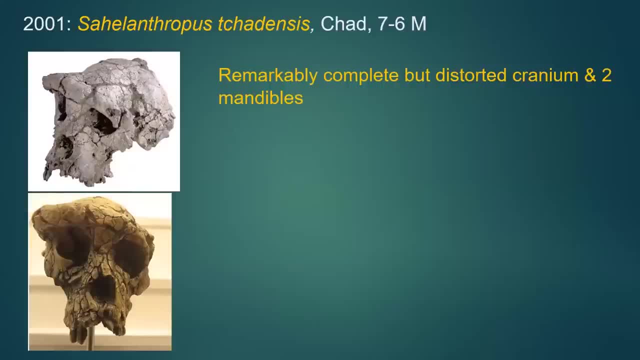 Remarkably complete but totally distorted cranium that had to be computer reconstructed and it is the largest brow ridge in the world. It was first found in Africa And that's why I did this. It was first found in Africa. in any fossil that's been found, that's a hominin type. 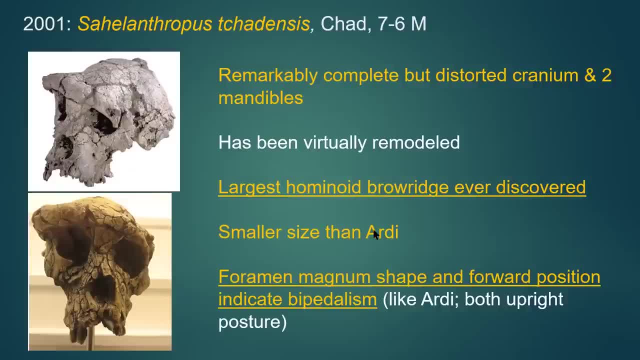 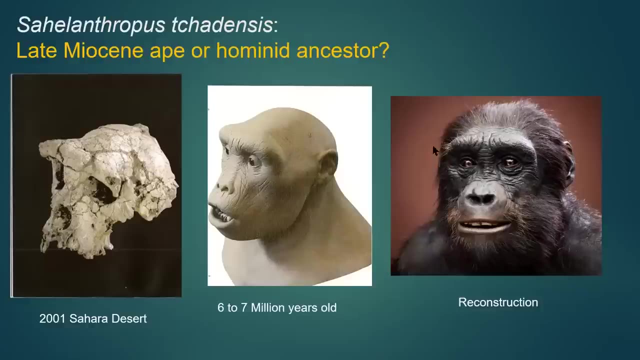 smaller than arty, and the form in magnum, the spinal cord hole, the shape and its forward position is partially proposed as indicating biketalism, And these are remakes and reconstructions. but the big question continues to be: is this a late Miocene ape as opposed to a hominin? 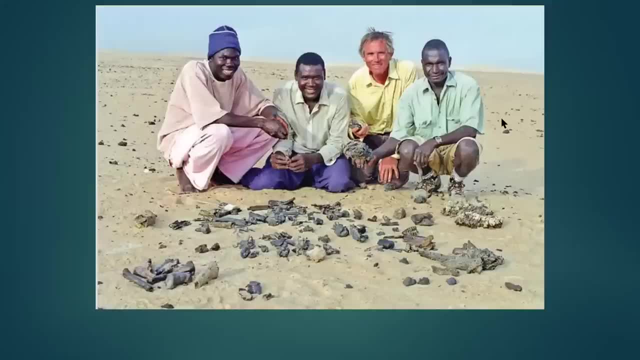 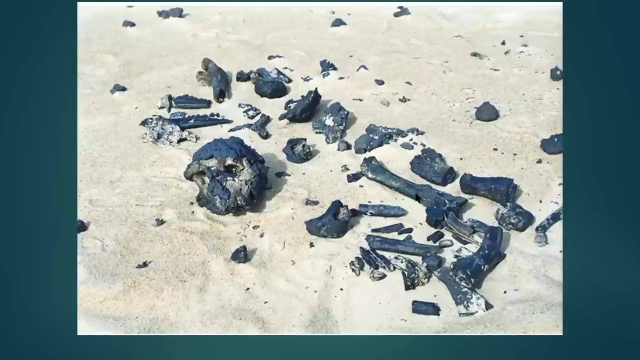 Because this was the original. this was the assistant director He's actually holding to my. this were the bones, but note in this picture, no femur. The skull is in his hand. In the next picture we get a femur, all right. 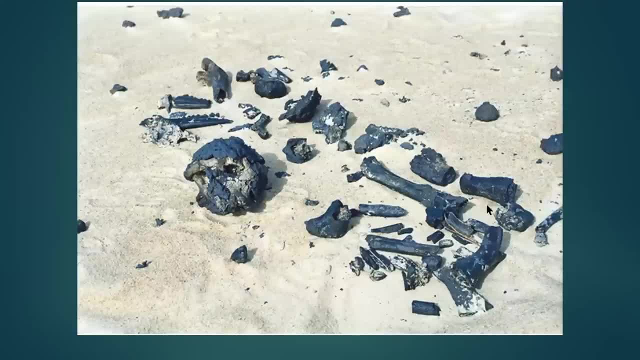 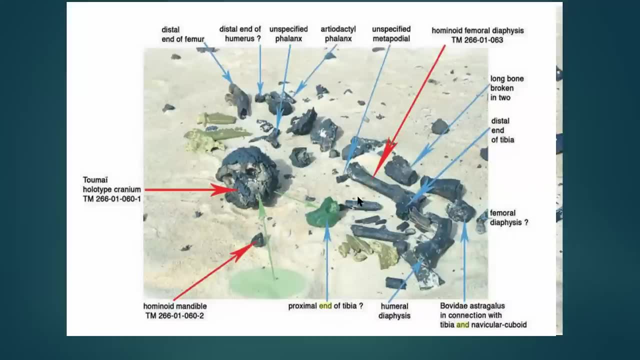 And then this femur disappears for 20 years. Okay, some great stories in paleontology. So that's the cranium and that's the disappearing femur. And the femur is hugely important because it tells us whether they were bipedal. 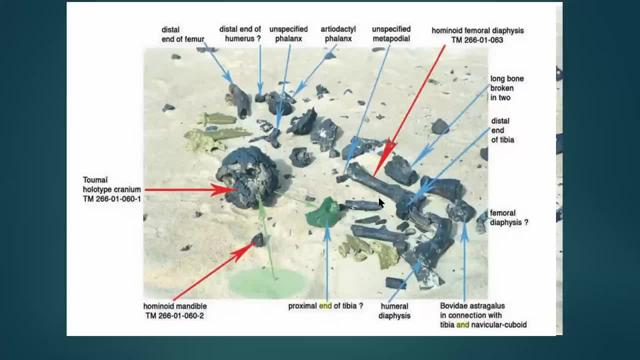 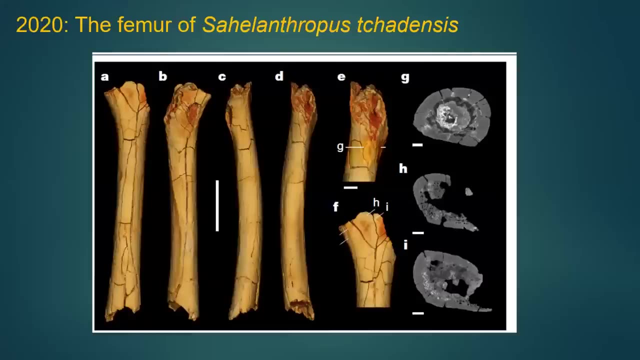 And that's the current controversy is: was this a bipedal creature? And the question: did camel hoarders rebury this fossil facing Mecca? okay, So in 2020, the femur- an article finally comes out. 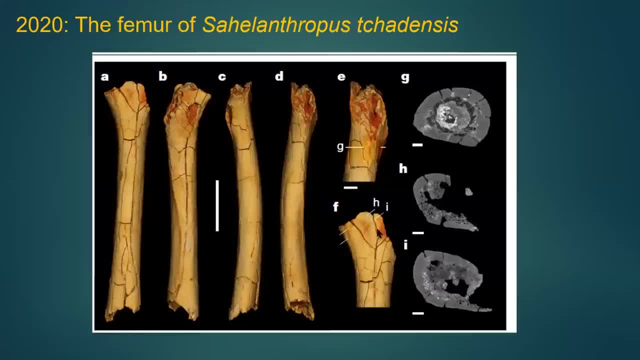 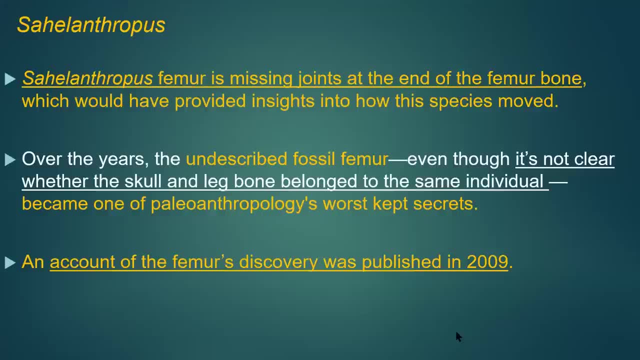 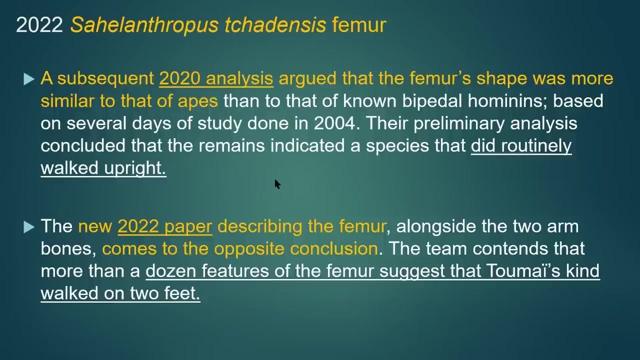 but no top or bottom, which makes it much more difficult to interpret, And so this was probably the worst kept secret of paleontology in terms of where was this femur? Something was published in 2009, then a 2020 analysis analysis indicating that they thought it was an ape, not a hominin. Then a 222 paper comes out. 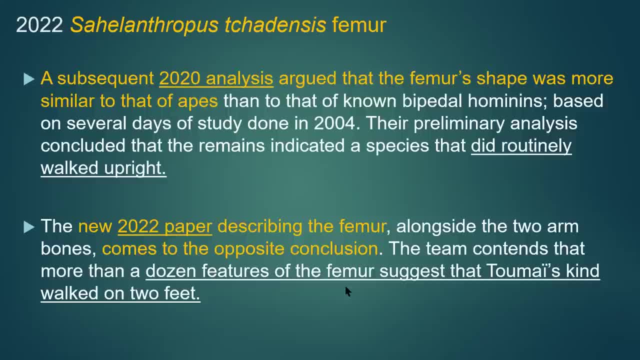 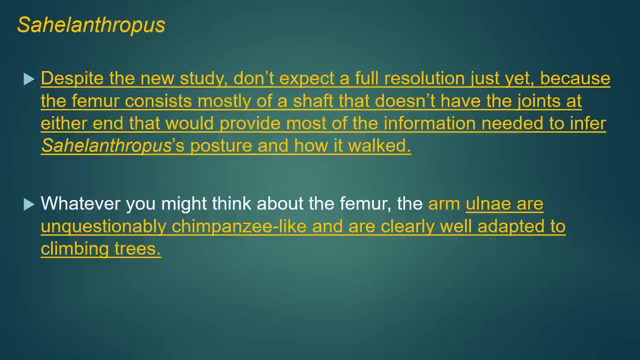 describing it comes to the opposite conclusion, thinking there's more data that it was in fact biped. So don't expect a full resolution just yet, because the femur consists mostly of a shaft that doesn't have the joints, And so we don't actually know whether it walked upright. The only 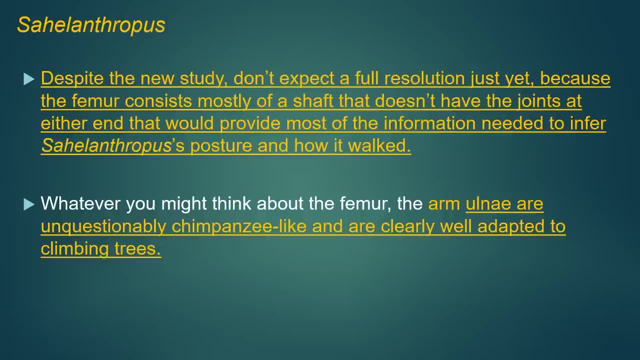 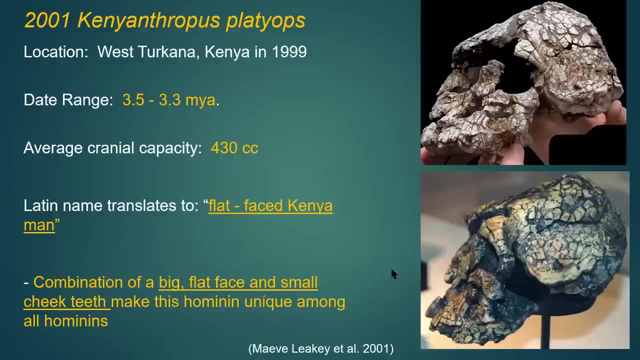 the arm, muscles or bones are unquestionably chimpanzee-like and are clearly climbing trees adaptable. Kenyanthropus platyops was found by Maeve Leakey, dated to 3.5 million years, Big, flat face, small cheekbone teeth, And it's highly, highly fragmented. 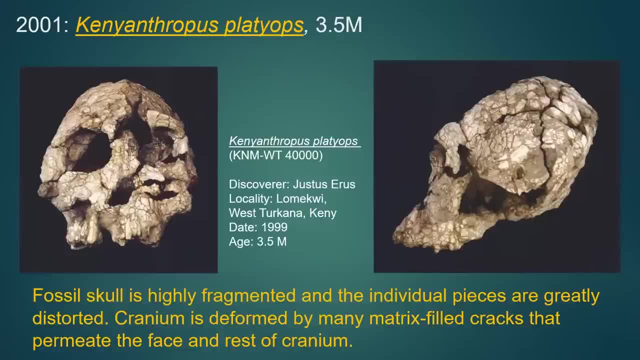 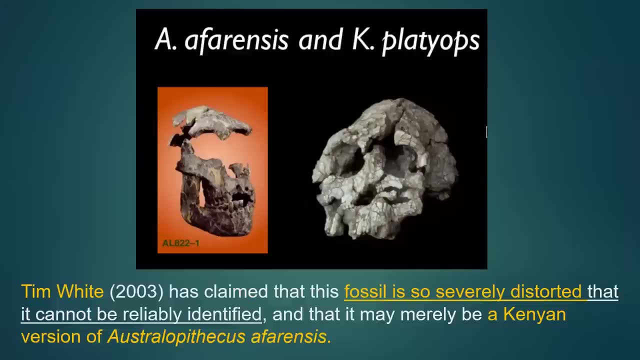 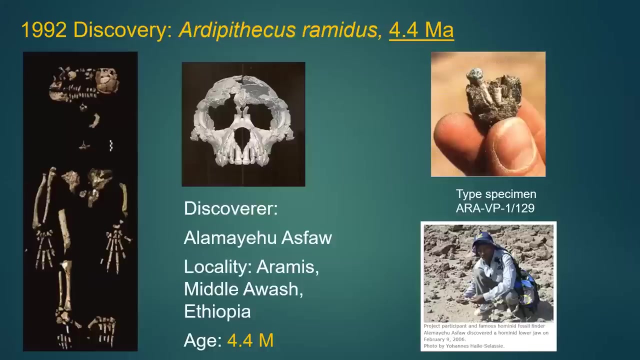 And the individual pieces are greatly distorted. The cranium is deformed by matrix-filled cracks And basically, again, Tim White thinks this is so severely distorted that it's not identifiable. He thinks it's a afarensis. basically, Then, in 1992, he, Tim White and gang, discover Ardipithecus ramidus. 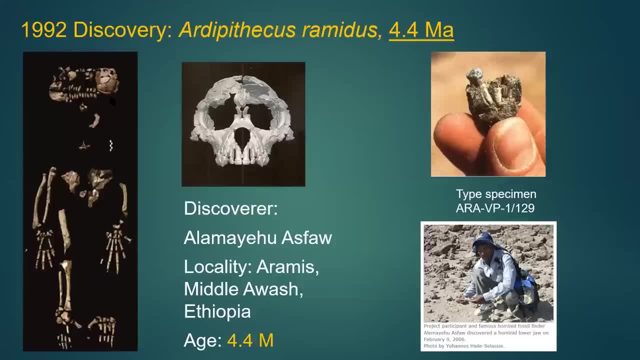 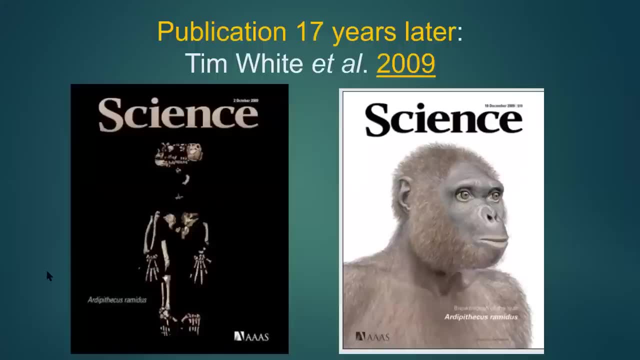 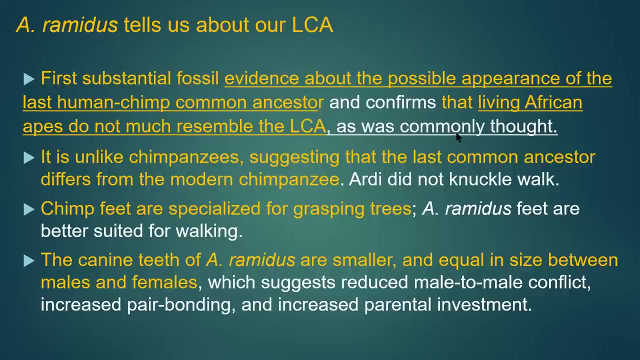 4.4 million years, Nice skull features and lots of bones, But Tim takes 17 years to publish. He is the academic scientist type, basically And, as you'll see, has some major critiques of others in the field, But it's the first substantial fossil evidence about the possible appearance of the last. 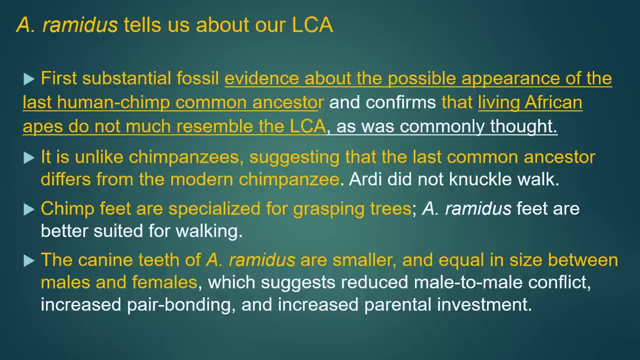 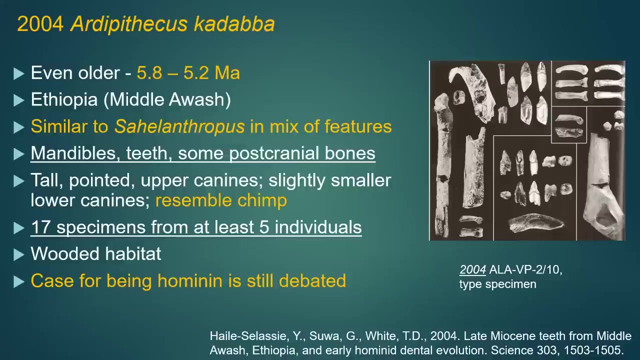 anderen bonding, increased parental involvement. Then comes Arte cadaba. This one is a million and a half years older, I think, probably ancestral to Arte Ramidus, similar to Sahelanthropus in features. 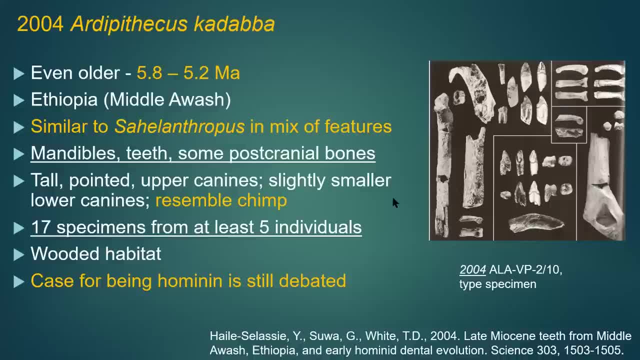 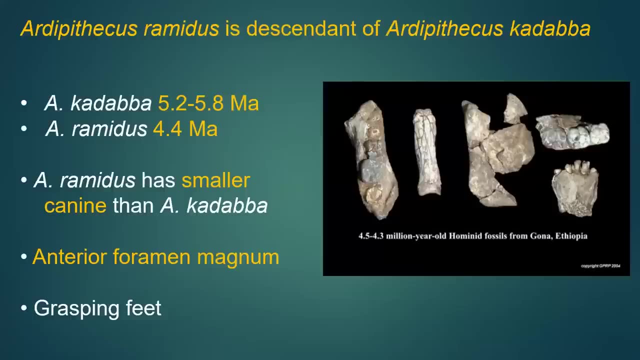 but we only have some postcranials and a mandible and teeth. We have 17 specimens from at least five. So the case of this one again being hominin is also debated. So it does have an anterior form of magnum. 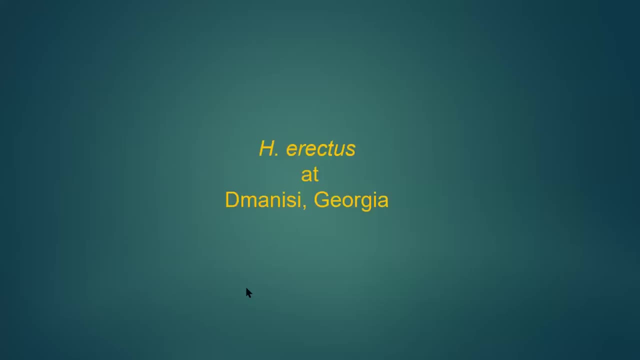 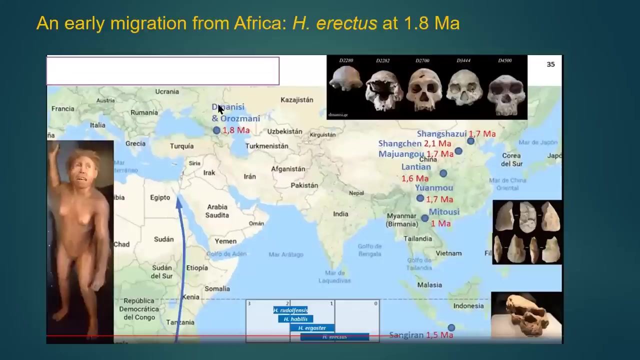 which is a bipedal indicator, but grasping feet. Then comes Homo erectus at Dmanisi, Georgia. So Africa Up here above Turkey is Dmanisi, but at 1.8 million years And although pretty soon we have a whole bunch in China. 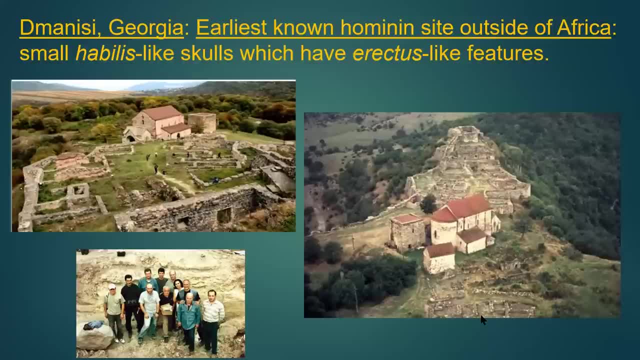 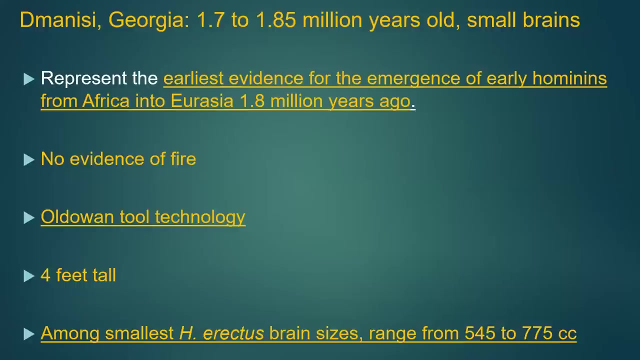 This is the earliest known hominin to leave Africa- Homo erectus. basically, This is showing small abelis-like skulls with um Homo erectus-like features under a medieval church. No evidence of fire. Aldoan tool technology- four feet tall. 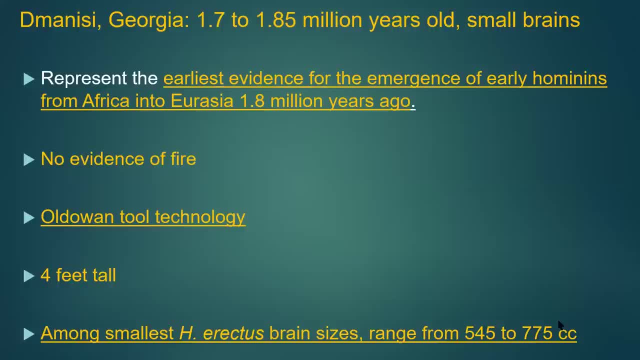 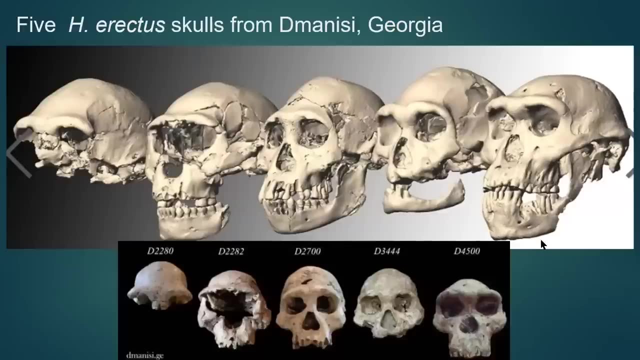 Among the smallest erecti brain sizes: 545 to 775.. Dated to about 1.8 million years. Probably these are the five skulls. The suspicion is that this is a human skull. This is a human skull. The suspicion is that these were the victims of saber-toothed lions, basically. 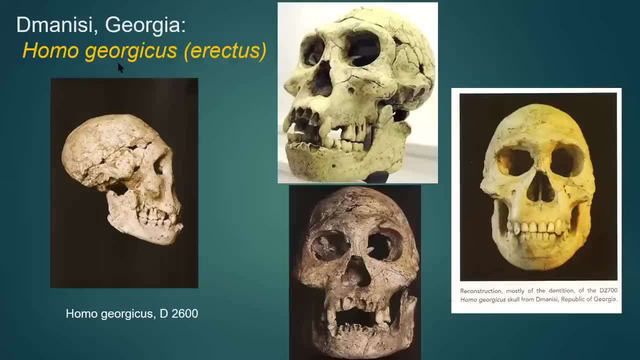 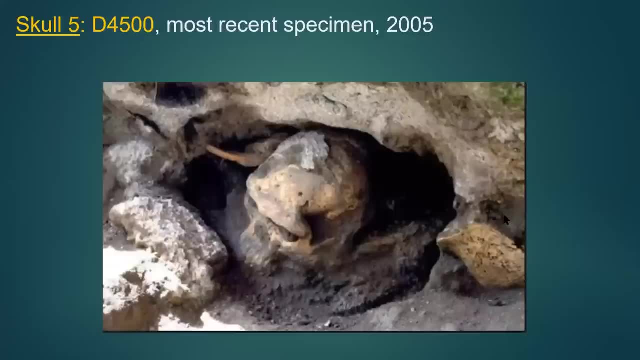 And called Homo georgicus by the Russians, who were the ones that found these guys. And this was the most recent specimen coming out of the ground: skull five. It is probably the most perfect skull ever discovered, because it's totally complete. 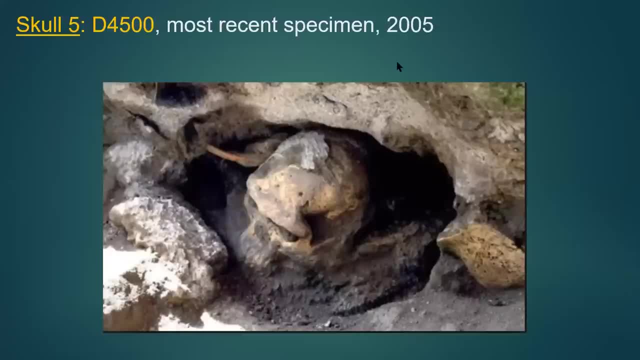 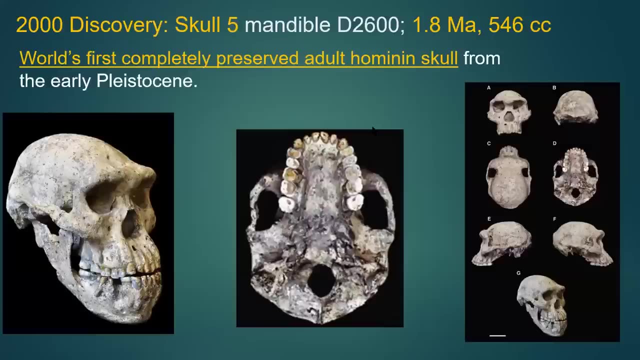 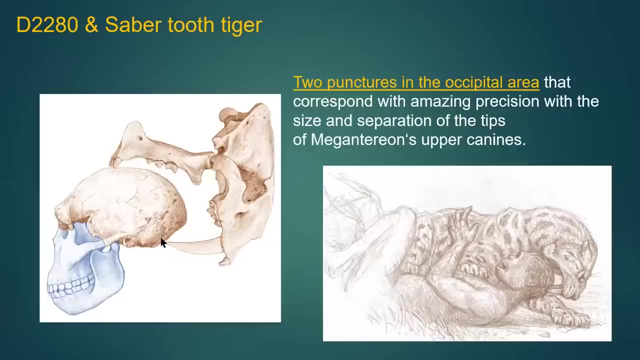 I keep getting people waiting in the waiting room messages, And so it's the world's first completely preserved adult hominin skull. It's beautifully preserved, basically, And one of them has the perfect puncture marks related to a sabertooth upper canine. 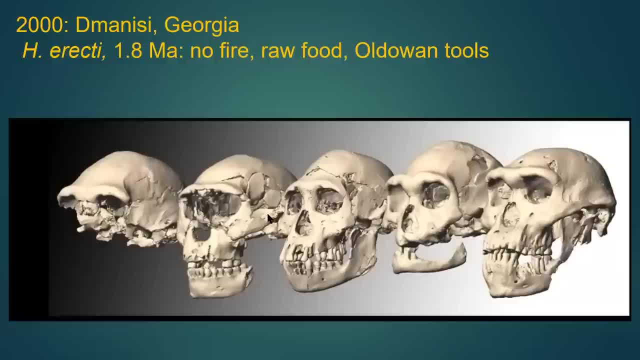 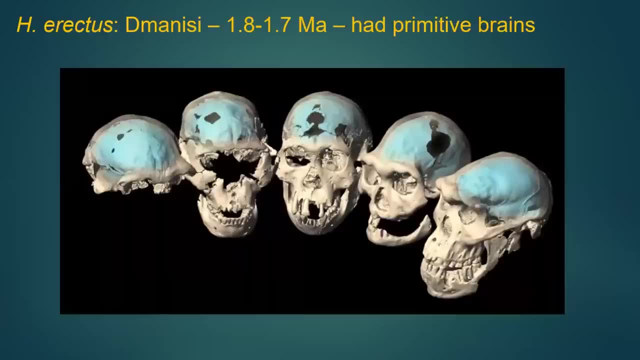 So this was a tough region to live in, And this is the most recent specimen coming out of the ground: skull five. I keep getting people waiting in the waiting room. messages to live in, basically: um so no, fire all the wand tools. uh, very, um uh, poor brain, uh, relatively. 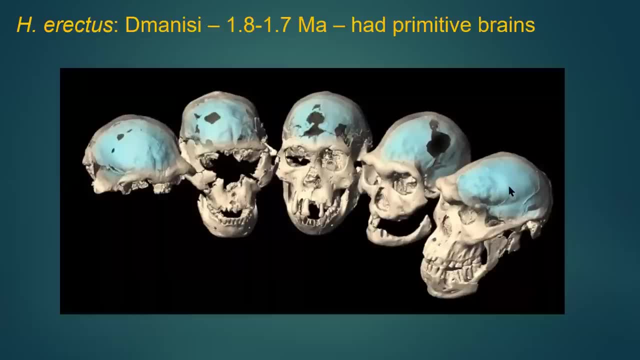 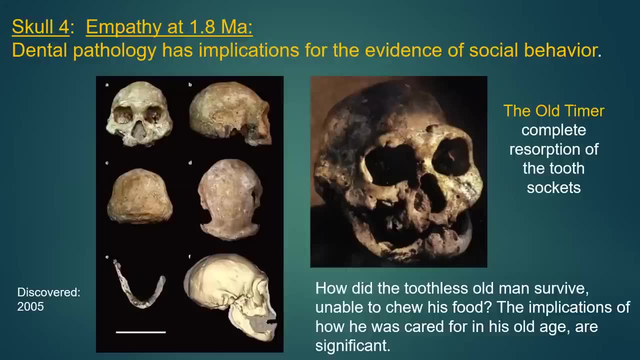 speaking, compared not much. uh, frontal lobe, relatively speaking. and then, um, we have the old timer. one of them has totally lost his teeth and the. there was complete reabsorption of the tooth sockets, which meant that he lived for a while after he lost all of his teeth, which means 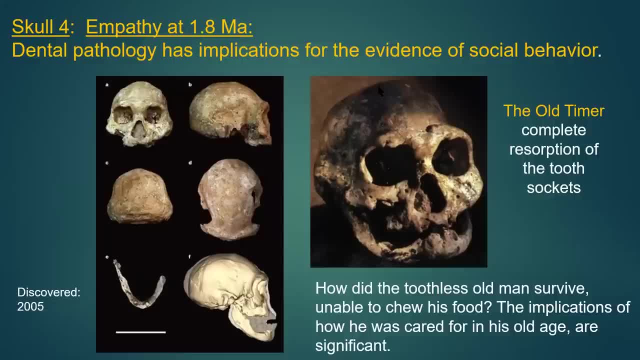 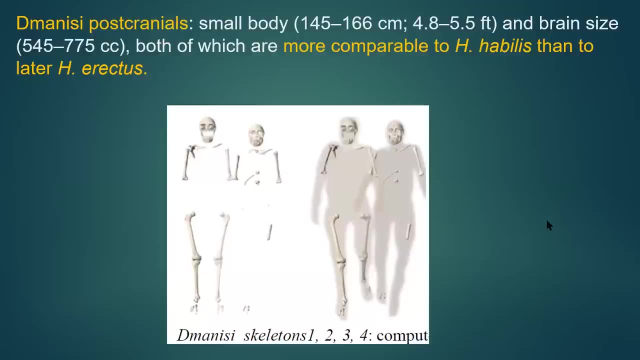 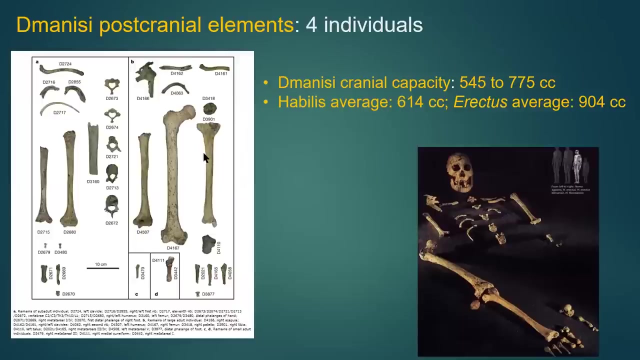 that basically, this is a potential example of empathy and caretaking. uh, almost two million years ago again, sociality was the way we survived and this is a good example to point out. there are post cranials available for this group. they think the um, uh, the brain size, um, populist was around 614, erectile typically around the. 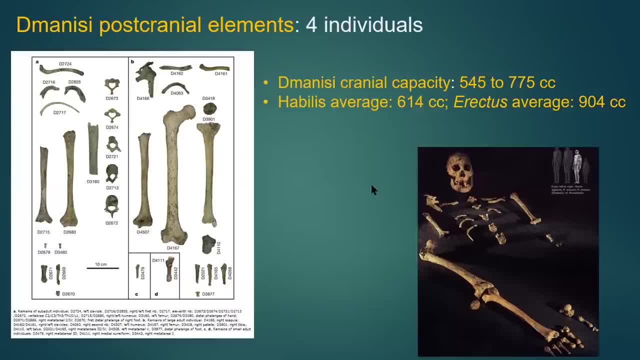 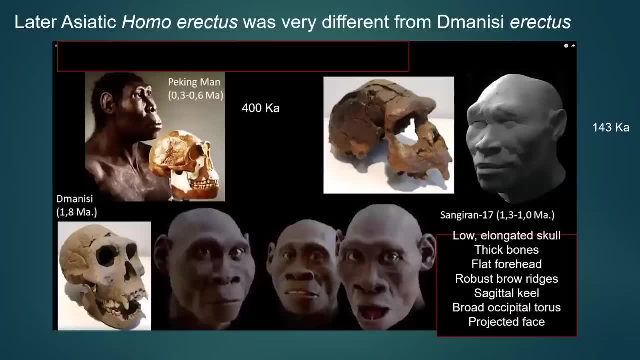 thousand mark and these guys are, uh in between, uh, there, um the later asiatic, um erectile like peking man at 400k and the indonesian san joran group who disappear at around 143. these guys are up to 1100 cc's, so they ended up moving around and, as 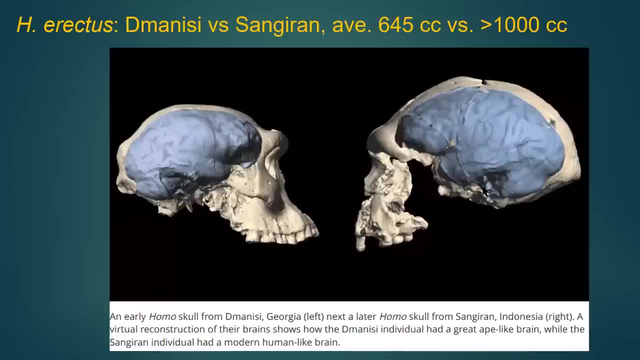 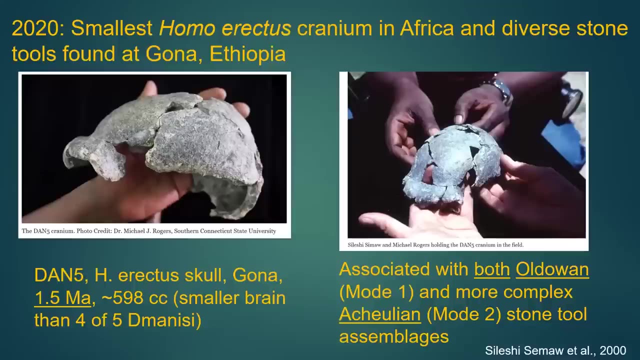 we'll see. uh, there's a connection to some islands as well. so demonese's brain um indonesian erectile brain- uh, significantly larger. and then, in 2020, the smallest homo erectus cranium was discovered, uh, with some small tools um, at dona, ethiopia. uh, so the these skulls were very 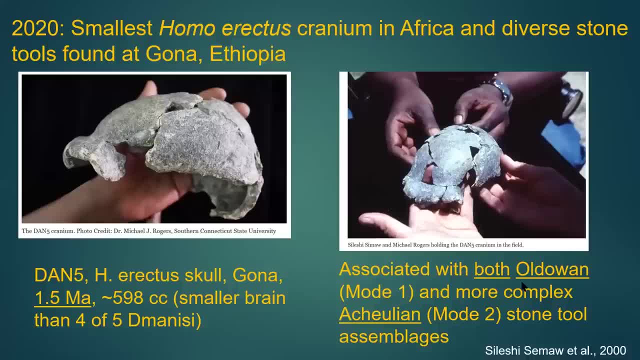 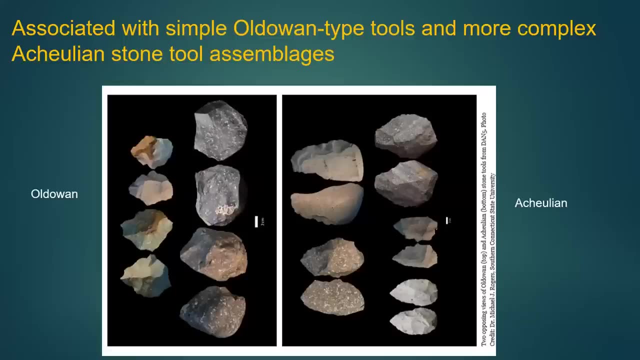 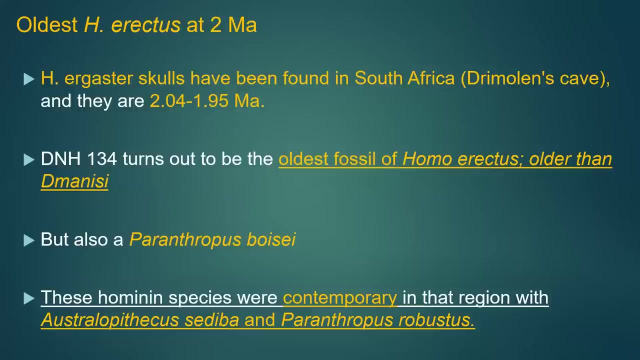 small. interestingly, um, they were found with both alduan and ashulian mode uh stone tools, so they were using both uh at this date of 1.5 million years. so old one uh plastic ashulian assemblages um the then they discover a homo ergaster skull that they date to just around 2 million years. 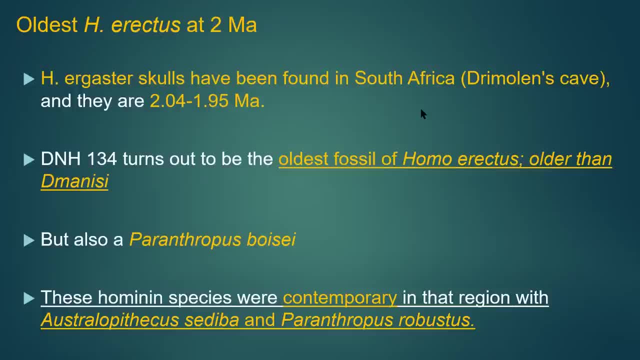 which makes it the oldest erectile skull available and uh, older than demonese. but also they find a paranthropus uh skull the same age. uh, quite neat. uh, it's quite unique and it affects the Helen Desmond. he was a famous professor of the University of California and then perfected it at the University of California in 1990 and he was a contact scientist at the University of California. so he was a fascinating professor of the University of California which I would be very happy to have a look at your work today, and I hope you enjoyed it. Thank you. 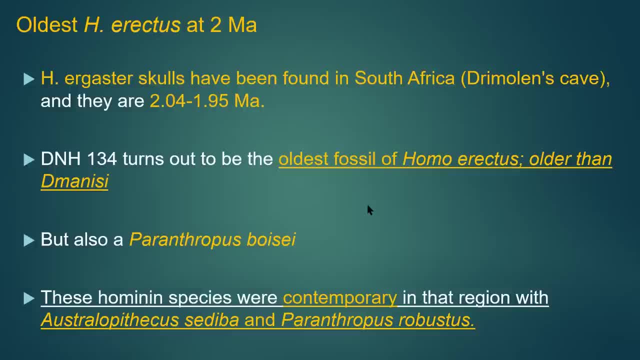 Um, All right, So the two oldest versions of these two that have been discovered in the nearby territory. We've got also Sediba and Paranthropus robustus. So examples of how multiple species in nearby territories not messing with each other for all we know, or who knows? 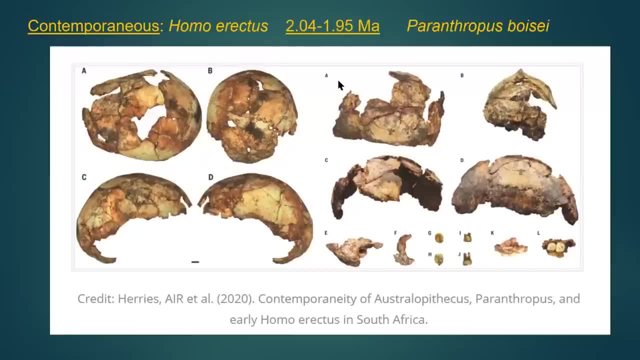 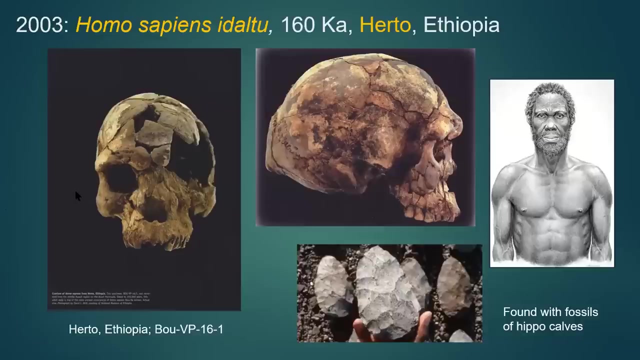 OK, but complementarity. This is the Homo erectus skull, This is the Paranthropus skull and partial identification because of their giant molars. In 2003,, Tim White discovers the Herto skull at 160 K. It's one. 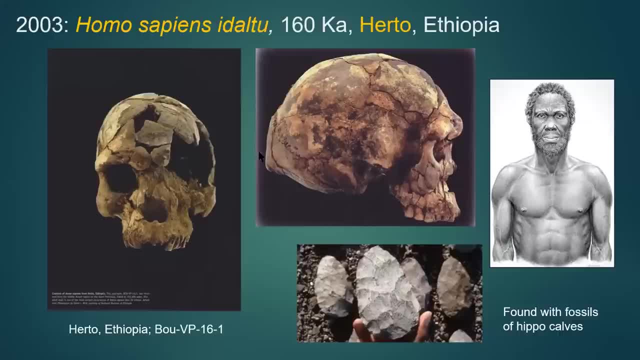 One of the first example where they start talking about globularity: anatomically modern humans because of the skull shape. But even this one is not totally globular. That doesn't actually happen until about 100 K, So found with hippo calves and tools. 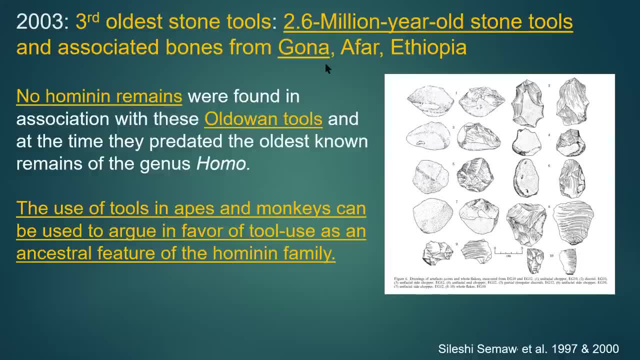 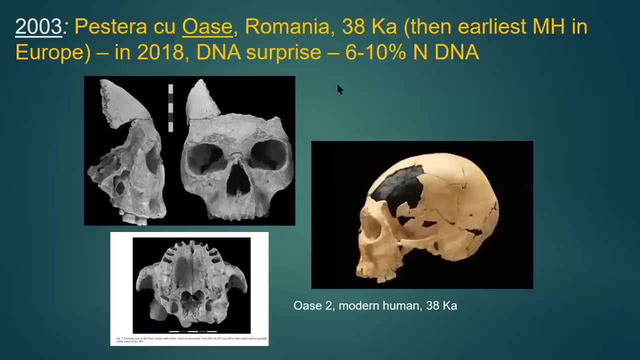 Then they find some tools again at Ghana, with no homo And in remains that are old the one, and these were at the time the oldest, old the one tools. then in Europe, in 2003, in Romania at a ways, they discover a 38 K hominid, modern human they believe, but in 15 years later they do the DNA. 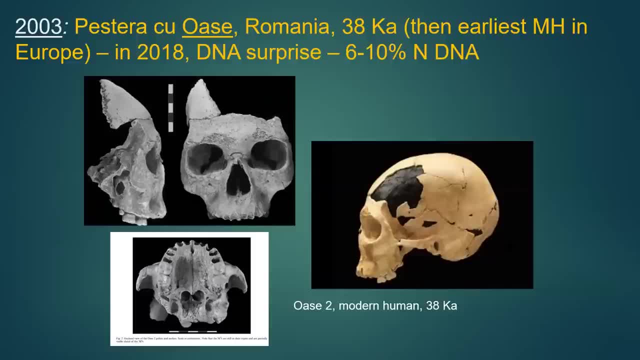 And they discover, And they discover He's got almost 10% Neanderthal DNA. So he's got a great, great grandparent who was a full Neanderthal And, as we'll see, almost all of the early hominins, that modern humans, African, modern given foragers who came into Europe around 45 K- all have the end of all DNA in them. 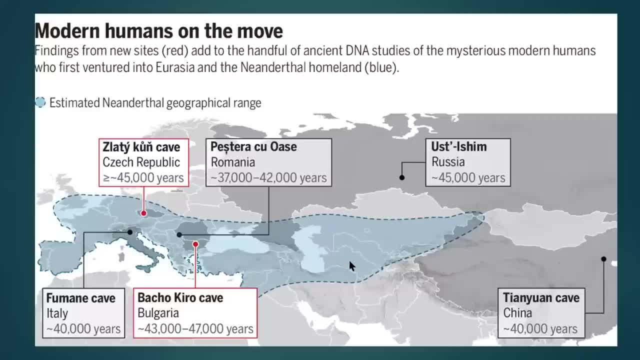 So these are the. So these are the the ones today. So these are the the ones today. Zloty Coon, Always A station in Russia and in Bulgaria. the Baku Kuro cave, are all in this time period when we moved out of Africa, probably at 50 to 60, but didn't enter Europe for another 10 to 15 K. nobody knows why. 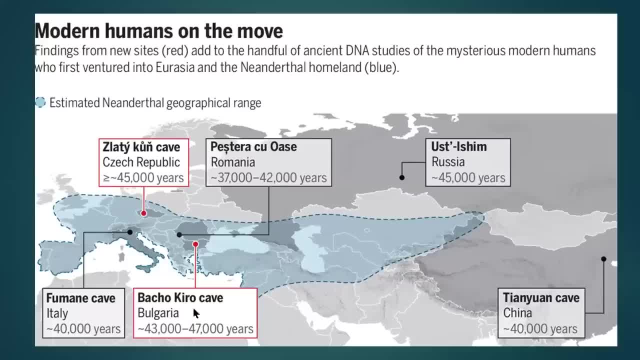 And in Bulgaria the Baku Kuro cave are all in this time period when we moved out of Africa, probably at 50 to 60, but didn't enter Europe for another 10 to 15 K. nobody knows why. All right, Probably because the Neanderthals were there. but 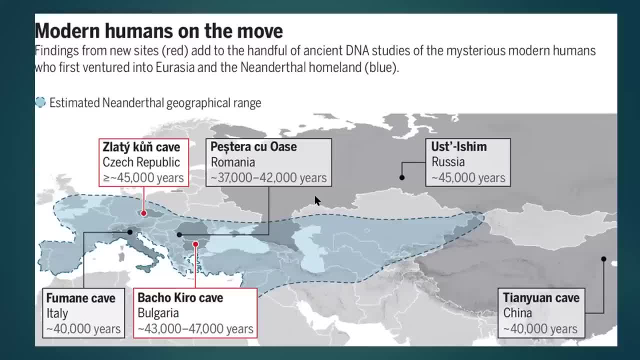 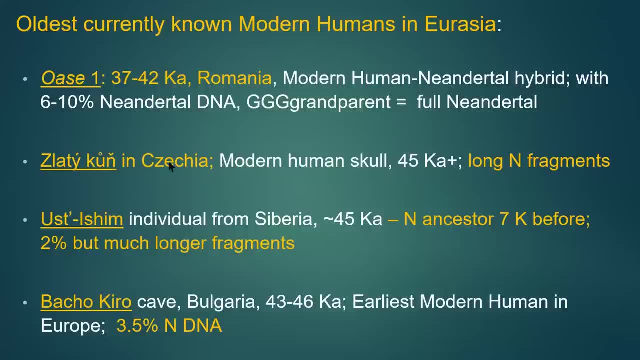 Probably because the Neanderthals were there, but All of them that we haven't currently discovered have Neanderthal DNA. All of them that we haven't currently discovered have Neanderthal DNA. So, and the other these guys down here all have much longer the André fall DNA fragments. 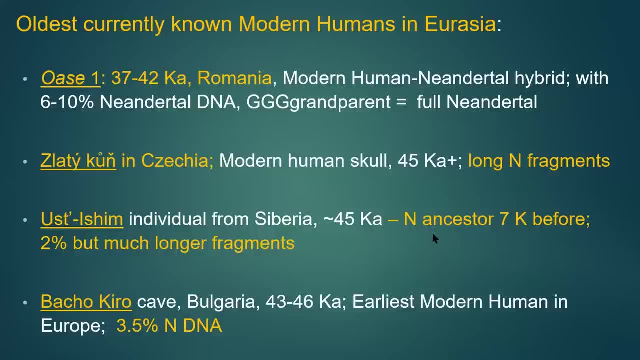 The characteristics of whether something is ancient DNA wise is: how big are the DNA fragments? uh? typically less than one millionth of a millimeter, kind of routine. but these guys had much longer sequences that were fully dna uh than we have today with our two percent um. so this is 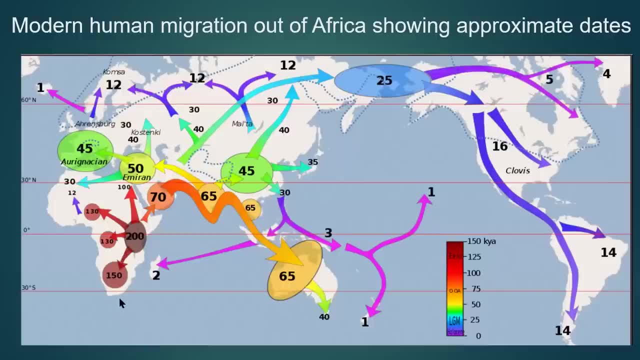 just the quick uh, uh migration out of africa routine somewhere between 50 to 70 is the big push out we've developed into what's considered anatomically modern humans and basically our hunter-gatherers, dark-skinned. we get to australia by 65k, we're in asia by 45k and move into 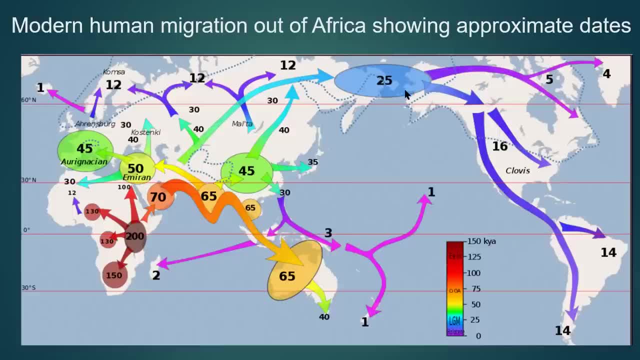 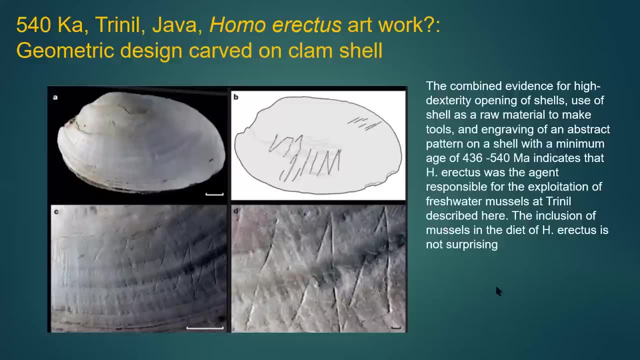 europe. we come across the beringian uh straight, uh at around 25k and into the americas, basically, um, this is the only artwork that i've seen that's been attributed to homo erectus, dated at 500k. basically, someone was carving some upside down v's and it's. 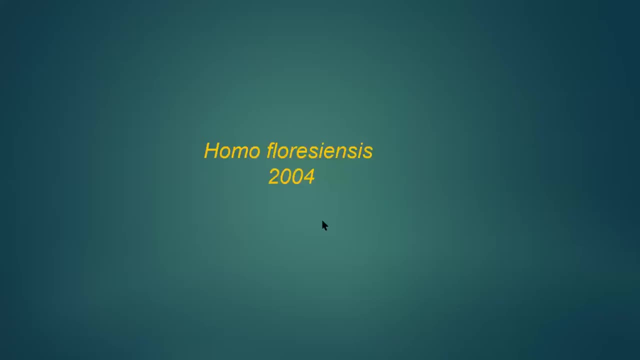 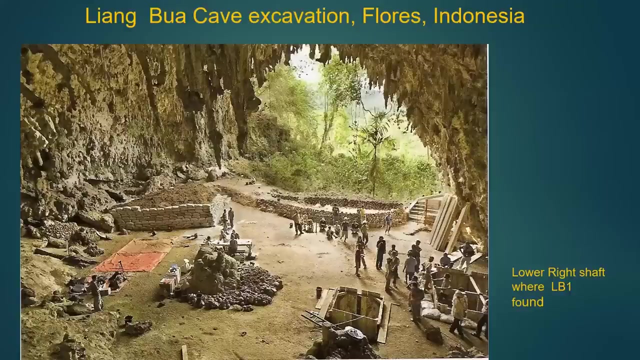 attributed to homo erectus. okay, um, then comes the big surprise of 2004. um, this is the, the lingbao cave in flores, in indonesia. the island is right next to komodo island. it's a giant cave and this is the area where they found lb1 flo. the hobbits got nicknamed. 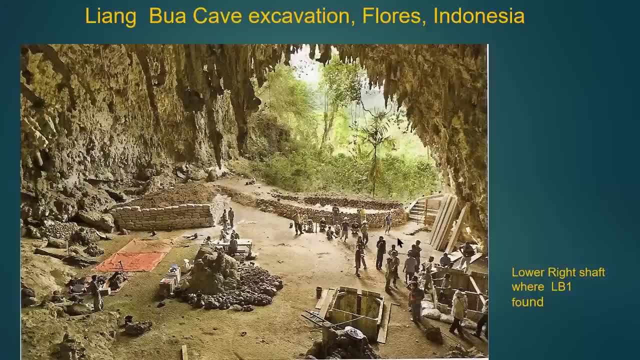 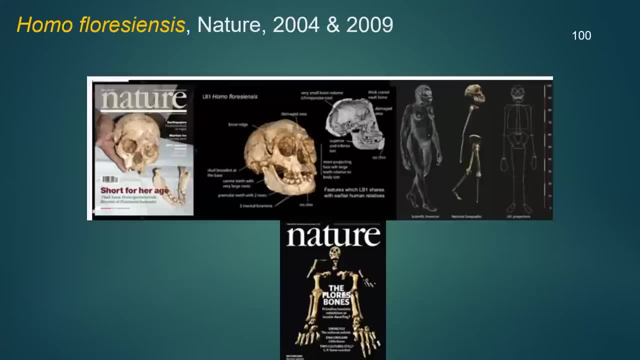 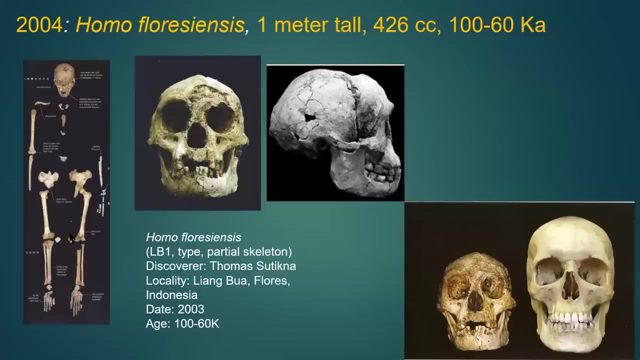 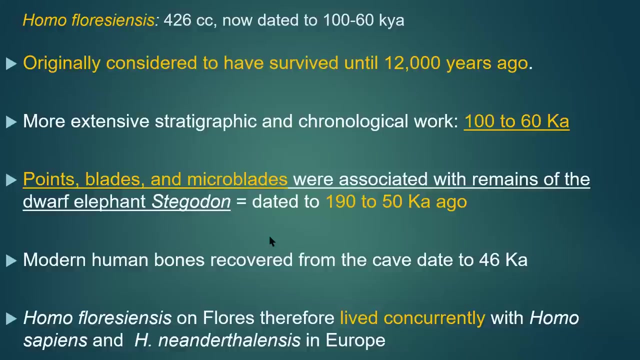 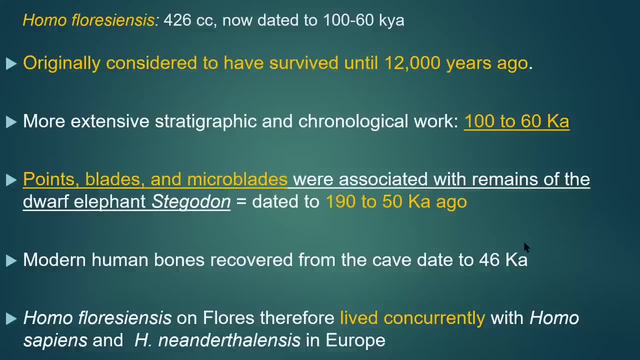 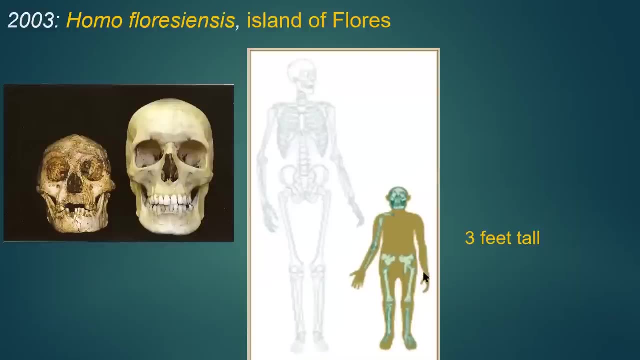 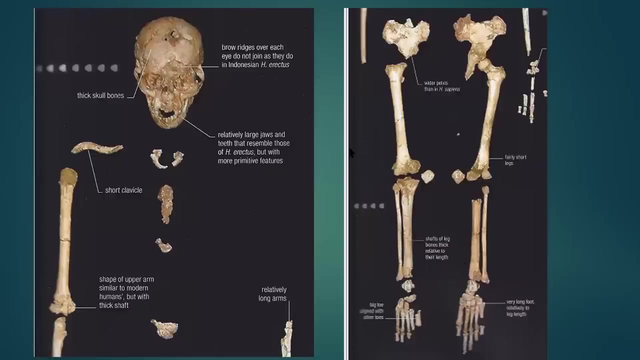 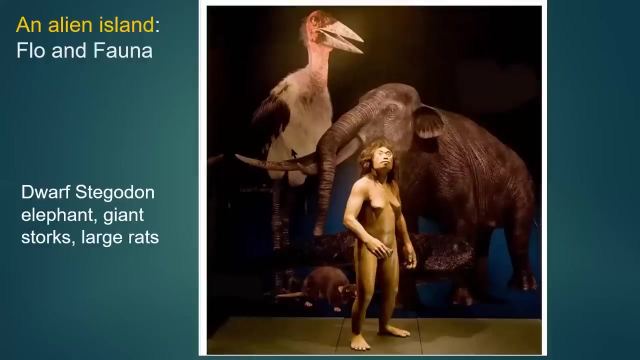 And so these guys live concurrently with sapiens and Neanderthal in Europe, but obviously never connected with each other. But diminutive three feet tall, And these are the post-Pranos. They got more than plenty of places do. They hunted giant rats, Komodo dragons, seven-foot storks. 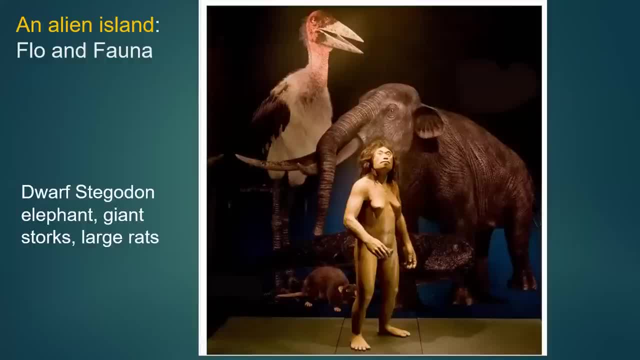 and dwarf Stegadon elephants. So a weird island. These two guys dwarfed. These guys grew extra big. OK, That's what happens when you get trapped on an island for hundreds of thousands of years. I was born on the island of Malta. 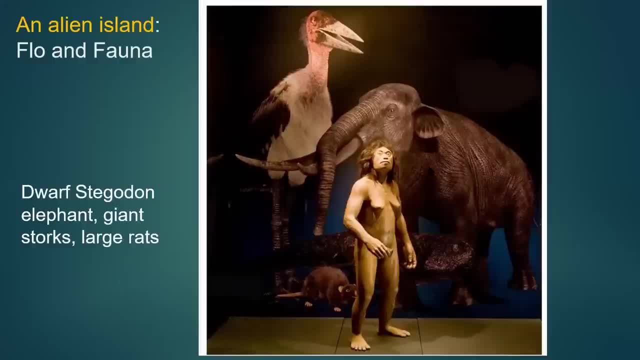 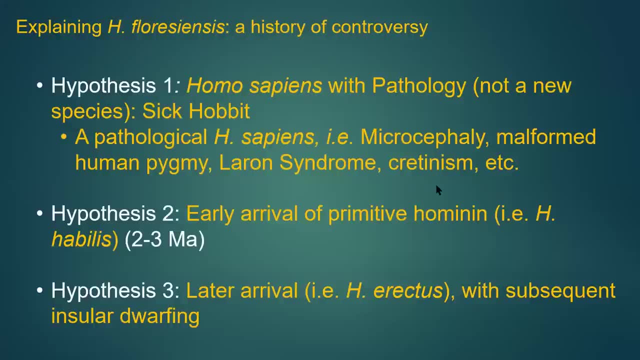 And we have Stegadon dwarf elephants on the island, like Pete does, et cetera. So islands are interesting evolutionary workshops. Huge controversy at the beginning, multiple hypotheses. The first one was that this is a Homo sapiens with a pathology. 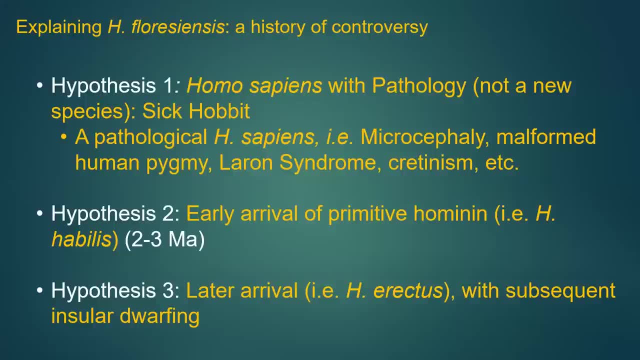 It is not a new species, It is a sick hobbit. Theories of microcephaly, malformed human pygmy, loran genetic syndrome, fretonism et cetera. Nobody buys that anymore. Second hypothesis is an early arrival. 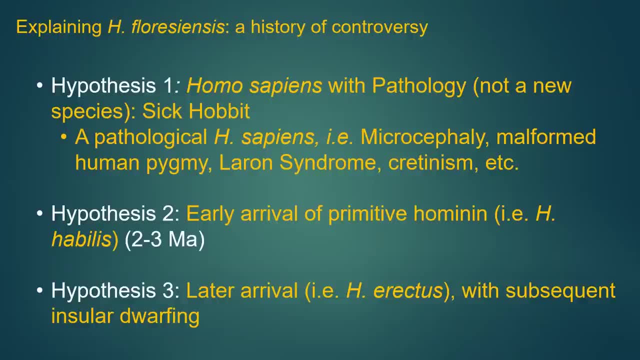 of a primitive hominin, ie habilis, from two or three million years ago. Last hypothesis: This is a later-arriving Homo sapiens. This is a later-arriving Homo sapiens. This is a later-arriving Homo sapiens. 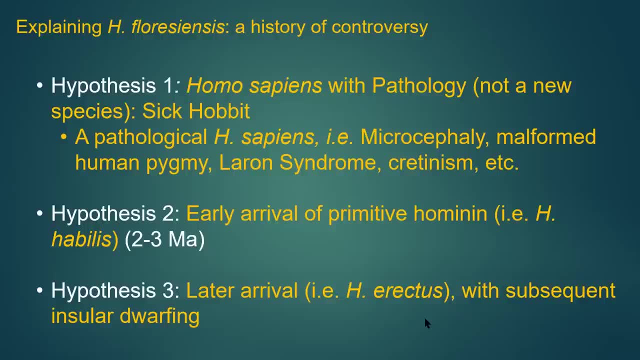 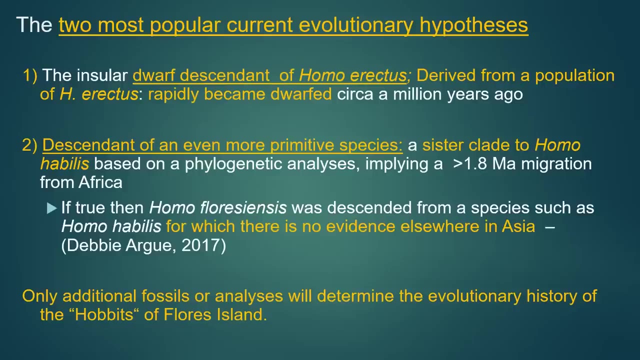 This is a later-arriving Homo erectus And that Flores is basically an example of an erectus having insular dwarfism, that if you get onto an island and are big and there's not enough food, you begin getting smaller, And that is currently the leading theory. 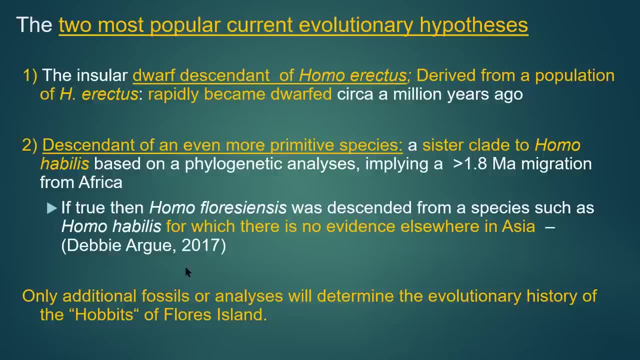 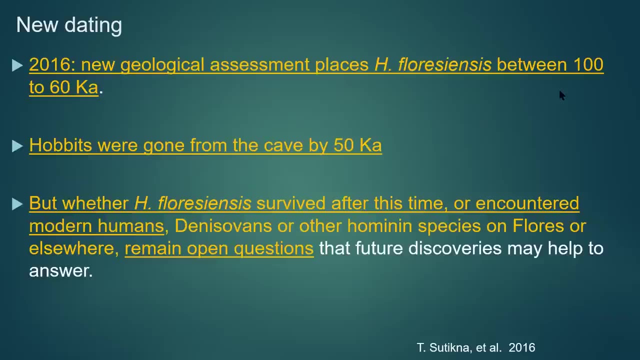 although the last big study by Debbie Arguey thinks again that it's a sister. It's a sister clade to Homo habilis. So the controversy goes on. The latest dating puts them again at 100 to 60k. 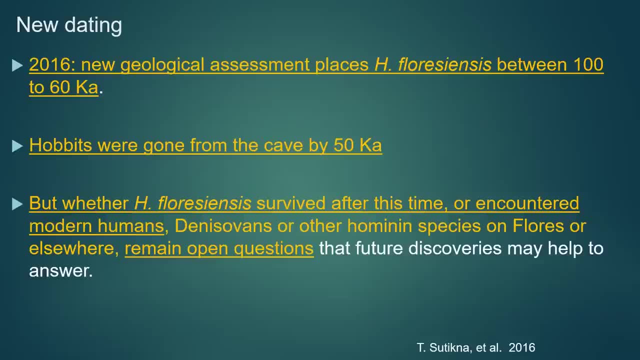 with the bones that were found And they're gone by about 50k, because at 46k you get a layer of modern humans in the cave. So, but again, continued questioning of flow and other things. It's a very similar hypothesis. 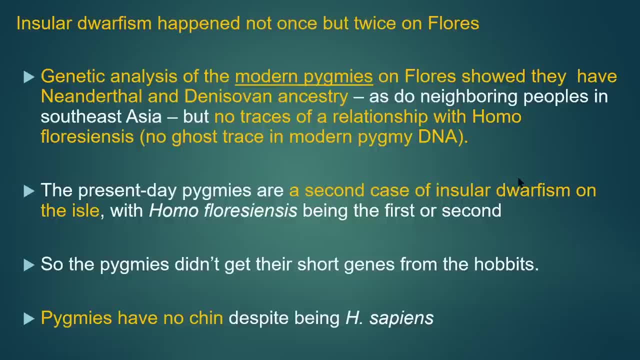 But it's also a later�ar experience. So this was a study by the University of Michigan, which the University of Michigan worked on. This is a research study and how she got there, etc. um, the uh. they've attempted uh dna um on flow and it didn't work. 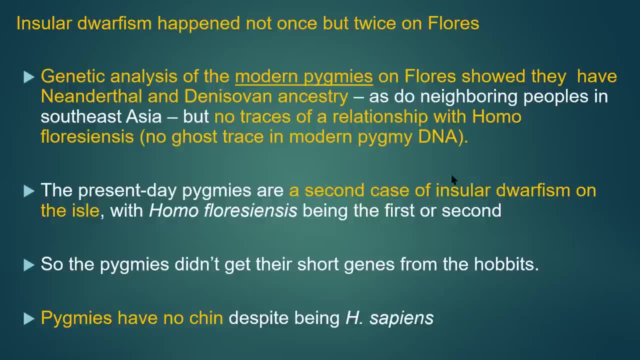 there are present day flores pygmies. so dwarfism happened twice on flores, once with uh, uh floresiensis and this other uh interesting group, this modern human group, or pygmies, have no chin. okay, interestingly, and when they did the dna of this group, uh, they show that they had. 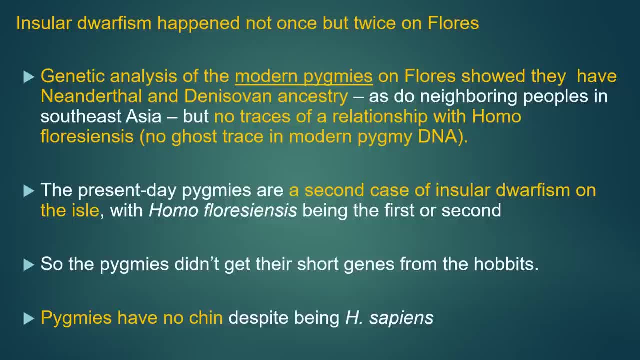 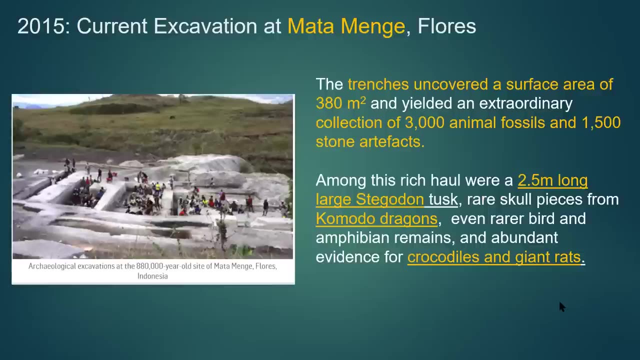 a neanderthal and denisovan ancestry, modern human ancestry, but no traces of any ghost uh geno ghost trace that could indicate uh flow and her gang being connected. they're not. previously there had been ongoing excavation at a place called uh uh matamenje, which is about 70 miles from the cave. 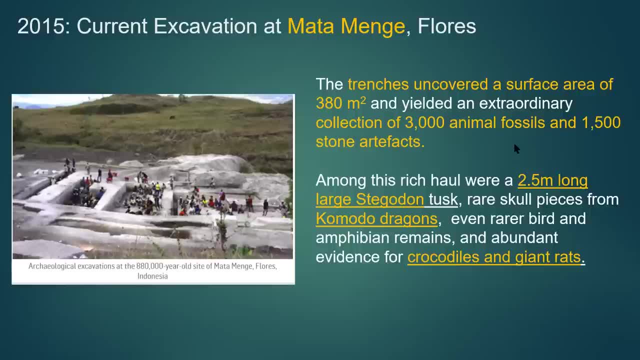 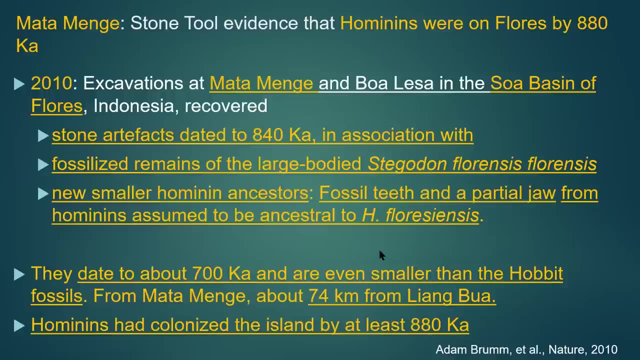 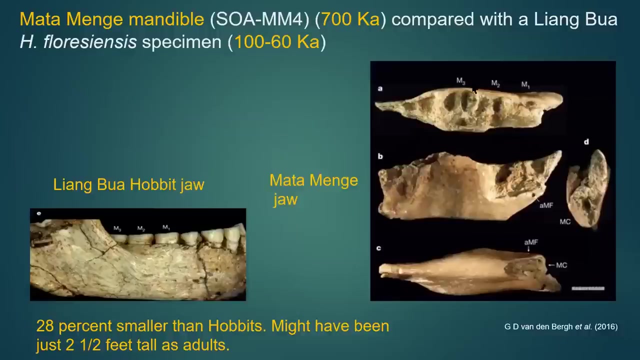 and they found 3 000 animals, fossils, 1500 stone. they've got large stegadons- not dwarf- and large komodo dragons at this site, giant rats as well, and they've dated this group to at least uh 700k uh. so, um, there's this alternate group and the discovery of an even smaller jaw. 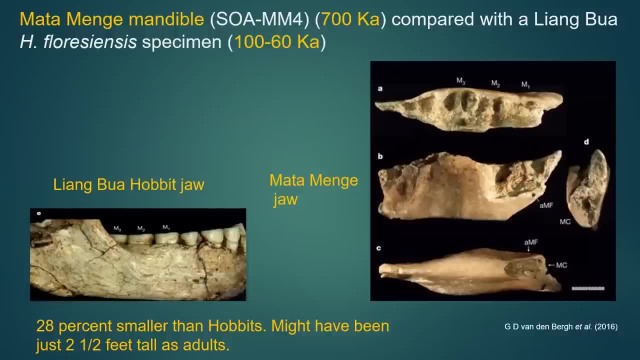 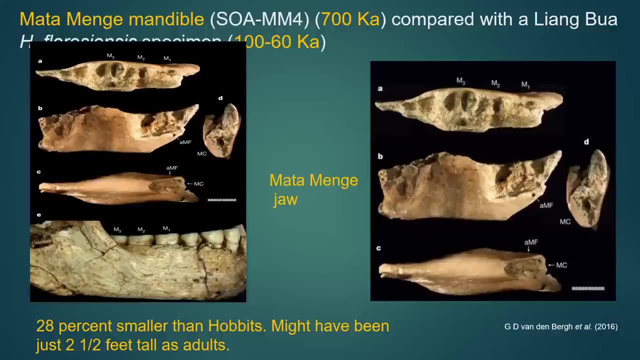 that's 28 smaller than the hobbits. um, at leon. wow, this group may have stood two feet tall, okay. so in comparison to flo's jaw, this is the size of their jaw. so we have a pre-existing? um, they have not named this species, okay, they just think of it as ancestral to the flow uh group on the island. 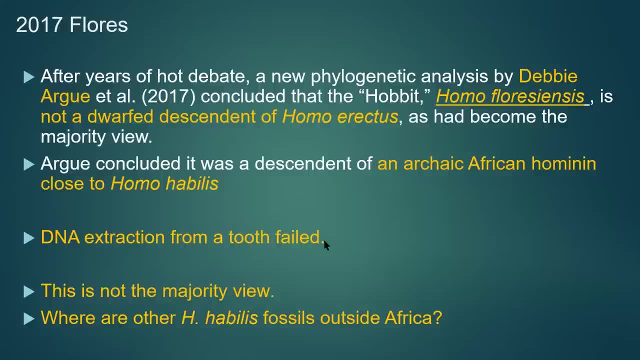 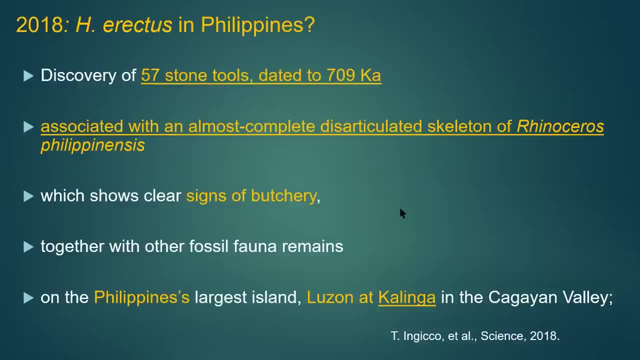 uh dna extraction has failed um and and uh, so continued continuing to come information. basically they in 2018. they Heil chaturk. guide name is Ensler billy and management has been associated with fo個n missionary density. origin. They discover 57 stone tools dated to around 700 K and associated with a rhinoceros Philippine ensis skeleton that's been cut, marked and butchered. 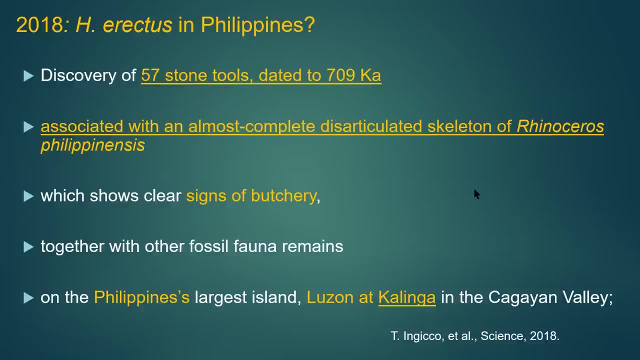 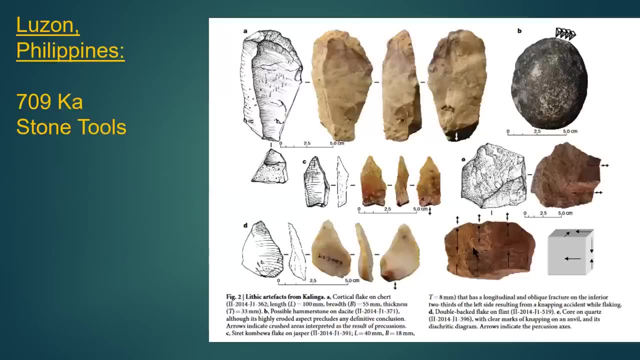 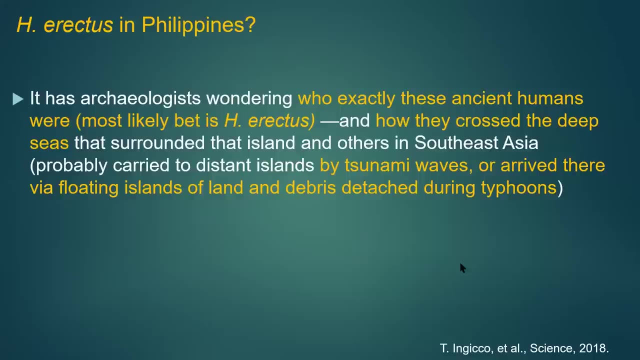 And they think this was probably Homo erectus- on the island here in the Philippines with these stone tools. They haven't actually said Homo erectus, but that's the thinking, And the idea for these islands is that there was a tsunami wave or floating island of land and wood debris that detached during a typhoon and ended up on the island. is how these guys get there. 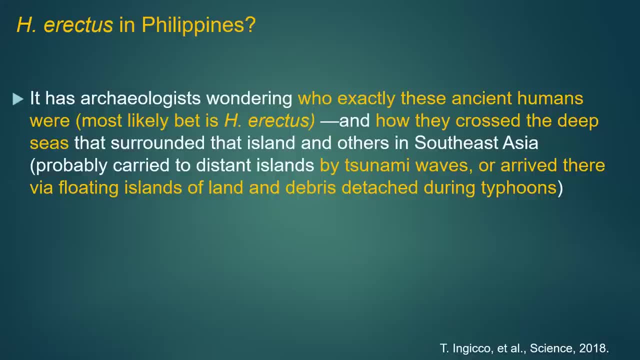 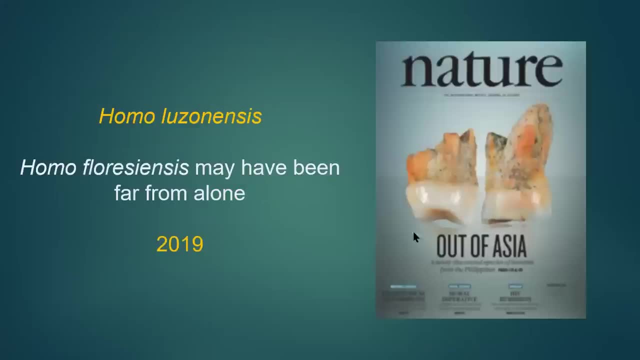 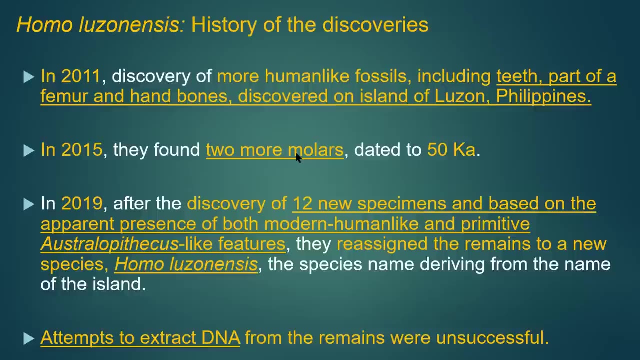 I'm betting that the Indonesia in the next 20 years is going to be a hotbed of discoveries. OK, We will see. And then, of course, another one. Flo was not alone: Homo luzon zensis on the island of Luzon in the Philippines, the big island. 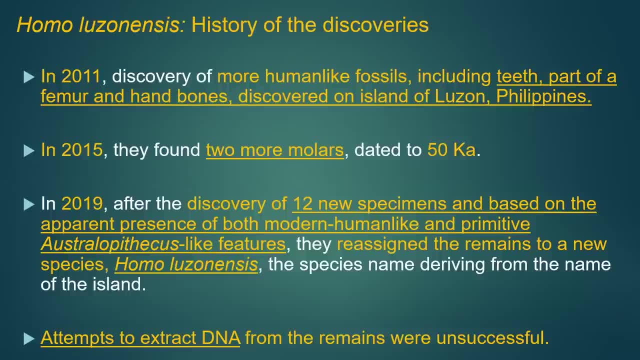 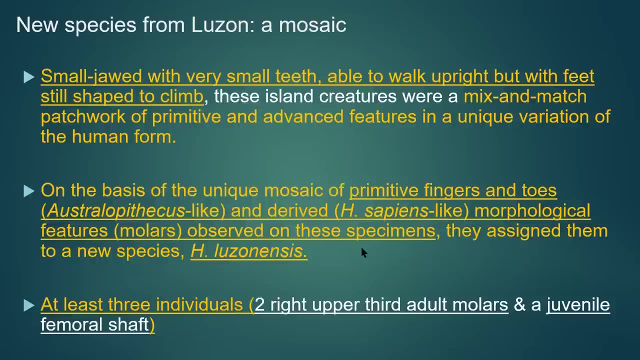 They find teeth, part of a femur and some hand bones. more moldings then, and then 12 more specimens which are both modern and primitive looking, And they attempts at DNA. We're unsuccessful, but they name it as a new species. 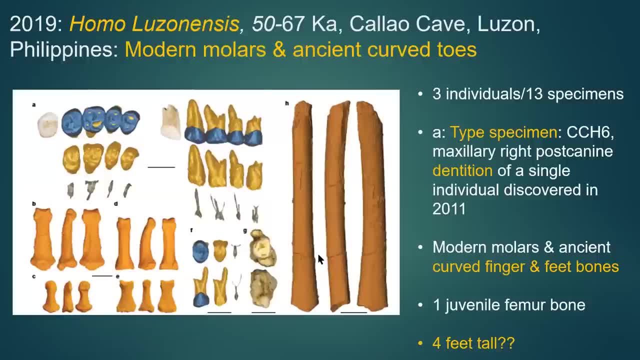 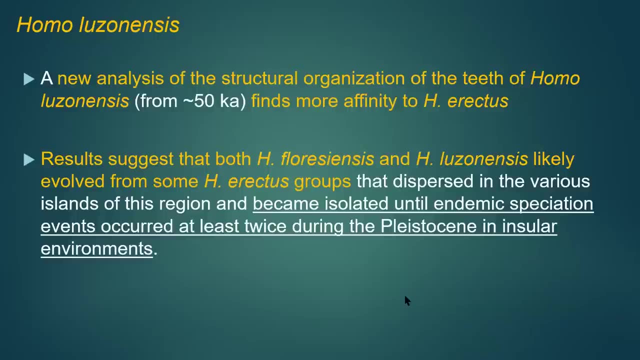 There are these three individuals here with some parts of femur and a bunch of teeth and some very curved finger bones, So again like a flow, a kind of mosaic basically. So again like a flow, a kind of mosaic, basically. 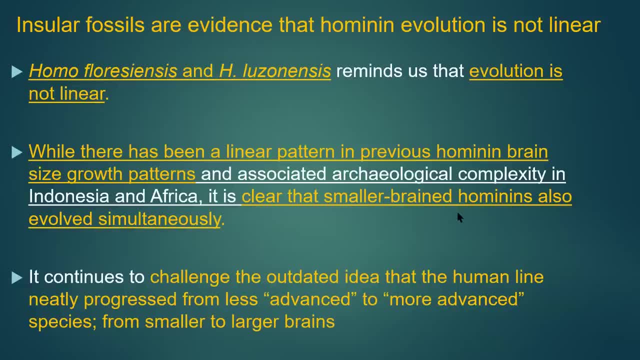 Capable of walking, but also capable of climbing, And this. these clearly indicate that evolution of hominins is not linear. OK, here we have, at the same time period, modern humans with big brains in Africa, And then we've got these small brained, small brains. 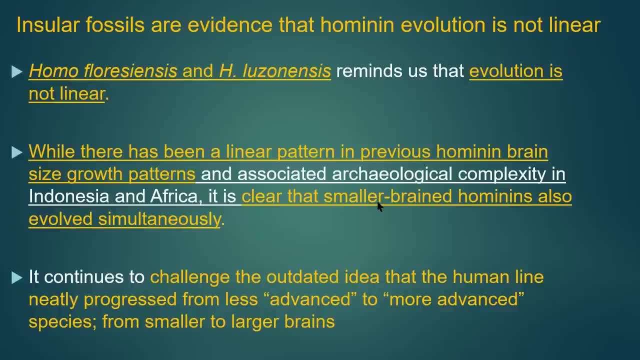 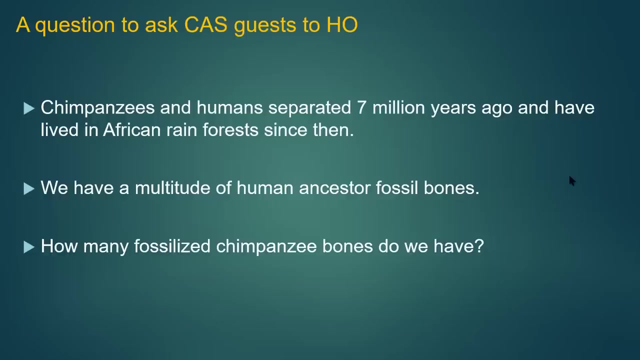 And then we've got these small brained, small brains in Africa sized hominins in the island. So it clearly challenges the outdated idea that human line neatly progressed from less advanced to more advanced, smaller to larger brain, etc. We need to keep thinking our model is more like a bush braided stream, etc. One of the questions 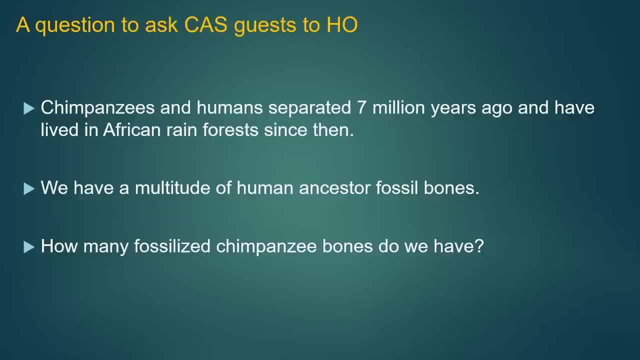 I liked when I showed the chimpanzee skull is that chimps and us separated 7 million years ago and lived in African rainforests. They did since then. We've got a multitude of human ancestor fossil bones. The question I asked the people in front of me: how many fossilized chimpanzee? 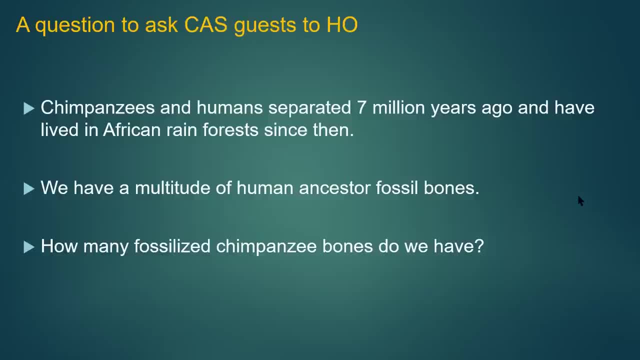 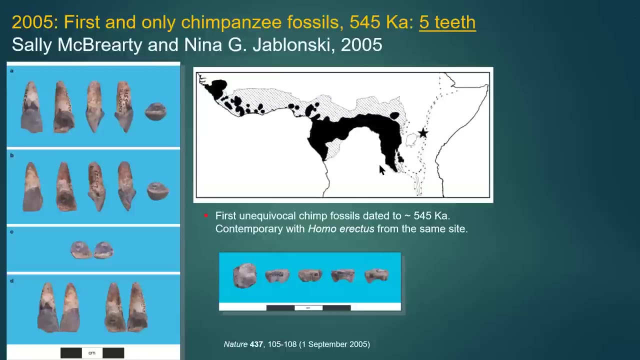 bones. do we have Anybody that know the answer: None, Okay. Well, the answer is none, Okay. Seven million years: no fossil chimp bones or gorilla bones. The only findings by McBrayer T and Jablonski is that they, in 2005,, discovered five 500,000-year-old 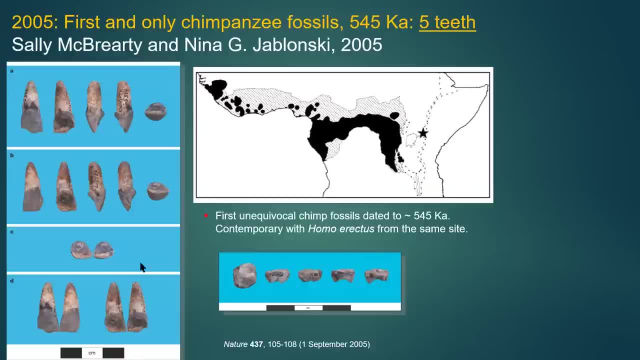 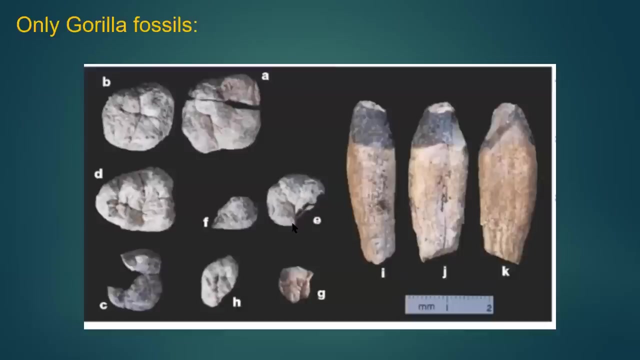 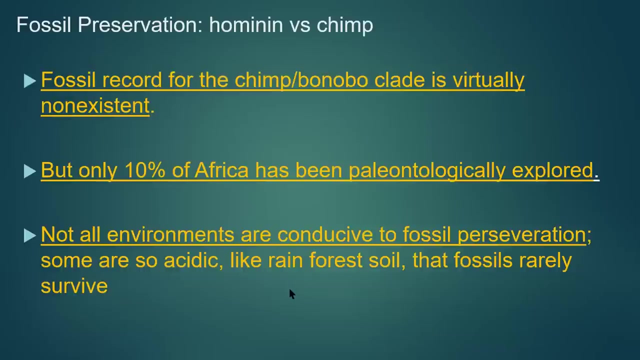 chimp teeth. these teeth right here. That is the entire collection of chimpanzee fossils. Okay, Remember that 7 million-year-old Sahelanthropus lived in a forest, but was found when it became desert. Okay, These are the only gorilla fossils that we have, So fossil preservation is the issue. 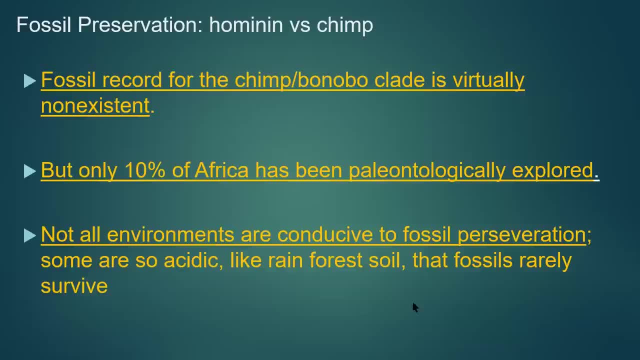 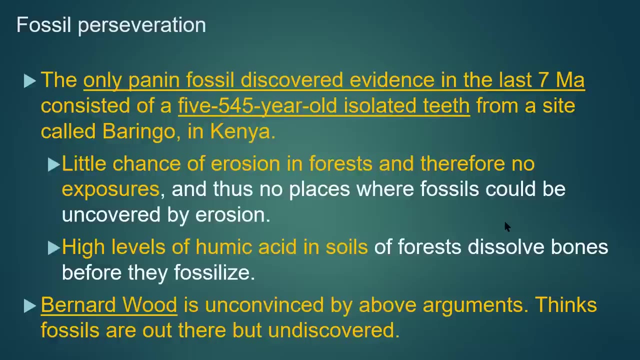 here. Only 10% of Africa has been explored. Not all environments are conductive to fossil preservation. Rainforest floors are acidic And, as a consequence, they eat bone, And these are the only ones. we found high levels of humic acid in forest soil. Bernard Wood from U Washington, who I 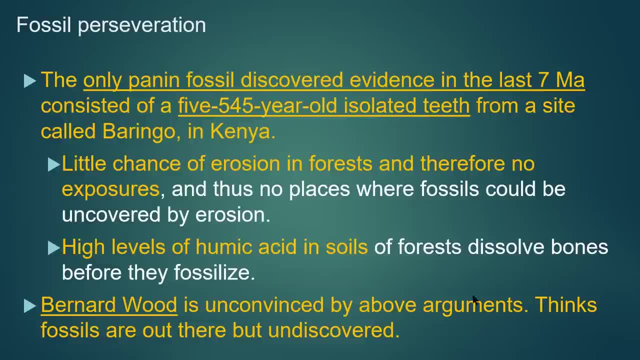 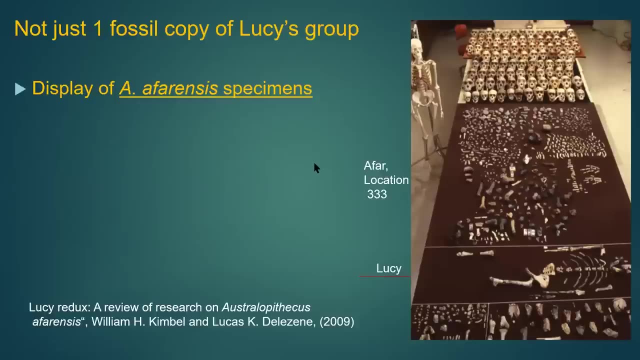 love, is unconvinced of these arguments and thinks we just haven't found them. Okay, That they're out there somewhere, just like Sahelanthropus. We eventually will, And just I love this picture because it shows. this is a display of all of the 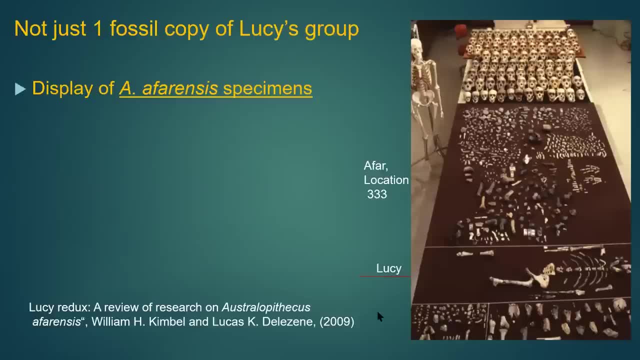 afarensis specimens that we have. This is Lucy over here And by 2009, we've got 400 specimens. We've got 96 Lucy-style afarensis skulls. Okay, Lots of repetition of the same, So. 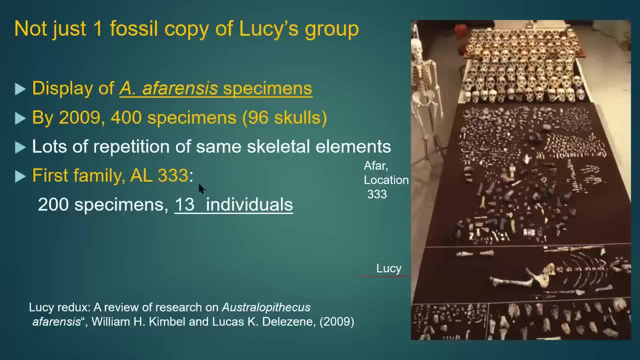 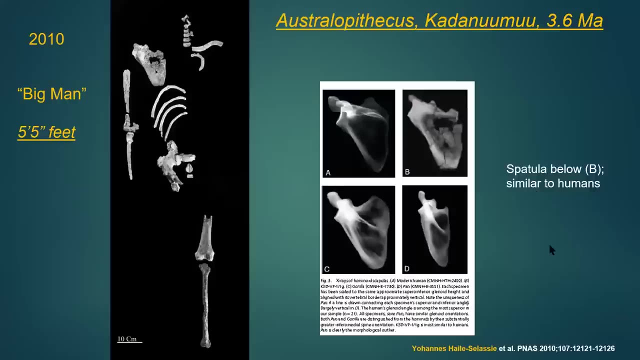 here's a photo of Lucy. Awesome. This woman is a little bit waiver for what we call the late 13th century, But even before she's built up to be an African American, she was like: you need this for their properties. this is what it looks like, And there's a little bit of like. 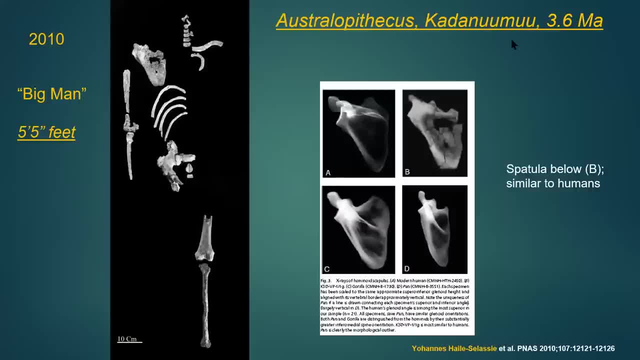 a Beverly Hills someday, But so we can talk about those, And then I'll also give you some more background information. So when I was just talking to the last student, I just noticed that there are a lot of these and I think a lot of it is really amazing. So now we're going to talk about what we've done in the 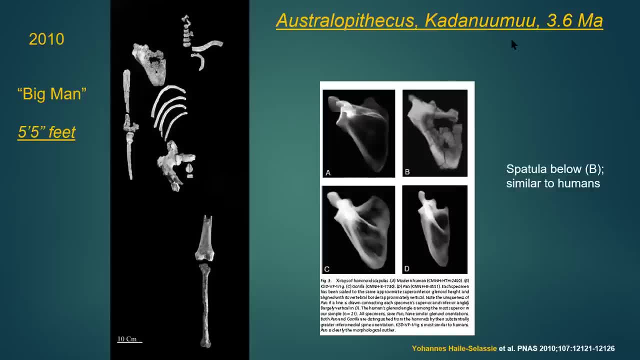 construction of fossil experience. So the first family that we've got is the form of a skeletal element, Banu Mu, from around 3.6 million years, same time as Lucy or so Big Man, this guy was 5'5" okay. 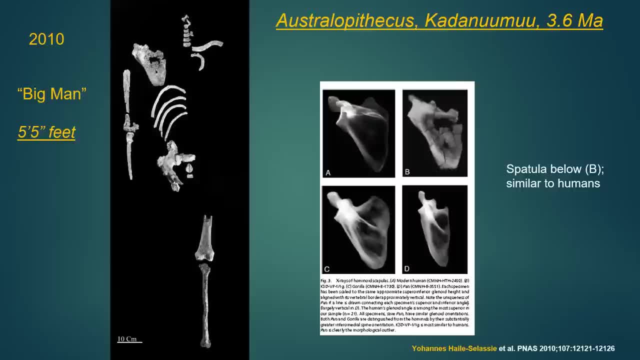 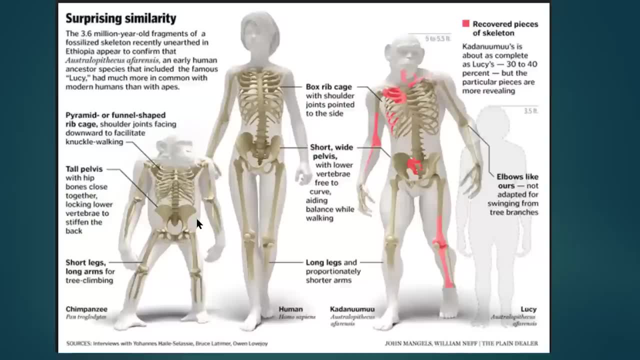 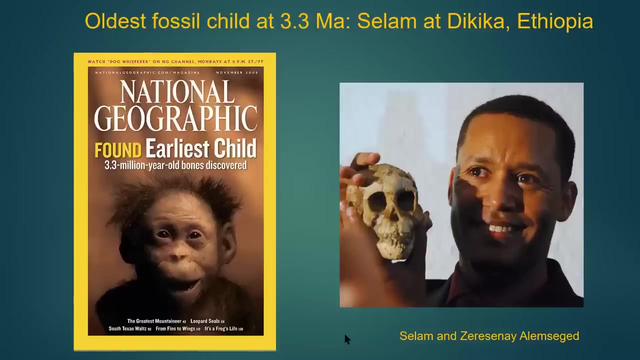 So whether this was the dimorphic male sex version of Afarensis kinds of species. so chimpanzee us him and Lucy for comparison. okay, So lots of variability out there historically. Then we get our place's hotshot, Salam, discovered by Zeray Al-Ghed. 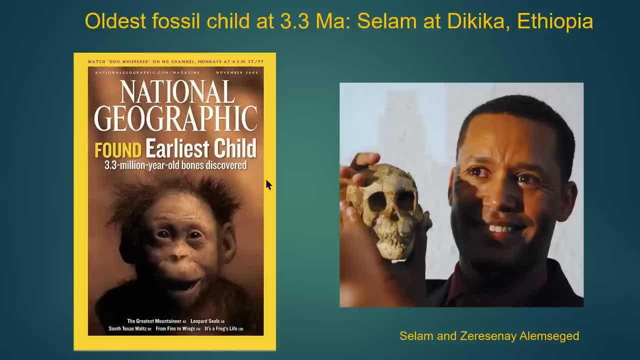 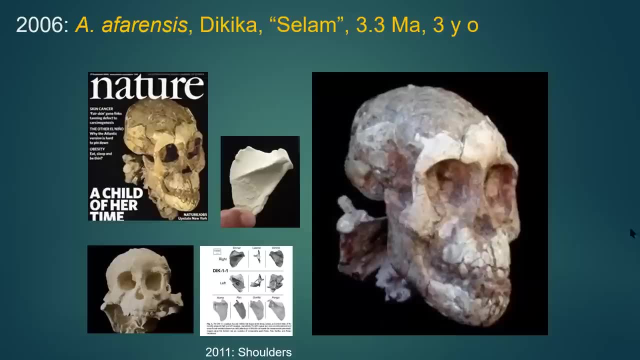 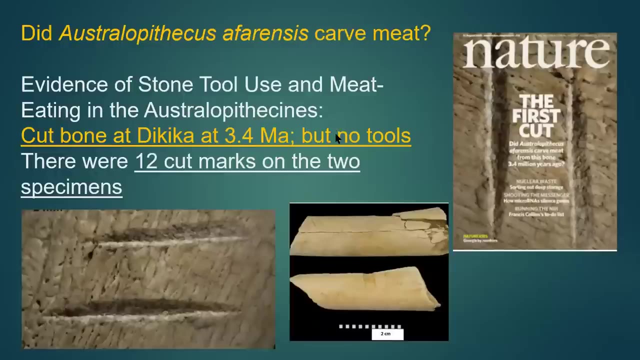 and the earliest Afarensis child that we have, basically at 3.3 million years. okay, And of course, it took Zeray six years to get this fossil out of the stone. okay, Good tale Stone. 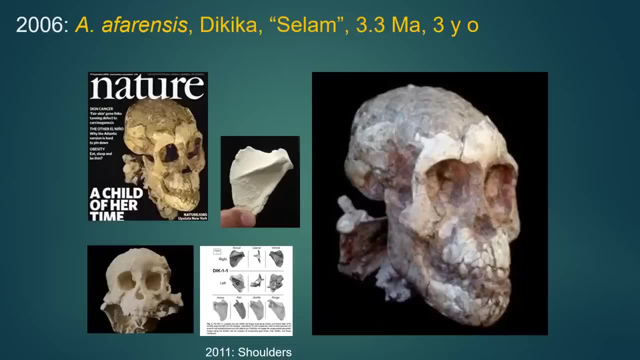 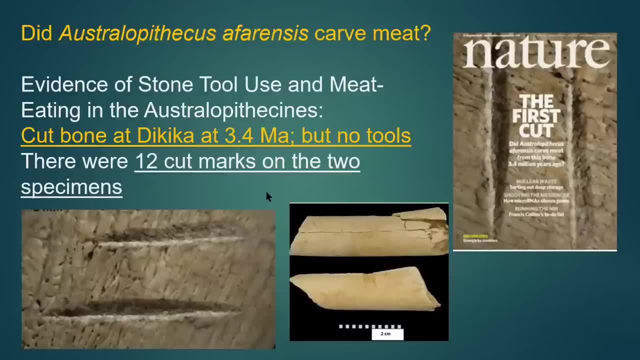 Skull Stone Stone. sorry, you're right. So this is at Dikika. And then Zeray also became famous because he claimed that a cut bone at Dikika at 3.4 million years showed that Australopithecus were eating. 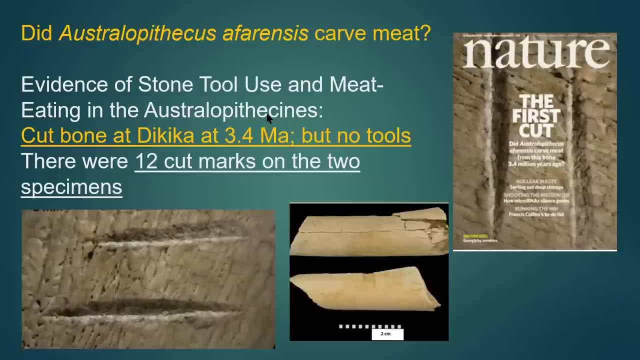 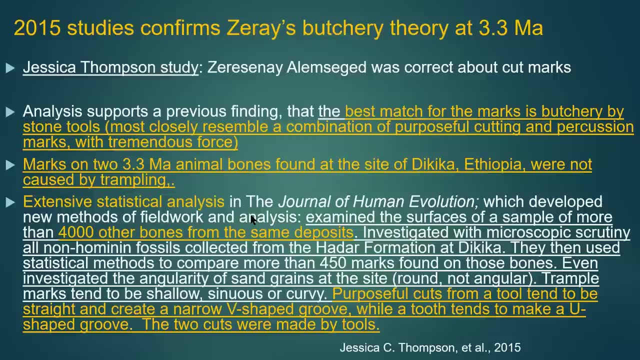 eating meat and using tools. okay, There are 12 cut marks on two specimens. It was highly controversial at the time, but a researcher named Jessica Thompson did an amazing statistical study of 4,000 bones around the same site and showed that the cut marks were consistently more like those made by a stone tool rather than by 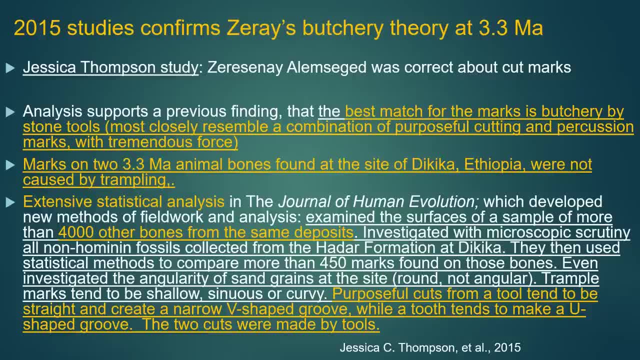 you know a stone tool. You know a stone tool Either being bitten or being trumped upon. so supporting his idea that this, in fact, was an accurate conclusion that again, Australopithecines were using stone tools at 3.4.. 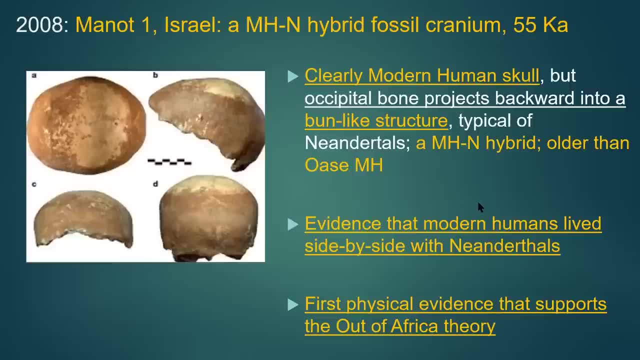 Minot. I was found in 2008,. a clearly modern skull, but it's got a bun. And what are buns historically characteristic of? It's a Neanderthal skull sign, and so they think this is a modern human Neanderthal hybrid. older. 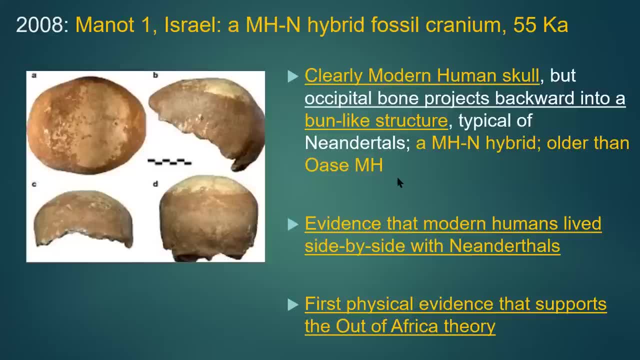 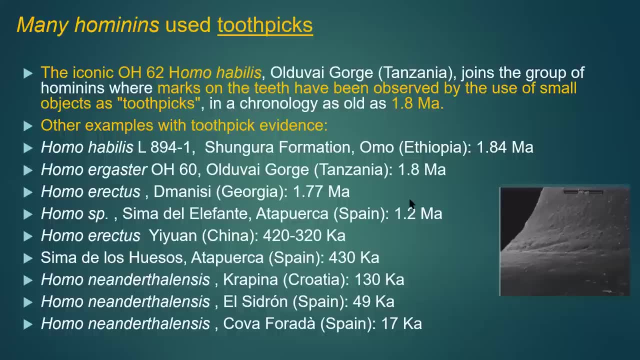 than the Oase modern human that we just talked about, and they consider this the first physical evidence that supports an out-of-Africa theory at this time. Just for a quick comment, we've got lots of cut mark data to indicate that everybody. 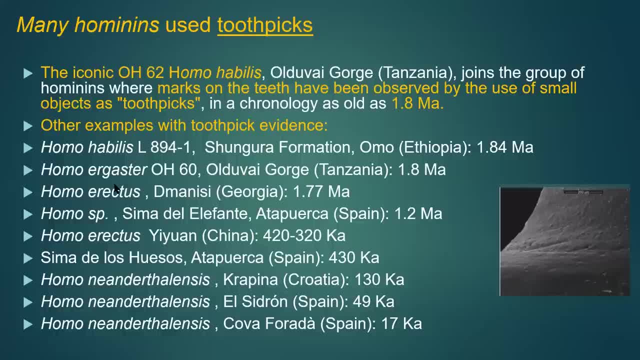 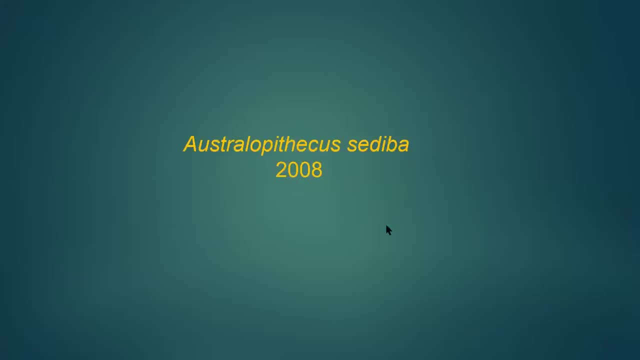 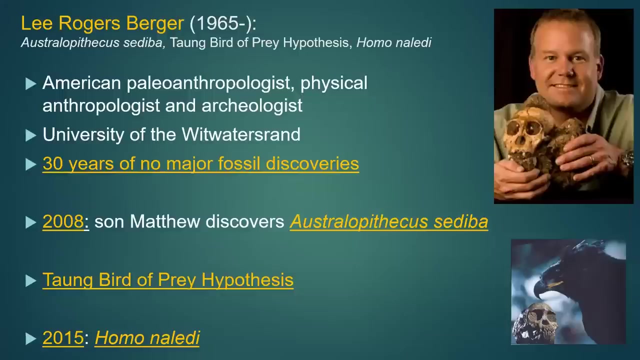 beware of the U-shaped. only used tooth picks forever. Okay, I'll be less, or gaster Neanderthal at Crippina and El Cidron and Spain, etc. etc. Okay, Then comes 2008,. Sadiba Lee Burger. 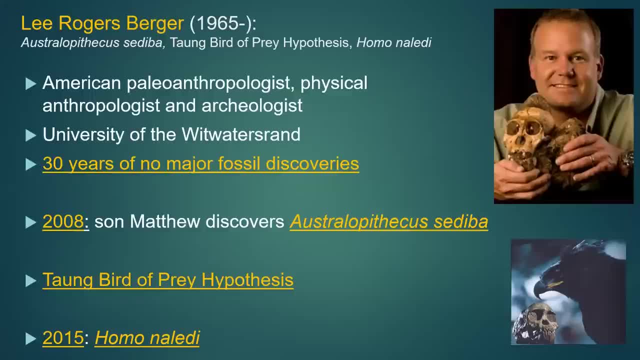 I have a mixed relationship with him of this water strand: 30 years of no major fossil discoveries And then, in 2008,, his son Matthew stumbles across a bone that turns out to be Australopithecus sediba. He's also famous for the Tong child bird prey hypothesis. 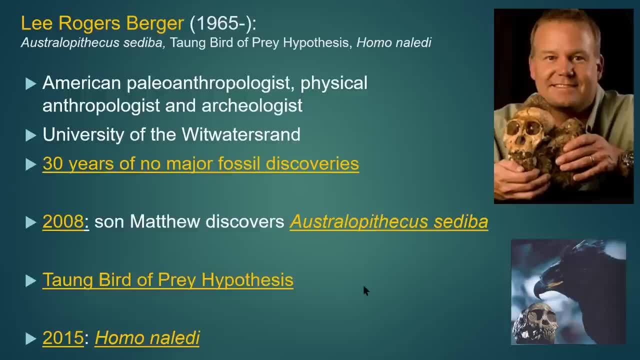 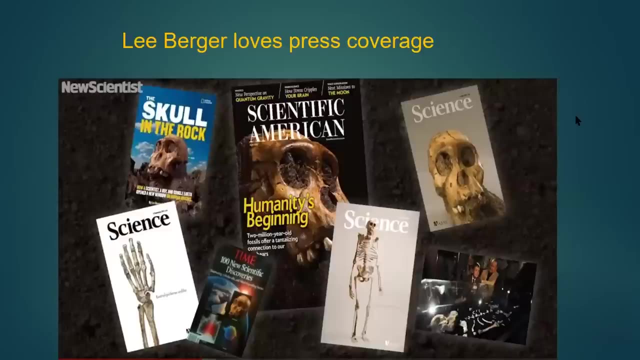 that there's good evidence that the Tong child was lunch for an African Eagle. okay, That's how he died. And then, in 2015,, of course, comes Home Owned Living. So Lee Berger loves press coverage. okay, That's how he makes his money. 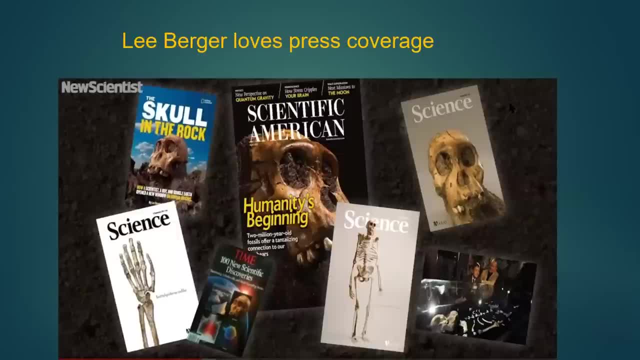 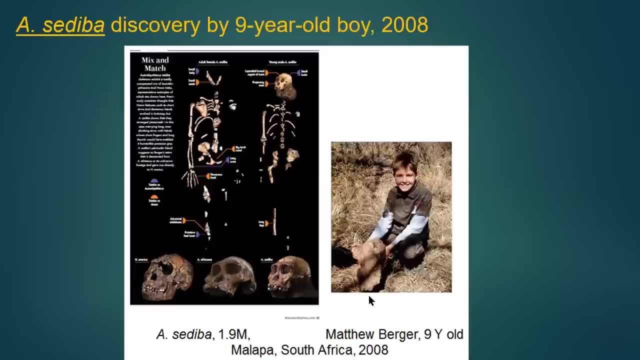 gets lots of funding, et cetera, But he loves doing the press before he writes the articles. His son, Matthew, at the age of nine, stumbled on a stone that had a nice bone sticking out of it, And that's how, at Malacca, South Africa, 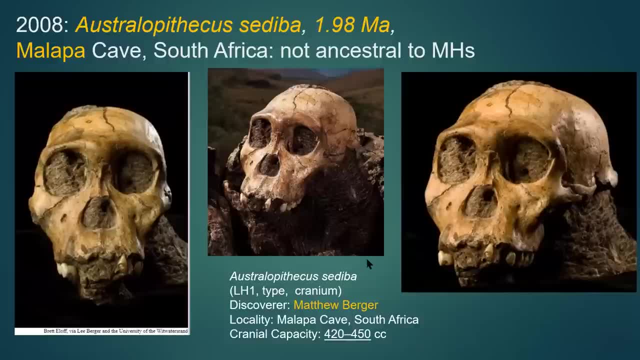 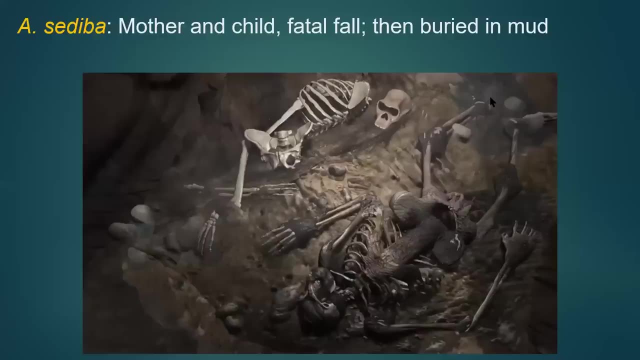 Australopithecus sediba was discovered. We don't. he claimed originally that it was ancestral modern humans, but it ain't. 1.98 million years ago, They think a mother and child had a fatal flaw: fatal fall into this cave. 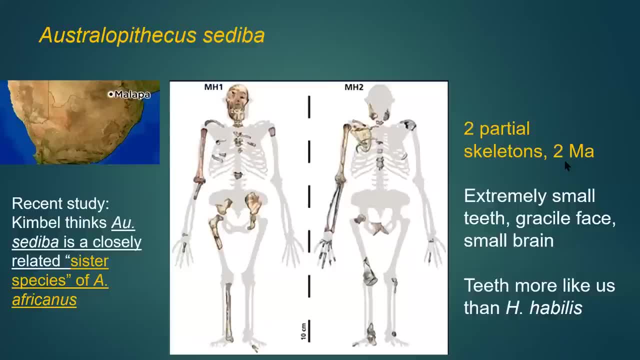 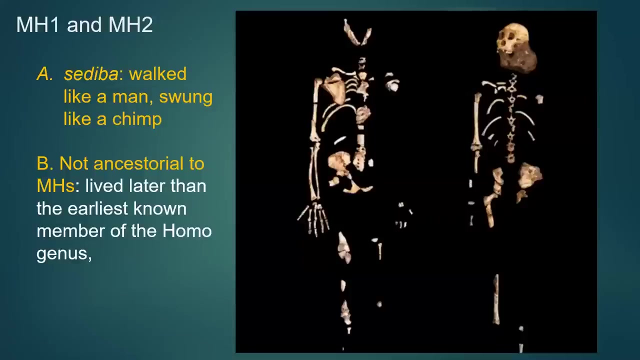 which is where they found them. Two partial skeletons dated to right around two million years ago, And Will Kimball from Arizona thinks that it's a sister species to Africanus. They walked like a man, but swung like a chimp, basically. 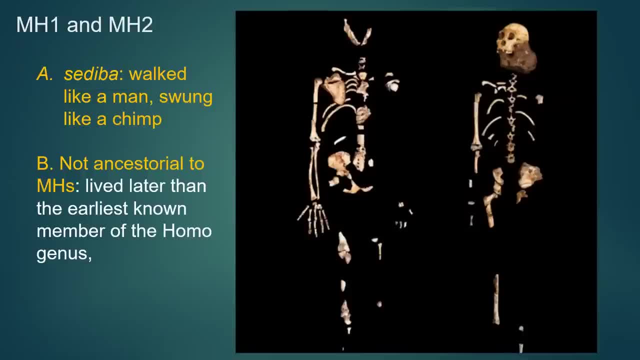 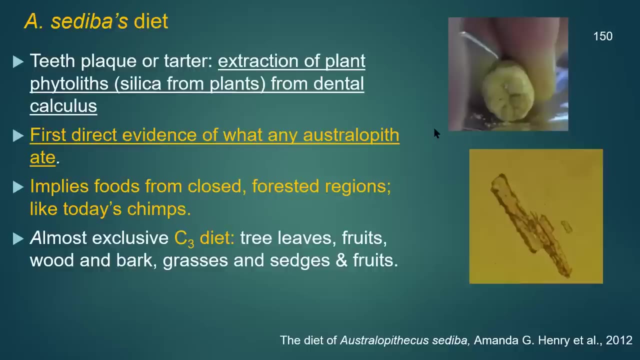 So they were bipedal, but indications that they were quite capable of climbing. They're not ancestral because they've lived lightly than the earliest known member of the Homo genus, So that hypothesis is probably wrong. And then teeth plaque, that was taken, the calculus. 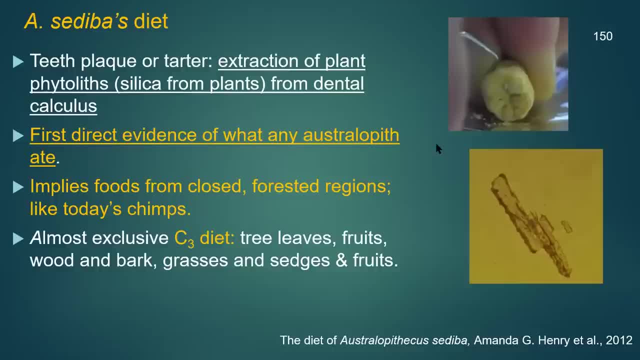 is the first direct evidence what any australopith ate, And they implied that they were almost eating exclusively C3 kinds of food from a closed forested region, like today's chimps. It's tree leaves, fruits, wood bark, grasses, sedges, those kinds of things. 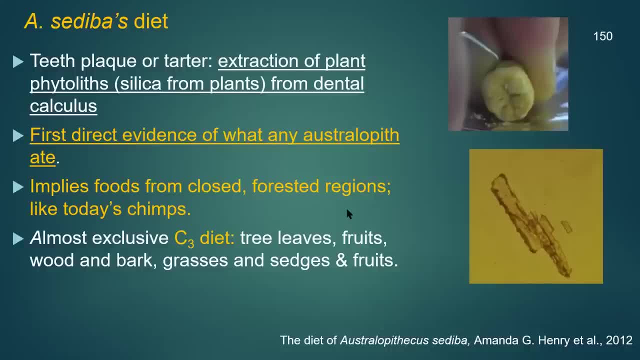 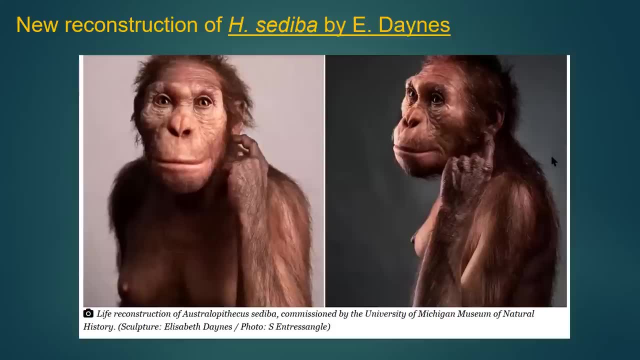 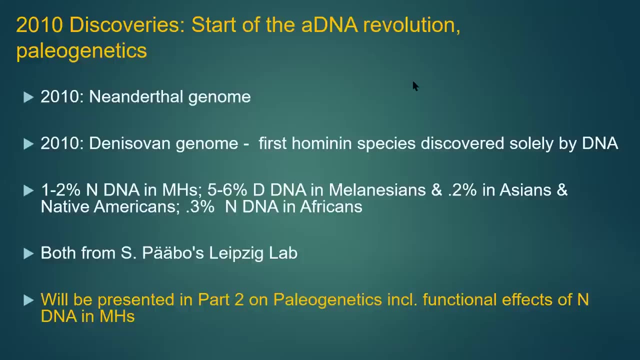 This is the little silica that can be found in plants. I can tell you information about them, And this is the most recent reconstruction of Mama Sediva. And then 2010 comes, the year after I joined the academy, and basically the ancient DNA. 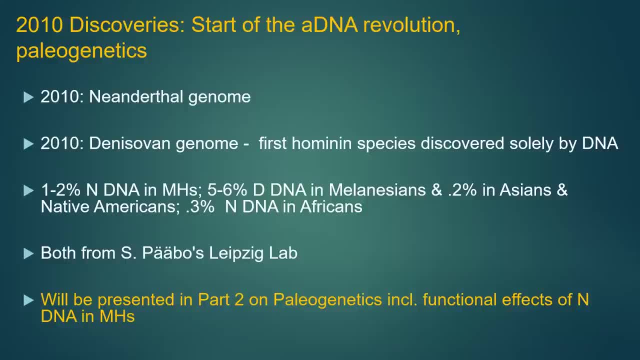 So you can see, this was done in the year after I joined the academy, And then some of the information about other species is also being used in this research, And it's a great way of understanding what the local population is like. And so there are there are a lot of time and space. 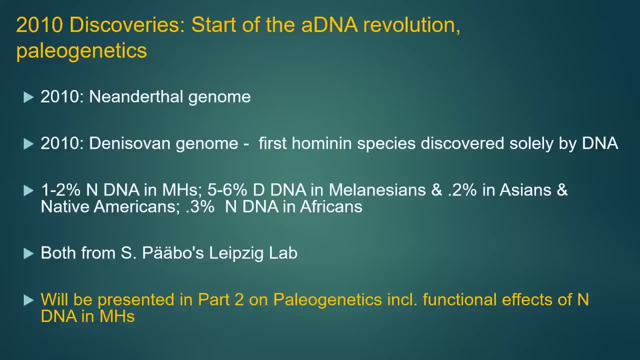 to go back to this theory. I think there is a lot of interest in the history of biology, So I think it's interesting to get started, But I think it's also interesting to deal with the data that we get. Thank you, Thank you. 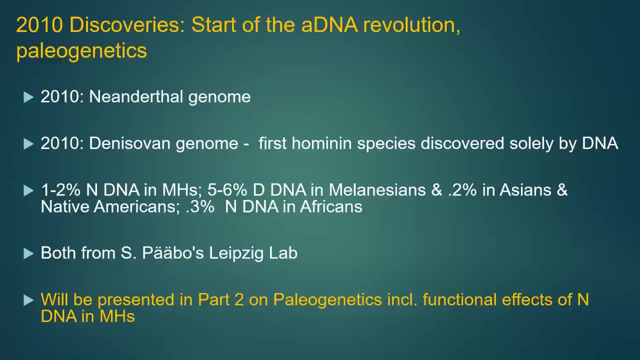 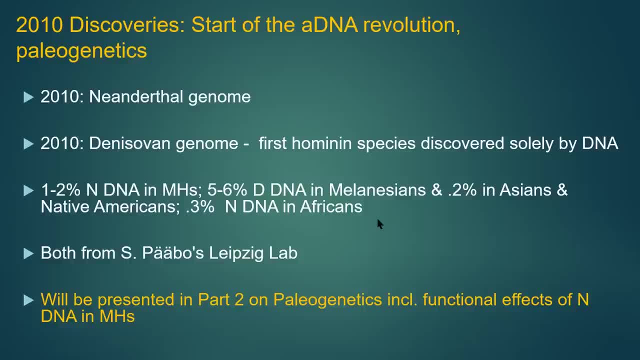 for the Africans getting Neanderthal DNA. is that probably 20 or 30,000 years ago there was a black flow from Asia and Europe back into Africa and more sex and more introgression of DNA between groups. We'll talk all about this in part two. okay, if you're interested. The skin color: 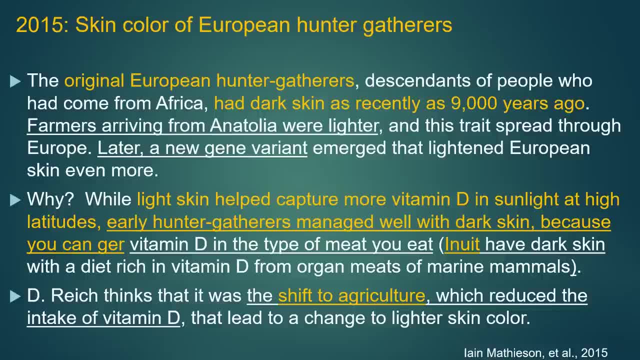 they now think, the original European hunter-gatherers that came out of Africa was basically dark skin. until as recently as about 9,000 years ago, Farmers arriving from Anatolia were lighter and then eventually the Yanmaya from Russia had more light variants. So light skin captures more vitamin D. 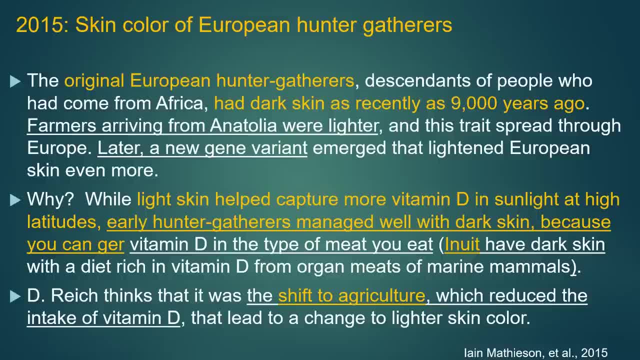 but the early hunter-gatherers managed with their dark skin because probably they were getting their vitamin D, So they were getting more vitamin D from the meat, the venison, they were eating. Today's Inuit have dark skin because they have a rich diet of vitamin D from organ meats of marine mammals. So you can be dark and still get your vitamin D. And then David Reich thinks that the shift to agriculture 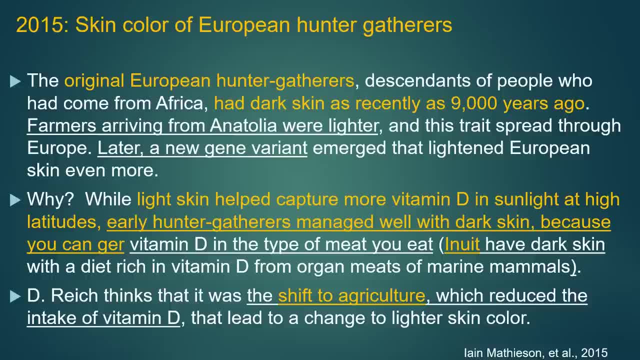 Sorry, hold on. Bill Marks reporting No tracks. Bill Marks reporting No tracks. Bill Marks reporting. Bill Marks reporting Alarm No tracks. Bill Marks reporting Alarm. He thinks the shift to agriculture reduced the intake of vitamin D and led to eventually. 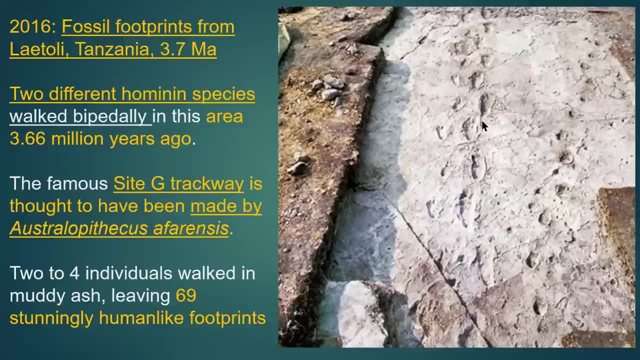 lighter skin as well. This is the famous Laetoli fossil footprint track that was dated to 3.7, and that's some version of Australopithecus afarensis. showed us that they were walking bipedally, just like us. 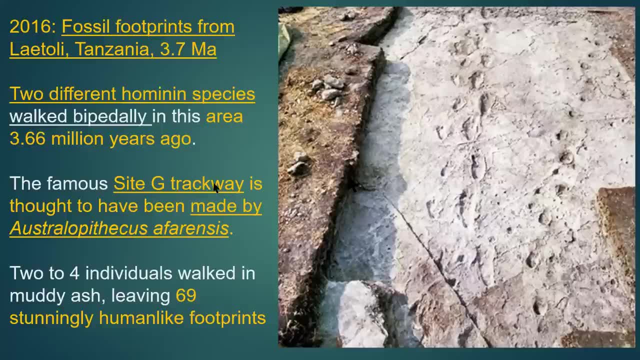 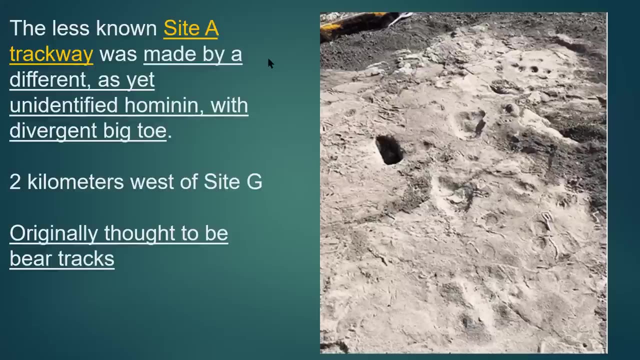 This is the Site G trackway. okay, Offer ends as 69 stunningly human-like footprints, But there is a Site A okay, which is a couple of kilometers away, less known, and originally they were thought to be bear tracks. 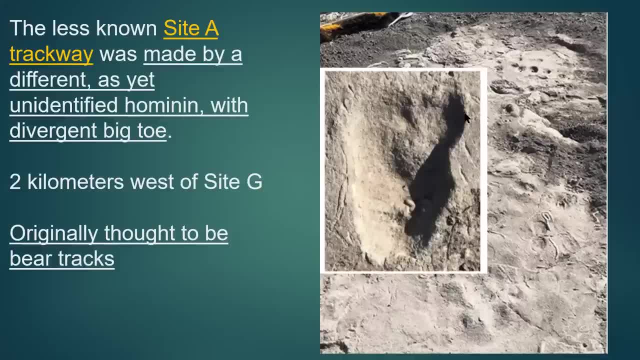 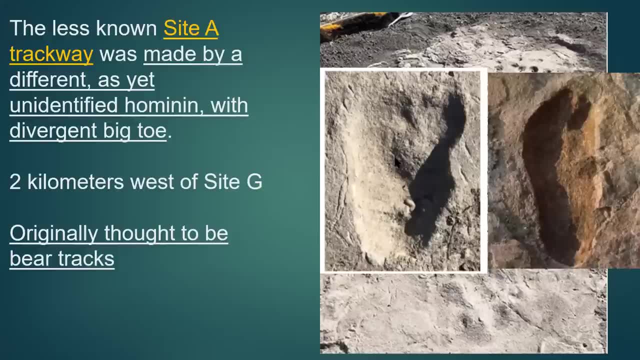 The important is to note the divergent toe. okay, This is Site G. Offer ends as: and this is another hominin that was making its way pretty much at the same time. So again, contemporarity, okay, of species. 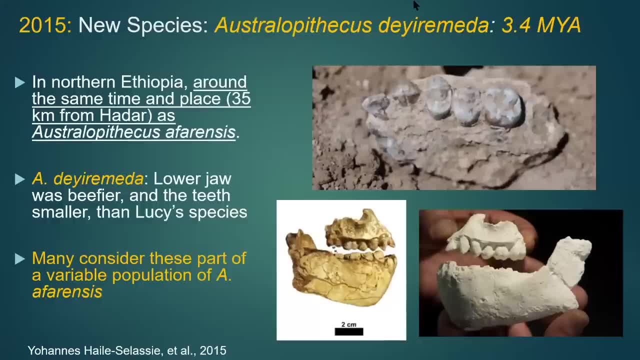 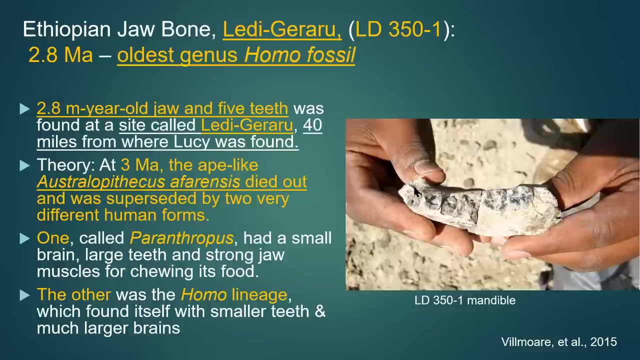 Then they discover Dairamida in Ethiopia. Probably many contemporaries People considered this a variant population of Offer ends as basically okay, not many people talk about it. But then, much more importantly, at Ledi-Jiraru they discovered this jaw and it's dated to 2.8 million years and is now considered the oldest Homo fossil that we have. okay. 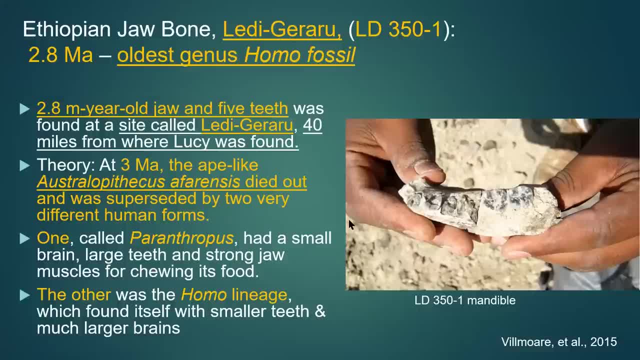 So the thinking is that around 3 million years ago, the ape-like Australopithecus Offer ends as die out and then are superseded by one Paranthropus with its big teeth and strong jaw muscles. 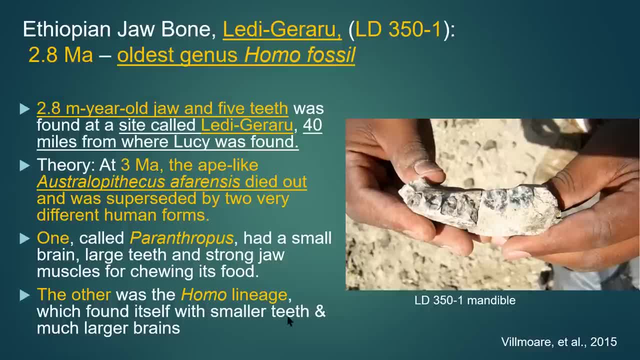 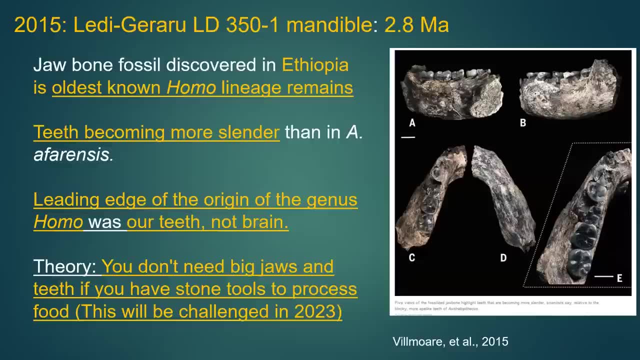 and the Homo lineage, which is smaller teeth and much larger brains. okay, These are the fossils. It's the oldest known Homo lineage. The teeth become more slender. Some people think that the leading edge of the origin of the genus Homo is our teeth. 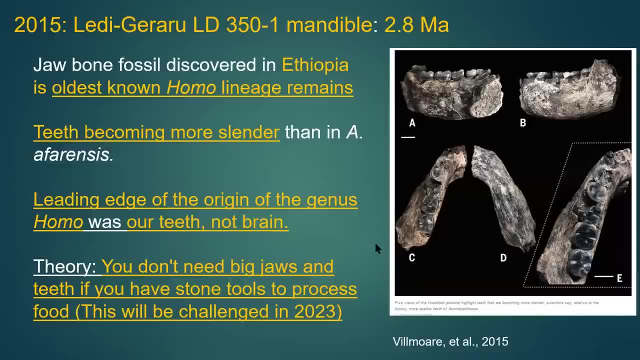 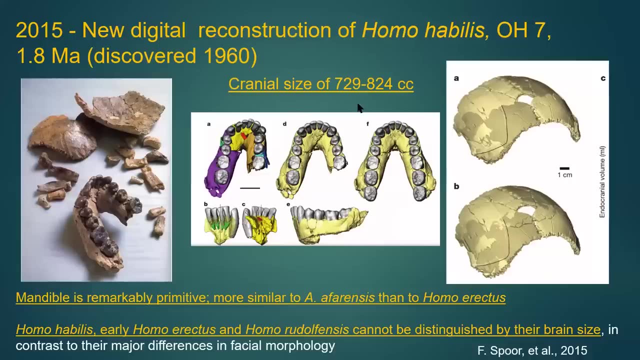 not our brain, and that you don't need big jaws and teeth if you have stone tools to process food. But this will be challenged this year, as we'll see. They then do a digital reconstruction of one of the original Homo Habilis. 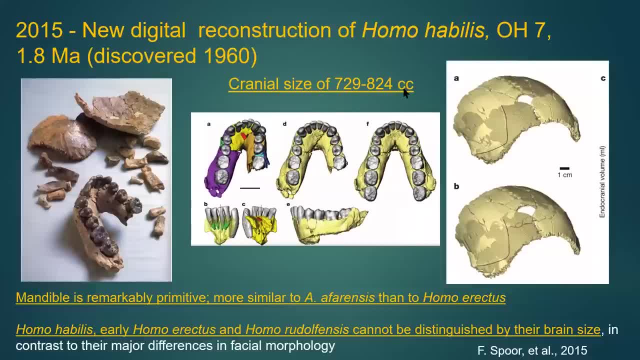 and their cranial size is much bigger than the old 600 mark. They think it's somewhere in the 700 to 800 cc range. The mandible is remarkably primitive and more similar to Alpharensis than to Erectus. 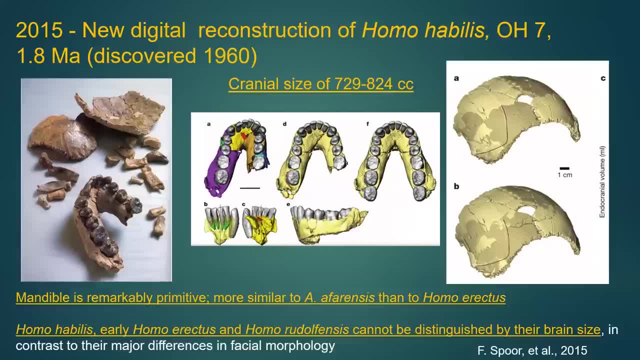 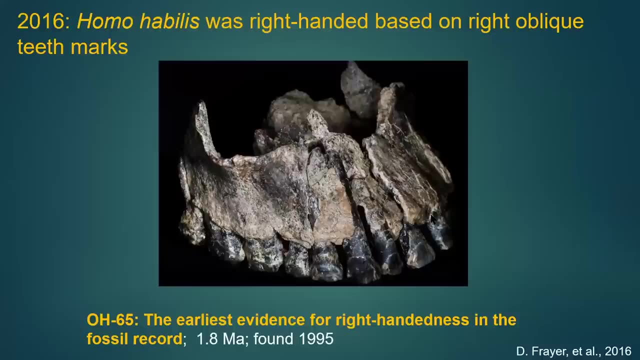 And so Homo Habilis, early Homo Erectus, Homo Rudolfensis, a larger version of Habilis can't be distinguished by their brain size. Okay, so there's lots of mixing going on, And this is on these teeth. 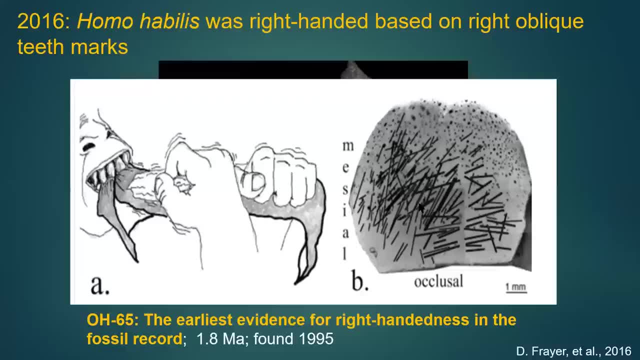 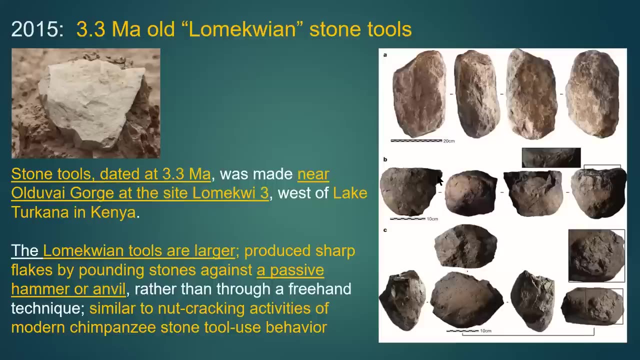 they found the earliest evidence for right-handedness in Homo Habilis. because of the way he missed the meat he was cutting and cut his teeth, going in an oblique angle, that indicates he was right-handed. Okay, And then, most importantly, 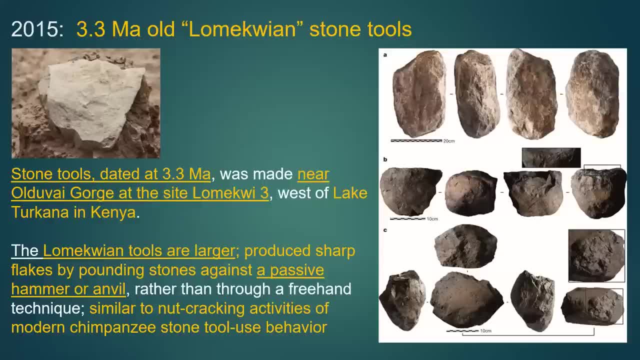 hugely important. at Loma Kui, near Turkana, Kenya, they discover stone tools that are dated to 3.3 million years ago, literally predating any known Homo fossil, And they think these are larger and slightly less sophisticated than the old one. 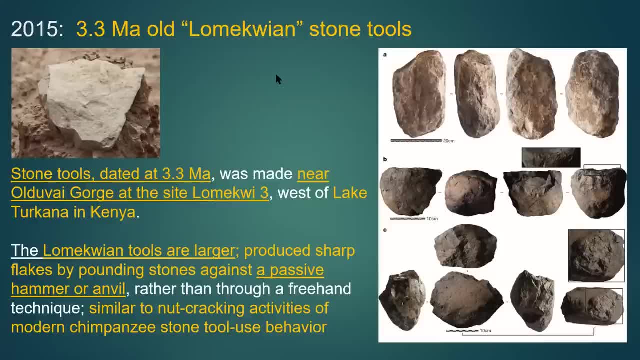 And, unlike old one being hit from one hand to the other hand, they think they were used using stones to hit an anvil stone to break them up, And this methodology is almost identical to what modern-day chimpanzees use to break up nuts. 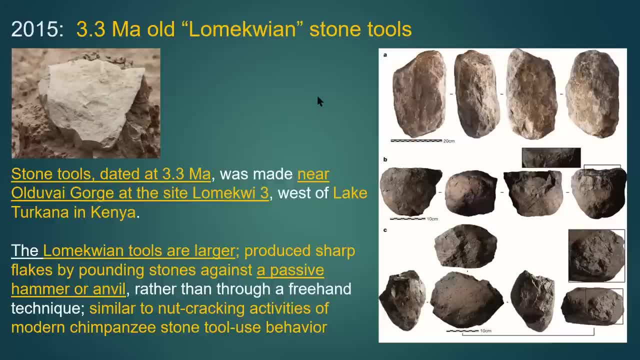 as an example. So here the best current evidence for Australopithecus scenes using tools. before we did Okay, And some people now think that stone tool using may not be a marker of Homo sapiens, but in fact, 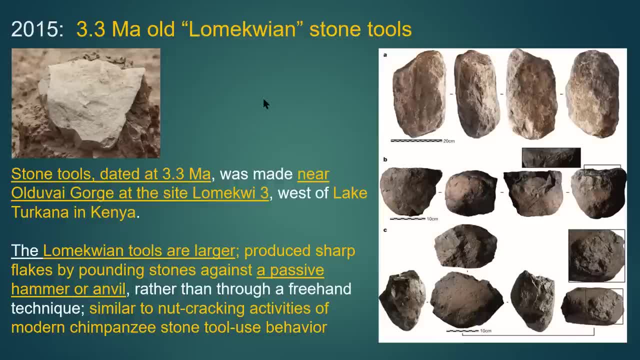 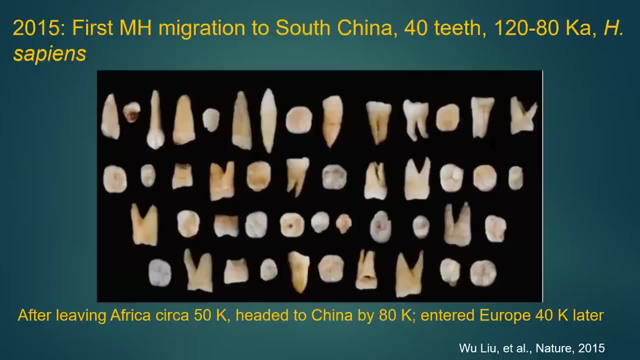 of the last common ancestor. So we will see The okay. And then 2015,. they discover these modern human teeth in South China, dated to 120 K, So 60 years before the Great Migration. they discovered that Homo sapiens were moving out of Africa. 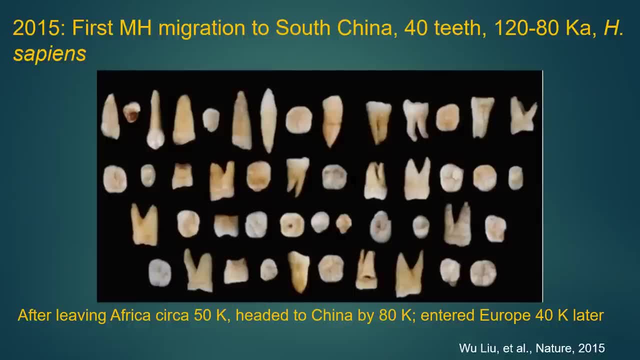 Another indication that we were actually Africans of a human type, were moving out of Africa multiple times before 60 K Okay, And this is one of the first to indicate that It's likely that we actually left Africa headed to Asia first. 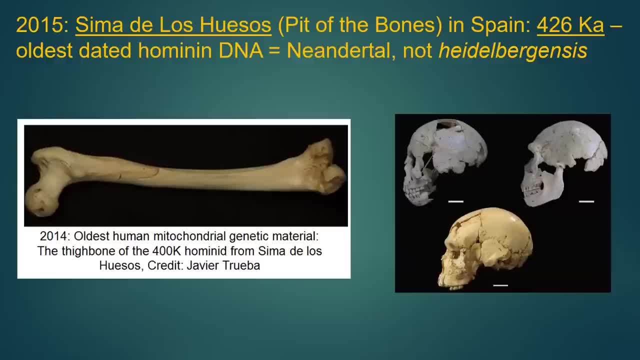 and then around 40 K or so, And then an amazing group of fossils at the Cima de los Huesos pit of bones in Portuguesa, Spain It is. it was originally considered Heidelbergensis, but the oldest. 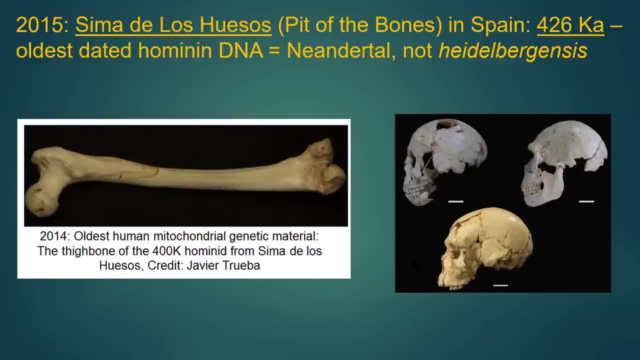 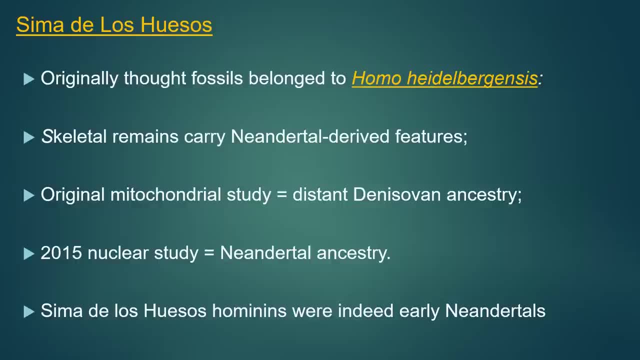 the current DNA data indicates otherwise. Okay, So they clearly have Neanderthal features. The original mitochondrial study said it's a distant Denisovan ancestry And then, in 2015,, the nuclear DNA said: nope, these are Neanderthals. 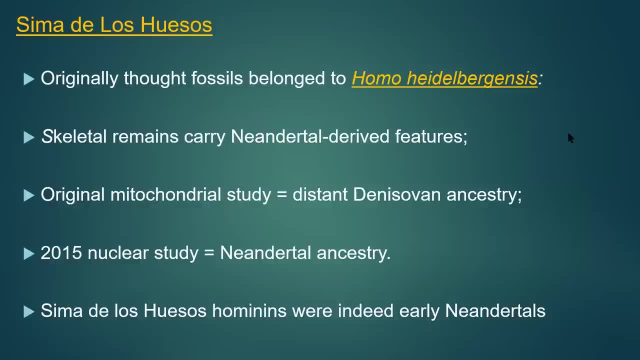 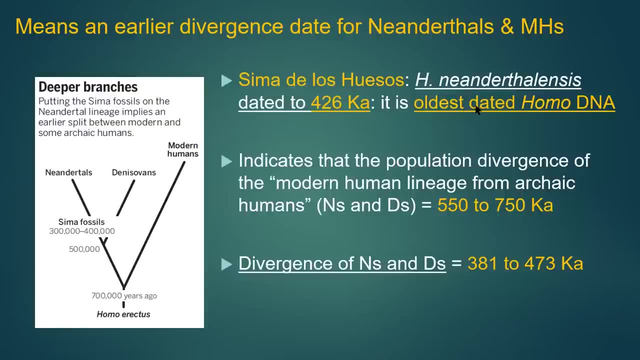 So these are the earliest Neanderthals that we have, dated to 426 K, which is the oldest dated Homo DNA, And the skull five that we have in the collection, the one with sort of the broken teeth and the hole in his left side of the skull. 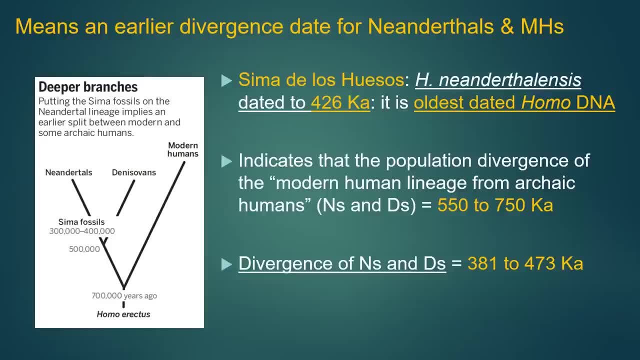 is the actual skull that they got the this DNA from his bone in his ear region. This immediately said that the divergence between modern humans and Neanderthals had to be earlier than they used to think, And now it's dated to 550 to 750 K. 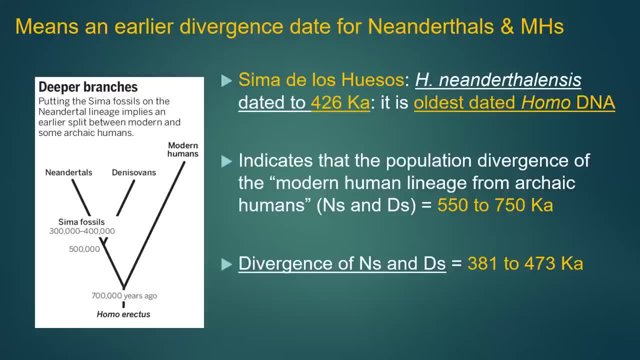 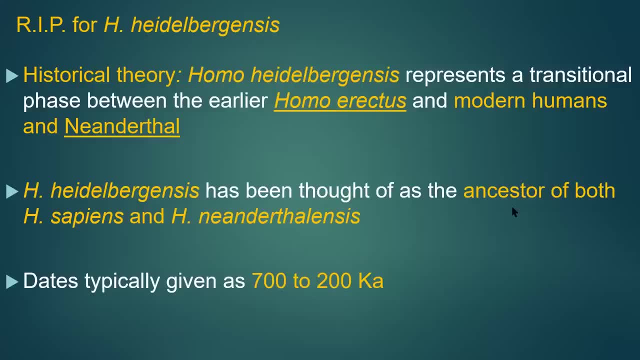 And that the divergence between Neanderthals and Denisovans came later, at around 400, 450 or so, And then increasingly we're seeing sort of a RIP for Heidelbergensis. The historical theory is because of the. 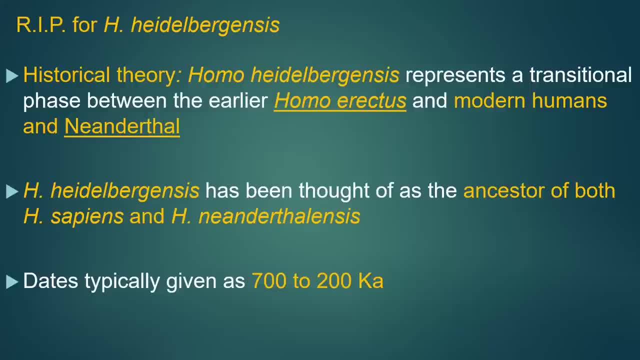 the kinds of skulls that they found in Europe, the Maurer jaw, that Heidelbergensis represented a transition between Homo erectus and modern humans and Neanderthal, And that Heidelbergensis was, in effect, the ancestor of both Sapiens in Africa and Neanderthal in Europe. 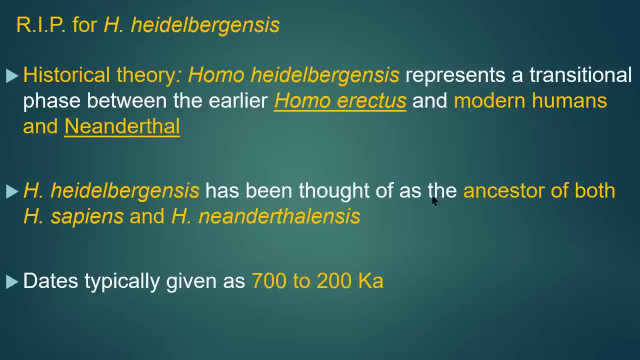 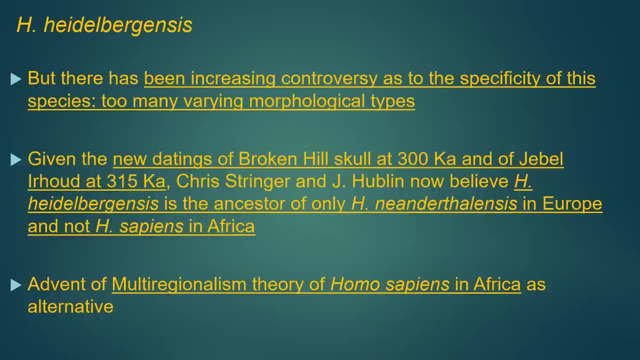 The classic dates are 700 to 200 K or so, But there's increasing controversy as to the specificity of this species because too many burying kinds of skulls have been put into this group. And then, with the recent new datings of the Broken Hill Skull in Africa to 300 K, 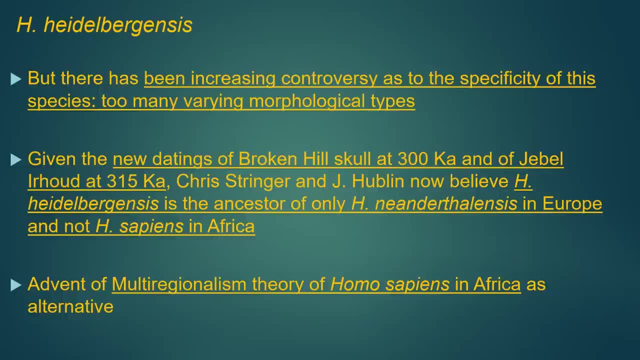 and the Jebel Irhoud modern human skull at 315 K. both Chris Stringer and Hubland in France now believe that Heidelbergensis is only the ancestor of Neanderthal in Europe, but not of us in Africa, And this comes on the heel of this new theory called multi-regionalism in Africa. 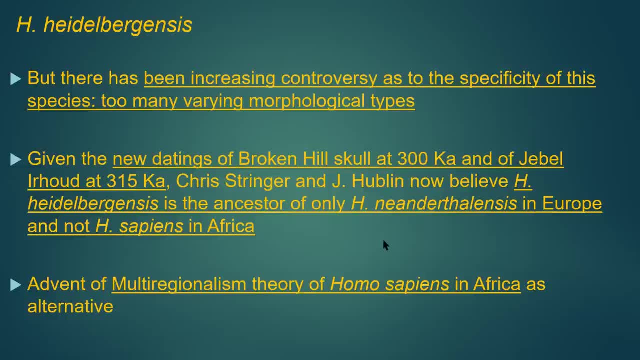 which we don't have time today. But basically the idea is that there's no single homeland on anatomically modern humans In Africa, that East Africa is not the Eden of us all, but that modern Homo sapiens is a blend of a whole bunch of interconnections all over Africa. 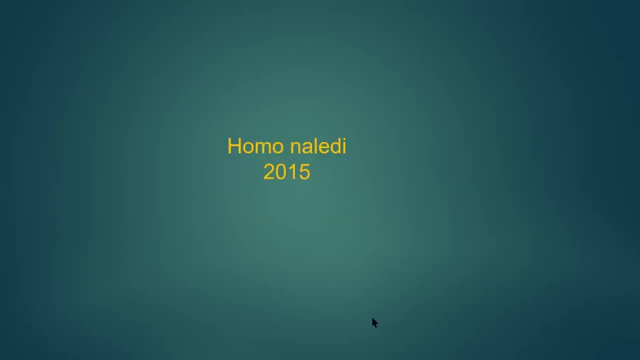 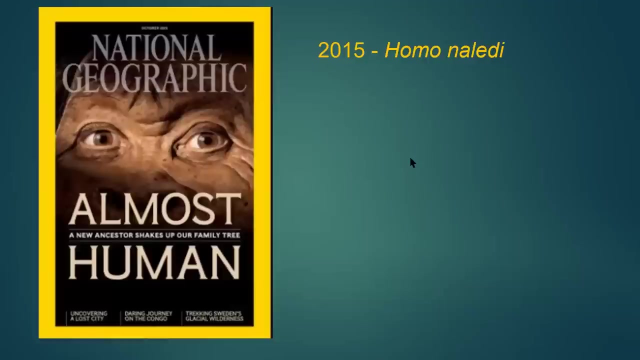 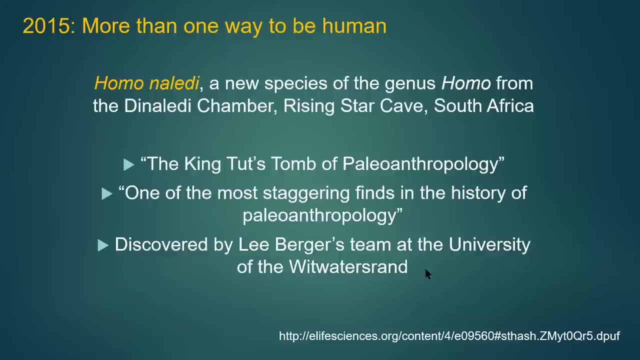 That's the gist of the multi-regional theory. Then comes the major discovery in 2015, Homo Nelidi and Berger kissing the skull. Okay, This is an amazing discovery. There's no question about that. It's been called the King Tut's tomb of paleoanthropology. 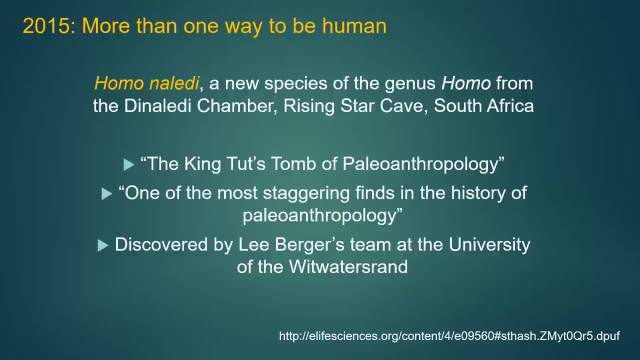 one of the most staggering findings in the history of paleoanthropology discovered by Lee Berger's team. It's a great story. If you haven't read it, you should read it. I'll just give you a couple of highlights. 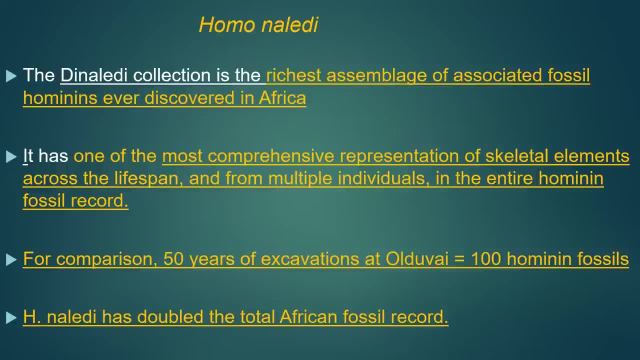 but it's the richest assembly of fossil hominins ever discovered. It actually doubled the number of fossils that have been discovered in Africa In 50 years of excavating. at Olduvai, they only found a hundred hominins. They have found more than 2,000 in the new collection. 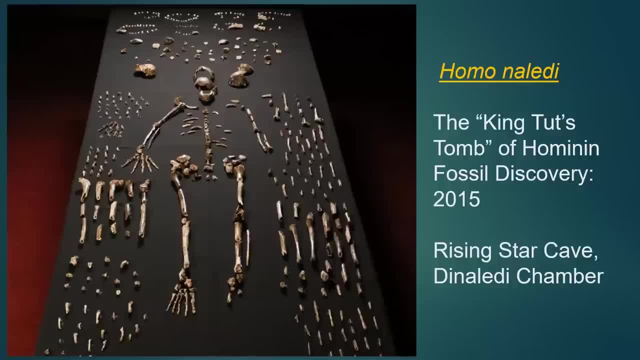 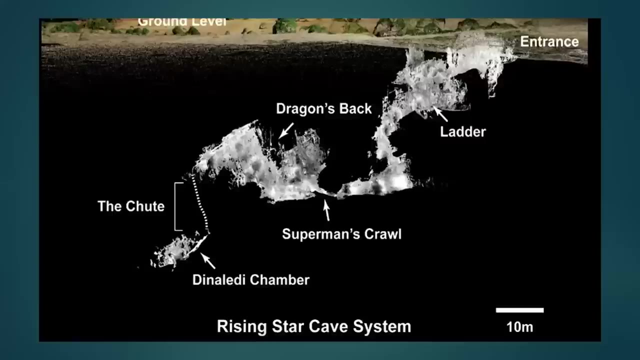 So they have every single bone element of the skeleton in multiple versions, multiple ages, et cetera. The Rising Star Cave, the Nelidi Chamber, where much of this discovery happened. The entrance is up here. You have to go down in pitch blackness. 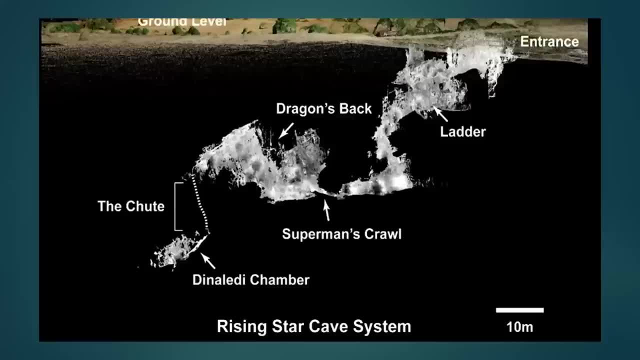 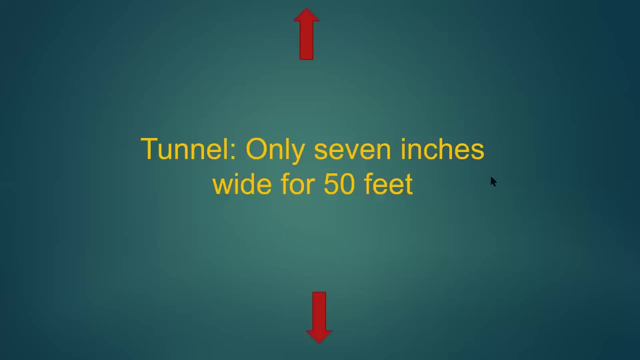 Originally there's the Superman Crawl area You have to then climb, And before you get to the chute that leads down to the Nelidi Chamber, you have to go through a 50-foot length tube that's only seven inches this wide. 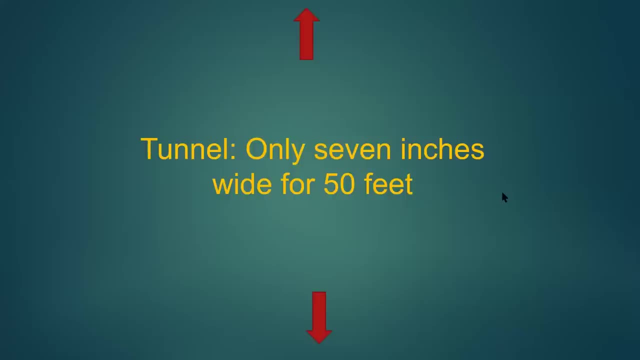 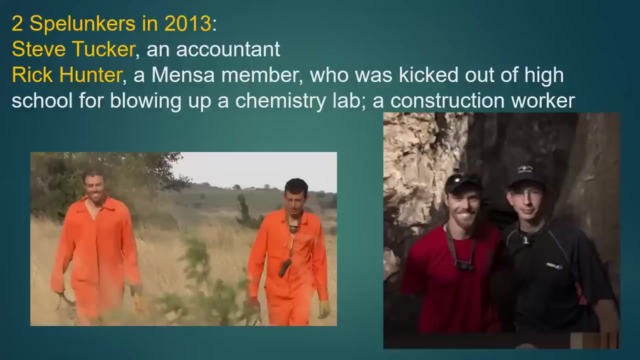 Okay, Imagine doing this. Okay, It all starts with two spelunkers in 2013,. Steve Tucker, an accountant, and Rick Hunter, a Mensa member who was kicked out of high school for blowing up The chemistry lab, is a construction worker. 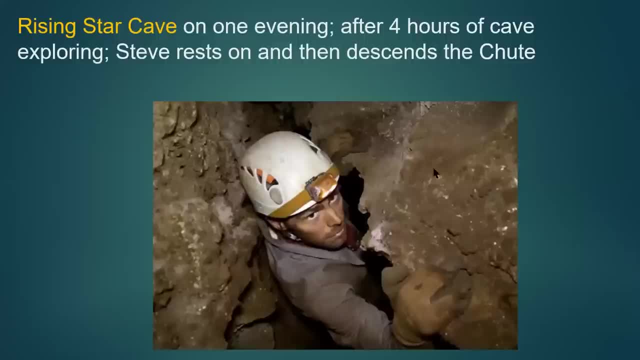 They love to do caves, All right. And one night, after four hours of exploring, he leans up against something and realizes there's a shaft. He doesn't know how far the shaft is or that it doesn't open onto a thousand foot empty hole. 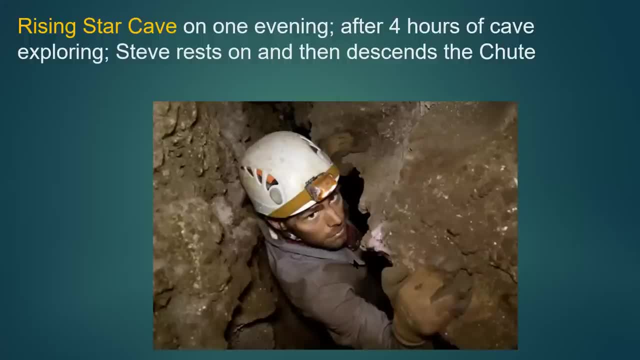 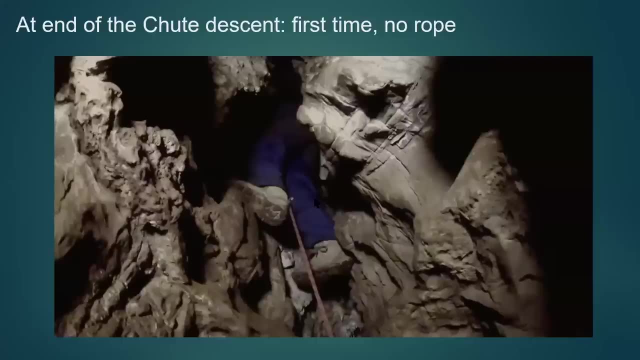 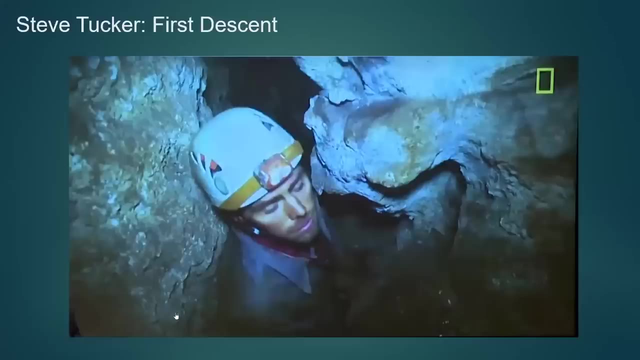 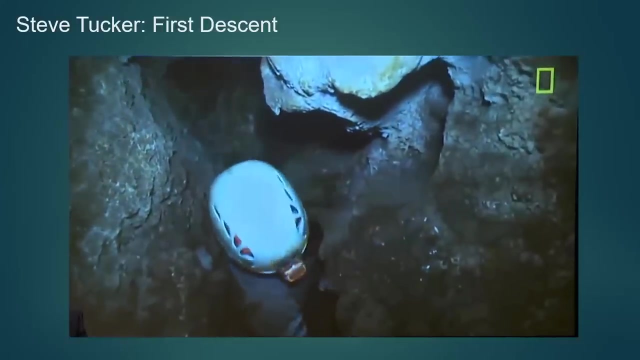 Okay, These guys are stunningly either stupid or adventurous, And at the end of the chute this is where you end up, before you eventually hit the floor. They didn't have a rope in the first climb And this was the first climb into the shaft that leads. 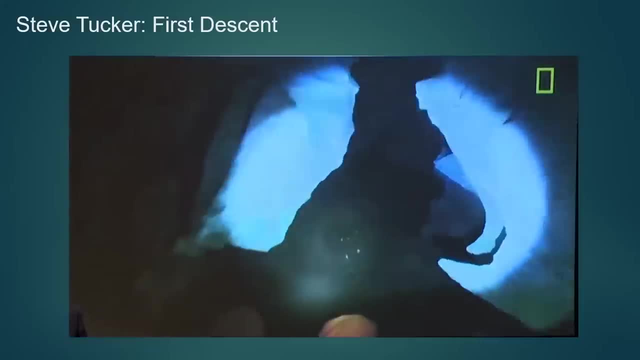 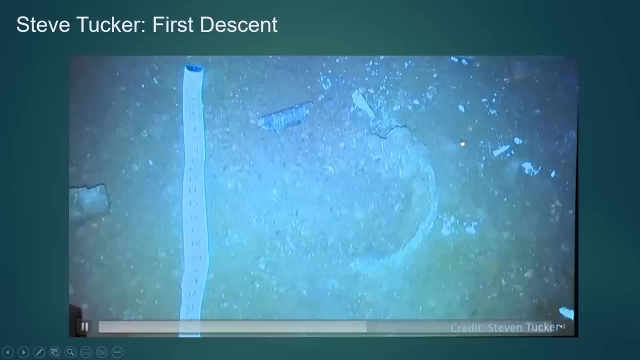 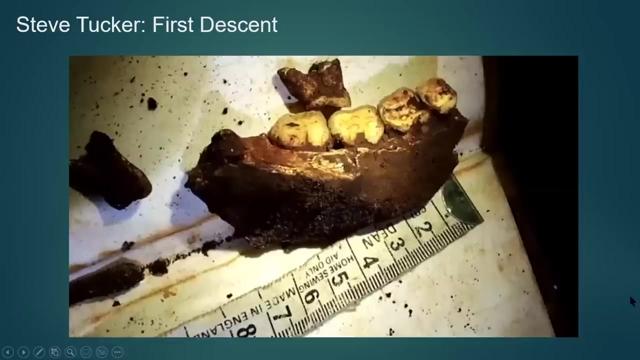 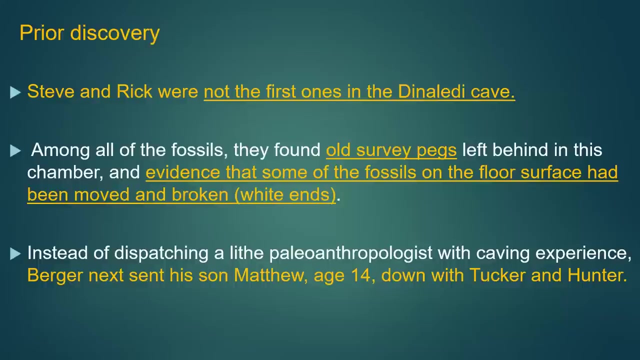 the cavern Incredibly tight spaces. And then they come down and there are 400 bones just sitting on the surface. Hugely important one. But it turns out they're not the first ones in the cave. Okay, there are old survey pegs, evidence that some of the fossils on the floor had been moved and broken because there are white ends on some of the bones. 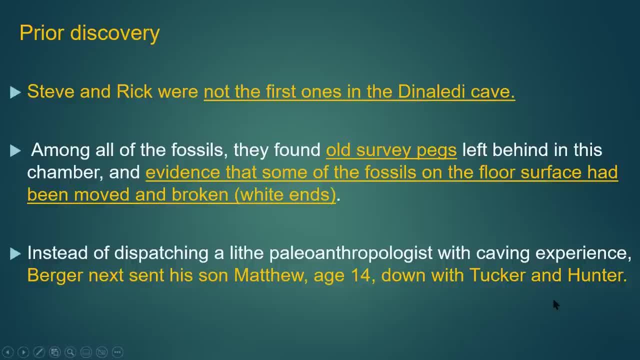 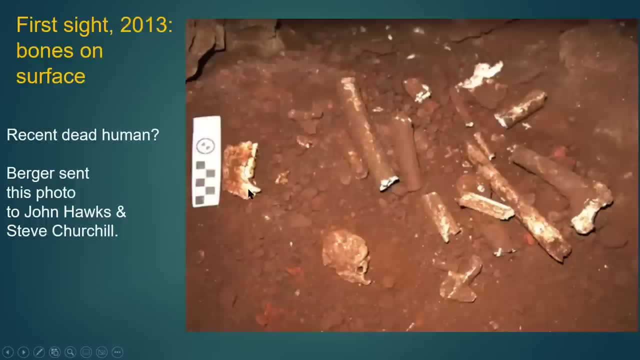 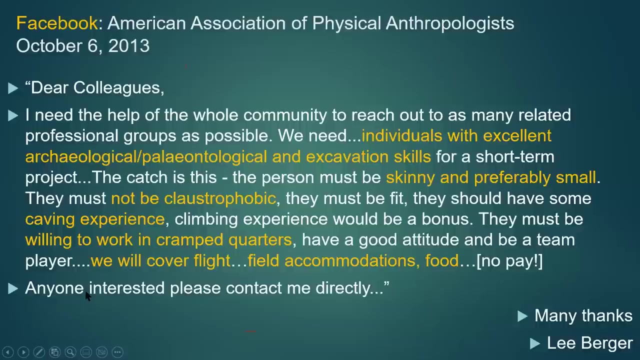 Berger next sends his 14 year old son down with Tucker and Hunter. And the first- this is one of the first sites, and this is, uh, the jawbone. Berger sends these photos to John Hawks in Wisconsin and Steve Churchill, who famous Neanderthals specialist. 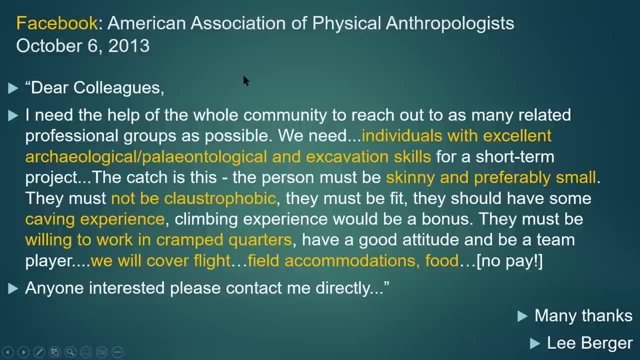 And in Facebook on October 6, 2013,, they put out the following ad: I need the help of the whole community to reach out to as many related professional groups as possible. We need individuals with Excellent archeological and excavation skills for a short project. 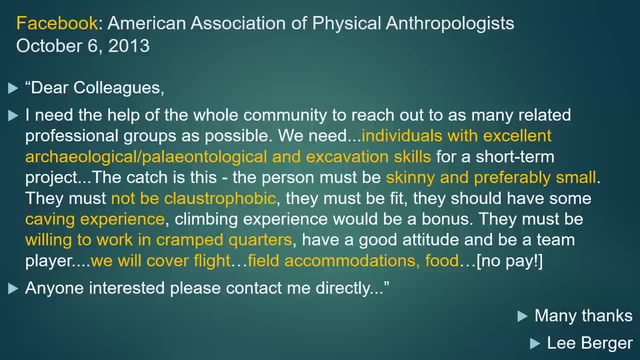 The catch is the person must be skinny and preferably small. They can't be claustrophobic. They need caving experience and willing to work in very cramped quarters. We will cover the flight, the field, accommodations and the food, but no pay. 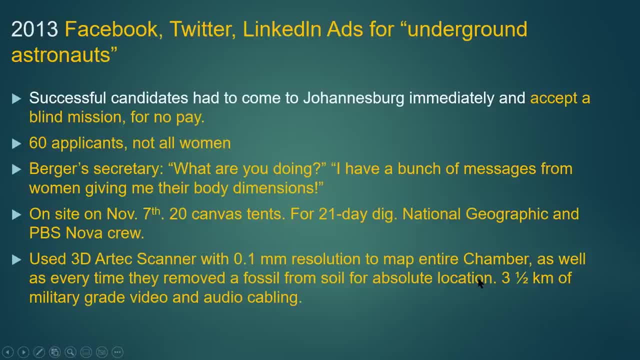 Okay, 170 people, or actually this is wrong. About 170 people. originally applied with only a couple of men. Berger secretary asked him: What are you doing? I have a bunch of messages from women giving me their body dimensions. Okay, so they set up a 21-day dig. National Geographic and PBS Nova crew. 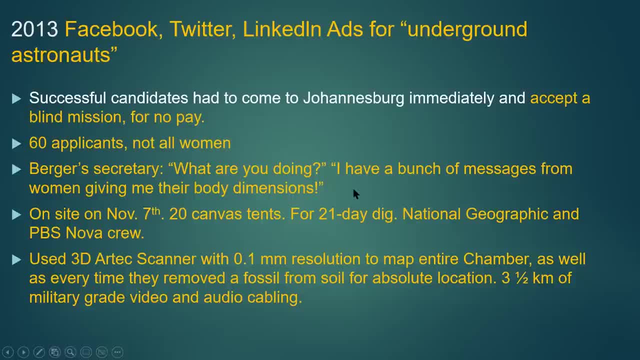 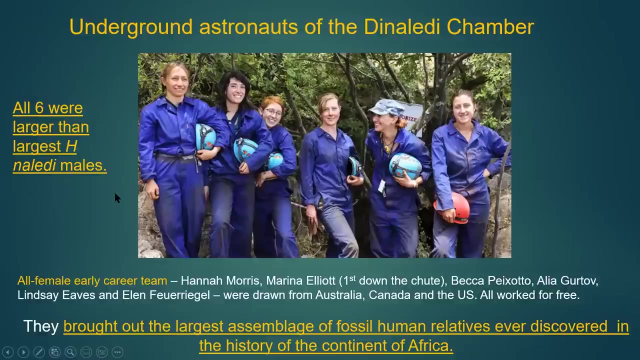 They photograph everything and they put it on the internet. This is- he gets credit for that in terms Of sort of universalizing- a new finding, basically- and they do massive amounts of photography, videotaping, They put in cabling all over, and these six women are the ones that went down first. 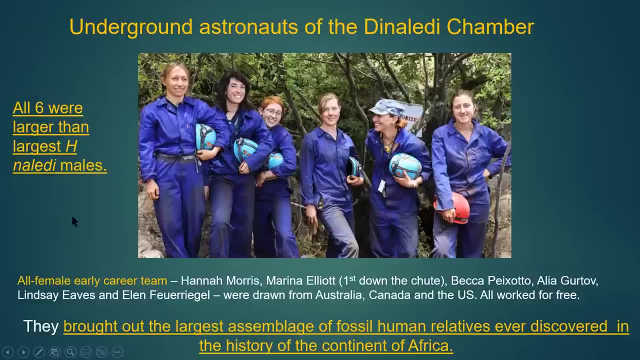 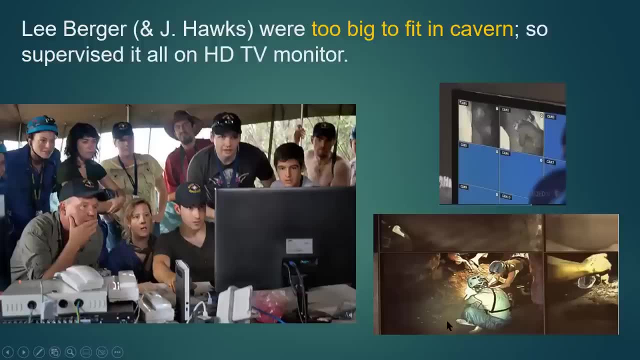 And they're all larger than the largest homo naledi male, but they brought out the largest assembly of fossil humans ever discovered in Africa. Berger and Hawks had to look at it all on TV monitors above ground and sort of tell them what to do, what to look for. 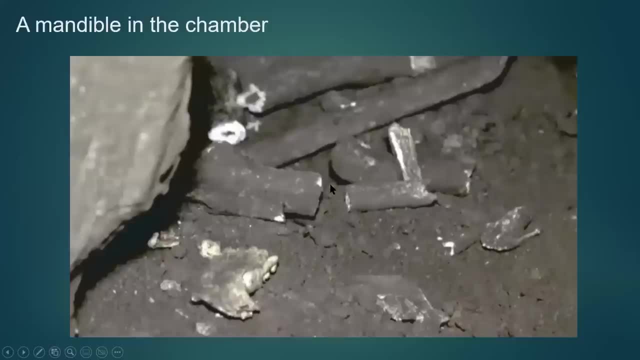 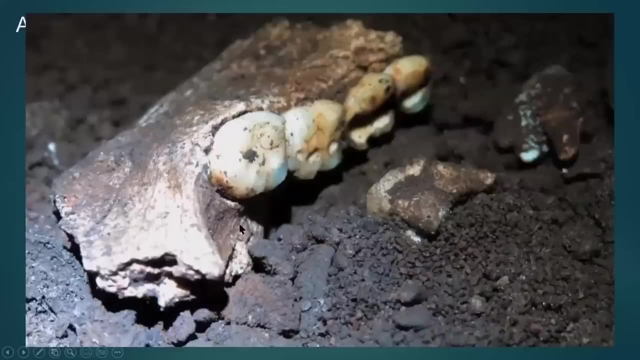 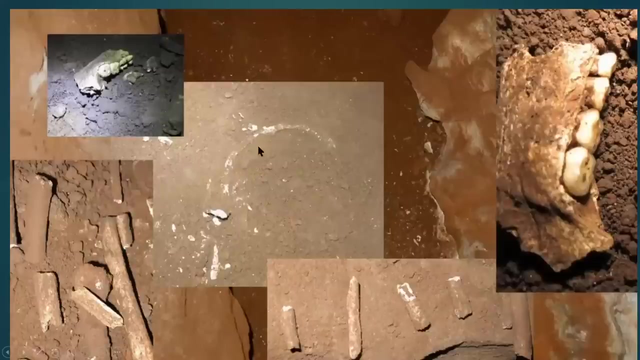 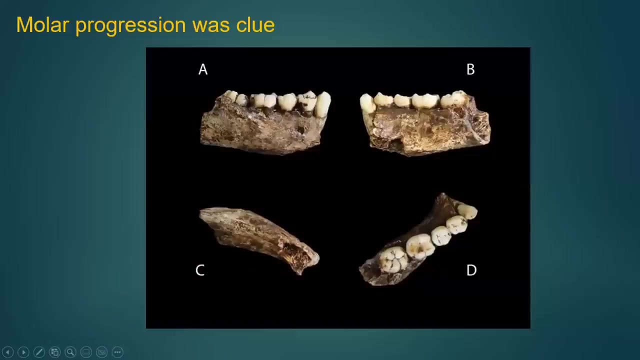 But a whole bunch of them look like they had in fact been recently broken, And this is the jaw bone that led to lots of excitement- Basically, clearly, a skull, So molar progression in hominins is really important to tell you how old they are. 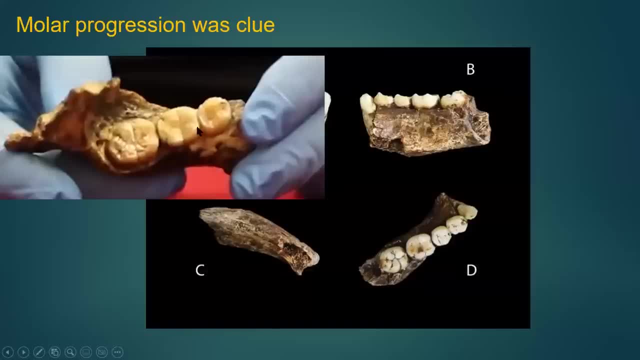 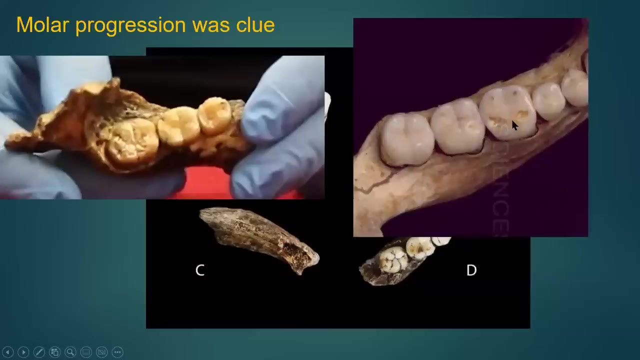 Note: First, second, third, molar, smallest is the smallest. last is the largest in modern humans. It's the reverse direction. What That's a lot. We've gone from about 3 million years to nearly more than 20 billion years later. 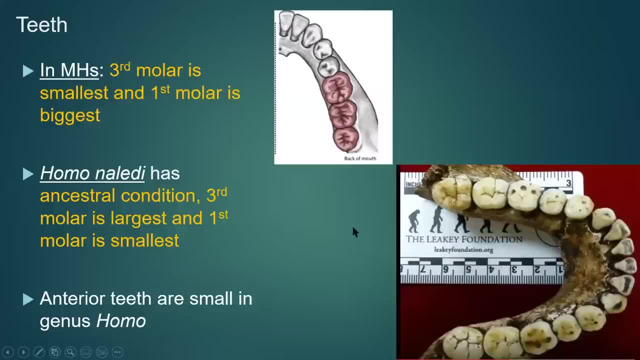 Somebody is talking Sorry, Okay, so that's how you tell, basically, whether it's a modern motor setup or a more ancient ones. and homo naledi have the ancestral conditions, third molar being the largest, um, and they've got lots and lots and lots of teeth, basically, 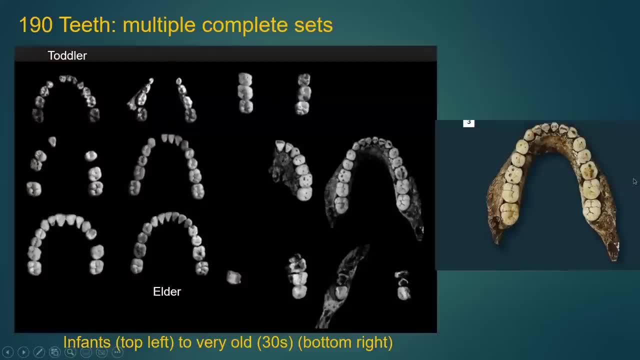 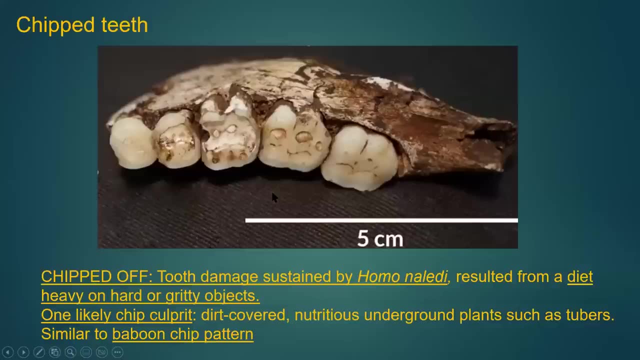 lots of ages, going from toddler to elder. um, but, interestingly, the chipping pattern. this group is heavily chipped, indicating that their diet was heavy on hard and gritty objects. so these guys should be called the nutcracker people, not uh, paranthropus and um baboon chip. 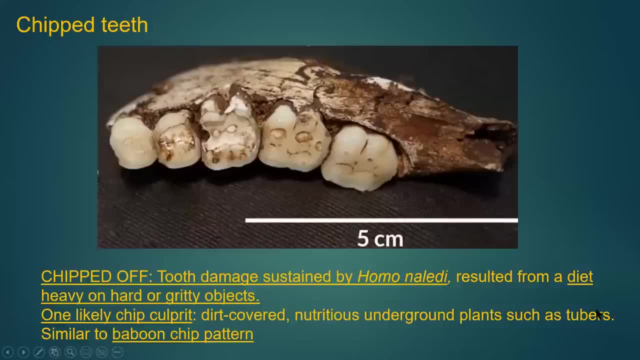 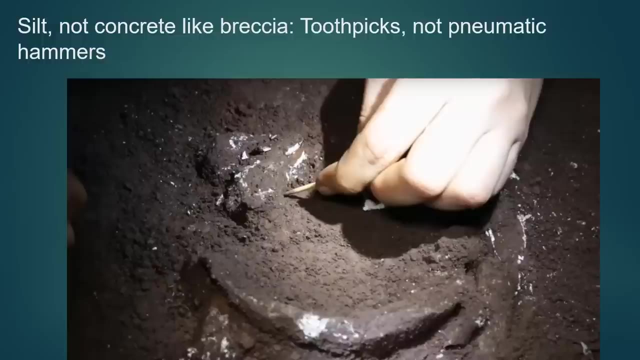 pattern, basically, who also tend to eat a lot of tubers, uh, dirt covered kinds of uh stuff. so a comment about potentially what diet they were doing: and this was silt, not breccia concrete, like in the south african caves. they needed toothpicks, not hammers, basically to 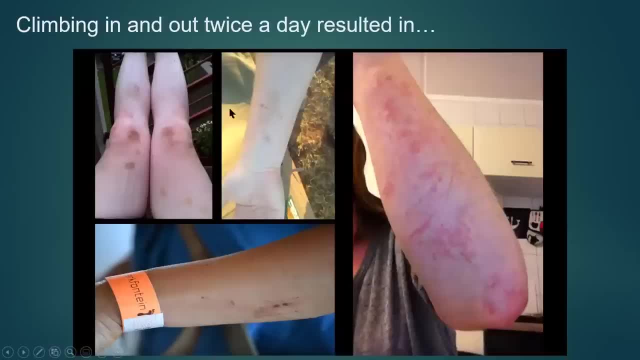 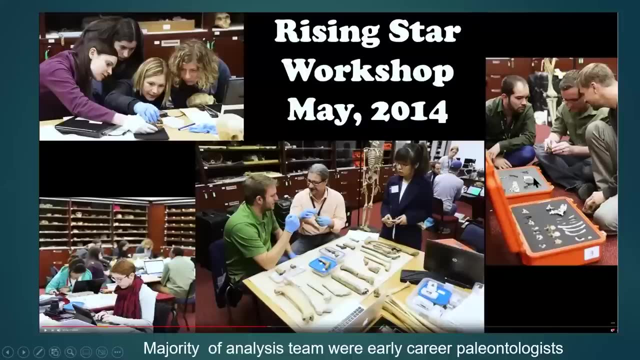 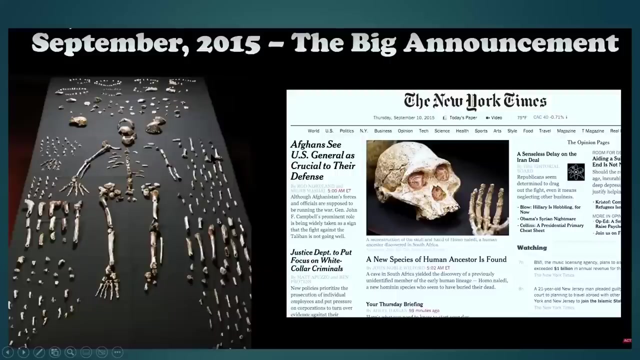 get these fossils out, and climbing in and out- okay- resulted in lots of abrasions- okay. they then do a workshop. they bring in lots of early career paleontologists, which was a good mark, but it also didn't necessarily bring in expertise. in september 2015, they announced it to the world- new york times. 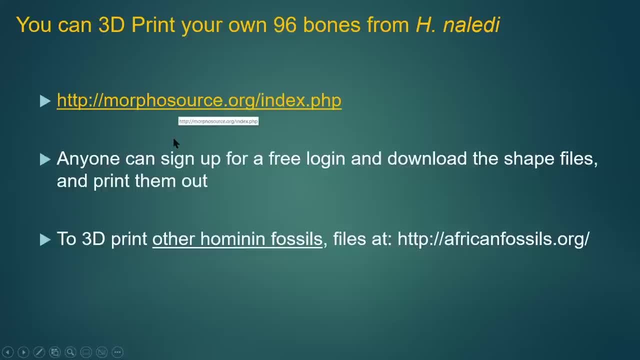 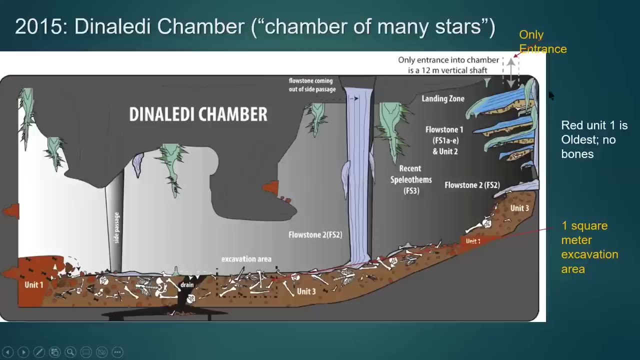 they also put up uh 3d printing of a whole bunch of the bones from the cave, including the skull. if you can afford doing a download and then doing the 3d printing of it, okay. this is what they found. they found 400 bones simply lying on the chamber floor. 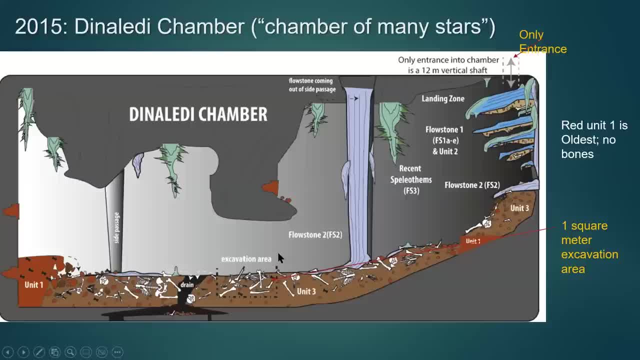 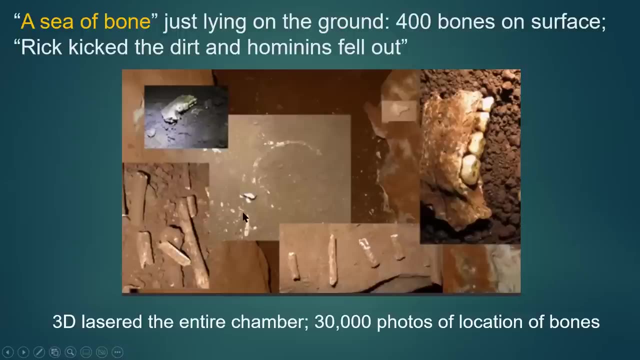 and this is a one meter by one meter deep excavation site, which was what they originally did and what the publication papers are, uh, all about. okay. um, it was basically a sea of bones. rick kicked the dirt and hominins fell out. basically, they've taken 30 000 photos of the entire chamber. uh, there are originally 15 individuals. 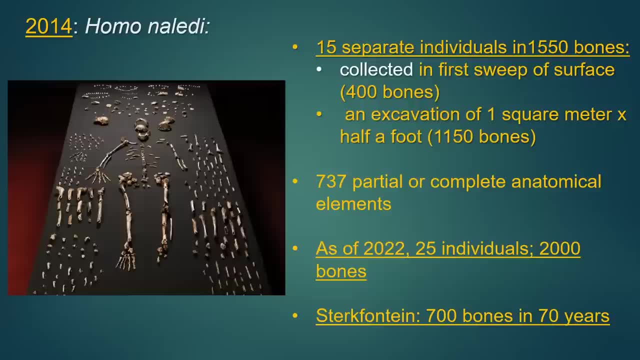 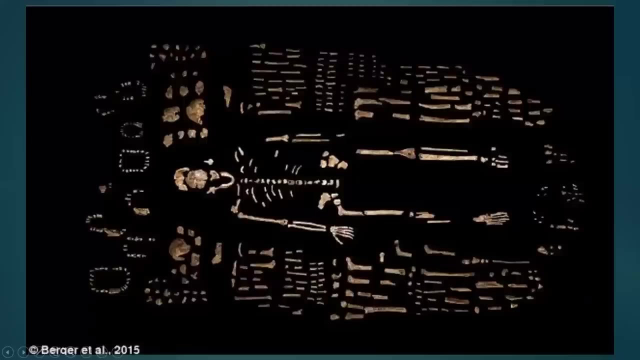 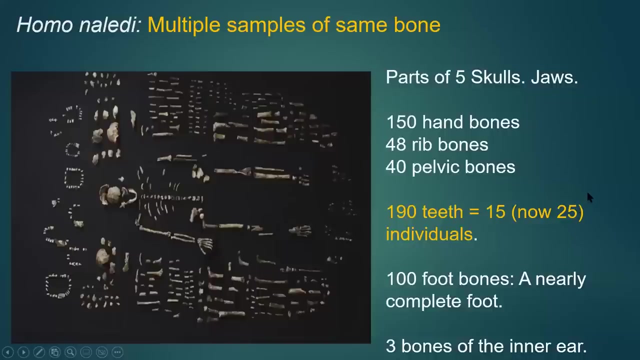 with 1500 bones. uh, and by 2022. there are 25 individuals who have been killed by the НАЯ from похun ran a story about 1400 individuals who were killed and half of those are still alive, but in the end, not much of the lives of those people are sold. they're gone. 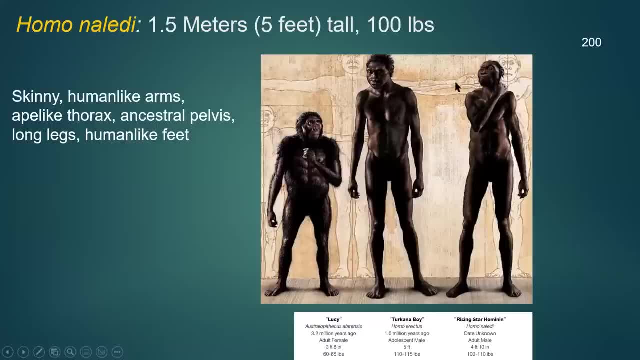 this is a beautiful picture of this group of individuals with 2000 bones compared to foundation in south africa, which had 700 bones in 70 years. so this was a massive collection. basically, just a beautifully, profoundly important discovery: lots of hand bones, rib bones, pelvic bones, 190 teeth, beautiful feet, okay, and so you can think of naleenah. 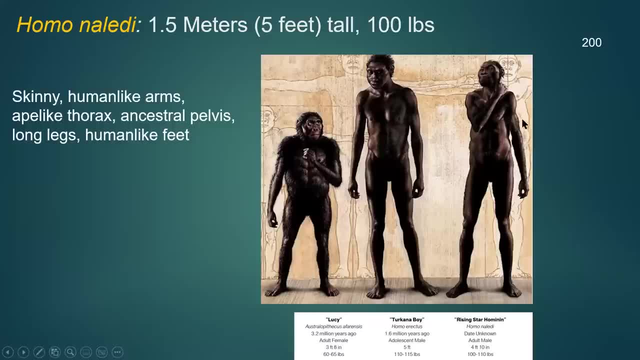 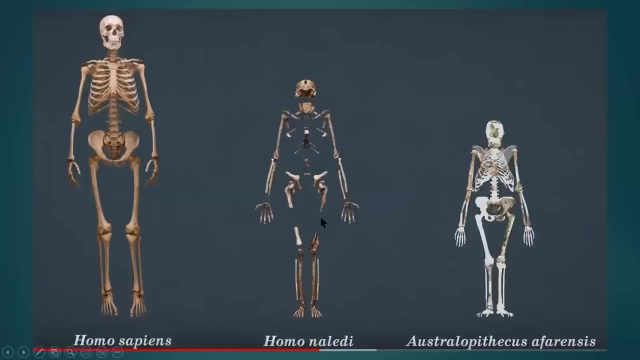 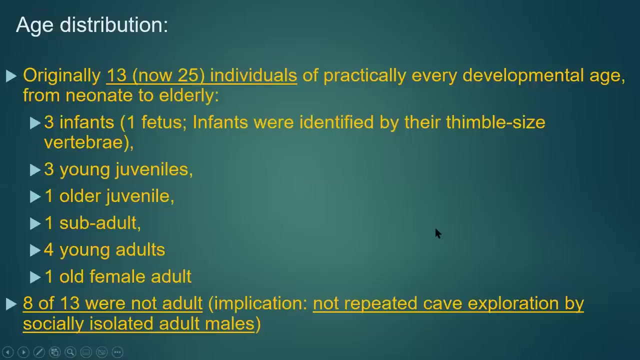 liddy as a one uh five foot skinny version of homo erectus, and that's one of the contentions is. in fact, he is simply an alternate uh version of homo erectus that got isolated in south africa- you uh homo and eliti uh lucy uh. in effect, okay for comparison and the age distribution is really. 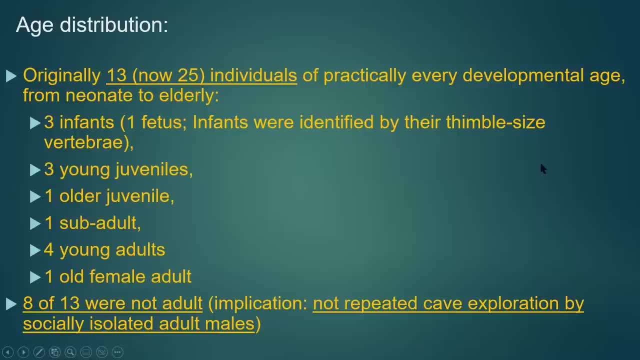 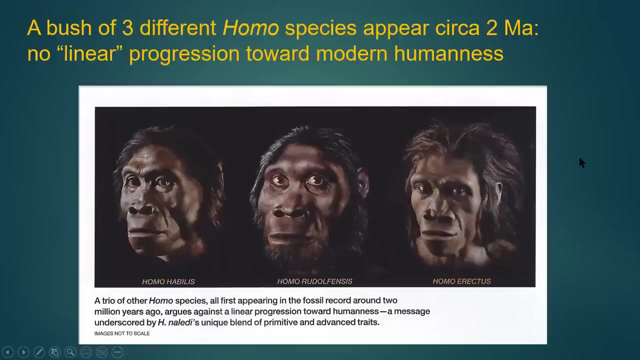 interesting because eight of the 13 are not adults, so this rules out that this was cave exploration by isolated adult males. that's not the pattern here. it looks like a group entered and didn't get out, and again here we have a bush of three different homo species at the same time. 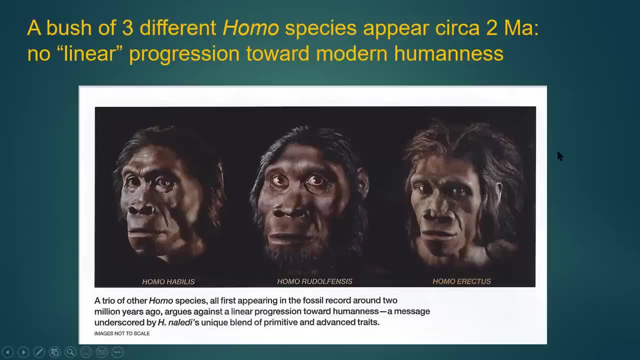 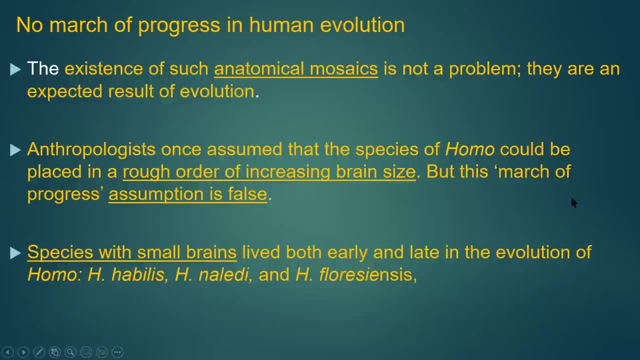 here here, hobbyless rudolphensis erectus, again showing no linear progression. basically, and most of these newer findings are all anatomic mosaics that they are- have show features that are ancestral and derived at the same time, and the old idea of a rough order of increasing brain size has now been falsified. species with 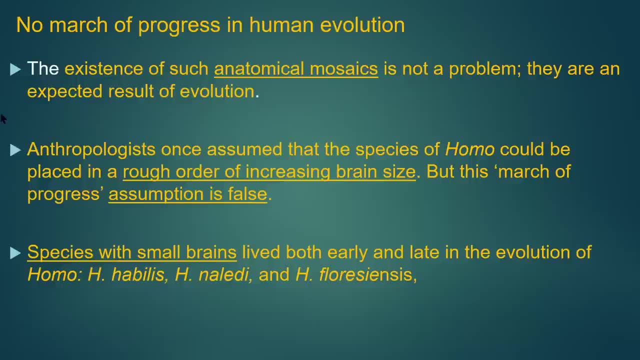 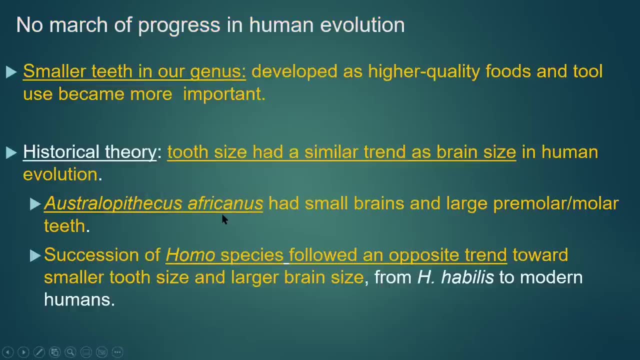 um shown that if you look at the, the inf iPhone also that the female of the female, male, male, but it shows the bigger range that the female is the smaller range the male is the same. uh, um, the male, that is the female male is the same age and the female is the same age. 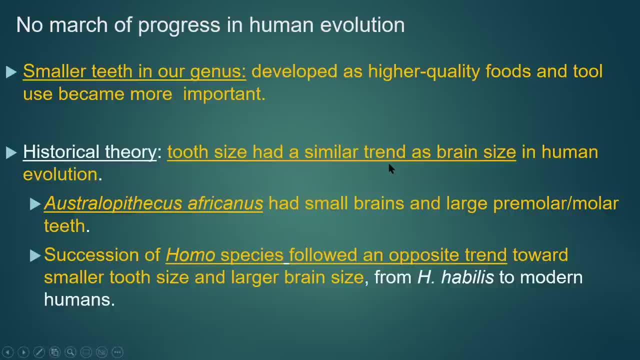 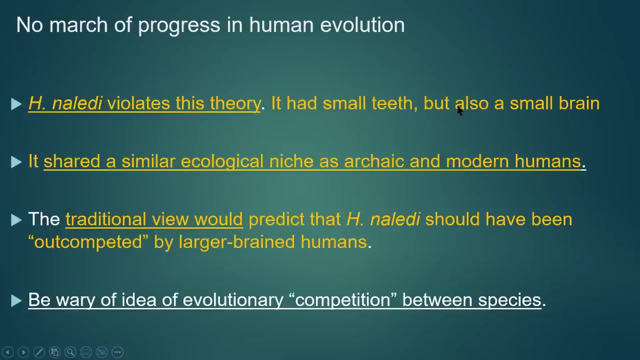 it's kinda a different thing. uh, there's a direct correlation between the two. we now in the these guys- mess this idea up. it's got small teeth but a small brain, and it shared the same ecological niche as some archaic and modern humans as well. so be wary of the idea of competition. 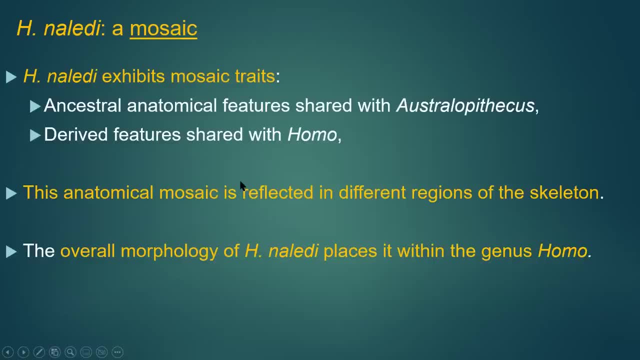 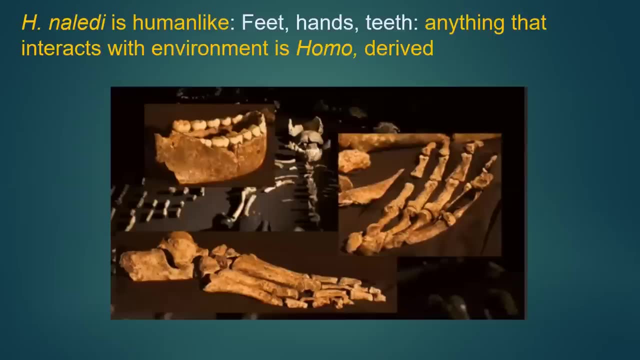 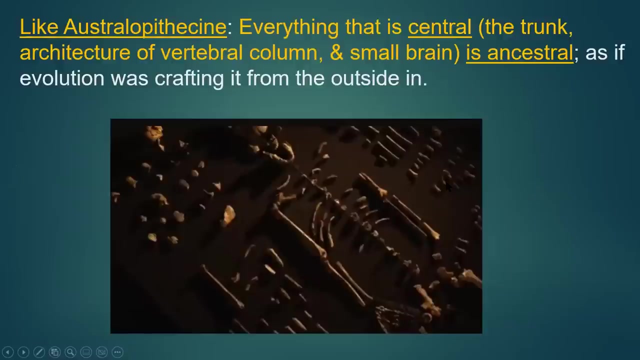 between species, because it may fool you. so mosaic traits: the homo naliti is human when it interacts with the environment. so feet, teeth, foot are all homo like, but it's like Australopithecus means ancestral on the inside stuff, pelvis, etc. okay and interestingly, naliti. 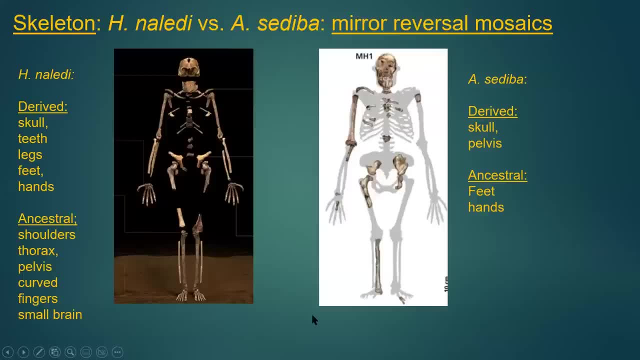 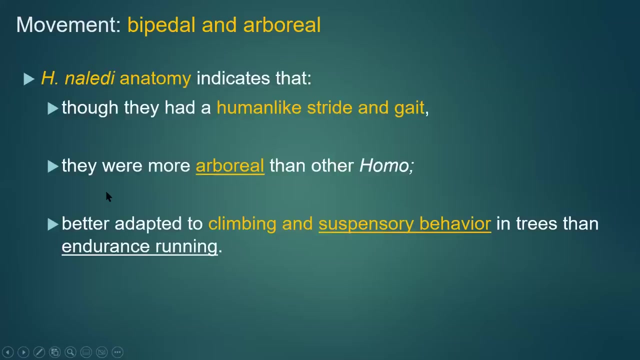 and sediba are the exact opposite in this regard. they've got derived skull, teeth, legs and hands, whereas that's ancestral in sediba, and the opposite pattern for shoulders etc. so an interesting sort of mirror opposite imaging. they were clearly arboreal then the other homos at the time. they clearly were able to climb and suspend themselves. so 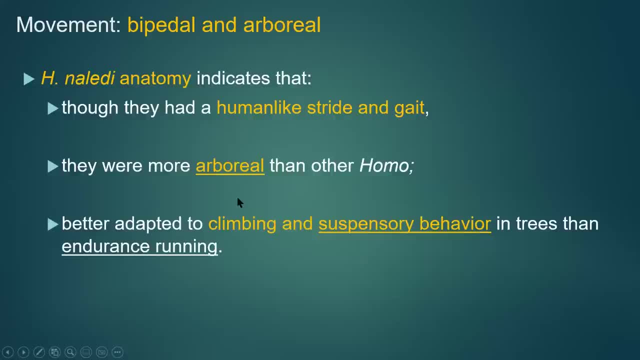 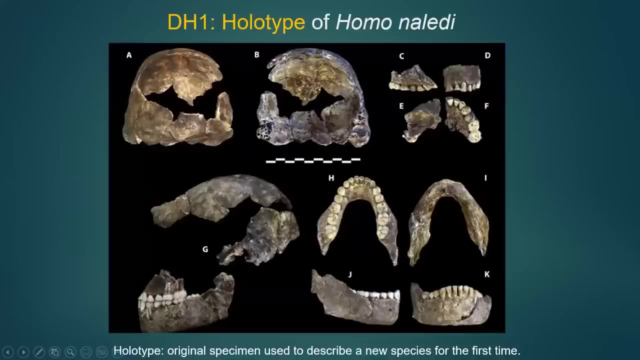 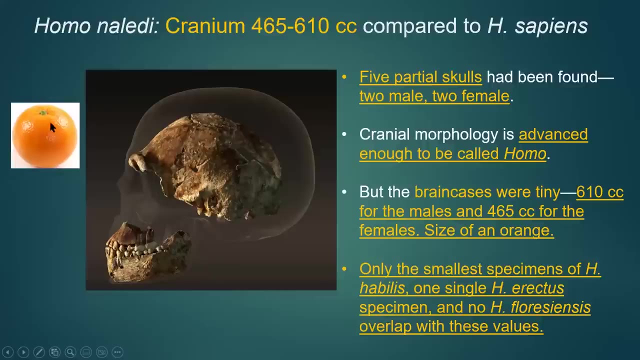 they weren't just walking and their gait, apparently, was looked somewhat different. this is one of the skulls from the denality cave. this is the holotype, very small brain size of an orange. okay, um, and they are a very interesting species. for this species, they are, of course, defined as homo and only the smallest species of hobulus, one of erectus and no. 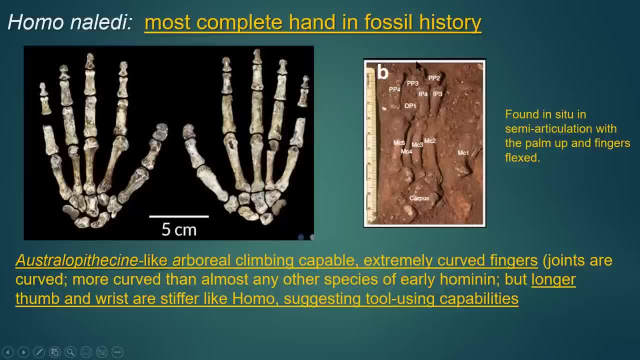 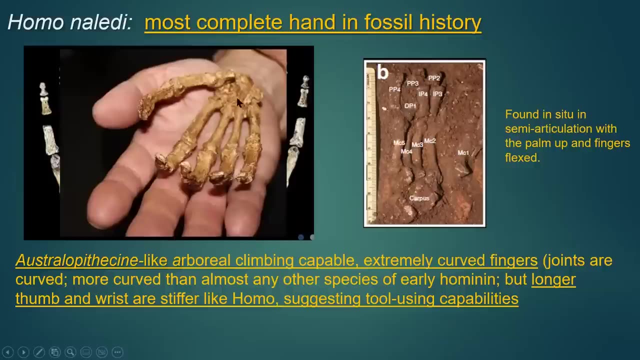 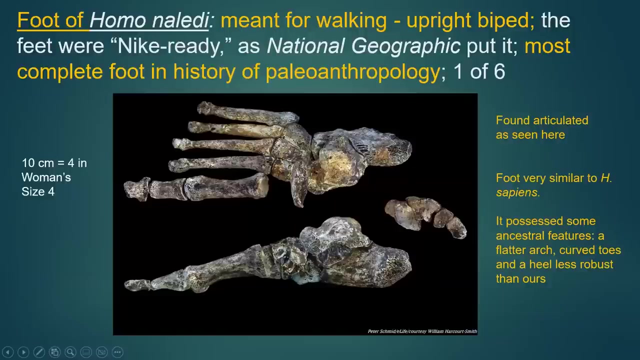 floresiensis overlap these values there. the hands are beautiful, okay, and they were found exactly sitting the way they look, basically, but amazingly curved, built for arboreal existence, and incredibly diminutive, okay, compared to us. And this is an incredibly beautiful foot that was articulated just like that. when they 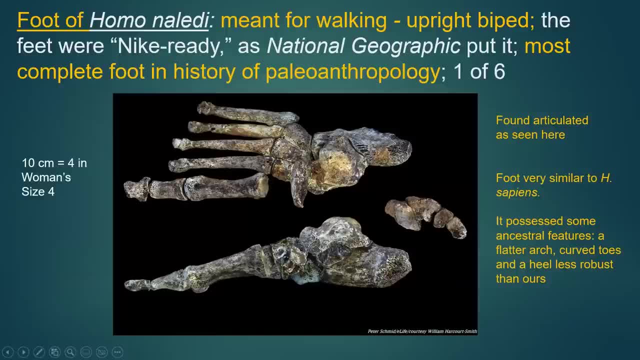 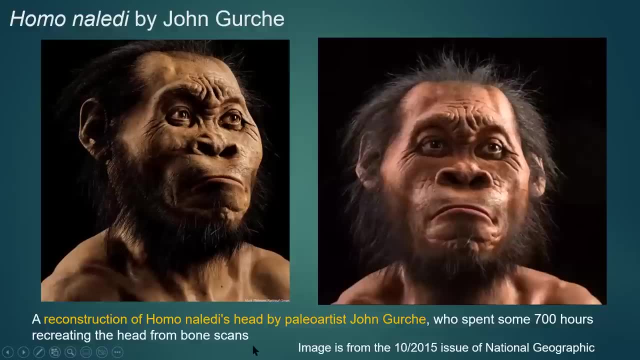 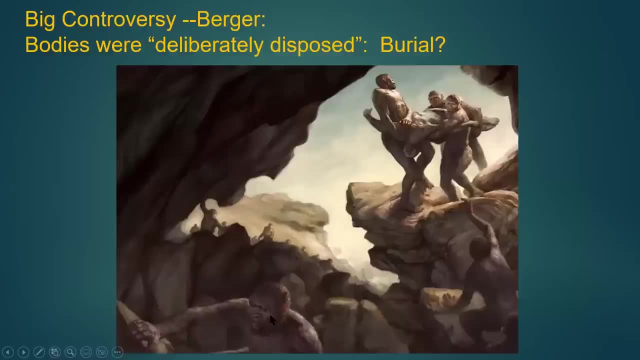 found it. It's the most complete foot in the history of discoveries. basically- And this is John Gurchy's reconstruction of what he thought- It took him 700 hours to come up with this. The hugest controversy of all was when Lee Berger concludes his journal article with: 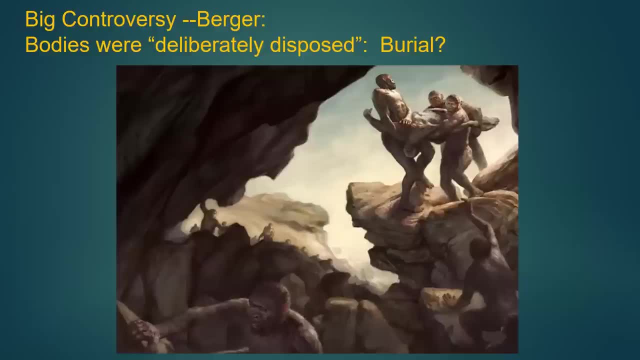 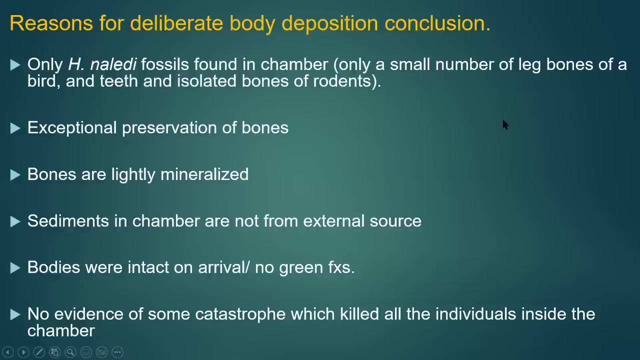 the proposition that he thinks that they were burying their dead. okay, The bodies were deliberately disposed, that they were bringing in bodies over time because some of the bone layering et cetera seemed to indicate that it wasn't just one group that ended up in there, And so their conclusion of this body disposal idea. 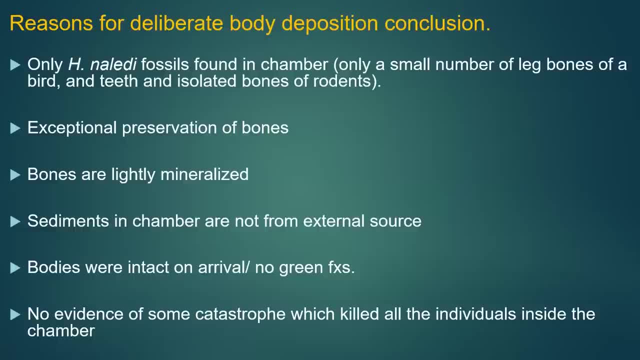 was that only Naledi fossils were found in the chamber. There are a couple of bird bones and a number of other bones. The bones are well-preserved. They're lightly mineralized. The sediments in the chamber aren't from an external source. The bodies were intact on arrival. There are no green 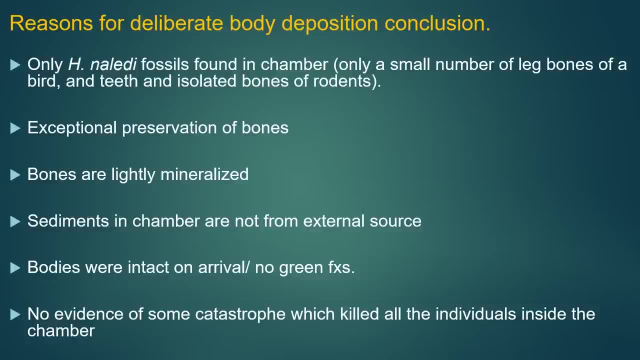 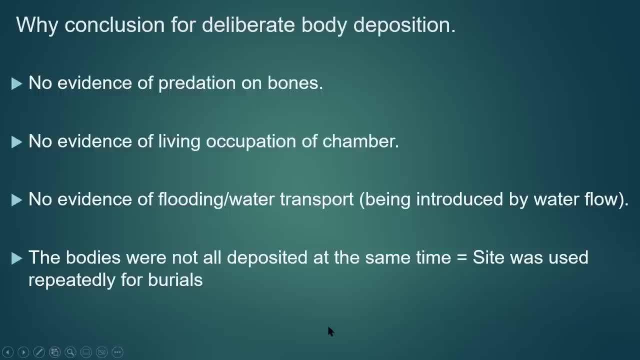 fractures. in that light, There's no evidence of a catastrophe which killed all the individuals inside the chamber. There's no predation on the bones. This is not a living chamber where they set up fires et cetera. There's no evidence of flooding that would have brought them in. The bodies were not all deposited. 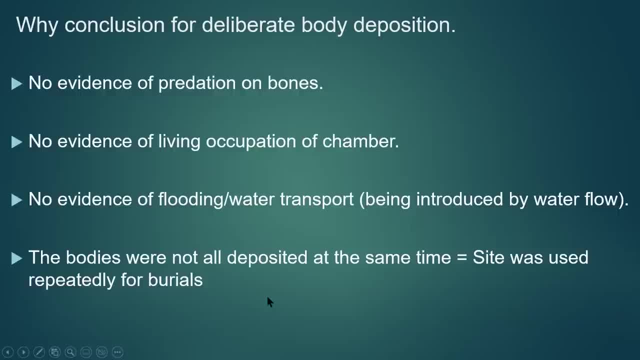 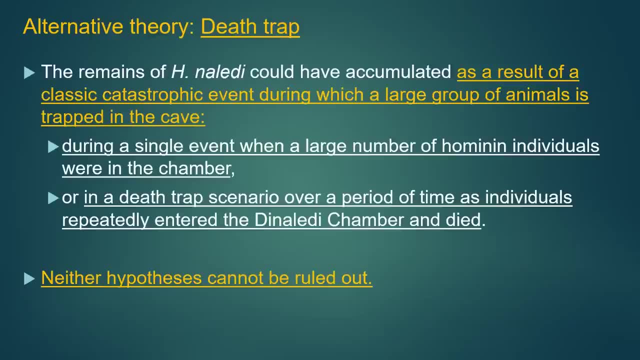 at the same time, so it was a repeat event, at least once. The alternative theory, of course, was that this was some kind of death trap that they entered because of predators or thunder or whatever and couldn't get out. Remember, this was a totally, absolutely pitch black. 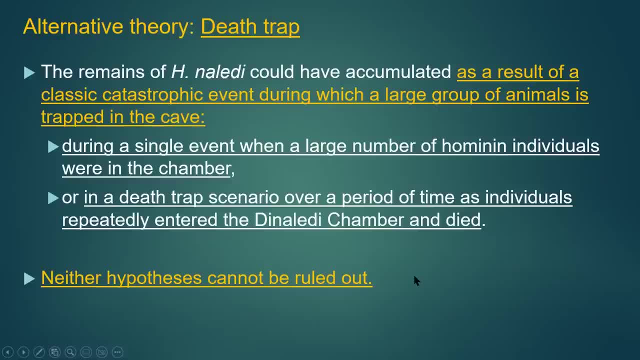 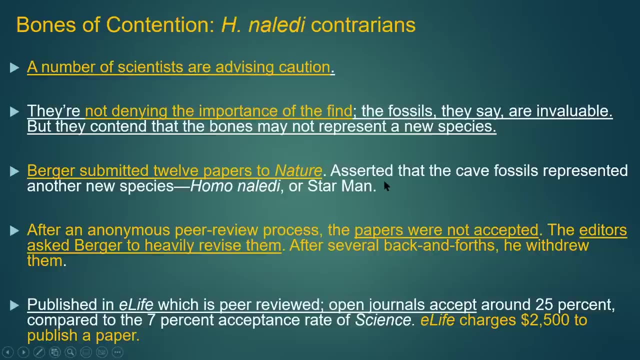 cave, okay, underground. They don't know that there was ever another opening to this cave And these death trap scenarios can't be ruled out, but the original authors poo-poo them, basically, Obviously bones of contention. Other scientists have submitted controversial stuff, So Berger submitted: 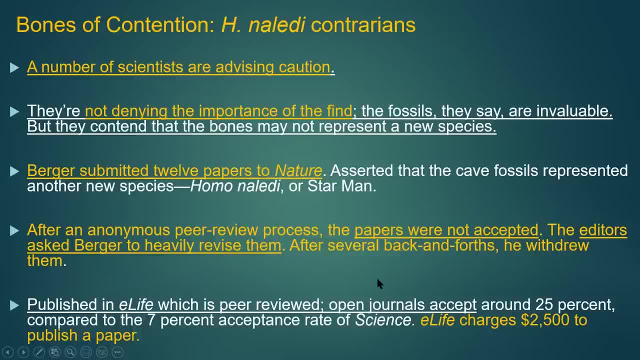 12 papers to Nature. After anonymous peer review, the papers were rejected. The editors asked Berger to revise them. After several back and forth, he withdrew all of them and eventually published them in eLife, which is peer reviewed. But open journals like this accept 25% compared to 7% by Science and 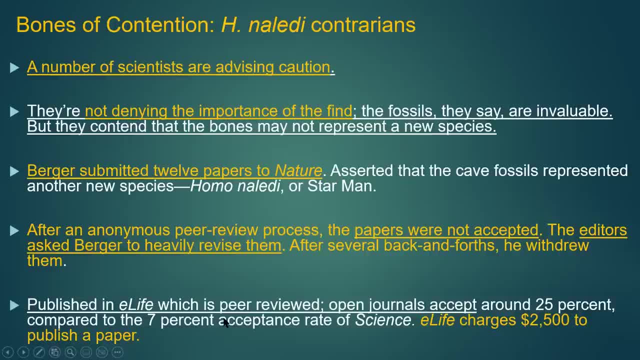 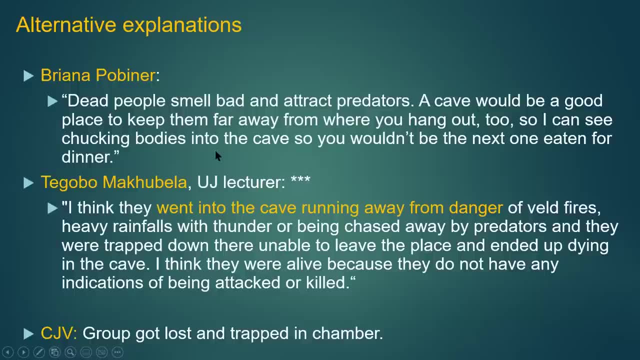 Nature eLife charges $2,500 for publication. So this is a good reason to go out and look at the data to see if there's any evidence that there's any other evidence that this was a trap. Okay, Rhianna Pobner says dead people smell bad and attract predators. A cave would be a good. 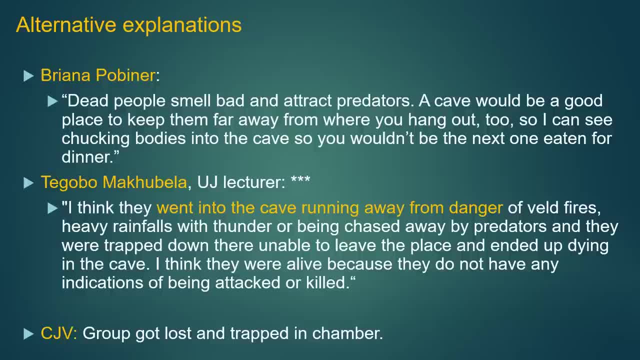 place to keep them for a while, from which you hang out, So I can see chucking bodies into a cave, so you wouldn't be the next one eaten for dinner. An African researcher said that he thinks that they went into the cave running away from some kind of disaster and ended up trapped there. 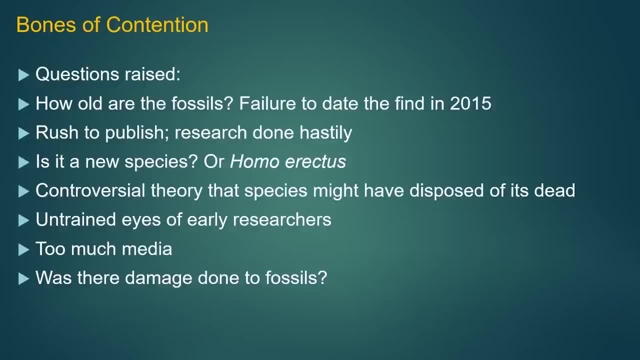 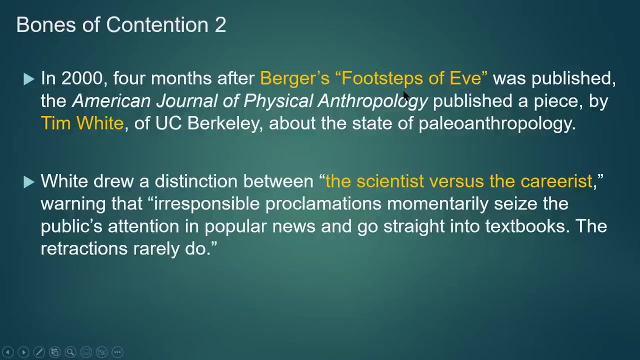 raised. How old are they? In 2015,, we didn't know. There was a rush to publish. Research was done hastily. Is this a new species or a version of Erectus? The burial controversy: too many early researchers, too much media. Was there damage done to them? Back in 2000,, Berger wrote a book. 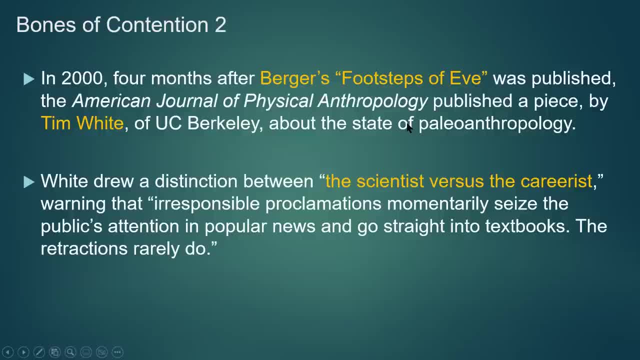 called The Footsteps of Eve. that was published And then Tim White wrote an article on the state of paleoanthropology in response And he drew a distinction between the scientist versus the careerist, warning that irresponsible proclamations momentarily seize the public's attention in popular 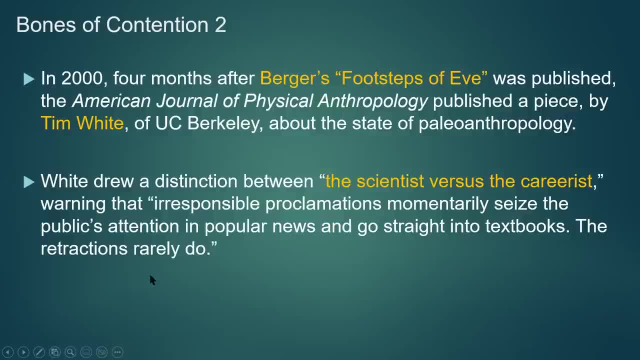 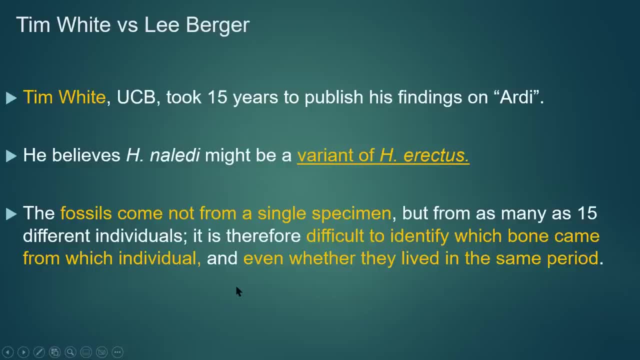 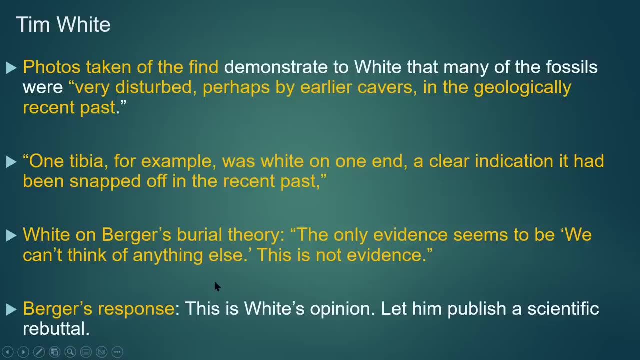 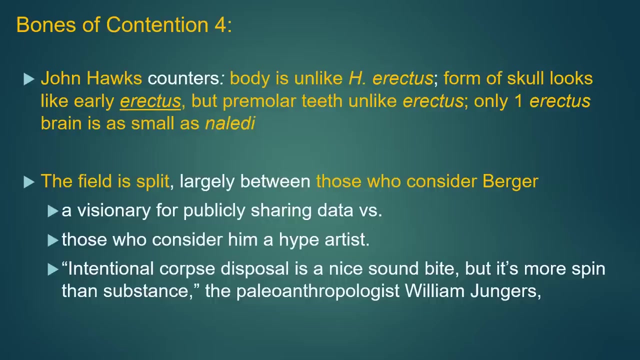 news and go straight into the textbooks and the retractions rarely do. Tim White does not like Lee Berger, It's pretty clear- And White thinks it's a variant of Homo erectus, not a new species, And so lots of controversy. John Hawks contends that it isn't Homo erectus. 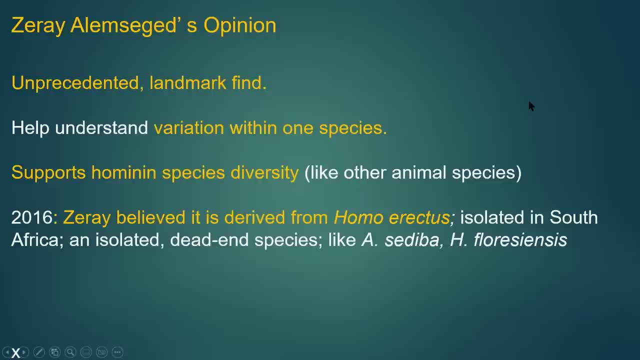 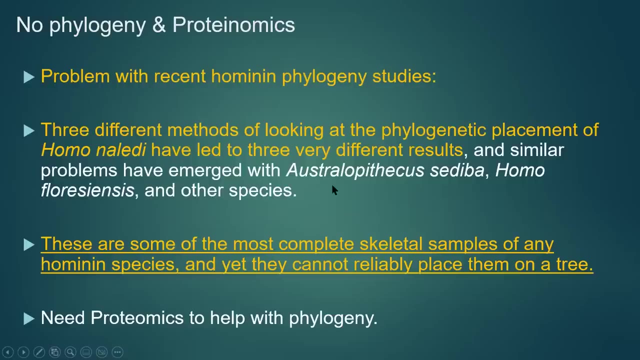 Zeray thinks it's an unprecedented landmark finding, but it represents variation within one species And he thinks it's probably derived from Homo erectus And, interestingly, both with Naliti floresiensis. we've got these lots and lots of bones And they keep trying to do. 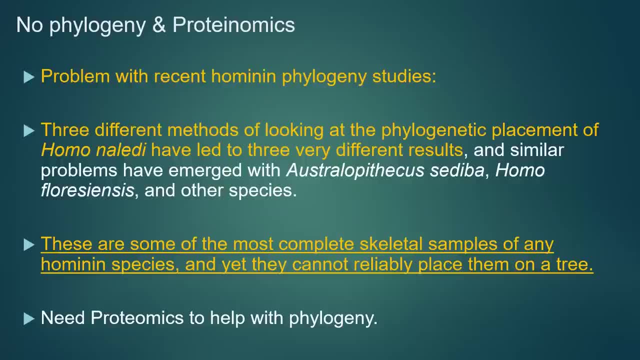 phylogenetic placement, taking one characteristic, comparing it to all others and then trying to figure out where they originated. And so he thinks it's probably derived from Homo erectus, And he thinks it's probably derived from Naliti floresiensis, because basically, these guys are 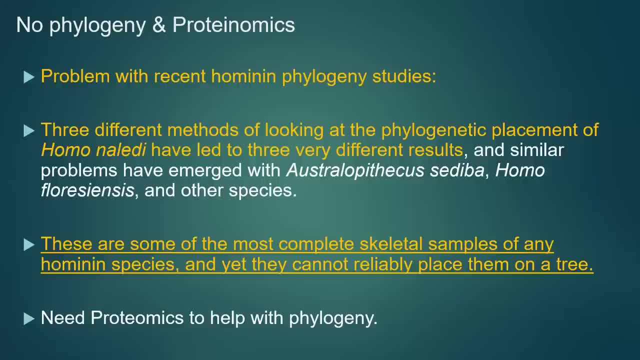 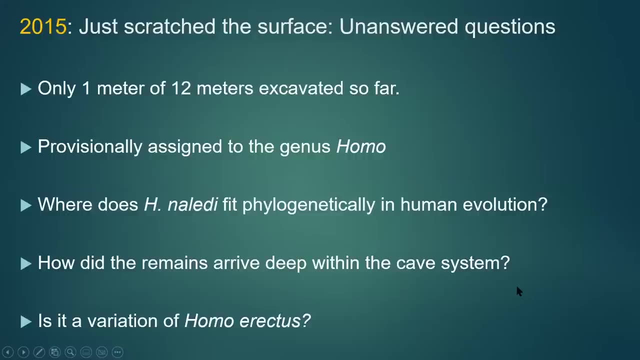 completely identical. So the phylogenetic attempts have not yet DNA has not succeeded in any of them, And they need to now do protonomics, basically to try to help figure out the phylogeny of these guys. So lots of continuing questions in this regard. Fabulous find, but lots of questions, And I don't want to get into the technical details of this, but there are lots ofág of questions in this regard. Fabulous find, but lots of questions. And so we will move on to the next insight, the next slide. 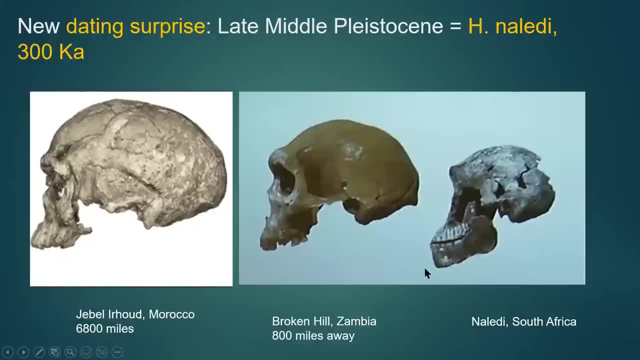 Okay, Okay, Okay, Okay, Okay, basically. And then they do the dating And it turns out to be exactly identical to Jebel Erhoud in Morocco, Broken Hill in Zambia, and Nelidi comes in at 300k. Okay, so they're right. 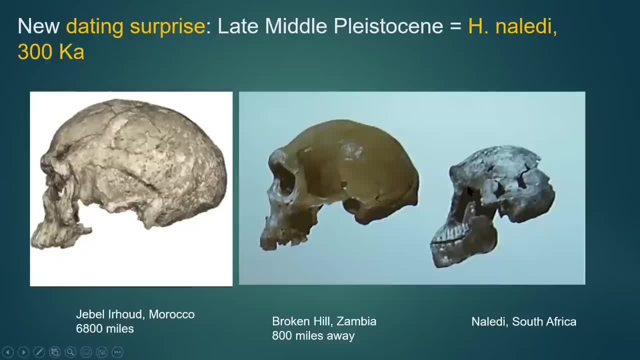 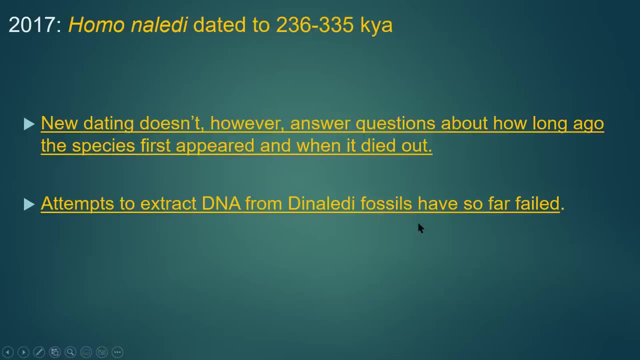 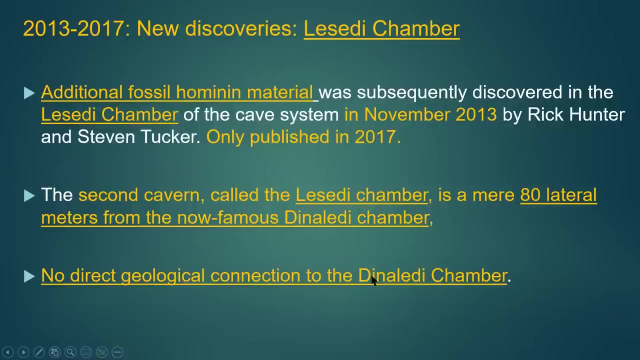 at the same time, at least these bones are 300k. We don't know when they started or when they disappeared. Okay, So continued mysteries And that was based on geological analysis, But we still have lots of questions there. And then, in 2017, after having been discovered by 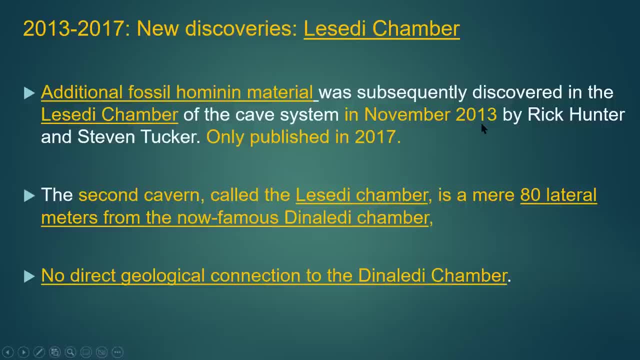 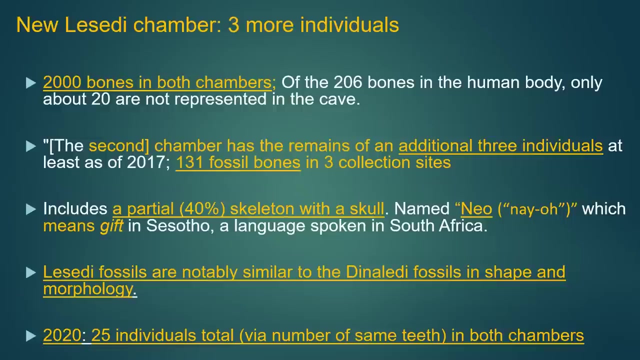 Rick and Steve in 2013,, a new chamber called the La Citi chamber, which is unconnected to the Nelidi cave And it's 80 meters away in a different cave. basically, There's no geological connection between the two caves And so between the two, they now have about 2000 bones in both chambers. 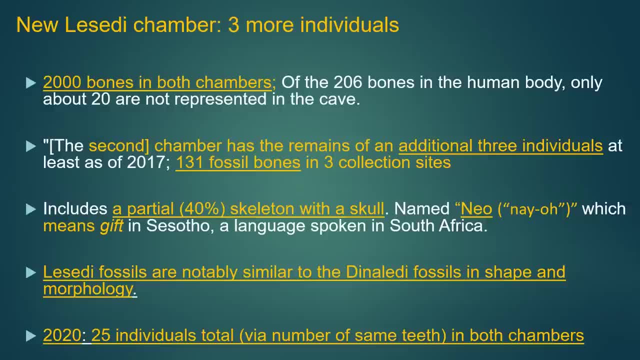 130 in the new one and 372 in the new one, And then there's a new skeleton called Neo in the new cave. That's interesting, But they now think there are about 25 different individuals based on the number of same teeth in the two chambers. 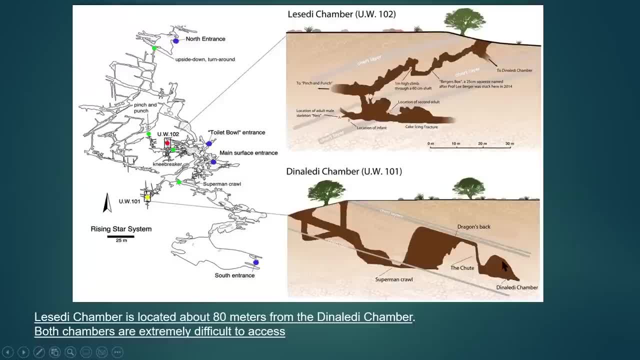 The one. this is the original Nelidi cave And this is the new La Citi chamber, but not connected to the Nelidi cave, And so they've been doing a lot of research on this, And they've. This is a massive cave system, by the way. Who knows? 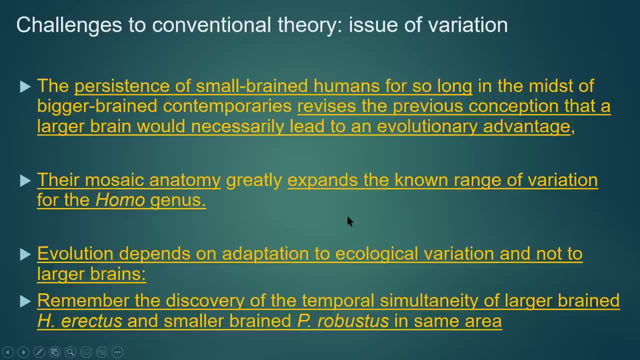 OK, so again sort of more challenges to some of our thinking. The persistence of small brained humans for so long kind of reverses our previous conception that larger brain would necessarily lead to an evolutionary advantage. Their mosaic anatomy expands the known range of variation in Homo. 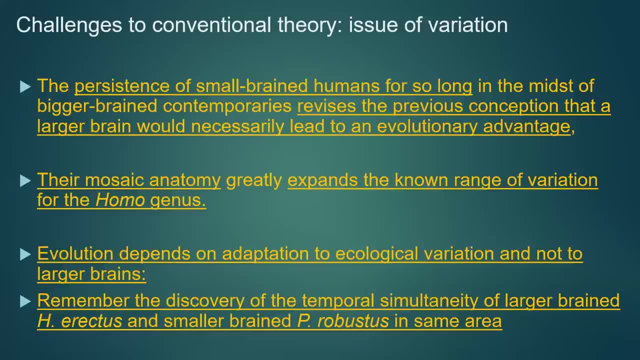 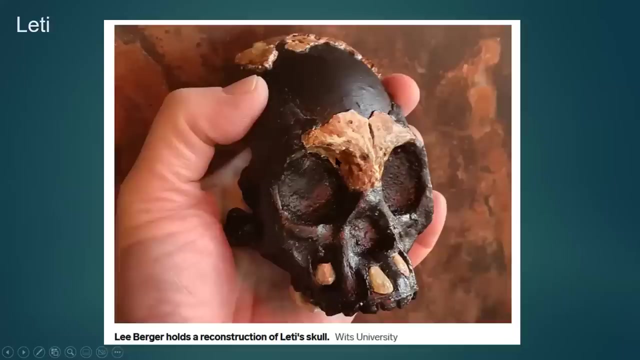 Evolution depends on adaptation to the ecological variation and not larger brains, basically, And remember that we keep finding different species of these groups in the same place at the same time. So lots of Bush Differences. basically, in the new cave they discover the first child of six years of age that they put together. 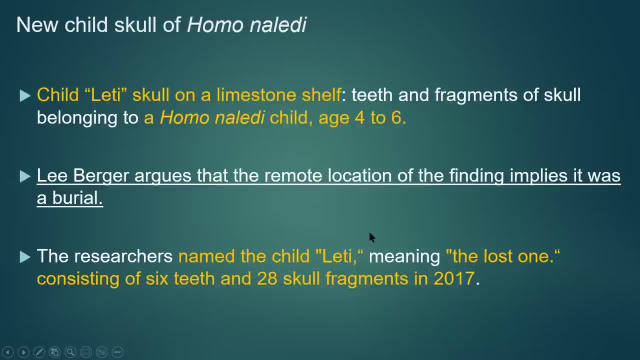 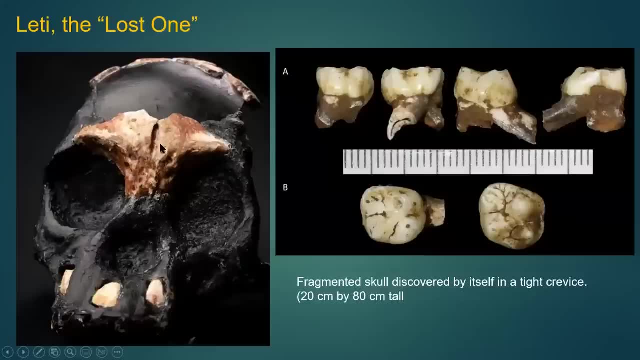 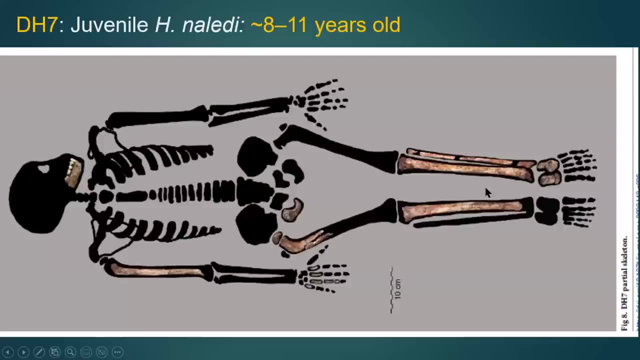 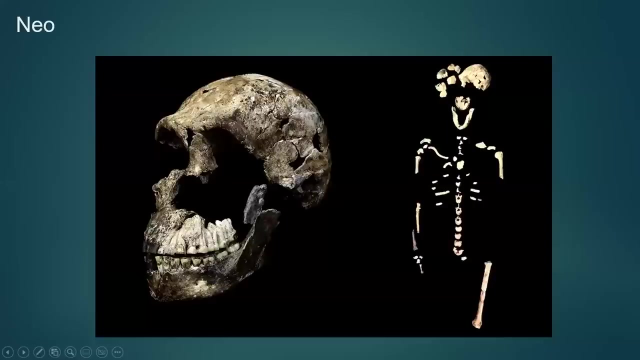 OK, All, let he they think four to six years old Teeth Skull bone parts, basically a third an eight to 11 year old juvenile, As some post cranials. This is neo skull and his skeleton. You need to be careful about the skeletons because they're put together by all kinds of bones. 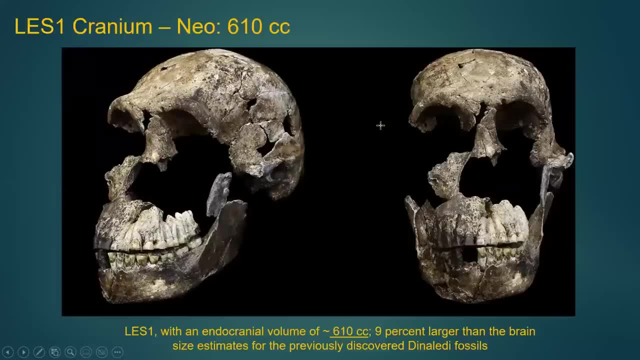 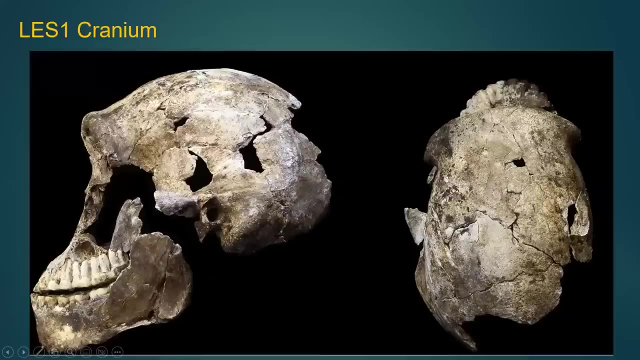 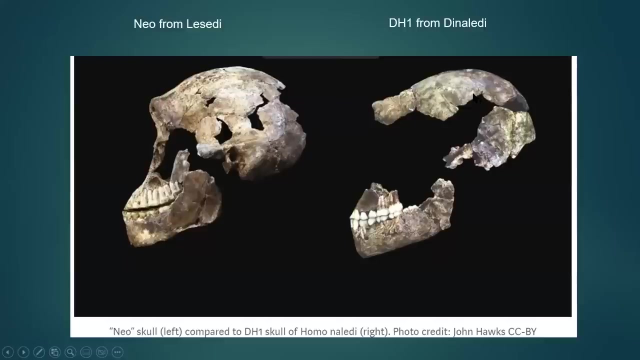 It isn't necessarily the original same person, but this is a very nice skull. Basically 200. I'm sorry, 610 CC. So the classic cortical Rubicon level. This is like city and this is didn't a lot That the two different skulls. 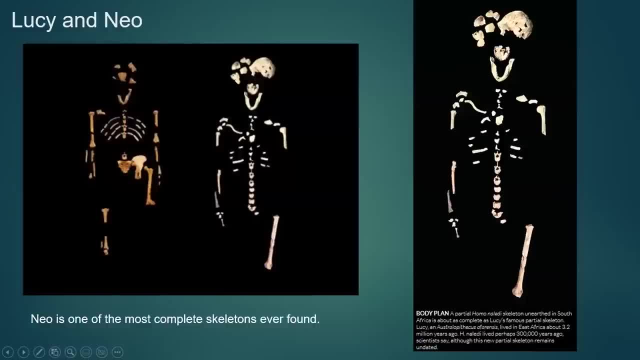 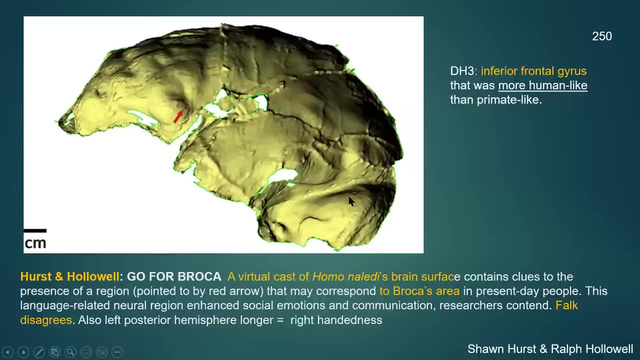 And this is Lucy And this is now They've even done an attempt at. They did a brain and a cast. Holloway, I did a brain and a cast They were hunting for broke his area And in modern humans, broke his area is the language known for its language expression ability. 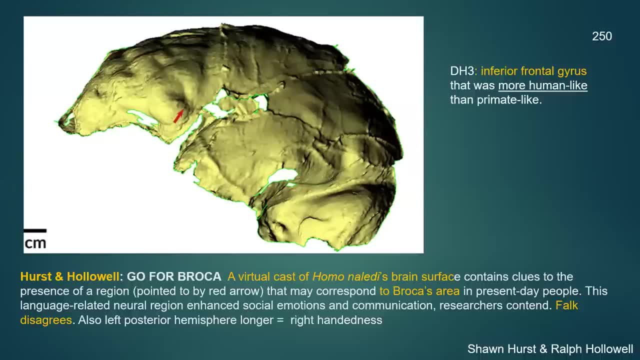 But originally it was the manual stone making region of the brain And that's an interesting connection between the kind of hierarchical step system that you have to do to carve a bone And that's the connection why this area got absconded for language in terms of hierarchical grammar etc. 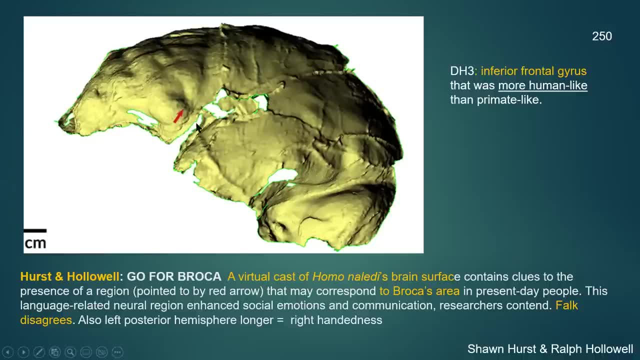 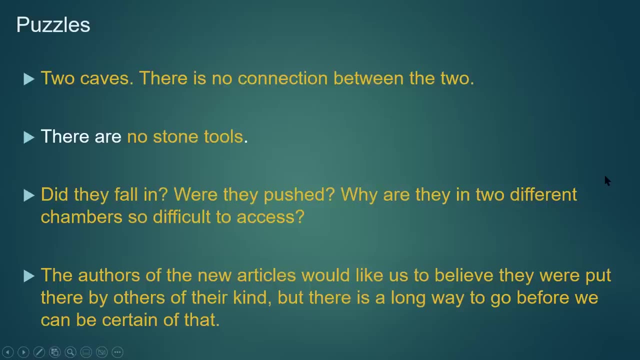 But Holloway thinks this could be broke. as Falk, his longtime nemesis, She disagrees: Okay, And this is the most recent reconstruction of nail. So two caves, No connection, No stone tools. Did they fall in, get pushed in, etc. 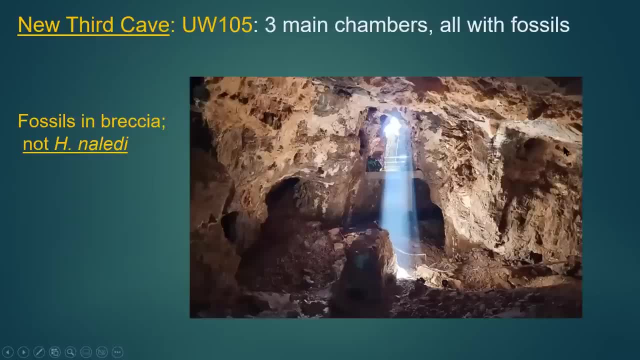 And then, of course, new cave, But this one is not home when they living. This is an old, rocky South Africa style cave that they have found a whole bunch of new bones. They have built a stairway going in. Apparently It was the site of a movie at one point. 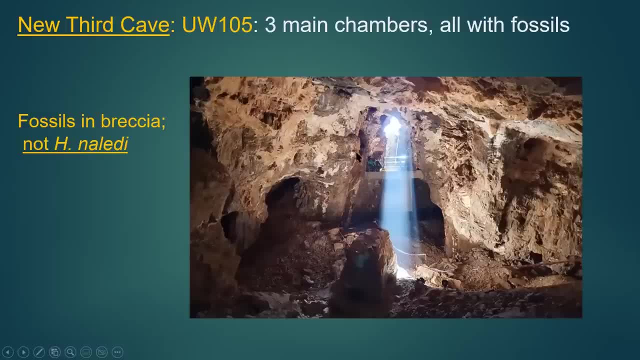 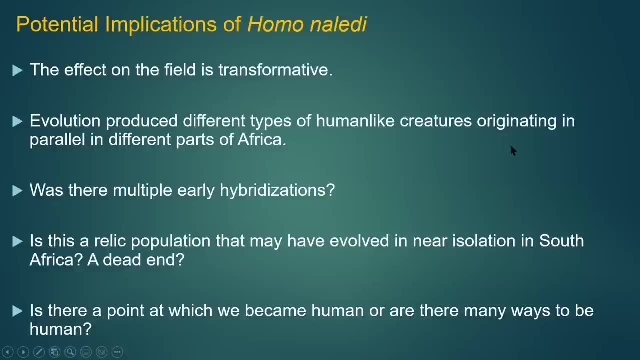 Because there's lots of movie evidence in it And this has not been published yet. So the implication It's been sort of transformative in some ways, But evolution clearly produced different types of, almost originated in parallel in different parts of Africa, Where their hybridization 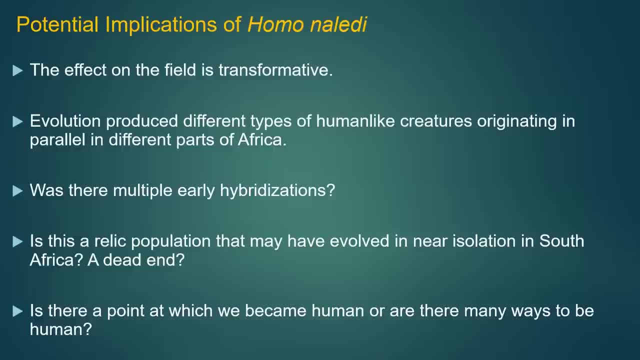 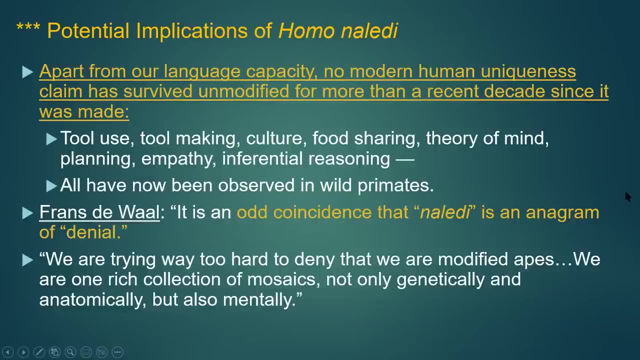 We don't know Where they dead ends, Probably. Is there a point at which we become human, Or are there multiple ways to be human? Most likely, Okay, And apart from our language capacity, It's really important to remember that no modern human uniqueness claim. 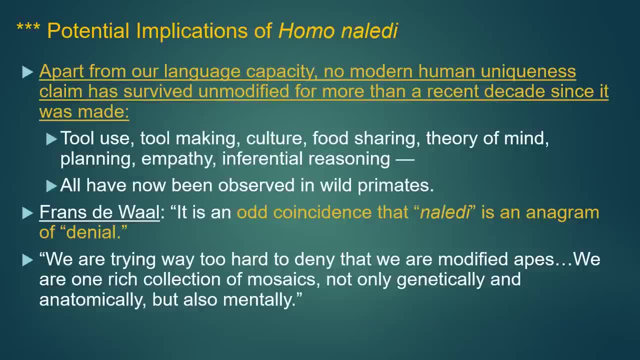 Has survived unmodified for more than ten years Since it was made Tool use. tool making, culture, food sharing, theory of mind, planning ability, empathy, inferential reasoning have all now been observed in wild primates. Franz de Waal says it's an odd coincidence that Neliti is an anagram for denial. 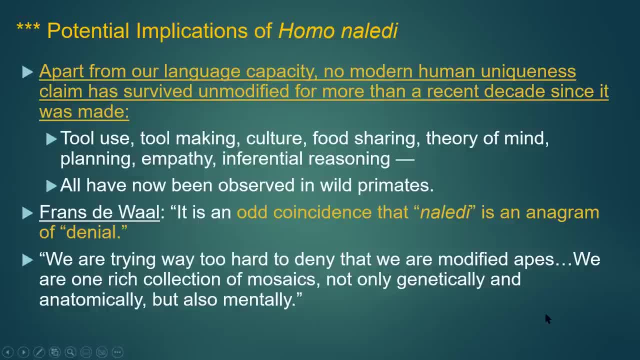 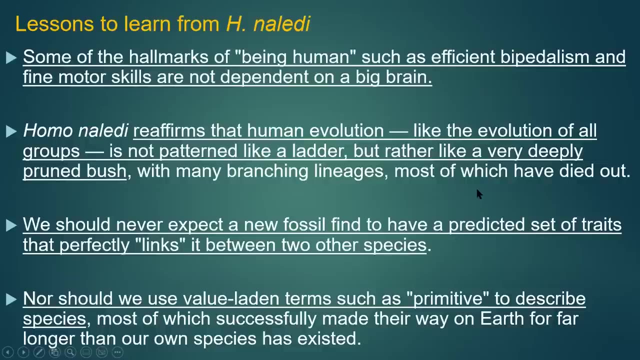 I like that one. We're trying way too hard to deny that we're modified apes And we are one rich collection of mosaics- genetically, anatomically and mentally as well. Some of the lessons, some of the hallmarks of being human, such as efficient bipedalism, fine motor skills, are not dependent on a big brain. 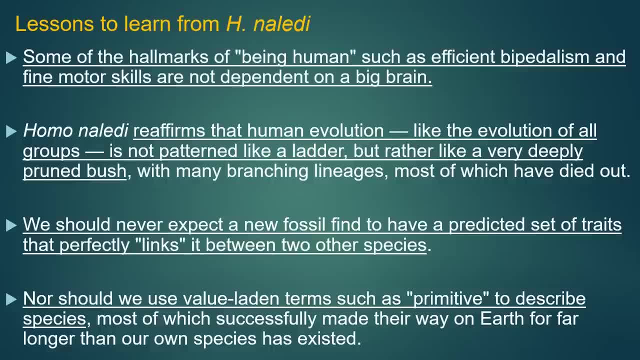 Neliti reaffirms that evolution, like evolution of all groups, is not patterned like a ladder, but rather like a deeply pruned bush. We should never expect a new fossil find to have a predicted set of traits that perfectly links it between two other species. 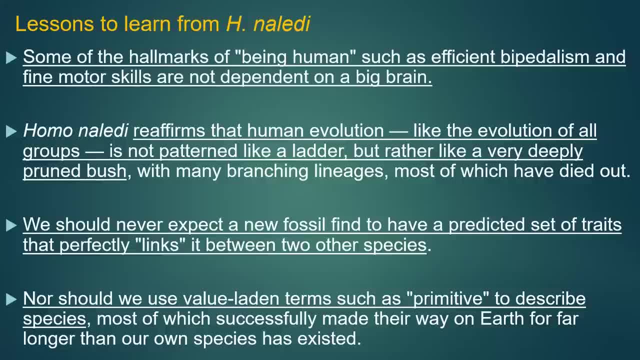 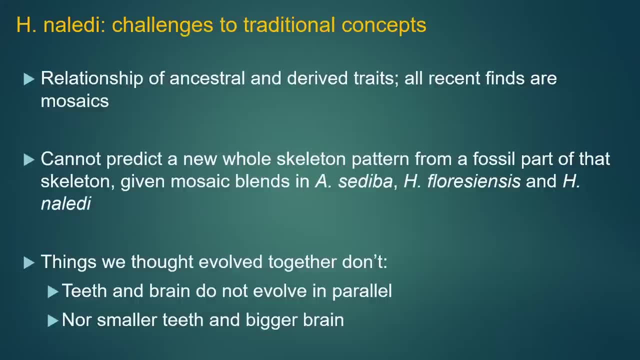 Nor should we use value-laden terms like primitive to describe species, most of which successfully lived on the planet for far longer than we did. okay, or have all right The finding that most of these guys are mosaics of ancestral and divine features. 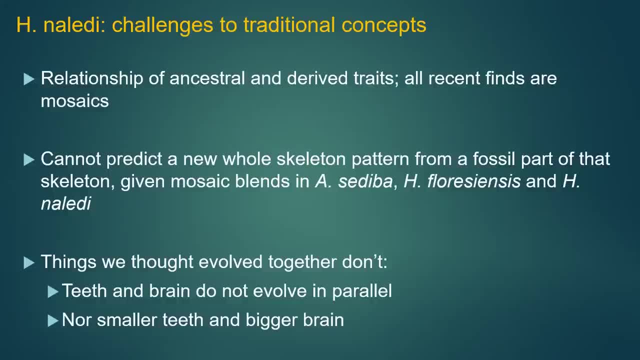 Okay Okay. You can't now predict if you find a little bone piece, predict what the rest of the skeleton is going to look like, because all of these guys turn out to be weird blends of ancestral derived et cetera. 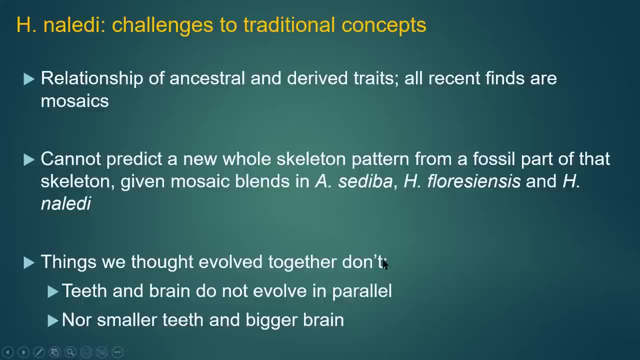 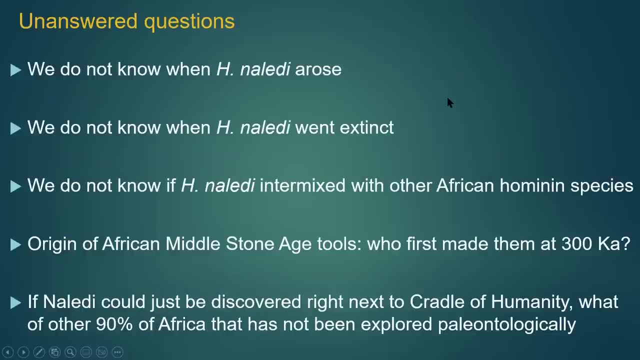 And what we thought evolved together don't Teeth and brain? smaller teeth, bigger brain, et cetera. Lots of unresolved questions. We don't know when Neliti arose or went extinct. We don't know whether they intermixed with other species. 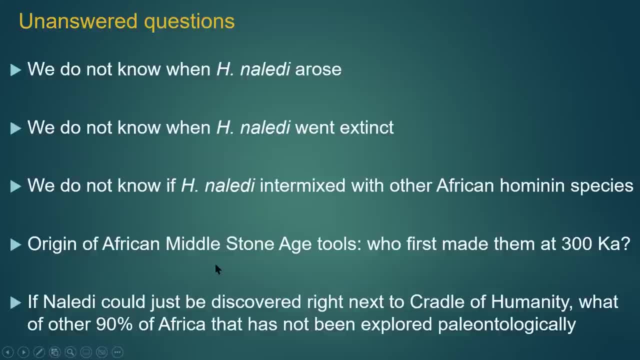 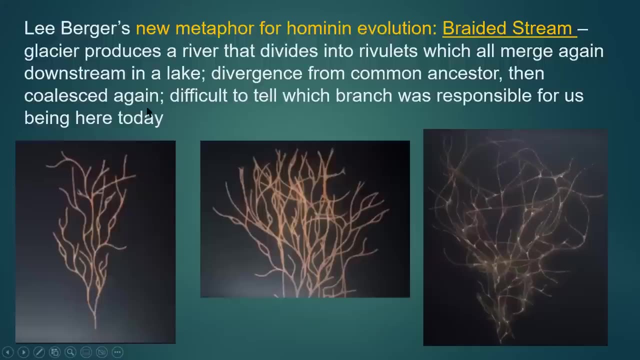 There's. Berger raises a question that we now don't know: the origin of the African middle stone age, which everybody thought happened at around 300 K. but was it us, was it Neliti, et cetera, he claims. And the one thing I do like about Lee Berger is he has he came up with the metaphor of a braided stream as being the way evolution works. 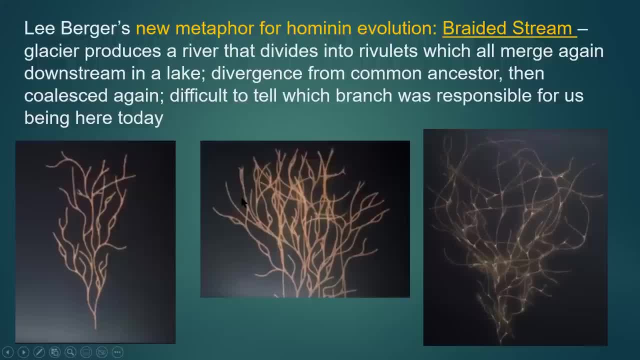 And the one thing I do like about Lee Berger is he has he came up with the metaphor of a braided stream as being the way evolution works, That divergence from a common ancestor, then coalesce again, then split again, then recombine again. 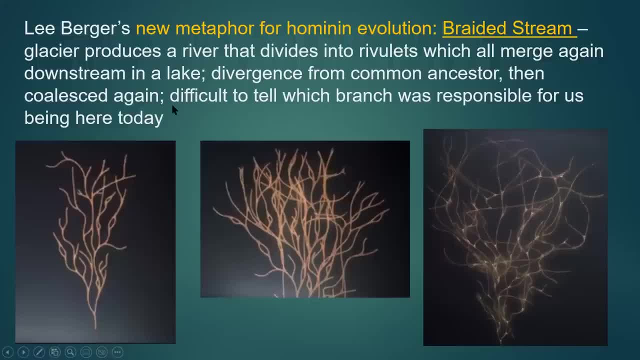 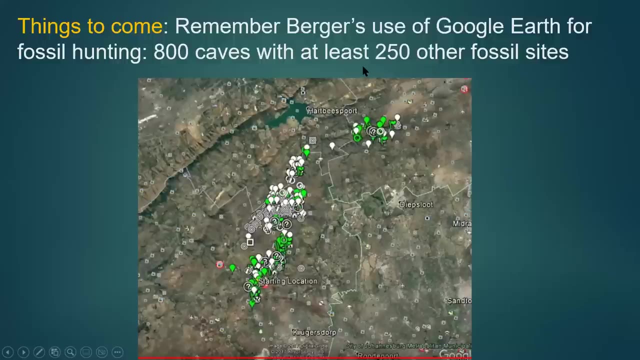 And it's difficult to tell which branch was responsible for us being here today. basically So the what happened in Africa Then. things to come. Originally, one of the good things that Lee Berger decided to do was that he used Google Earth. 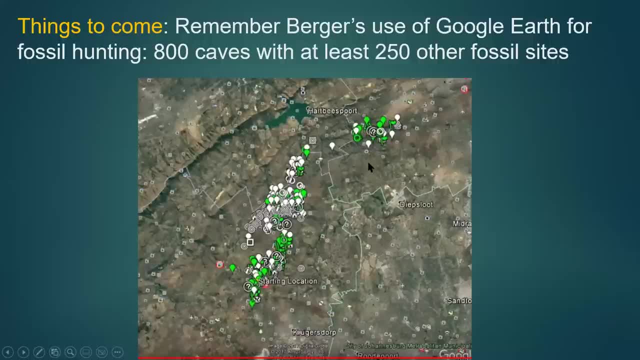 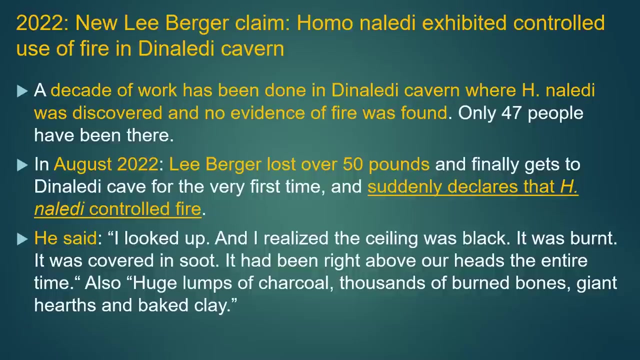 To begin looking at patterns of where trees and water and caves existed in South Africa, and he's discovered 800 caves. at least 250 may have maybe fossil sites. Okay, so lots to come, basically. And then, of course, always wanting to be in the news Late, last year he loses 50 pounds. 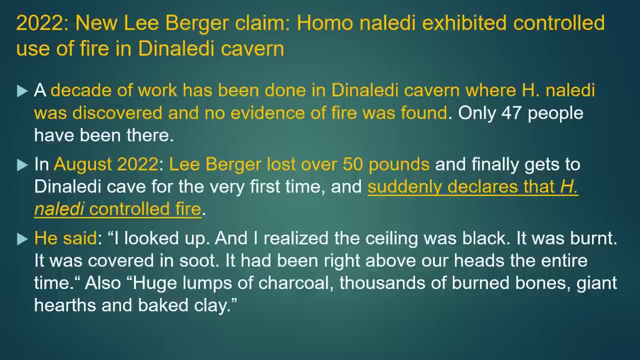 And ends up, finally, in The Dina letty cavern, where No evidence in 15 years of searching has been found for fire. And, of course, what does he declare? he declares that home on a lady controlled fire. I looked up and I realized the ceiling was black, it was burnt, it was covered in, so it had been right above our heads the entire time. 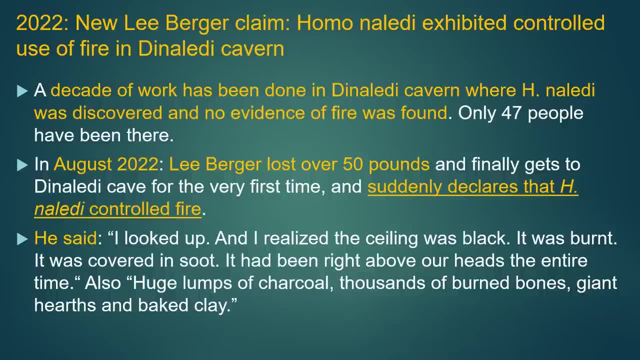 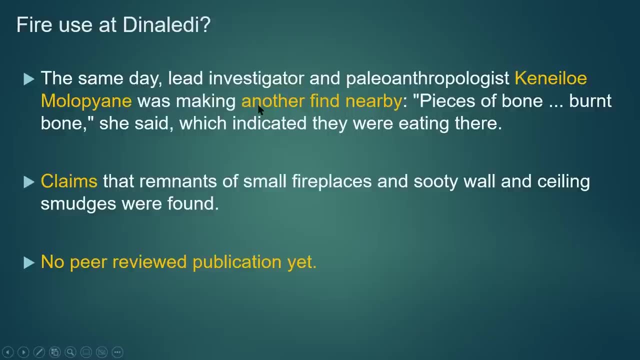 And no of the none of the other researchers and notice, Interestingly, huge lumps of charcoal, thousands of burnt bones, giant hurts clay, baked clay. His partner, an African researchers, Mulla pion, Said pieces of bone, burnt bone, which indicates they were eating here. 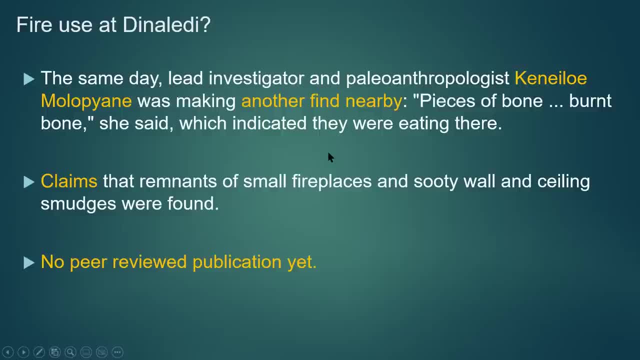 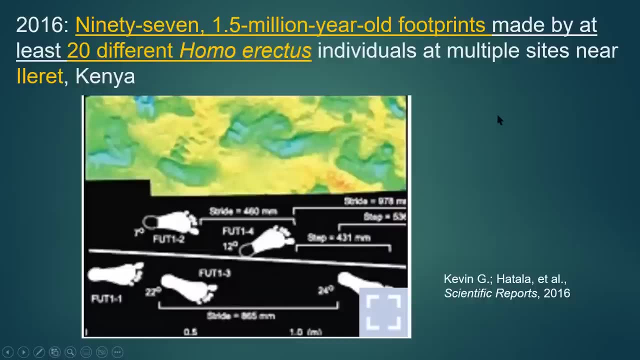 So this was a news conference? Okay, they've published nothing about this. Okay, so keep your fingers crossed. In 2016, 97 1.5 million year old footprints of homo rectus along a lakeside- I think Turkana- in. 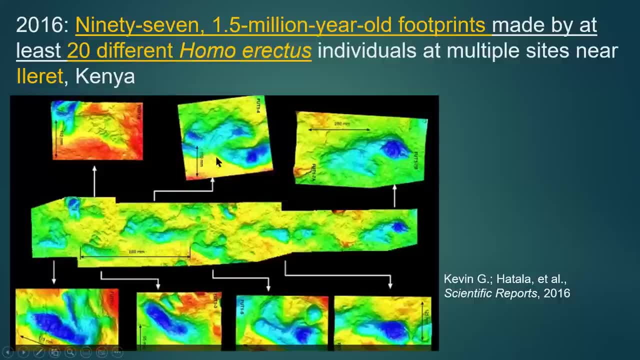 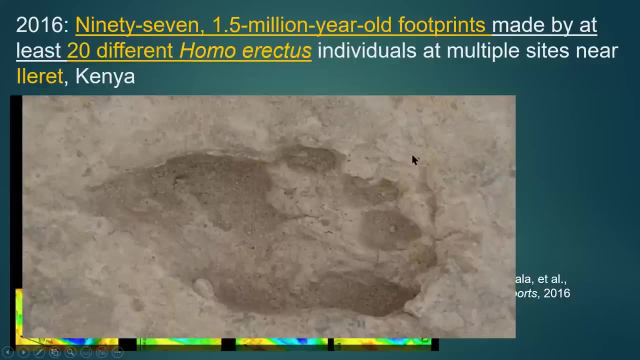 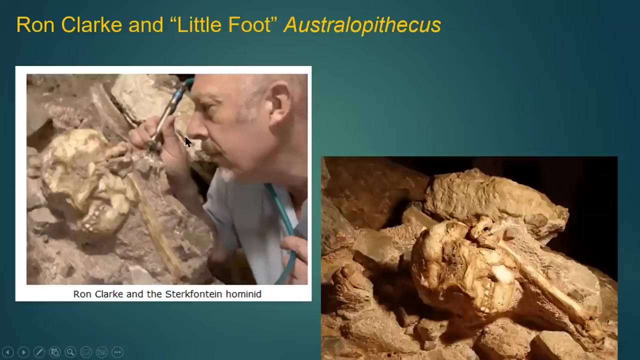 Billeret in Kenya. Okay, So they were started walking along a stream. They think they were probably hunting or foraging at this spot- And some beautiful footprints And some beautiful footprints And some beautiful footprints- prints that look exactly, uh, like ours. basically um wrong date there, um, and then we have ron clark. 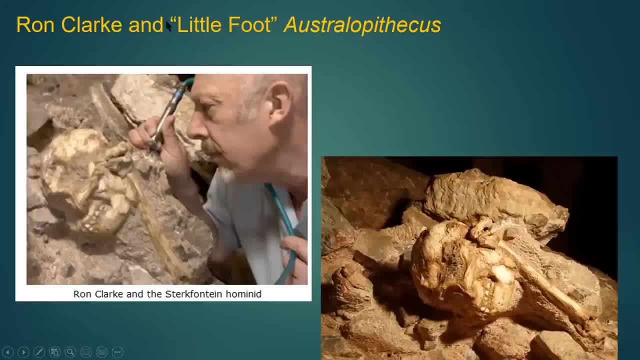 discovery of littlefoot and australopithecine, where there's a controversy as to uh which australopithecine but uh, he basically found a box with a couple of bones in it and sent his two african uh assistants down to the cave to see if they could find where they had been clipped. 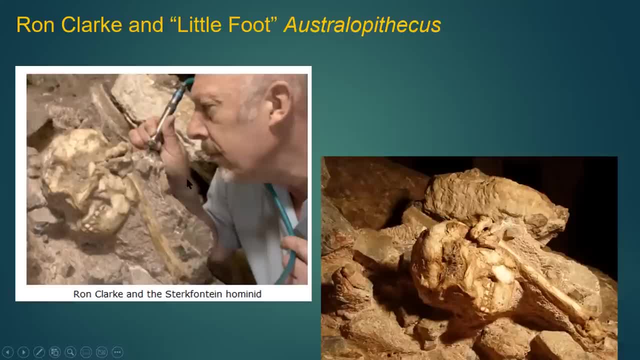 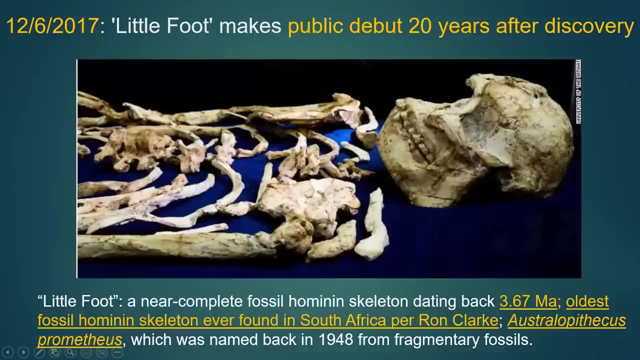 off in the wall. after two days of hunting they find them, and then for the next 15 years, those two assistants have been digging out, uh, this fossil. basically incredible job, right, and it is the most complete fossil hominin skeleton, dating back to either 2.2 or 3.6 million years ago. 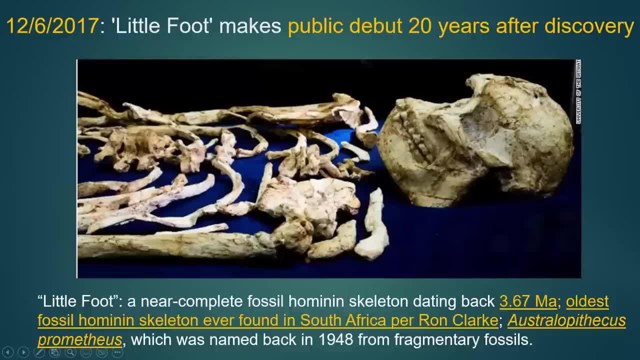 it's the oldest uh fossil hominin skeleton ever found in south africa for clark and he named it australopithecus prometheus uh, which was what was given a name in 1948 to another uh fragmentary uh fossil. but it's a beautifully preserved, incredible work by these two. 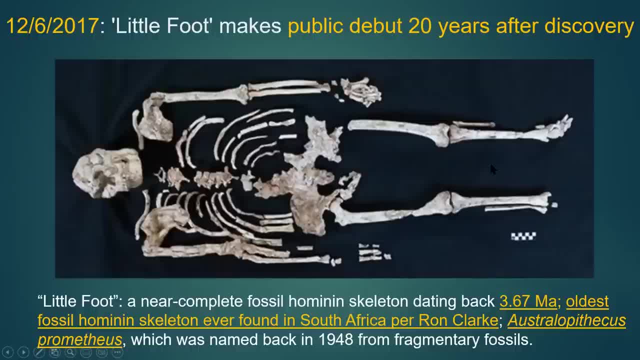 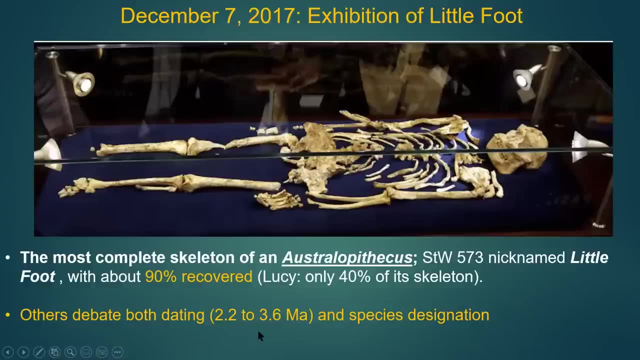 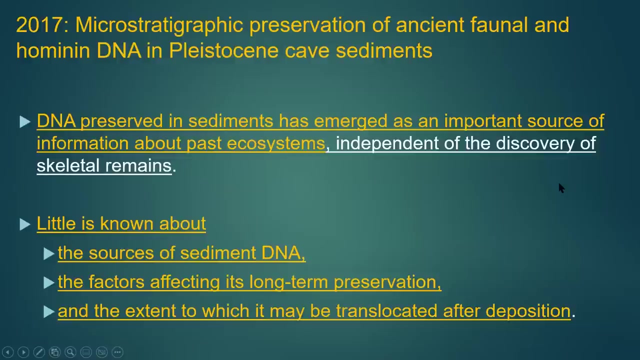 assistants and nicknamed littlefoot, basically, and was finally publicized after 15 years of work. the big debate is about how old it actually is, okay, and the species designation: um. and then in 2017- this jumps into our dna talk- but, um, they discovered that you could actually. 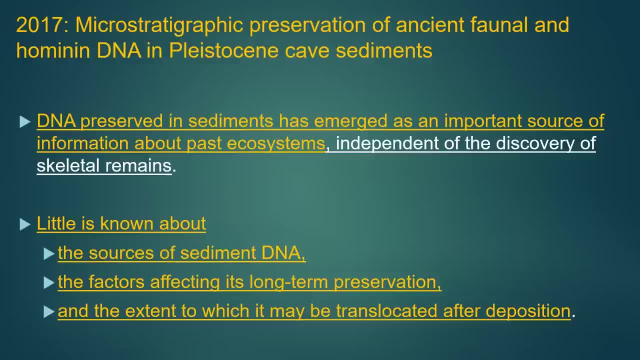 look at uh strategic stratigraphic geological layers and find dna alone in the sediment. this is an amazing discovery. um, there's little known about the source of the sediment dna. was it pee pooping, uh spitting? we don't know. okay, uh, the factors that preserve. 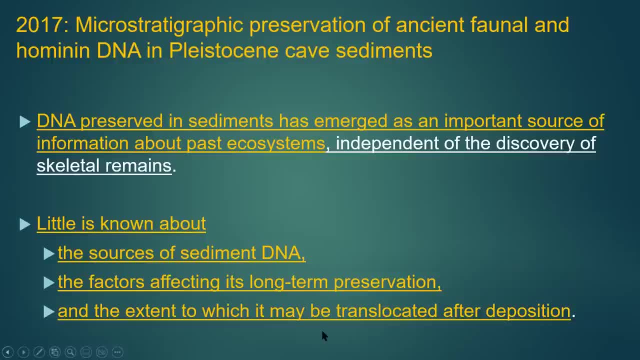 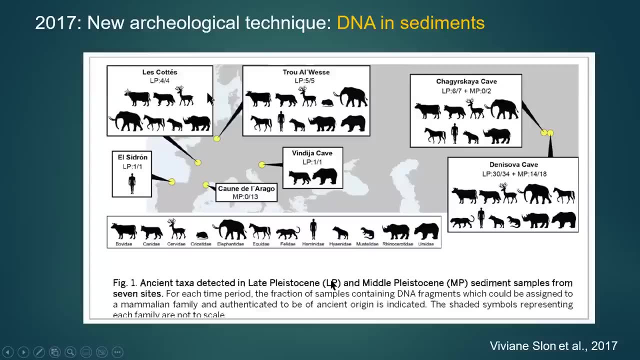 affect its long-term preservation, the extent to which it's preserved and the extent to which it's still preserved. toure' s have been dislocated from a different layer, okay, which is an issue in terms of dating, but basically they looked at um five different caves in uh europe and asia um and they found they were able to do uh species analysis based on some dna that was found in the dirt of these caves, without 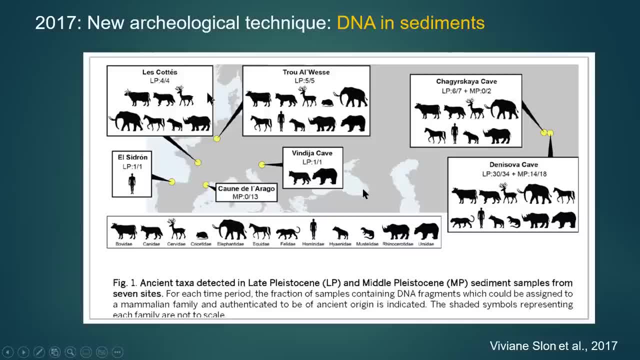 any fossil bone. an amazing achievement in terms of 1940 eti'mall 둬, exposition terms, of technology, including denisovan and neanderthal dna in the dirt. okay, they've now been doing a research on the naked mole rat, showing that you can get dna from the air. okay, 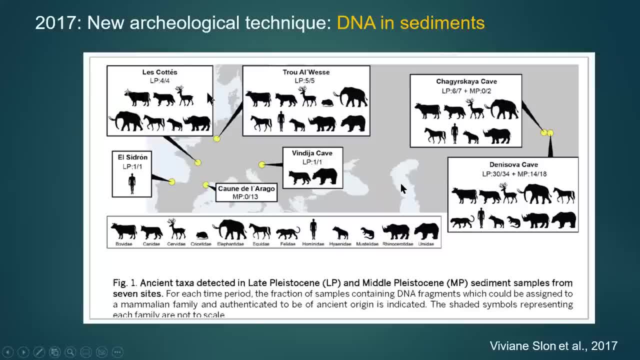 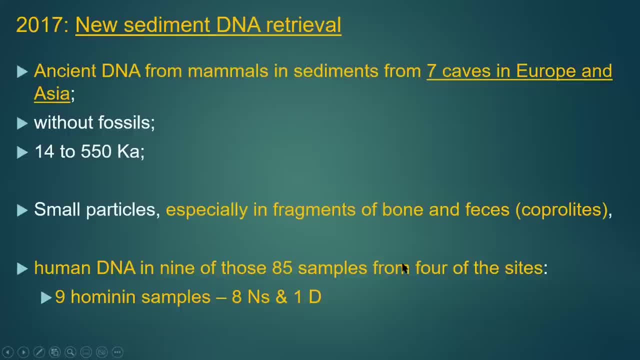 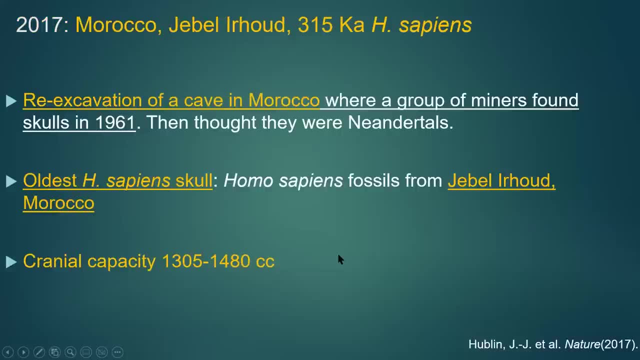 so just some amazing stuff in terms of dna, ancient technology. um, so they found nine hominin samples in this uh study, basically, and then in 2017, we get uh the morocco jebel erhud uh finding of the oldest homo sapien skull, uh dated to 315, so now it's the oldest uh modern human skull that we have. 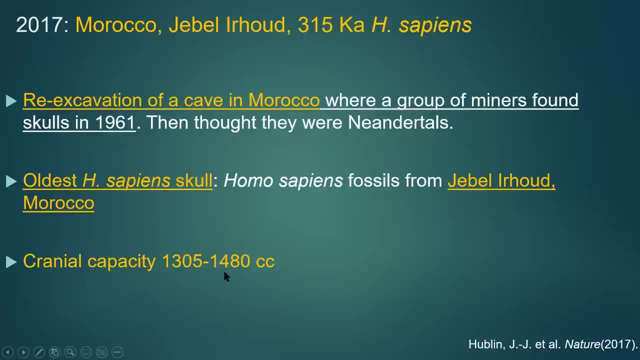 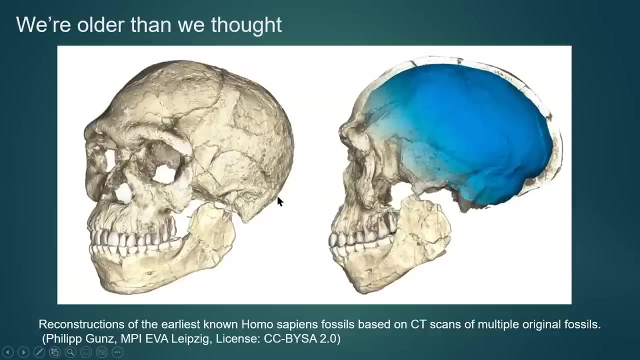 uh, the brain capacity is very large, equivalent to our own, even larger. so this is really. we have about 10 more minutes left. okay, sorry, i would like to suggest, if you've had any question, please email me. okay, so just, uh, i appreciate the time, but too much material. uh, this is what. 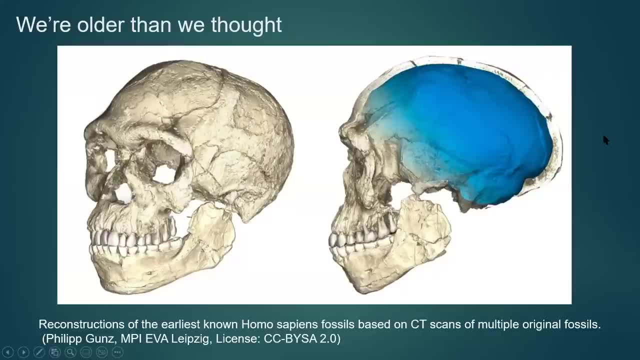 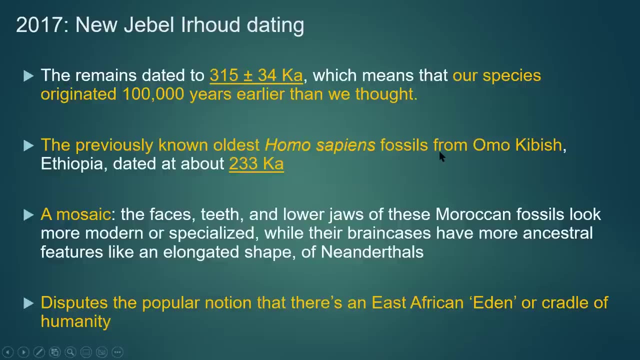 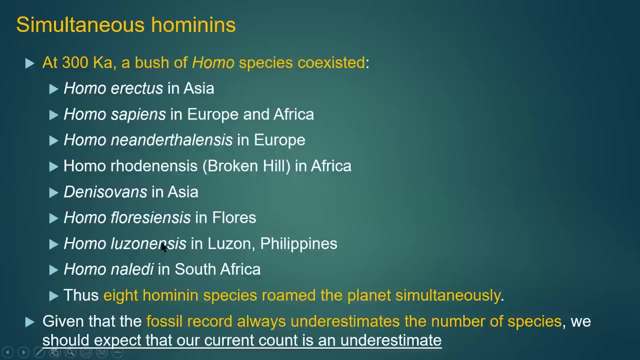 the face looked like very modern, but, interestingly, the skull looks much more like neanderthal. so we hadn't uh coalesced into our final form, but this is now, in morocco of all places, okay, uh, uh, the oldest modern human, um, and it's a mosaic again, of course, um, and at 300k we now have at least 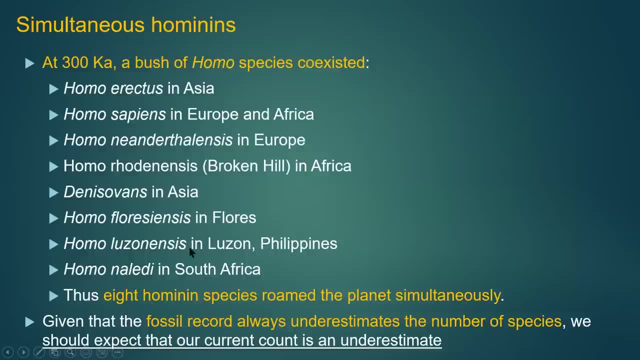 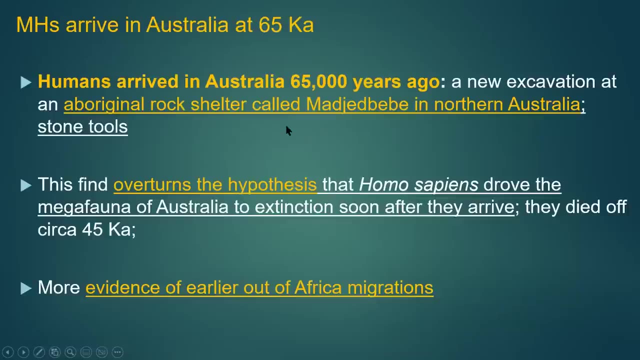 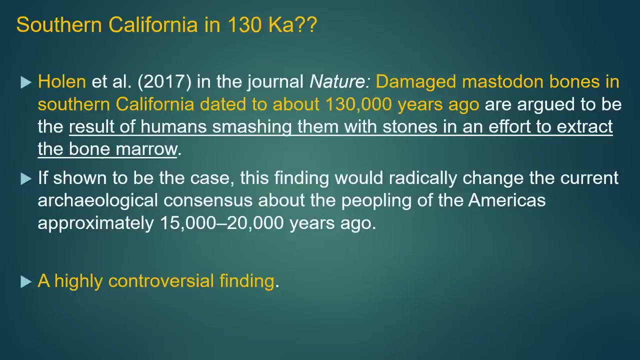 eight hominid species on the planet living together: okay, erectus sapiens, neanderthal, broken hill, denisovans, flow, luzon and naliti. okay, lots of characters out there. we get to australia by 65 000 years ago. controversial, highly controversial uh study that found damaged mastodon bones in santa. 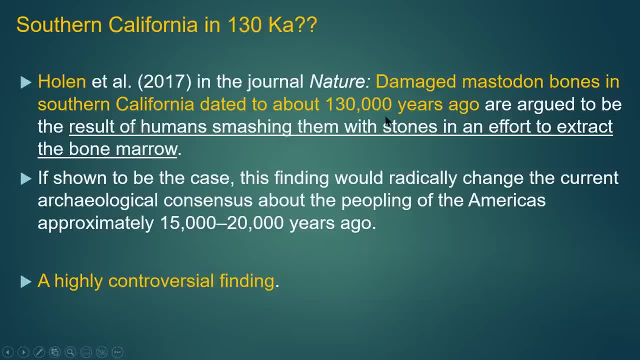 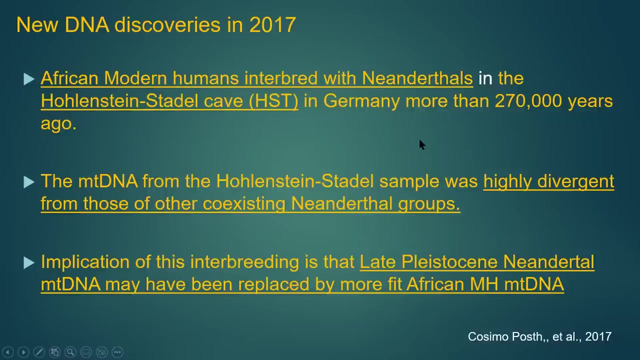 barbara, california, dating to 130k. uh. they insist that this represented, um, some hominin coming to america a hundred thousand years earlier than the standard 13k findings. okay, nobody accepts it. basically, um and uh. in germany they find a femur, uh and do the dna and discovered that it? uh is a neanderthal. 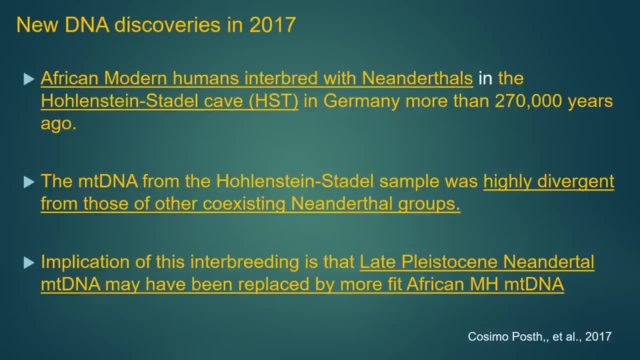 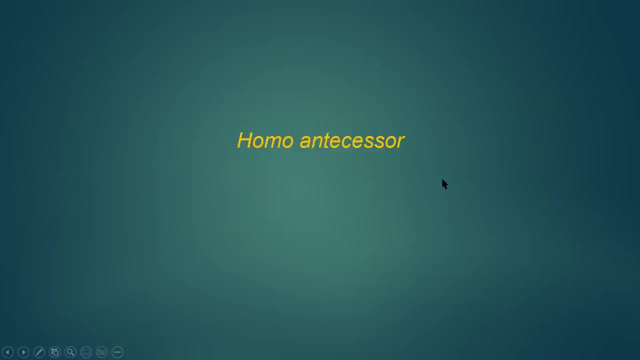 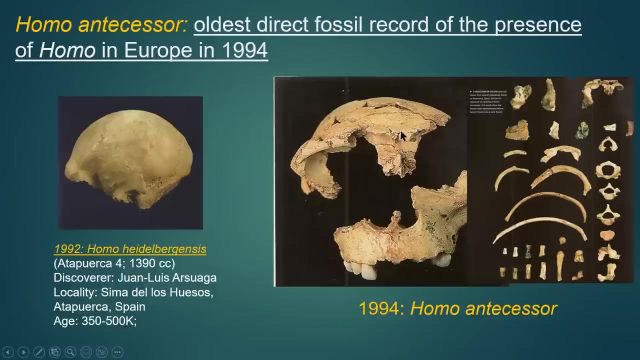 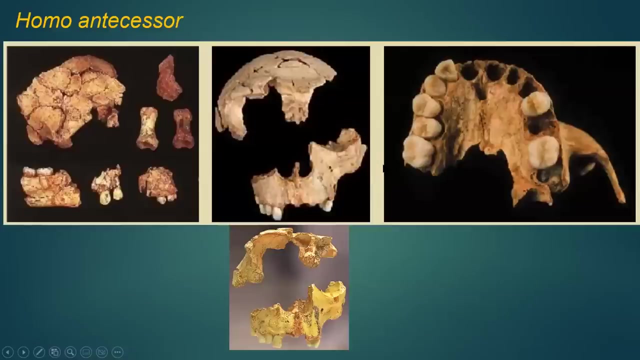 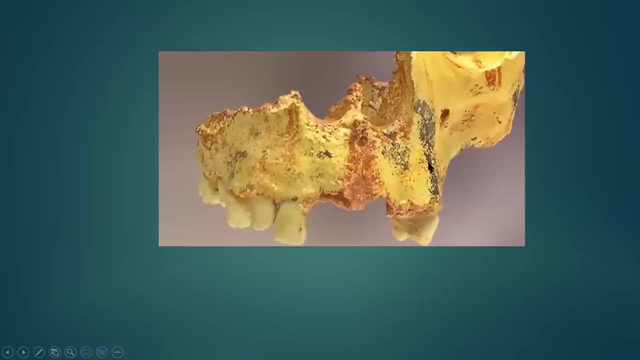 but the mitochondria is modern, human at 270k. all right, we'll discuss this a lot in the uh- paleo genomics. it's a an amazing study. okay, so we were in germany 270 000 years ago. i'm not going to go, we're making it up here. you're going to watch that video, um, on spotify. 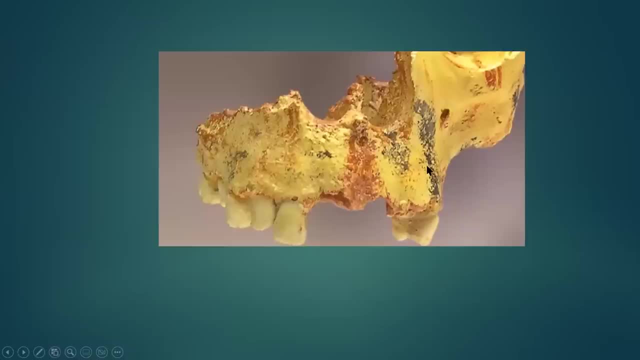 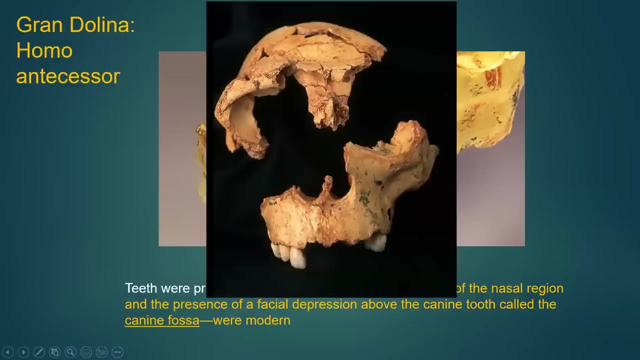 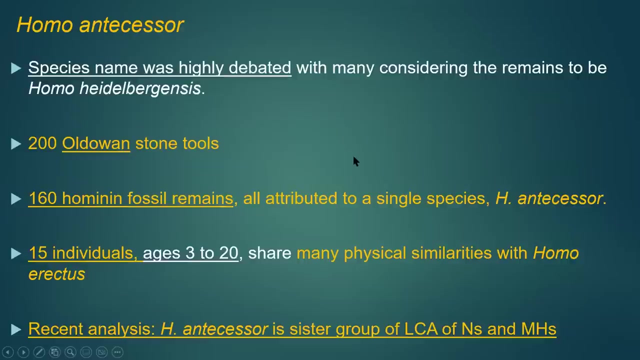 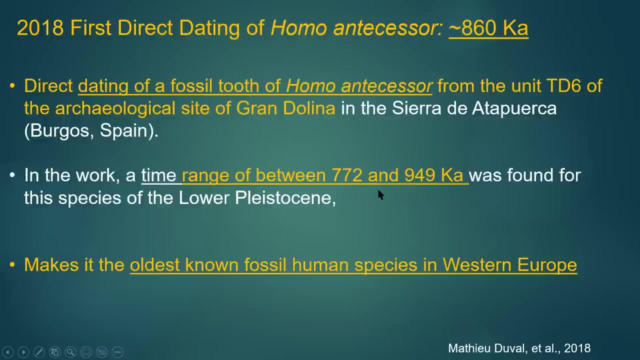 Chris Stringer now thinks that flat-faced like modern humans is the ancient version and that Neanderthals are the derived version. Okay, an interesting theory. but they're at the Gran Dolina area of Spain And they're finally they're with Oldowan tools, 15 individuals and eventually they do the dating and it turns out to be 770 to 950 or so. 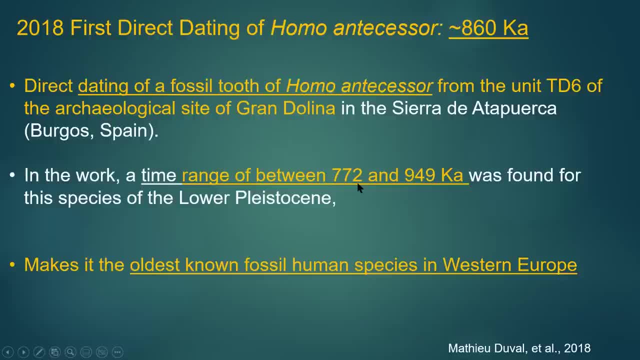 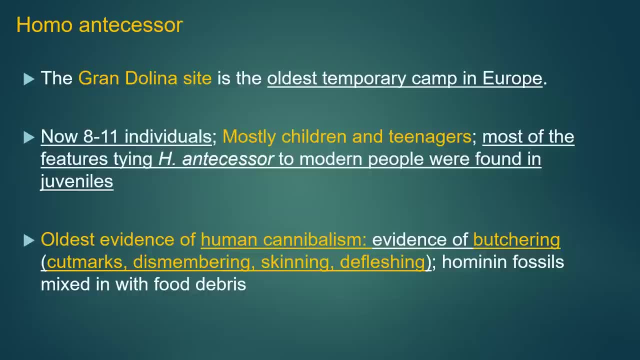 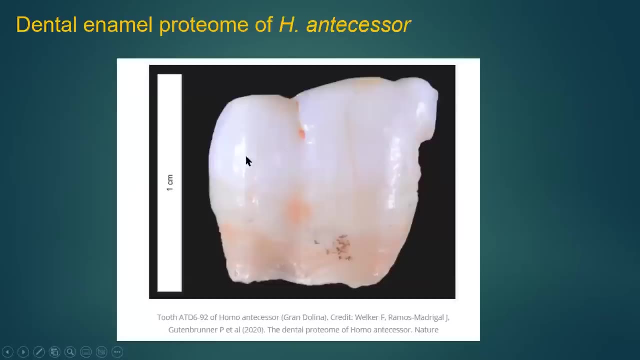 I'm sorry. Yeah, that's the dating range, okay. So among the oldest or close to the oldest Nearby, they discover a 1.4 million-year-old Nandibul that they think is also him, And they do some teeth, proteomes and fluid. 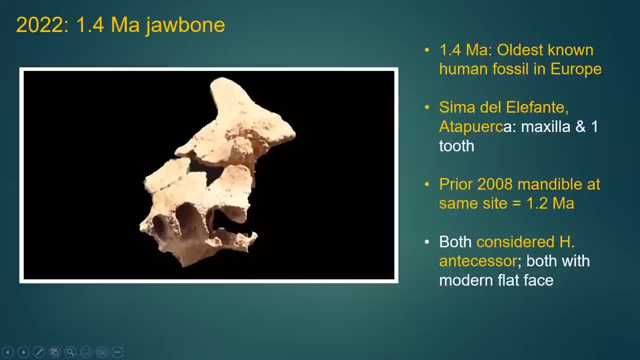 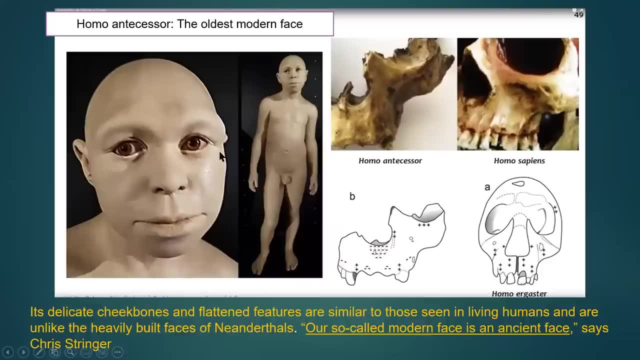 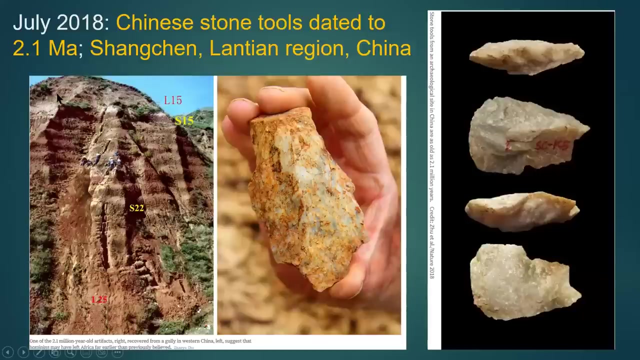 Old, old. This is the 1.4 million-year-old jawbone And they think he had an amazingly modern-looking face, basically from the bone structuring, So that Stringer thinks ancient, okay. They then discover that some species got to China at 2.1 million years, compared to the 1.8 demonica exit. 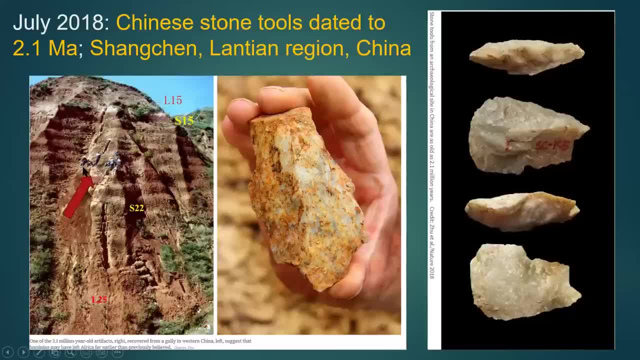 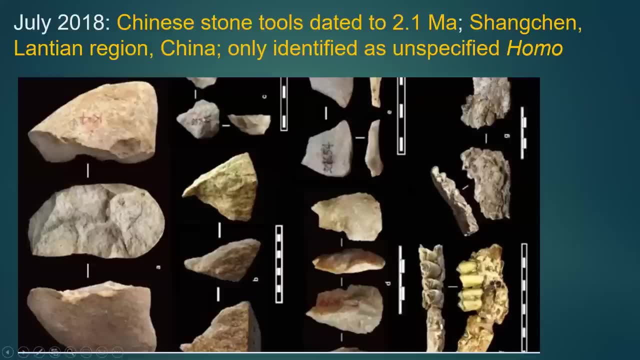 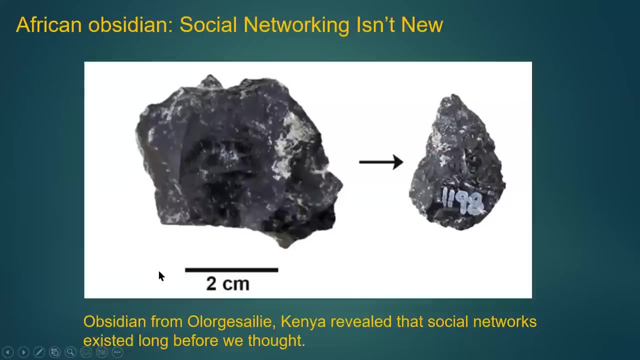 And this is where the site right here. right, They were high up there, But they do not identify the species of Homo that they think did this, but almost everybody thinks it had to be Erectus. They find that they are the original species of Homo. 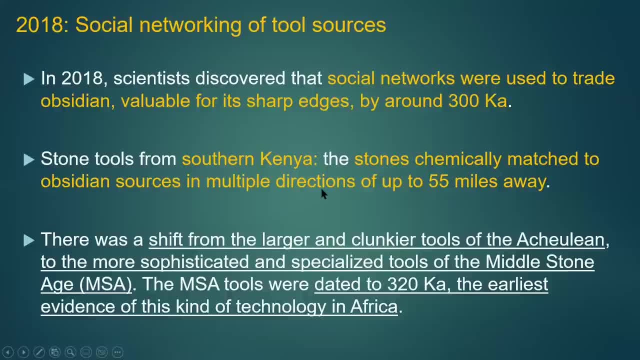 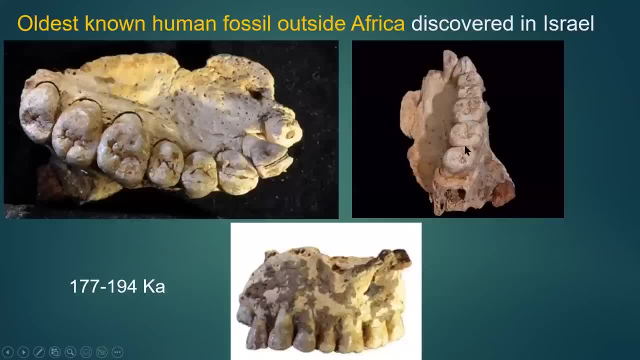 Find obsidian in Africa indicating social networking at more than at around 300K. This study- the oldest Israeli mandible from Ms Leah that we got out of Africa at this date, but much of these earlier exits are clearly dead ends- didn't quite make it. 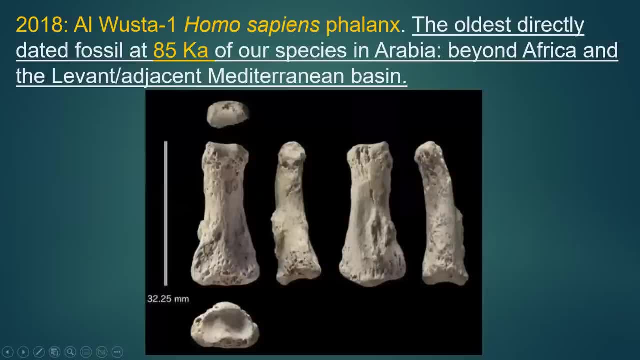 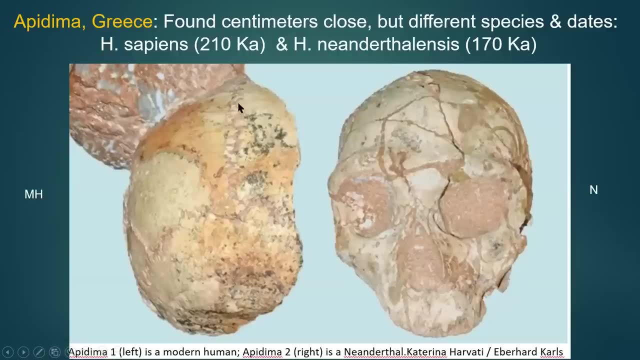 Arabia at 85K, bones, finger bones from 85K. We'll skip flowstones, Modern human and Neanderthal skulls right next to each other, probably due to a mudslide, But again in Greece, 210K, An earlier exit. 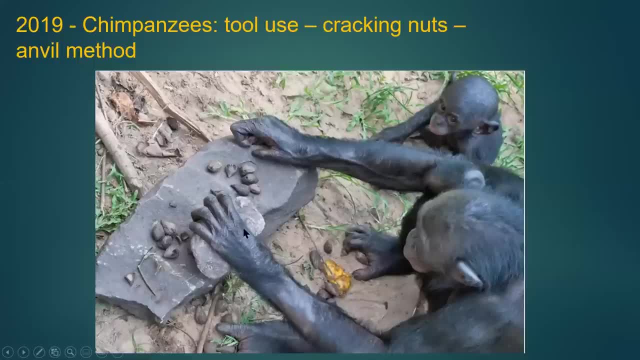 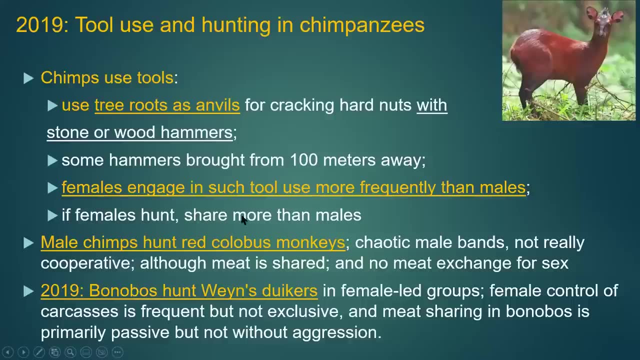 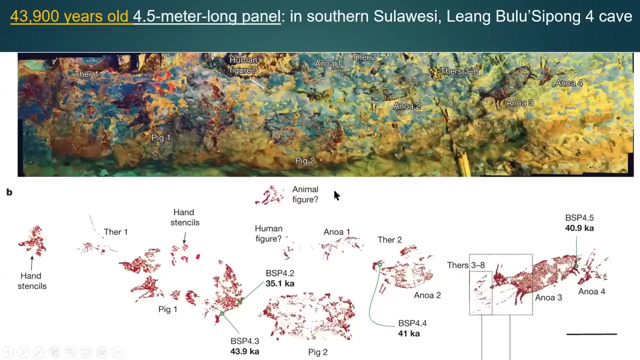 Chimpanzees use tools: anvil with a stone to crack nuts And turns out bonobos. hunt Wayans dukers, antelopes and chimps hunt Pelobus monkeys. So they're hunting and using tools, Okay. 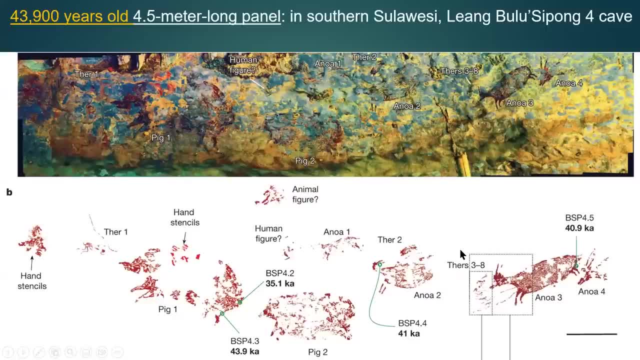 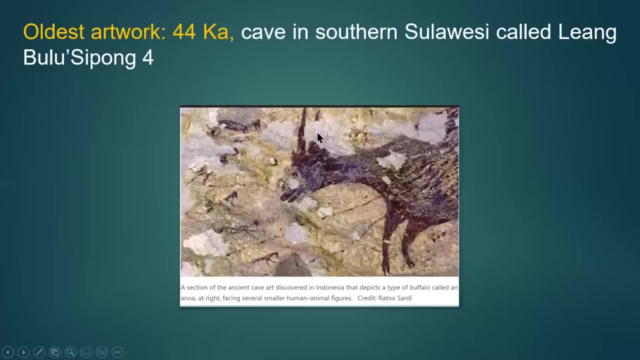 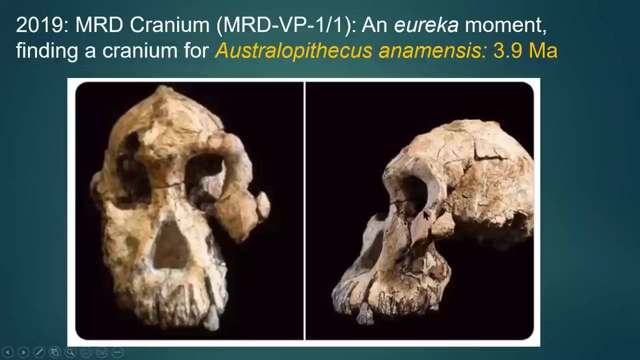 This is the oldest painting in the world at this point, A 43.9 thousand year old. in a Indonesian island with sort of antelope, pig creatures dated- We've said this one- They discover a full cranium of anamensis, which is potentially 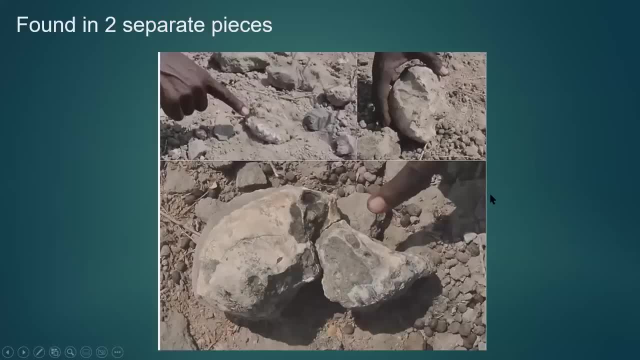 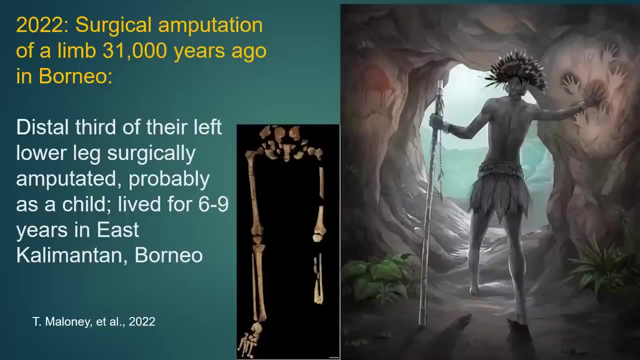 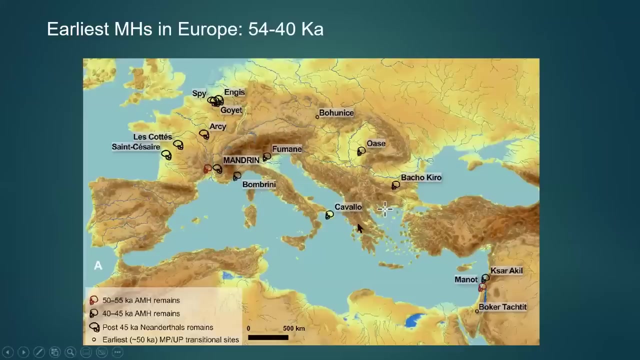 A related to Opharensis. We'll skip this guy. Okay, Data of a successful leg amputation at 31K in Indonesia And then the discovery at Mandarin cave in France That there were Layering of a musterian stone tools, then arrowheads, modern humans, then musterian stone tools, meaning at 54K. we were in Europe for a short periods in this study. 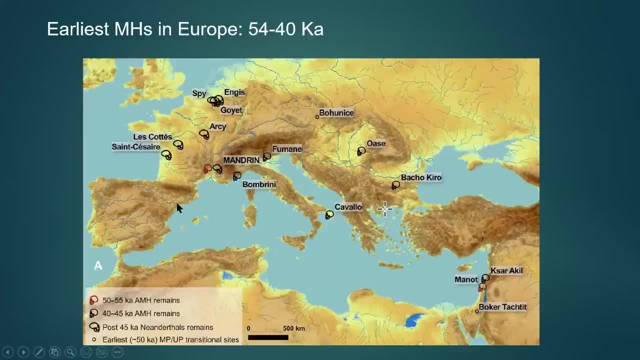 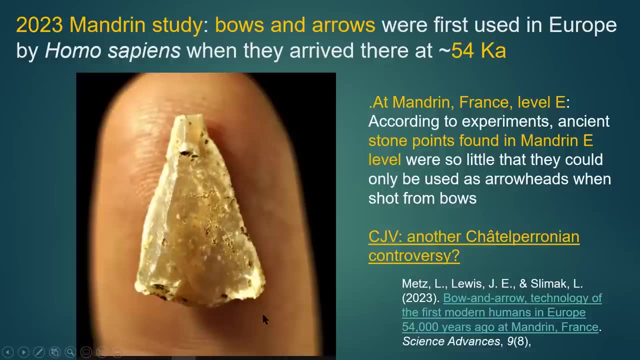 And then, a few months later- just a month ago- they, the stone tools, were these microscopes. And then, a few months later, just a month ago, they, the stone tools, were these microscopes. And then, a few months later, just a month ago, they, the stone tools, were these microscopic arrowheads in the same layer, at 54K. and they are claiming that modern humans introduce, used bow and arrow. 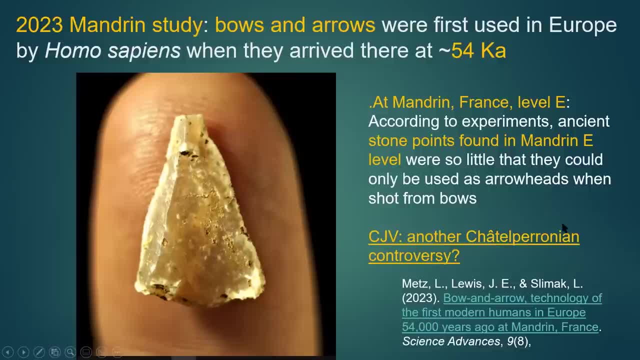 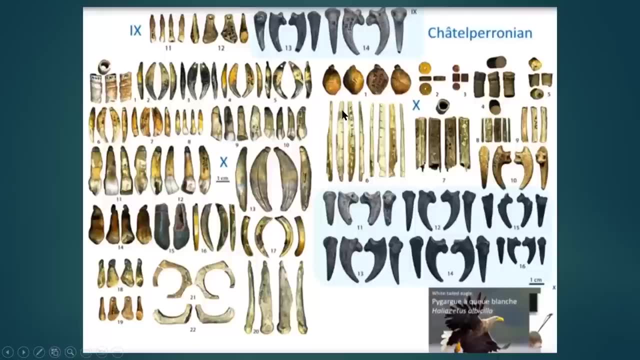 At this site, At this site. for me this is like the shot At this site: 合 w Q, W, Q, Q, W, W, Q, W, W, Q, W Q Q that they were Neanderthal and discrimination against Neanderthal, Upper Paleolithic behavior. basically. 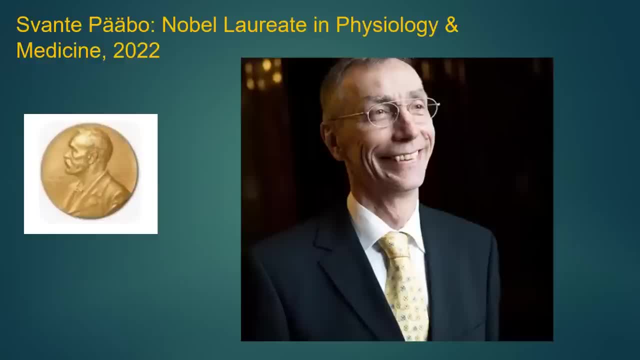 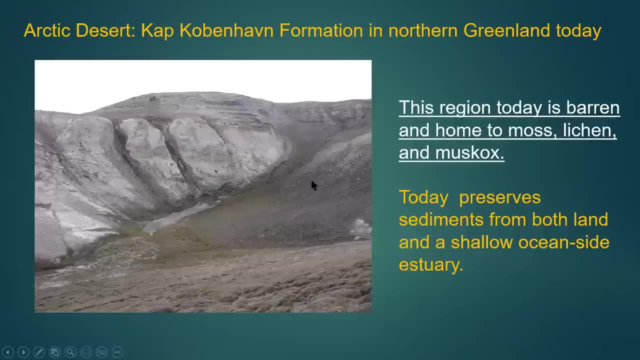 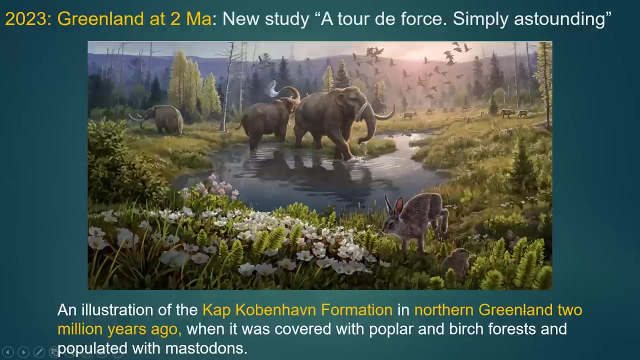 Okay, Paolo gets the Nobel Prize last year for his ancient DNA work. And the last thing: Arctic Desert and the Copenhagen Formation in Greenland And they basically this is 2 million years old and they are basically taking sediment DNA. at 2 million years they're able to totally reconstruct. 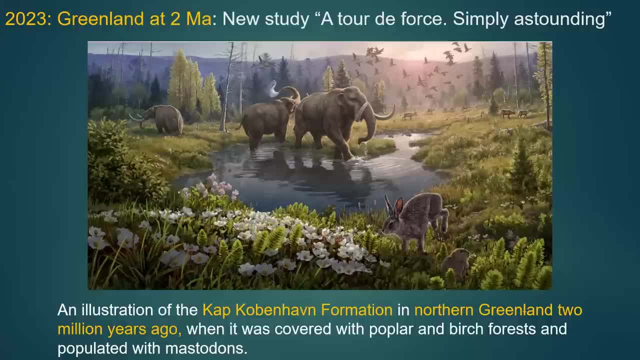 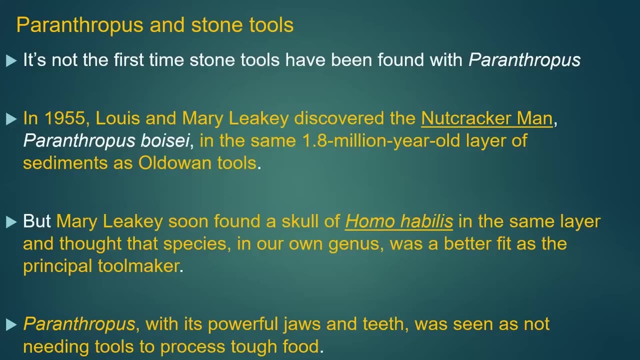 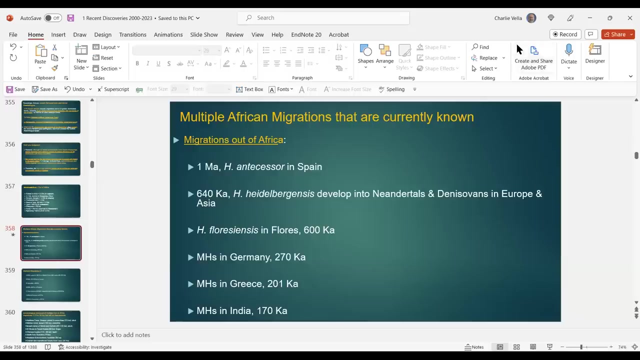 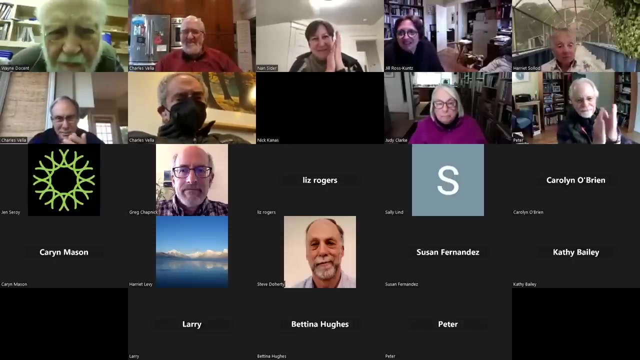 what it looked like in a warmer climate, when rabbits, plants and mastodons were populating this area, based on 2 million year old DNA, And we'll, I think, call it at that. Way too many slides, All right, Yay, thank you Charlie. 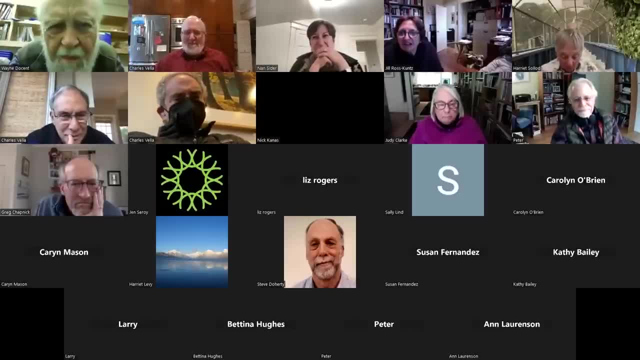 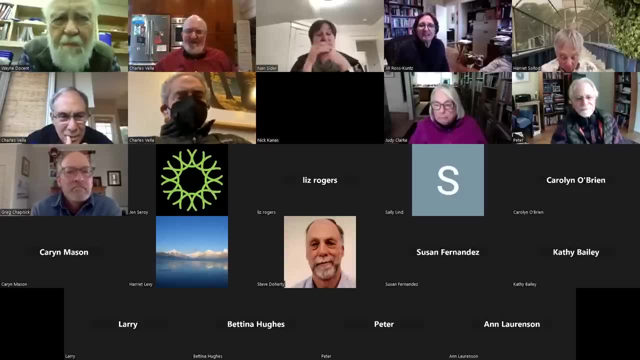 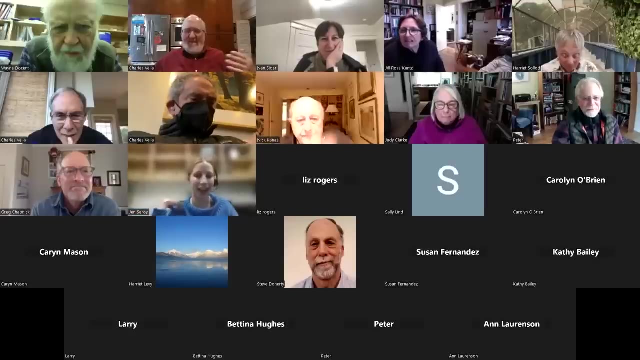 I'm trying to find where my picture is, but I'm here. Does anyone have any last? There I am. Any last questions or anything? Just a couple more minutes. As I said, there was too much material And if you have any questions about any of it, email me. 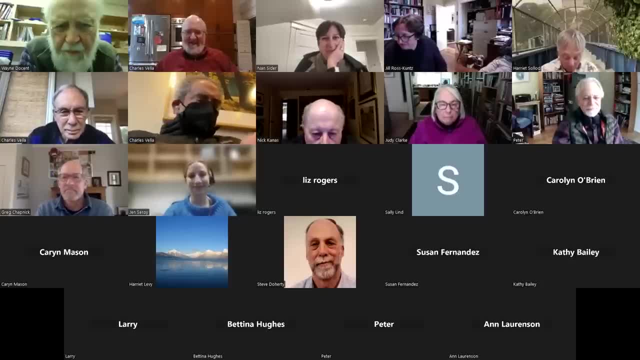 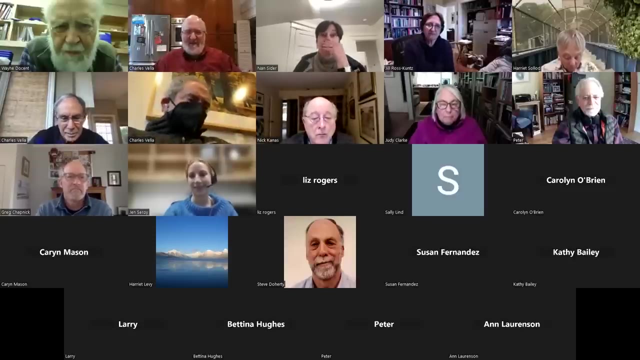 Okay, Charles Vela, at comcastnet, I'm willing to talk to any of you And, as I said, there's simply too much material. So if you're interested in doing two more sessions again, maybe the last Monday of the month, 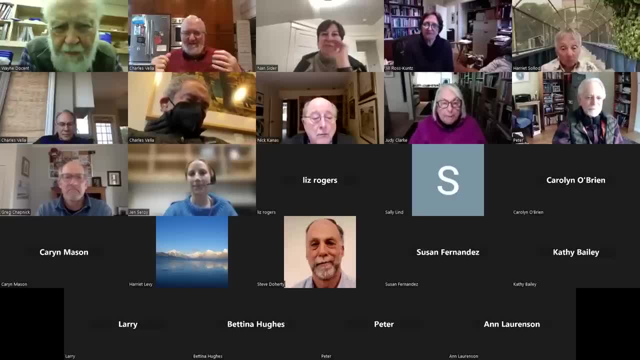 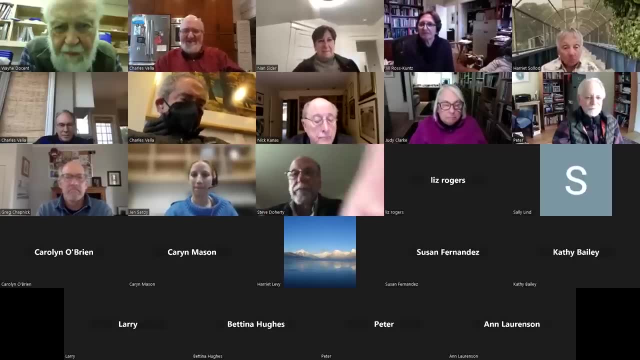 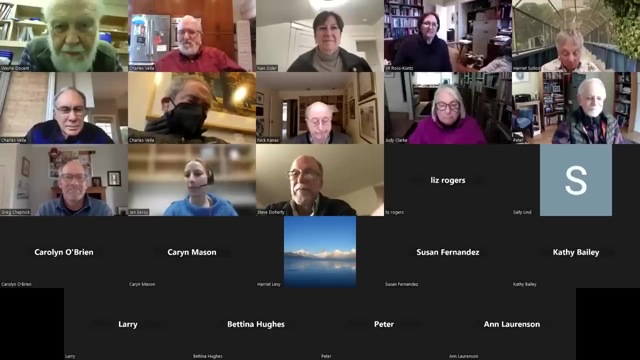 for the next two months. I'm perfectly willing to do it. Simply email me, Tell me your interest and I'll set it up, basically. Otherwise, any immediate questions? All right, People are just saying thank you in the chat. Thank you, thank you.